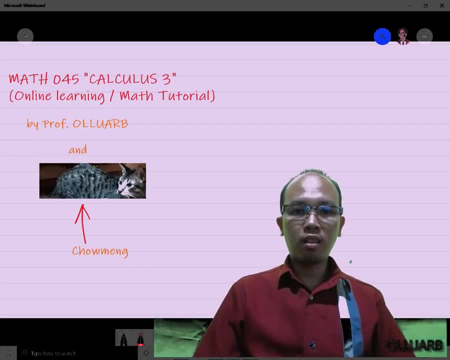 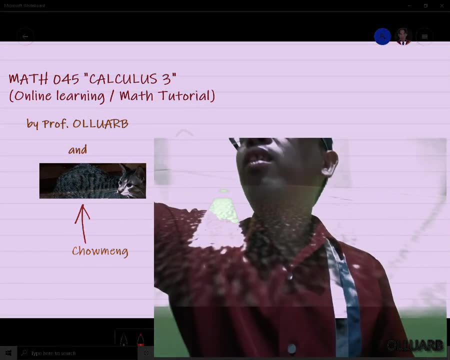 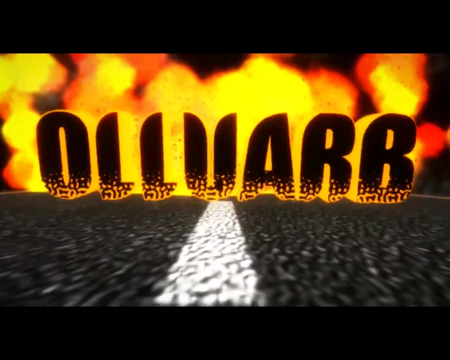 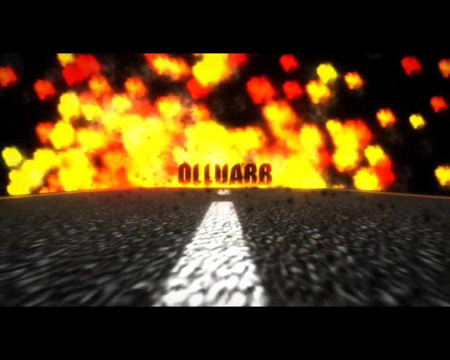 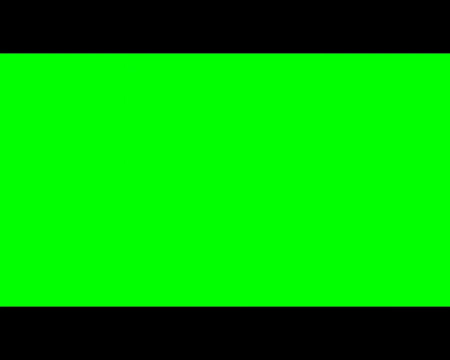 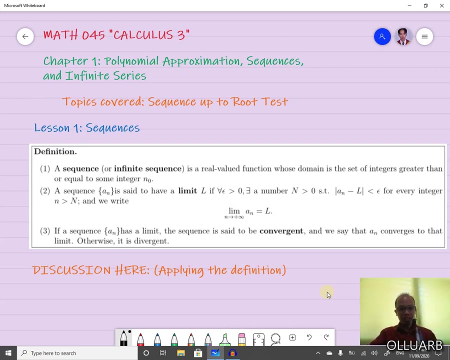 Hello everyone, welcome to this lecture video tutorial in calculus 3.. Enjoy learning. Hello everyone, welcome to this online class: Math 45, calculus 3.. This lecture video discusses all the topics in chapter 1 of calculus 3 entitled, as you can see here, polynomial. 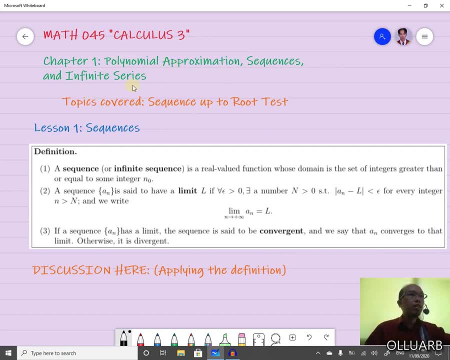 approximations, sequences and infinite series. However, I am going to divide the topics into two parts: The first part I will be discussing sequence up to root test, and then the second part is from power series up to binomial series. So, without further delay, let's start the session. 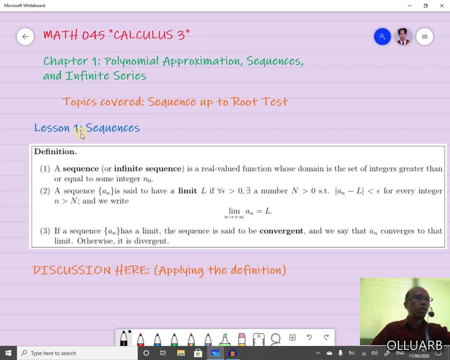 Lesson 1.. As you can see here, our lesson, the title of our lesson, is sequences. So before I am going to explain to you the definition, first let me remind you that this topic, the first topic entitled sequences, is very important in the whole chapter. 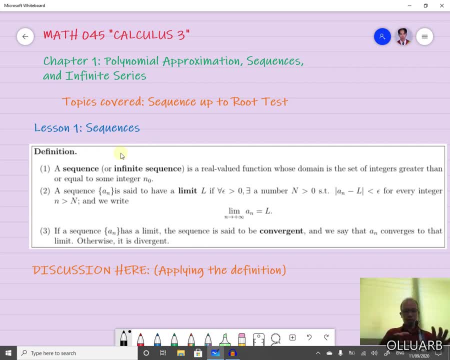 Why? Because, as you can see sequences, Why, if you don't understand the meaning of the sequence, then all would be meaningless. uh, you will not be able to understand what. what is infinite series? what is? uh, what do we mean by polynomial approximation? so all of that, so meaning to say, if you don't understand it, please uh repeat. 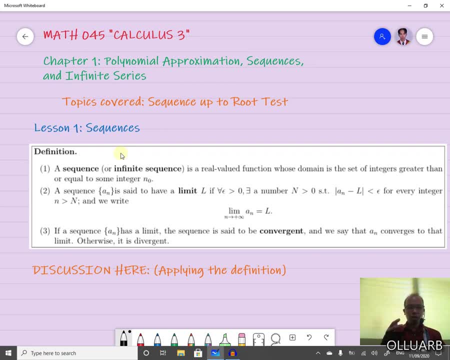 it again, and again, and again until, uh, you comprehend the idea of what it means to be a sequence. okay, so let's start. okay, a sequence, it says here in definition one, as you can see here, you can see here, definition one- a sequence or infinite sequence is a real valued function. 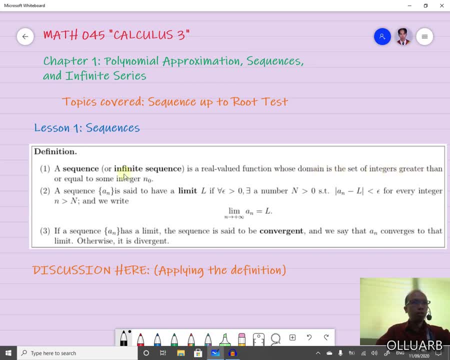 whose domain is the set of integers greater than or equal to some integer and not notice that some books, uh, they, they define it as a sequence- is a real valued function of domain is the set of positive integers. but i prefer to to choose this definition because, uh, as you can see, there are 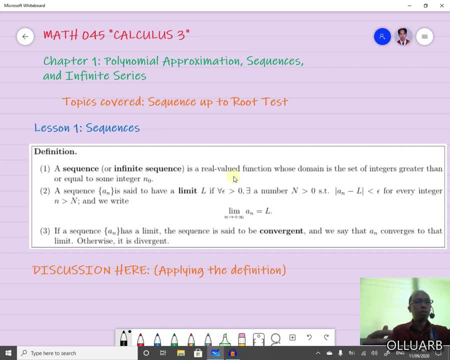 and in the in the next topic, when you talk about infinite sequence, they will uh, start at: n is equal to one, or maybe n is equal to two, four and so on and so forth. so that is why i write here. it will start at some integer and no notice. also the, the, the sequence is a function and the domain 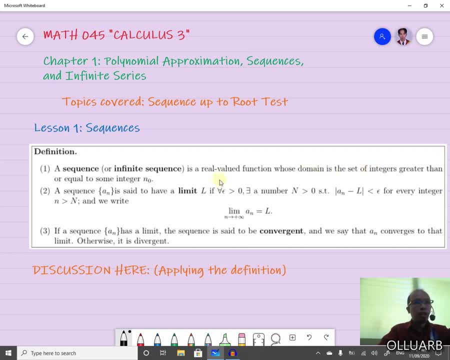 is the set, okay, so let's forget about this one, the domain, and so on, so forth. uh, let's focus on the keyword here, which is the domain, and so on and so forth. uh, let's focus on the keyword here, which is the word function, so forget about real value to understand the definition of a function. 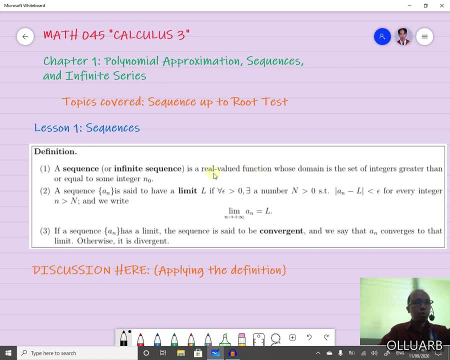 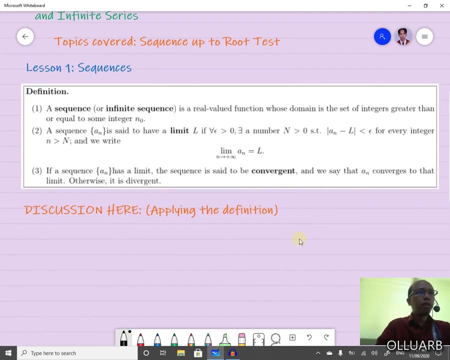 then later on, it's very easy to understand what do we mean by real valued function. okay, so, as the key word here is: uh, as you can see, a sequence is a function, it is a function. so what do we mean by a function? so, as you can see here, 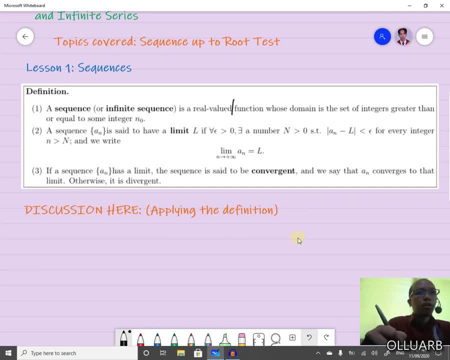 uh, sorry, i will try to put a color red. okay, so the keyword here is a function. so if you try to recall your algebra class, trigonometric class or pre-calculus class or basic calculus class, uh, a function. so let's uh try to recall this recall. 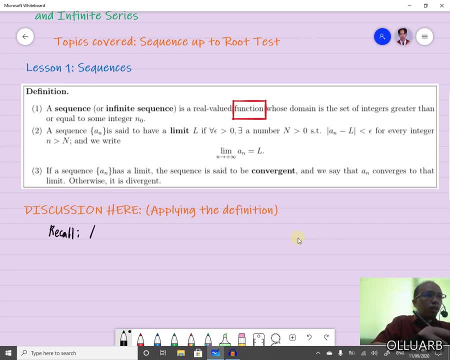 so from this a strike color red, a function is a rule that assigns to each element x, small x- in the domain one and only one, element y, one and the element y in the co-domain. okay, so in the icon you have element y. there is a two elements: element element type, and there is a element element relationships, coded data, element言 steps, and that means we, you know if an element- there's one at the top of the screen, and that means available as a column 1. this is what is he. your domain can be registered in your domain. so you have told already, given growth, so you save it. that's quite simple, isn't it? 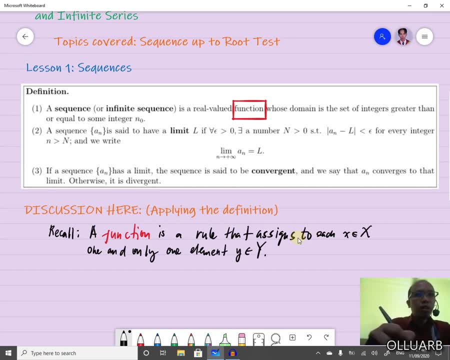 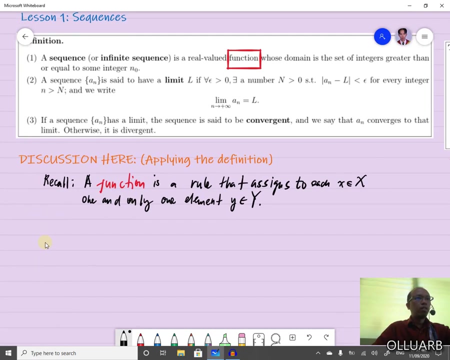 me okay. so our small y here and small x are notation for element and the big x and the big y is impatient for a set. so if you recall your, if you recall your algebra or trigonometry class says there that this is the the meaning of a function and, as you can see here, it's not clear. 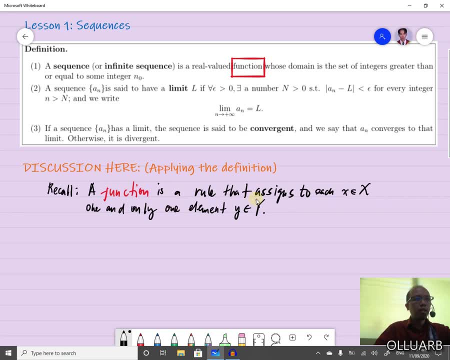 again, it is a rule that assigns. so what do we mean by that? okay, so what we will do here is: we will try, i will try to explain to you in layman's term. okay, there are, in order for you to understand the, the definition of a function. let's try to understand this by some, by describing it, or. 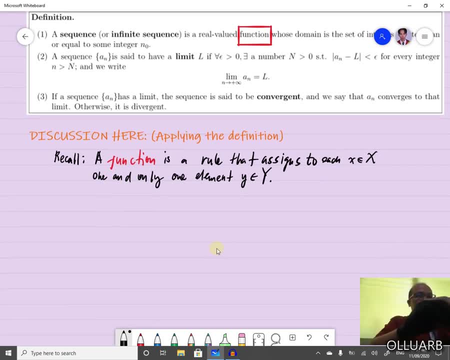 by visualizing it. so there are. so we are not talking here about sequence. first let's try to understand the word that, the word function. there are four ways on how to describe or visualize. visualize a function. okay, so if you remember, the first one is using diagram. I know you are familiar with this diagram, or mappings. 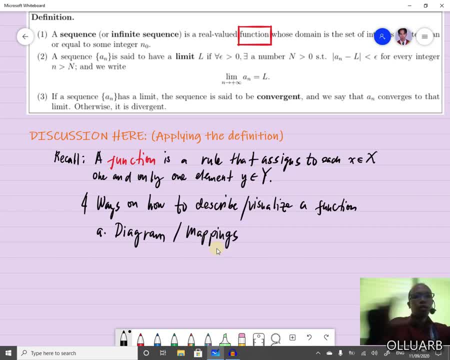 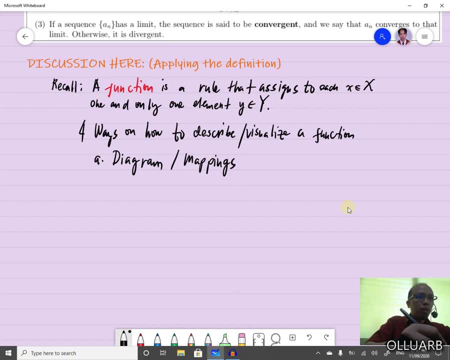 sorry, mapping okay. so I know you have an idea. now let's try to make a diagram. is with my diagram? Yes, I have a diagram. we just marked it, just pop out once again. marked: triviye changed an oblong, now the perfect oblong, that one. 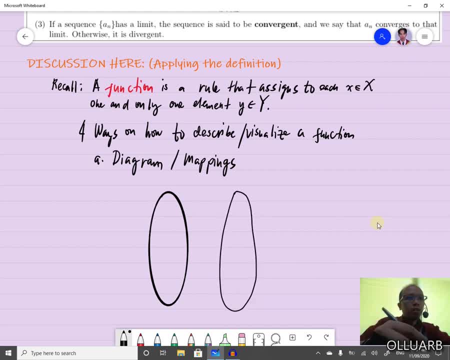 again. that's. I'm sorry this wait, oh, what happened? I think I have to copy this one. first make a copy and then paste, paste, control, paste that one. okay, then I'm going to drag here. I'm sorry I wasn't able to make perfect. okay, then I'm going to drag here. I'm sorry I wasn't able to make perfect. 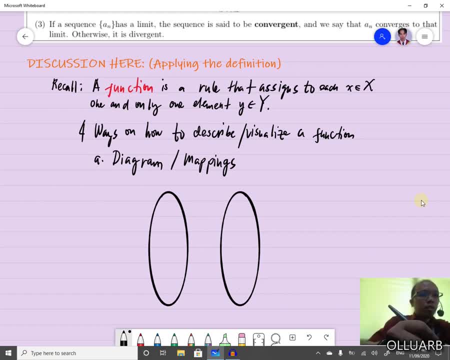 okay, then I'm going to drag here. I'm sorry I wasn't able to make perfect. okay, this is a diagram. as you have noticed here, this is our try. another color, that's a blue. this is set X and set Y. okay, and then we have a mapping. 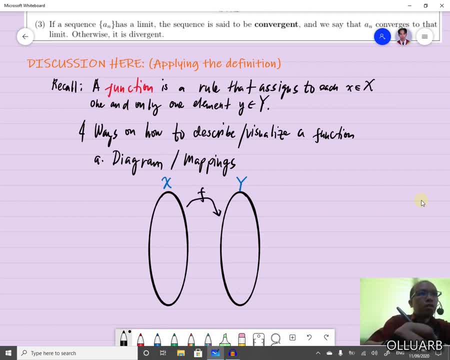 here let's denote this as F. and if you have an object, let's say negative 3, 2. here let's denote this as F, and if you have an object, let's say negative 3, 2. here let's denote this as F. and if you have an object, let's say negative 3, 2, 1, 7, 11 or 12, and then on the codomain. 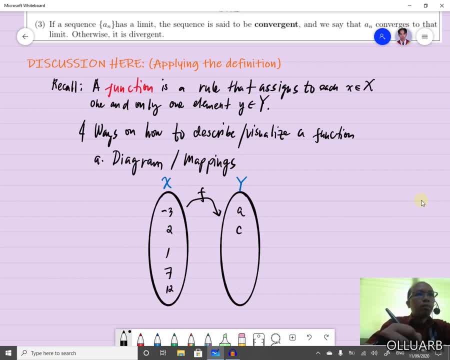 1, 7, 11 or 12, and then on the codomain: 1, 7, 11 or 12, and then on the codomain: I have a C C 5: okay, that one, there are four. I have a C C 5: okay, that one, there are four. 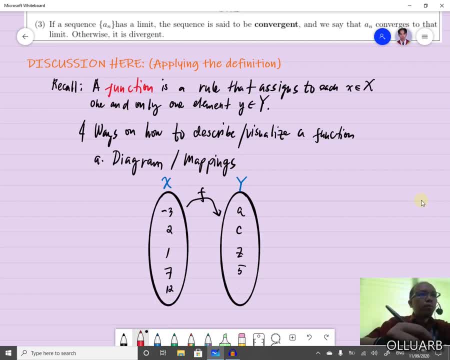 I have a C, C 5, okay, that one. there are four limits. so when you see in diagram limits, so when you see in diagram limits, so when you see in diagram and we say: when you see a function it, and we say when you see a function it. 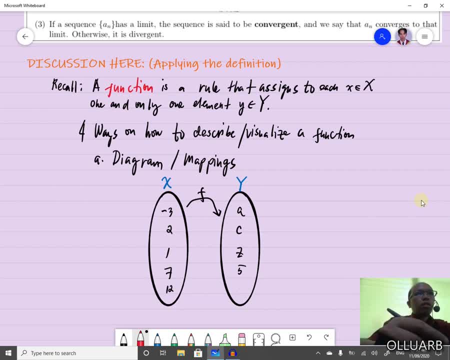 and we say: when you see a function, it says that the word there is. it is a. says that the word there is. it is a says that the word there is. it is a rule. it is in rule that assigns to each rule. it is in rule that assigns to each. 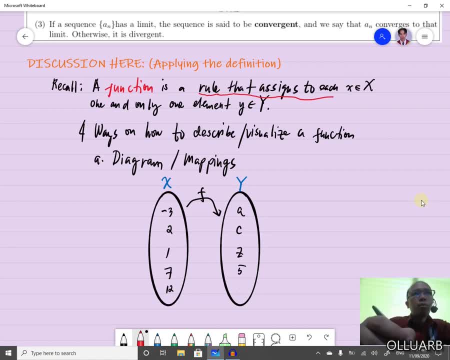 rule. it is in rule that assigns to each each mean to say every element of the. each mean to say every element of the. each mean to say every element of the domain must be map to one and only you. domain must be map to one and only you. 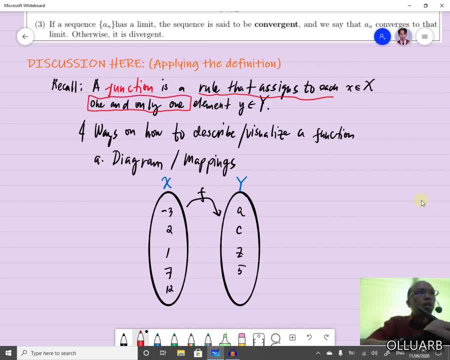 domain must be map to one and only. you can see the key where there is one and can see the key where there is one, and can see the key where there is one and only one and only one element. so means a: only one and only one element. so means a. 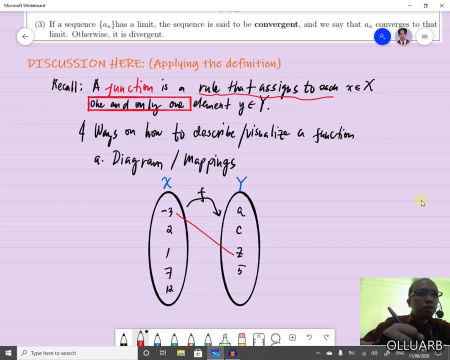 only one and only one element. so means a sample example. we have three. is map to sample example. we have three. is map to sample example. we have three. is map to you, you, you. your tool is not to see, one is not to. your tool is not to see, one is not to. 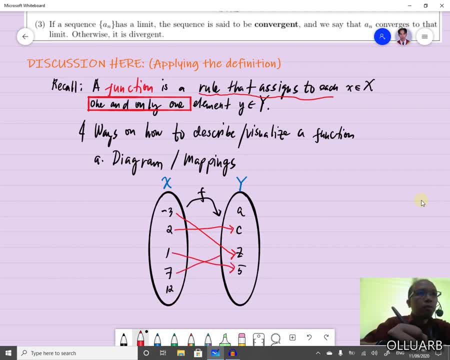 your tool is not to see. one is not to find your seven is not to see again. find your seven is not to see again. find your seven is not to see again. your job is not to let her see so as you. your job is not to let her see so as you. 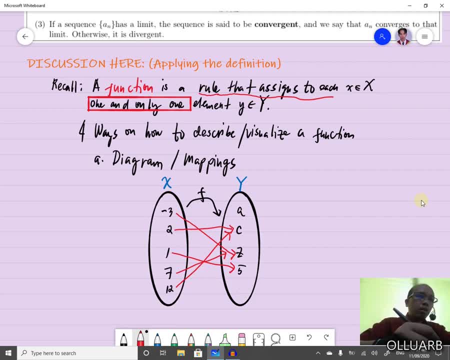 your job is not to let her see. so, as you have noticed here every element, every have noticed here every element, every have noticed here every element, every element in the domain is map to one and element in the domain is map to one and element in the domain is map to one and only only one. 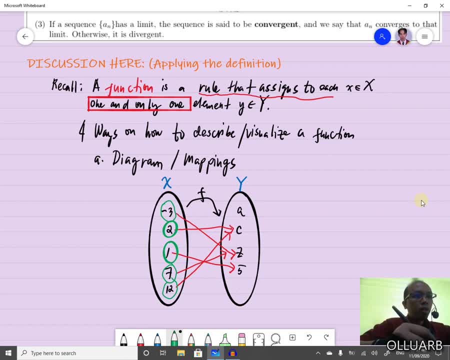 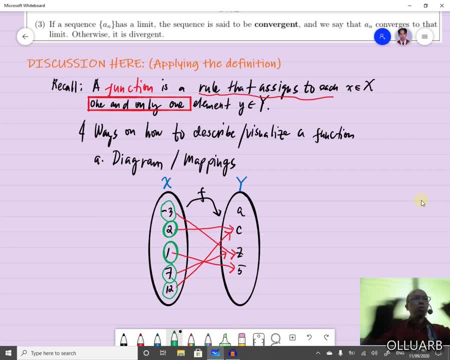 each object here. this means that it is a each object here. this means that it is a function okay. so what will happen if function okay? so what will happen if function okay? so what will happen if there's more than an arrow, if there's there's more than an arrow, if there's? 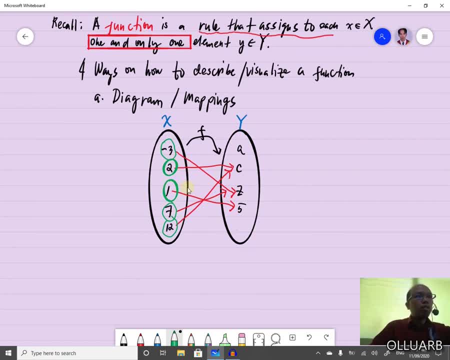 there's more than an arrow, if there's more, more arrows in here, this means that more more arrow in here, this means that more more arrow in here, this means that this is not a function anymore. okay, so, this is not a function anymore. okay, so, this is not a function anymore. okay, so the other term that for that is a. 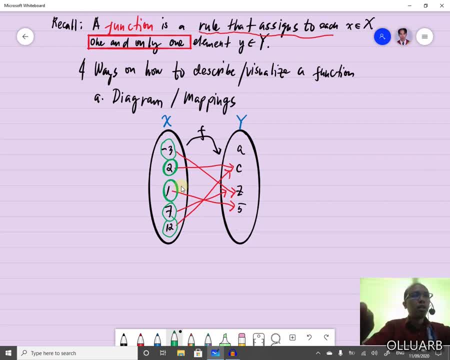 the other term that for that is a. the other term that for that is a relation. so remember in your algebra and relation. so remember in your algebra and relation. so remember in your algebra and regularity class we have, she remember if. regularity class: we have, she remember if. 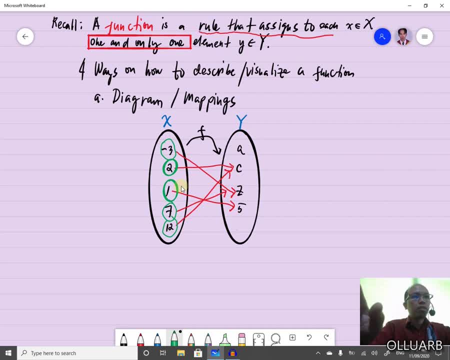 regularity class we have, she remember, if there is two or more mappings, more there is two or more mappings, more there is two or more mappings, more. arrows here, my arrows here. this means: arrows here, my arrows here. this means arrows here, my arrows here. this means that it is now called a relation. okay, so, 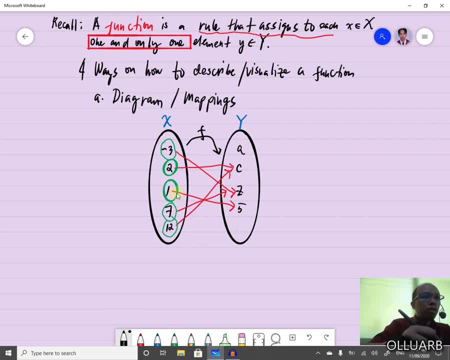 that it is now called a relation. okay, so that it is now called a relation. okay. so then notice that the domain the this is. then notice that the domain the this is. then notice that the domain the this is the domain here and the other one is this: 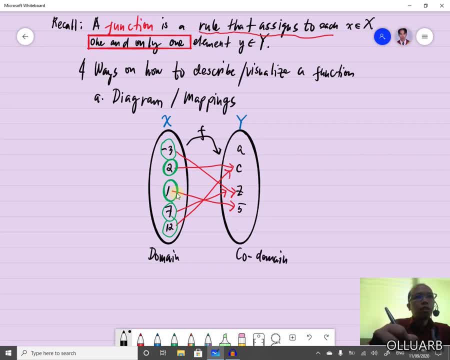 the domain here, and the other one is this the domain here, and the other one is: this is the crew, is the crew is the crew domain, and the other one is: this is the crew domain and the other one is: this is the crew domain. okay, for this sample for. 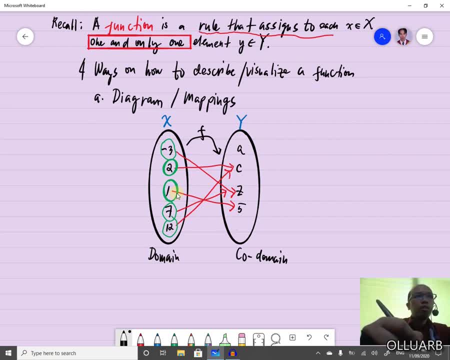 domain. okay for this sample for domain. okay for this sample for this example. and the. the domain here, which is this example, and the. the domain here, which is this example. and the. the domain here, which is X is hand and element negative. X is hand and element negative. 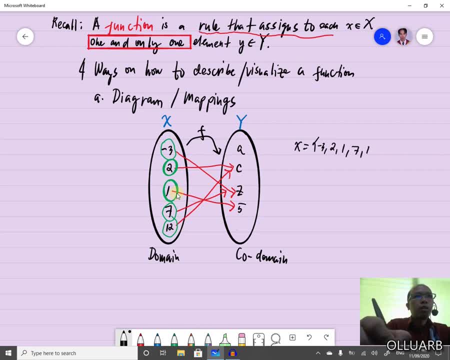 X is hand and element negative: three, two, one, seven and job. whereas the three: two, one, seven and job. whereas the three: two, one, seven and job. whereas the codomain had the element a codomain had the element a codomain had the element a, C, Z and 5 and the range of this function. 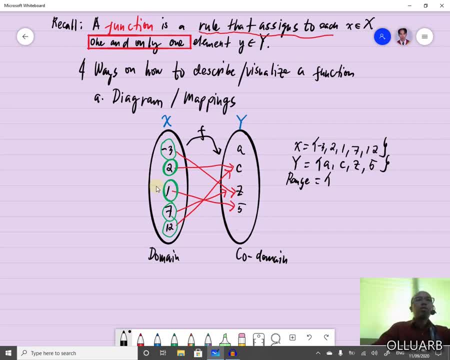 C, Z and 5 and the range of this function- C, Z and 5 and the range of this function- are those objects in the codomain that are those objects in the codomain. that are those objects in the codomain that is, map that has an arrow or meaning to. 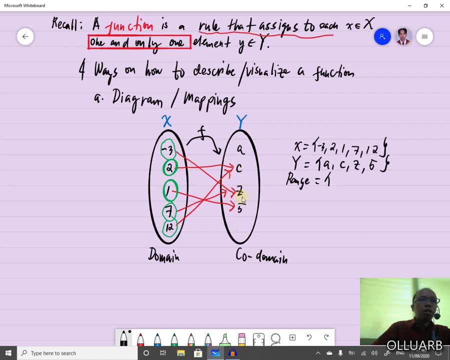 is map that has an arrow or meaning to. is map that has an arrow or meaning to say: notice here: only C, Z and five say: notice here: only C, Z and five say: notice here: only C, Z and five are map to every element in the codom, in the. 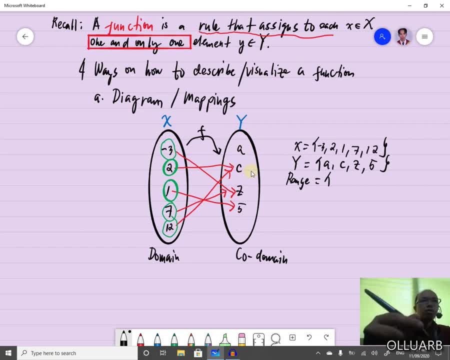 are map to every element in the codom in the. are map to every element in the codom in the domain. so mean to say a is not domain. so mean to say a is not domain. so mean to say a is not included. so a letter a, or the object a is not. 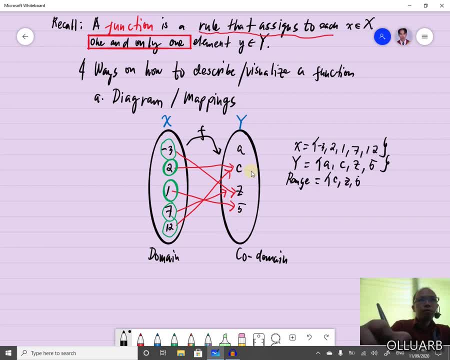 included. so a letter a or the object a is not included. so a letter a or the object a is not part of the it's not part of the part of the it's not part of the part of the it's not part of the range of this function. so please remember the. 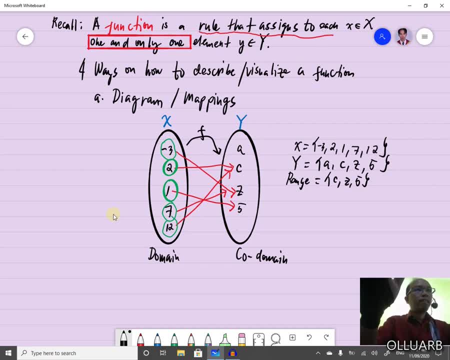 range of this function. so please remember the range of this function. so please remember the domain data, the. this remember the. the domain data, the the. this remember the. the domain data, the. this remember the the. how the function is visualized using. how the function is visualized using. 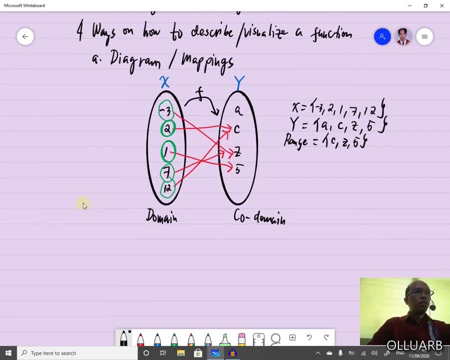 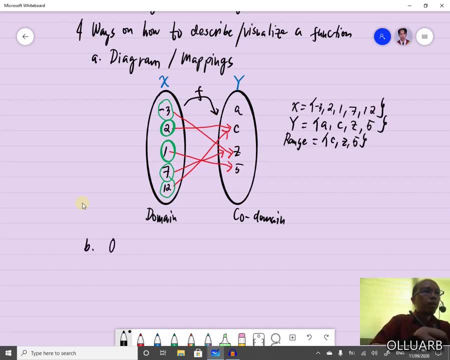 how the function is visualized using diagrams and or mappings. the second one diagrams and or mappings. the second one diagrams and or mappings. the second one, if you remember, is through ordered pairs, if you remember, is through ordered pairs. if you remember is through ordered pairs, ordered ordering pairs. okay, so for. 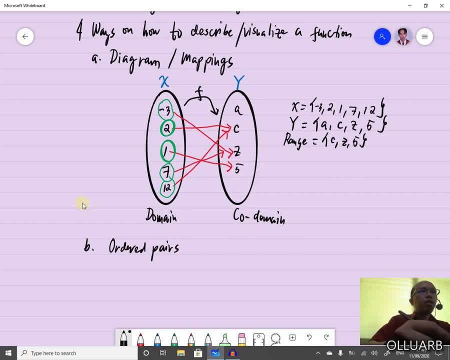 ordered ordering pairs: okay, so for ordered ordering pairs: okay. so, for example, this one, our division, our example. this one, our division, our example. this one, our division. our notation here is F for this example. our notation here is F for this example. our notation here is F for this example. our function is this: if we describe using 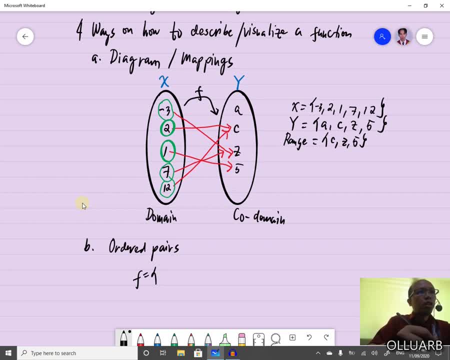 function. is this: if we describe using function, is this: if we describe using ordered pairs in, as you can see, this will ordered pairs in, as you can see, this will ordered pairs in, as you can see. this will be the elements. are this one negative? be the elements. are this one negative? 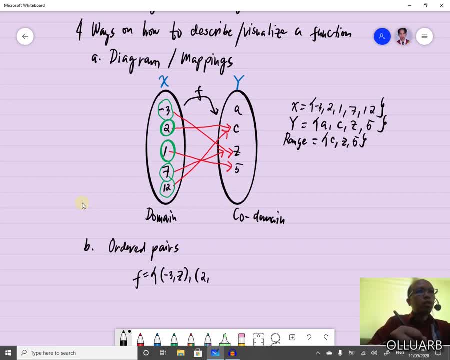 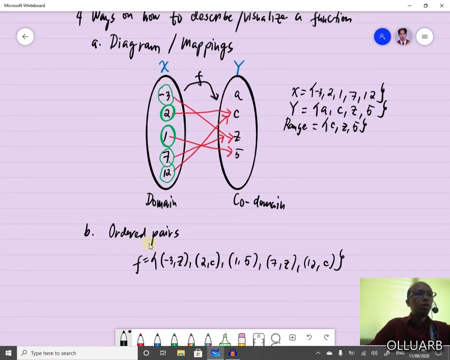 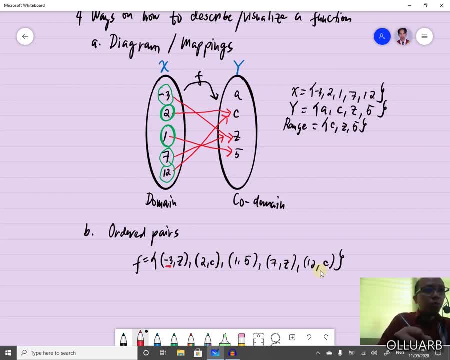 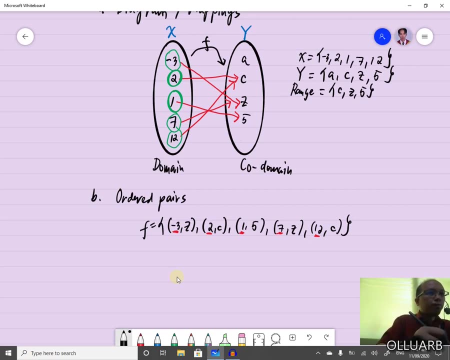 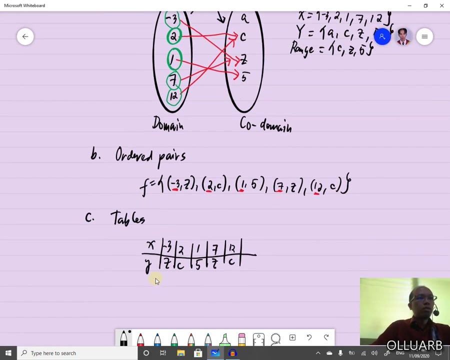 subject no two, first component, are the same. so that is a function, okay. the third one is using tables. tables. so, for example, if you have this one, that this is our X and Y, this example, here, as you can see, we have negative 3 Z to C, 1, 5, 7 Z and 12 C. so if you are going to describe the function using 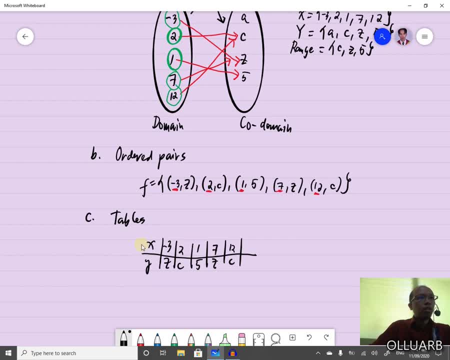 tables or tabular description of a function. the function using tables or tabular description of function. a function using tables or tabular description of a function. as you can see here in the upper part, no two first are no two object here are repeated: okay, so that that's what it means to be a function. the last one is: 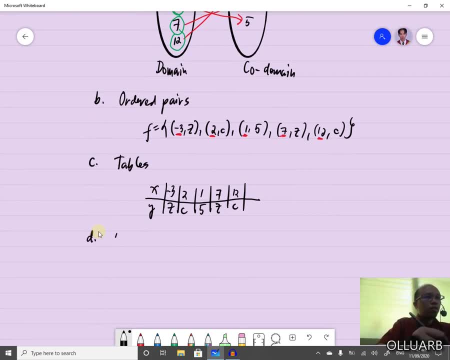 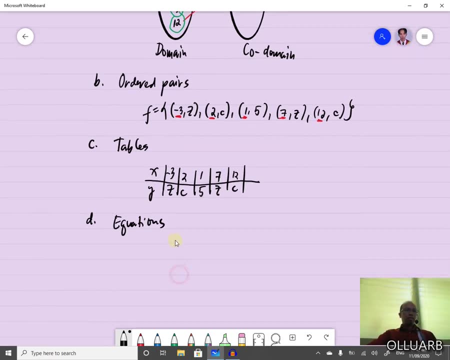 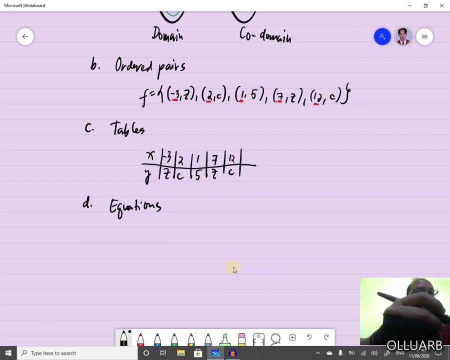 which is very important, is using equations. so there are in your algebra and trigonometry class. you will see that there are functions that we already discussed, like, for example. example of these are the linear functions. you know the quadratic functions. how about logarithmic functions? natural logarithmic? 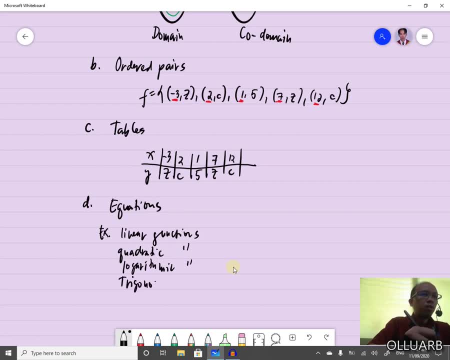 trigonometric functions, right on your metric functions, and a lot more exponenti functions, a lot more exponenti function. remember the exponential functions and many other? okay, so this is described by this notation: y is equal to f of X, and if you remember the vertical line test, the horizontal line test, the vertical line test, for if you want to, to 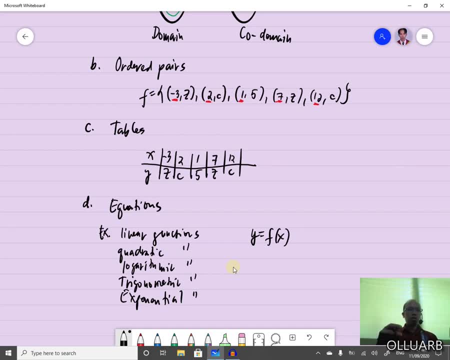 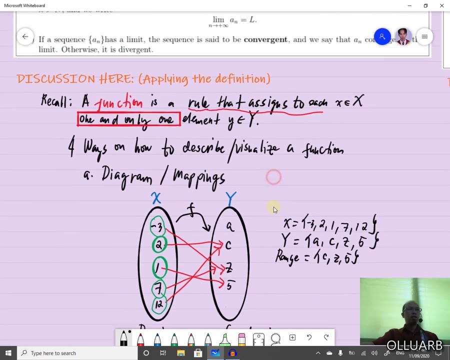 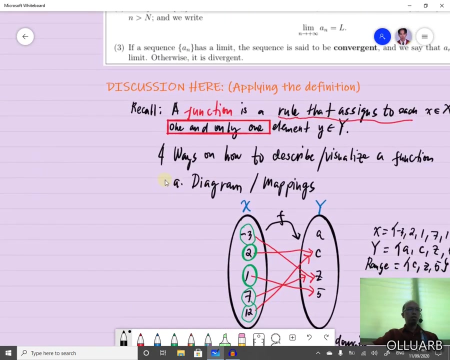 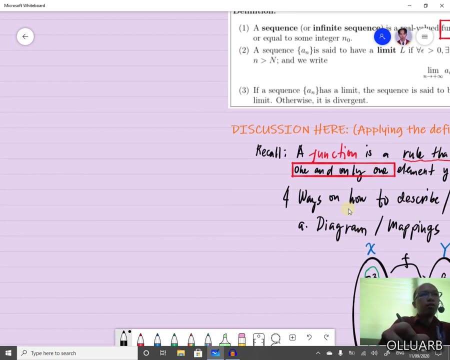 determine if the given equation is a function or not. of course you have a graph, so, as you can see here, I've already discussed to you what it means to be a function. okay, so for our notation, let's discuss it here. for our notation, for a function notation, this is described as f of X. this one f maps to. 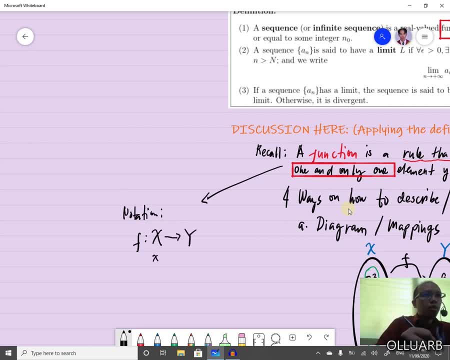 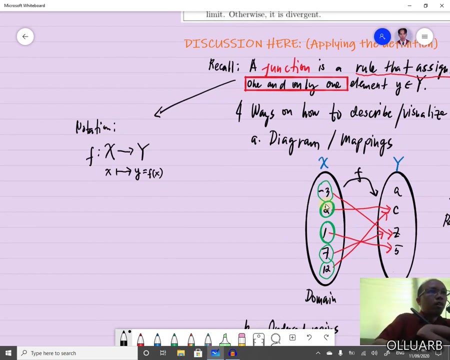 y, where our small x here is maps to small y, or you can write this one, as this is our f of X, okay, so meaning to say every element here. for example, this example: here our sample, our negative 3 is map to Z. here our sample, our negative 3 is map to Z. 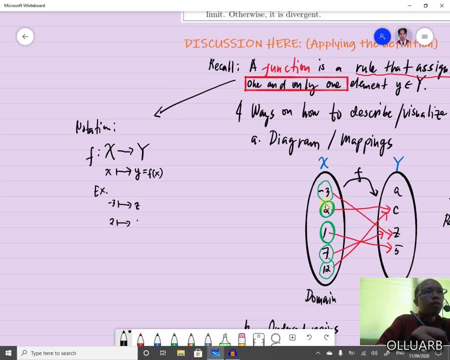 here our sample, our negative 3 is map to z, forth two. its map to Z: 1 mark to I I 7. it's not to G again, proteges mount room. forth two. its map to C, 1 mark to I 7. it's not to G, again, proteges mount room. 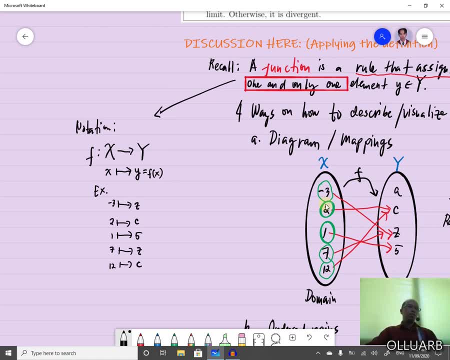 forth two, its map to Z, again proteges mount room C. so this is a function, because no 2 and 2 are 연els karimovuu. forth two, its map to C. so this is a function because no 2 and 2 are yen vent就是說, ah, marko. 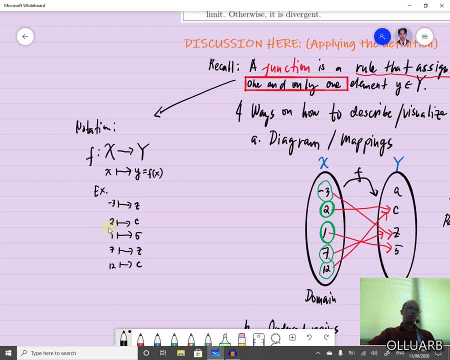 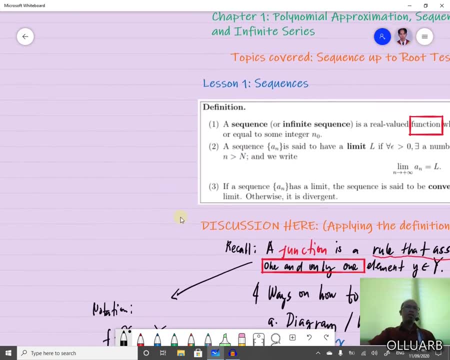 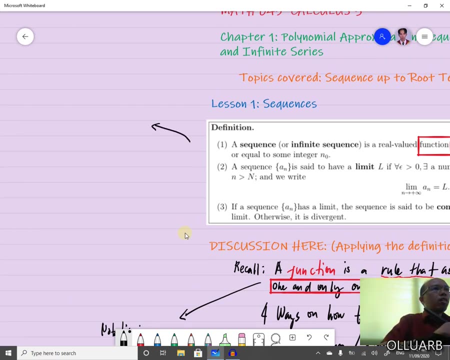 object here in the domain are repeated. okay, so let's go back now to our definition. it says here that a sequence- let's try to explain, explain this one- a sequence is a function, real valued function. meaning to say, when you say real valued is the domain, must be added. 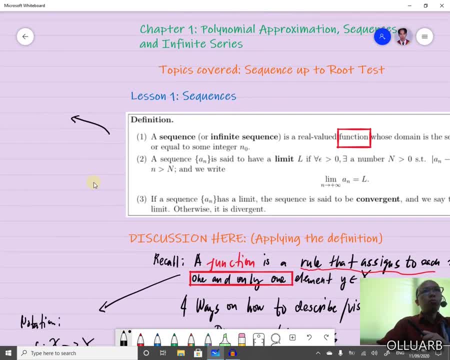 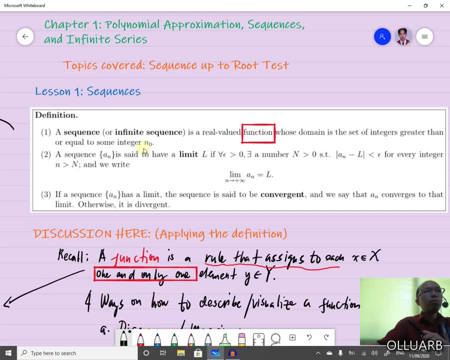 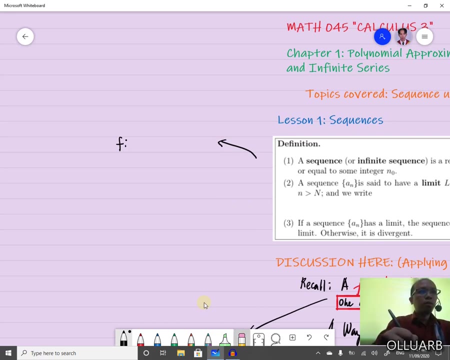 the codomain must be real. so whose domain is the set of integers greater than or equal to some integer and not? so we will be sorry, I had to erase this one and our function. whose domain is this one set of integers up to n sub o plus n? 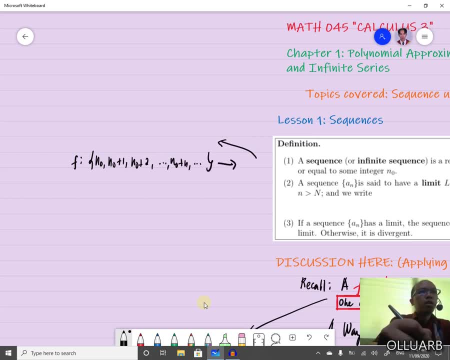 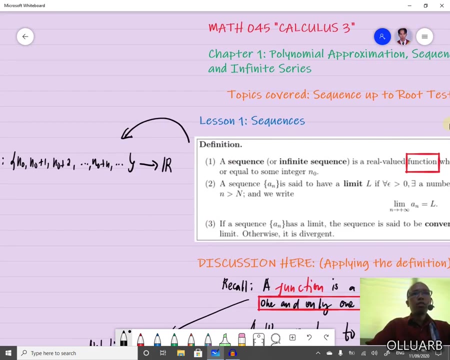 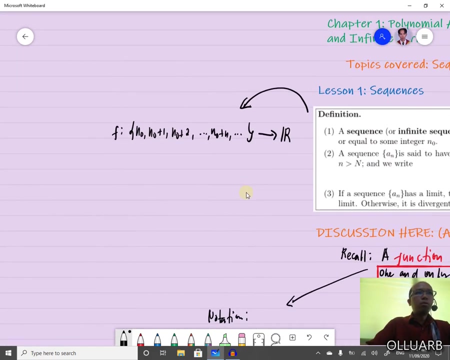 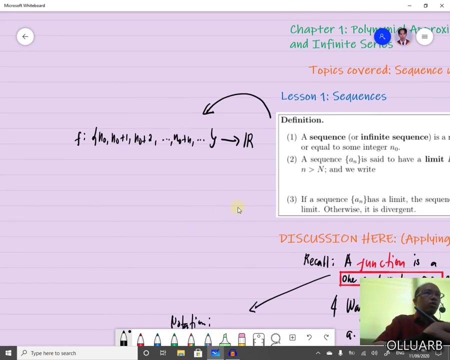 which is maps to the set of real number y. this is because it is a real valued function. as you can see, real valued function, it is a real valued function whose domain- but usually in our, in your book we take, usually usually our n sub o is always equal to 1. so meaning to say, if it's equal to 1, then our function now. 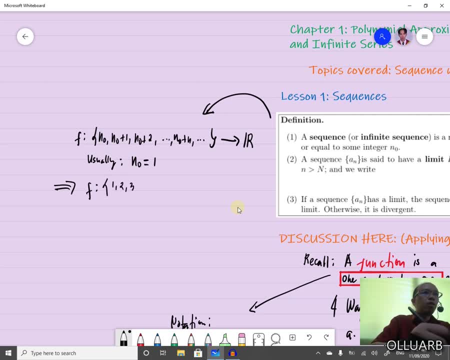 will be become 1, 2, 3, 4 and so on, up to a max, to the set of real numbers. if our n not, we is equal to 1. if n not is equal to 0, then it will start from 0, 1, 2, 3 up to n. if it will start from 5, then we have 5, 6, 7, 8. 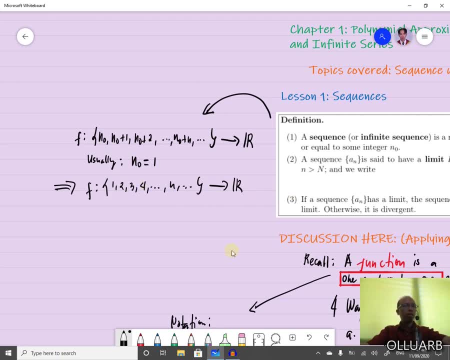 up to n, and so on, up to infinity. so meaning to say here, in the one here is map to our object in the code domain, which is we will be, we will be denoting it as a 1, okay, and then when it is 2, we have a sub 2, when it is 3, we have a 3, and so on. if you have n, 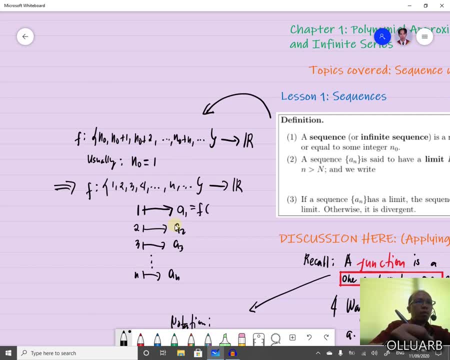 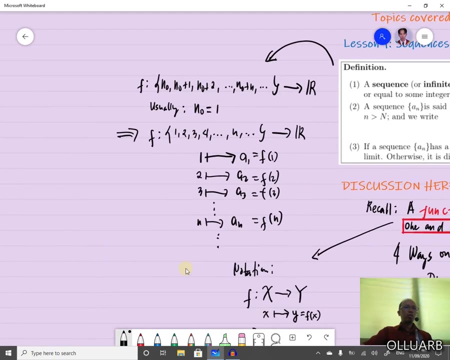 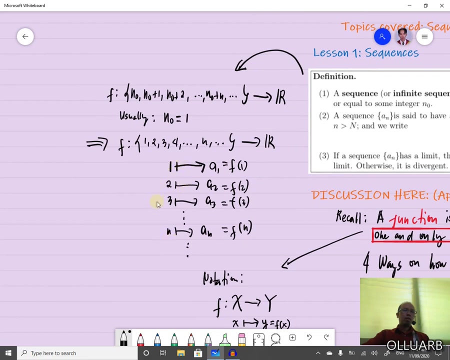 darfôn, and this is our f of 1, and this is our f of 2 is our notation before f of 3, and so on. okay, so what you will see here is that there's nothing much more pleasing. when we study the domain of the sequence the most important here is the, what they call this one. 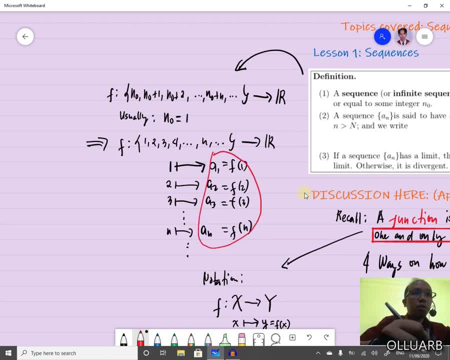 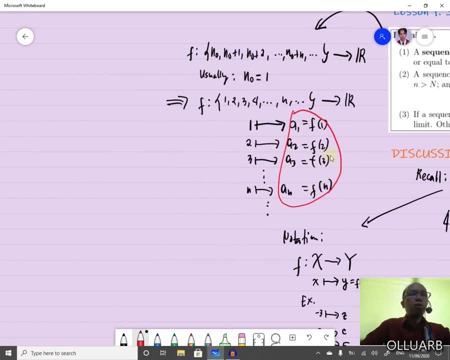 the range of the sequence okay. so meaning to say, we will be focusing our study in the range of the sequence okay, and as you notice here, I'm going to explain again here that we will be studying all these elements of the range of the sequence before up to here. so this is now our sequence. okay, and, as you notice here, I'm going to explain again here that we will be focusing our study in the range of the sequence before up to here. so this is now our sequence. okay, and, as you notice here, I'm going to explain again here that we will be focusing all these. 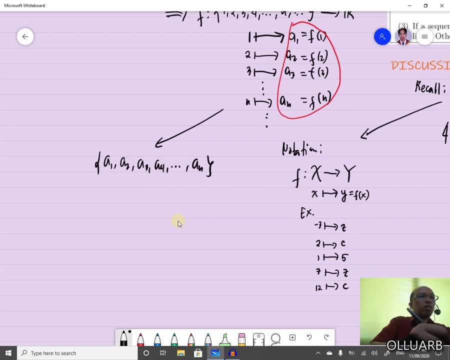 elements of the sequence before up to here. so this is now our sequence, okay and, as you notice here, I'm going to explain again here that we will be focusing all these elements of the sequence before up to here. so this is now our sequence, okay and, as you notice here, I'm going to explain again here that we will be focusing all these. 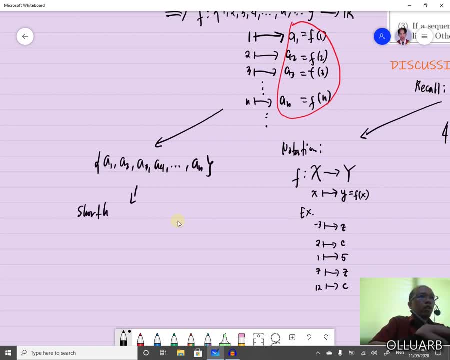 elements of the sequence before up to here. so this is now our sequence, okay and, as you notice here, I'm going to explain again here that we will be focusing all these elements of the sequence before up to here. so this is now our sequence, okay and, as you notice here, I'm going to explain again here that we will be focusing all these. 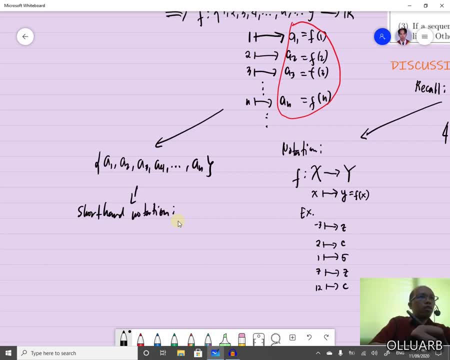 elements of the sequence before up to here. so this is now our sequence, okay and, as you notice here, I'm going to explain again here that we will be focusing all these elements of the sequence before up to here. so this is now our sequence, okay and, as you notice here, I'm going to explain again here that we will be focusing all these. 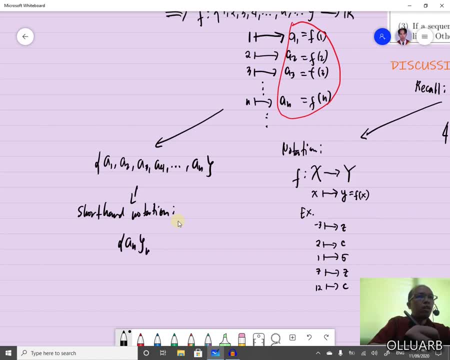 elements of the sequence before up to here. so this is now our sequence, okay and, as you notice here, I'm going to explain again here that we will be focusing all these elements of the sequence before up to here. so this is now our sequence, okay and, as you notice here, I'm going to explain again here that we will be focusing all these. 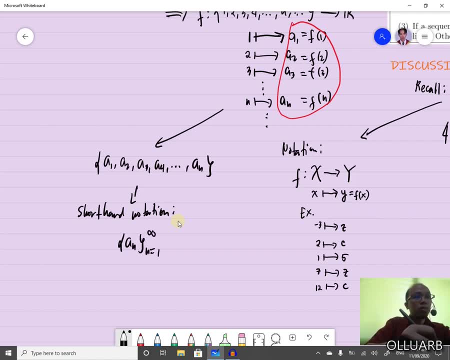 elements of the sequence before up to here. so this is now our sequence, okay and, as you notice here, I'm going to explain again here that we will be focusing all these elements of the sequence before up to here. so this is now our sequence, okay and, as you notice here, I'm going to explain again here that we will be focusing all these. 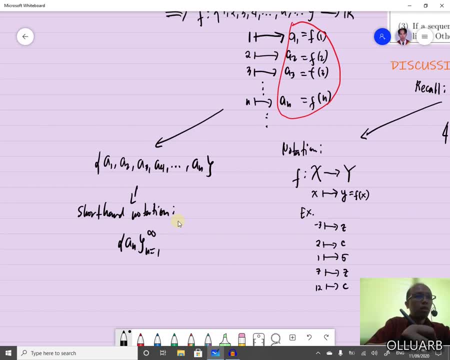 elements of the sequence before up to here. so this is now our sequence, okay and, as you notice here, I'm going to explain again here that we will be focusing all these elements of the sequence before up to here. so this is now our sequence, okay and, as you notice here, I'm going to explain again here that we will be focusing all these. 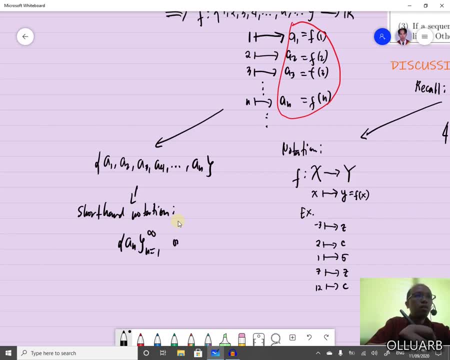 elements of the sequence before up to here. so this is now our sequence, okay and, as you notice here, I'm going to explain again here that we will be focusing all these elements of the sequence before up to here. so this is now our sequence, okay and, as you notice here, I'm going to explain again here that we will be focusing all these. 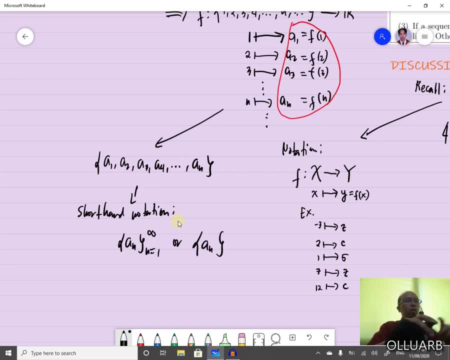 elements of the sequence before up to here. so this is now our sequence, okay and, as you notice here, I'm going to explain again here that we will be focusing all these elements of the sequence before up to here. so this is now our sequence, okay and, as you notice here, I'm going to explain again here that we will be focusing all these. 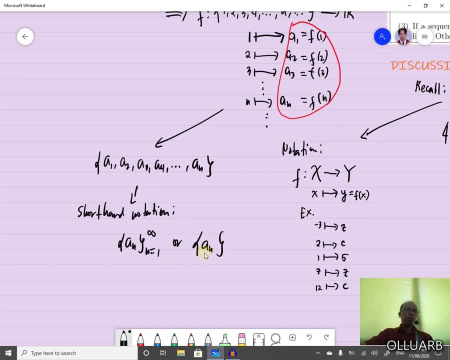 elements of the sequence before up to here. so this is now our sequence, okay and, as you notice here, I'm going to explain again here that we will be focusing all these elements of the sequence before up to here. so this is now our sequence, okay and, as you notice here, I'm going to explain again here that we will be focusing all these. 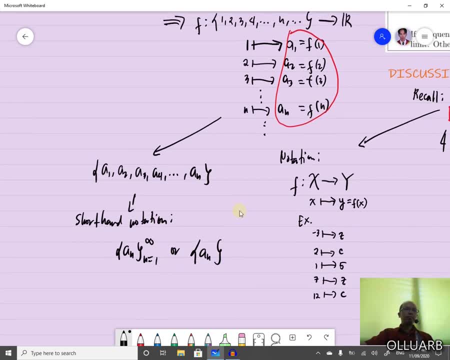 elements of the sequence before up to here. so this is now our sequence, okay and, as you notice here, I'm going to explain again here that we will be focusing all these elements of the sequence before up to here. so this is now our sequence, okay and, as you notice here, I'm going to explain again here that we will be focusing all these. 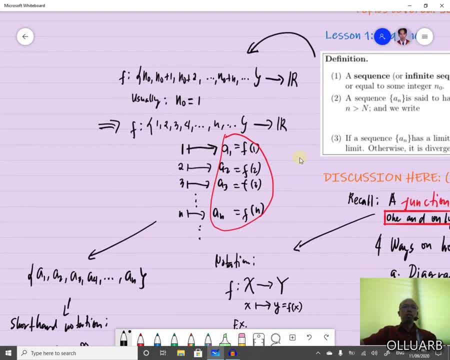 elements of the sequence before up to here. so this is now our sequence, okay and, as you notice here, I'm going to explain again here that we will be focusing all these elements of the sequence before up to here. so this is now our sequence, okay and, as you notice here, I'm going to explain again here that we will be focusing all these. 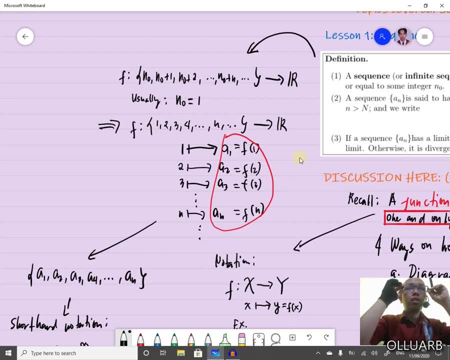 elements of the sequence before up to here. so this is now our sequence, okay and, as you notice here, I'm going to explain again here that we will be focusing all these elements of the sequence before up to here. so this is now our sequence, okay and, as you notice here, I'm going to explain again here that we will be focusing all these. 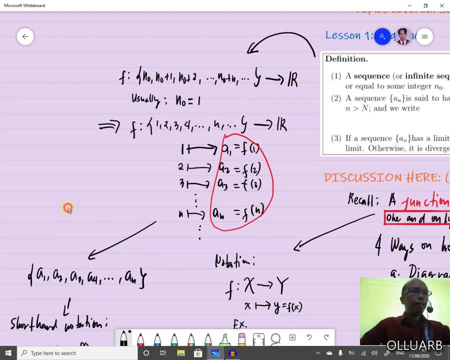 elements of the sequence before up to here. so this is now our sequence, okay and, as you notice here, I'm going to explain again here that we will be focusing all these elements of the sequence before up to here. so this is now our sequence, okay and, as you notice here, I'm going to explain again here that we will be focusing all these. 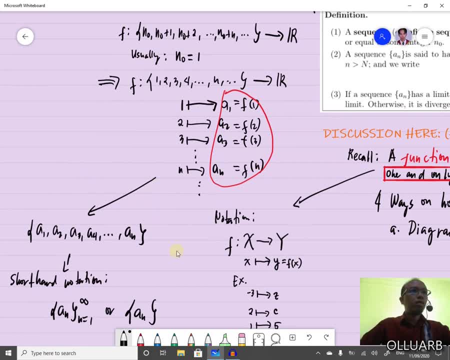 elements of the sequence before up to here. so this is now our sequence, okay and, as you notice here, I'm going to explain again here that we will be focusing all these elements of the sequence before up to here. so this is now our sequence, okay and, as you notice here, I'm going to explain again here that we will be focusing all these. 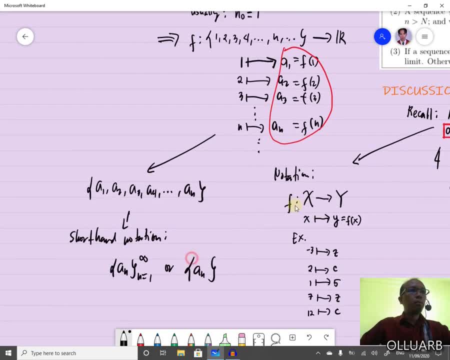 elements of the sequence before up to here. so this is now our sequence, okay and, as you notice here, I'm going to explain again here that we will be focusing all these elements of the sequence before up to here. so this is now our sequence, okay and, as you notice here, I'm going to explain again here that we will be focusing all these. 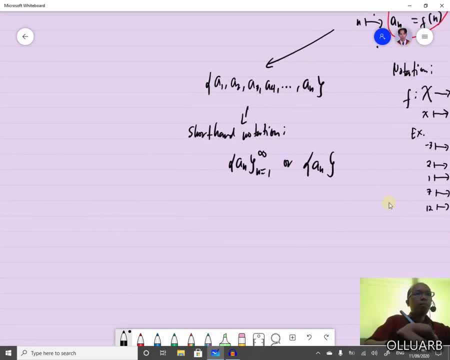 elements of the sequence before up to here. so this is now our sequence, okay and, as you notice here, I'm going to explain again here that we will be focusing all these elements of the sequence before up to here. so this is now our sequence, okay and, as you notice here, I'm going to explain again here that we will be focusing all these. 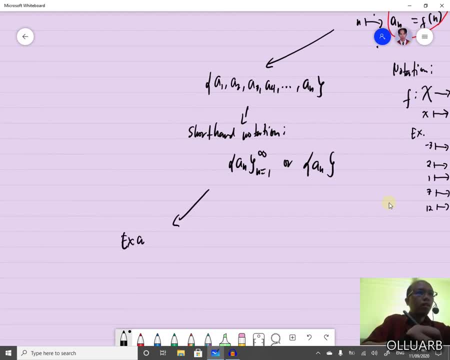 elements of the sequence before up to here. so this is now our sequence, okay and, as you notice here, I'm going to explain again here that we will be focusing all these elements of the sequence before up to here. so this is now our sequence, okay and, as you notice here, I'm going to explain again here that we will be focusing all these. 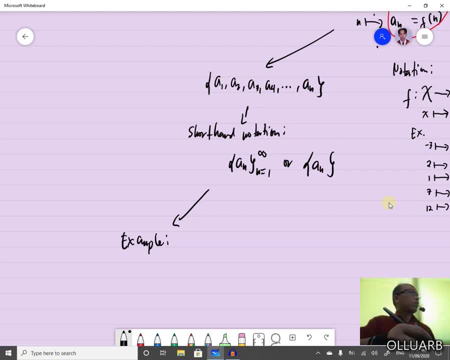 elements of the sequence before up to here. so this is now our sequence, okay and, as you notice here, I'm going to explain again here that we will be focusing all these elements of the sequence before up to here. so this is now our sequence, okay and, as you notice here, I'm going to explain again here that we will be focusing all these. 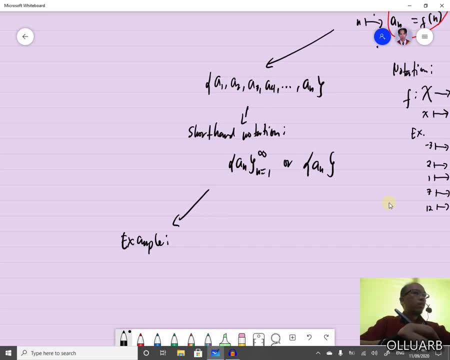 elements of the sequence before up to here. so this is now our sequence, okay and, as you notice here, I'm going to explain again here that we will be focusing all these elements of the sequence before up to here. so this is now our sequence, okay and, as you notice here, I'm going to explain again here that we will be focusing all these. 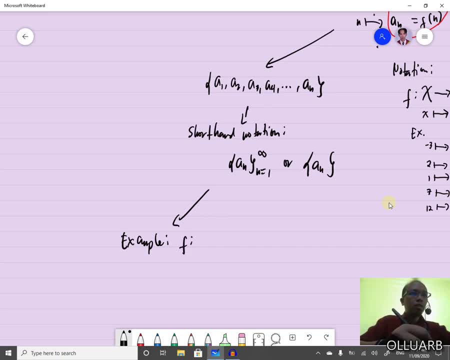 elements of the sequence before up to here. so this is now our sequence, okay and, as you notice here, I'm going to explain again here that we will be focusing all these elements of the sequence before up to here. so this is now our sequence, okay and, as you notice here, I'm going to explain again here that we will be focusing all these. 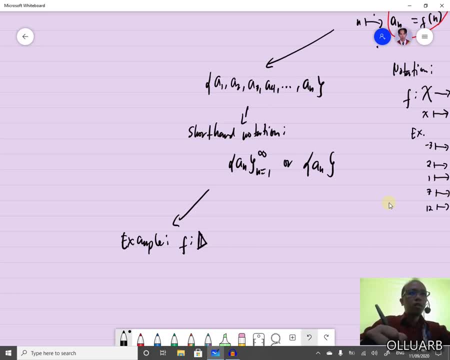 elements of the sequence before up to here. so this is now our sequence, okay and, as you notice here, I'm going to explain again here that we will be focusing all these elements of the sequence before up to here. so this is now our sequence, okay and, as you notice here, I'm going to explain again here that we will be focusing all these. 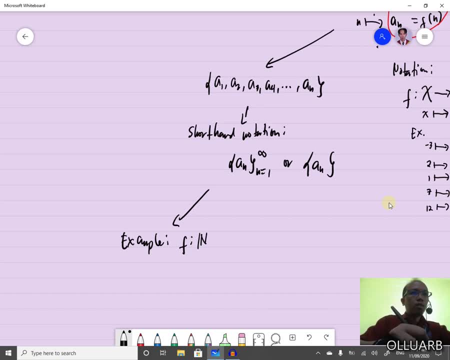 elements of the sequence before up to here. so this is now our sequence, okay and, as you notice here, I'm going to explain again here that we will be focusing all these elements of the sequence before up to here. so this is now our sequence, okay and, as you notice here, I'm going to explain again here that we will be focusing all these. 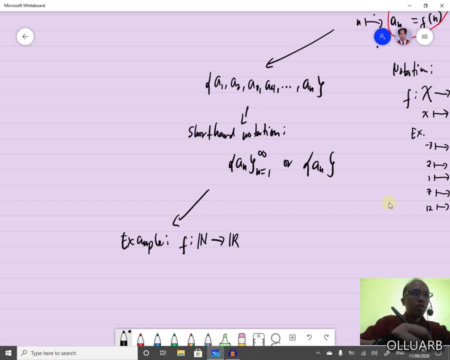 elements of the sequence before up to here. so this is now our sequence, okay and, as you notice here, I'm going to explain again here that we will be focusing all these elements of the sequence before up to here. so this is now our sequence, okay and, as you notice here, I'm going to explain again here that we will be focusing all these. 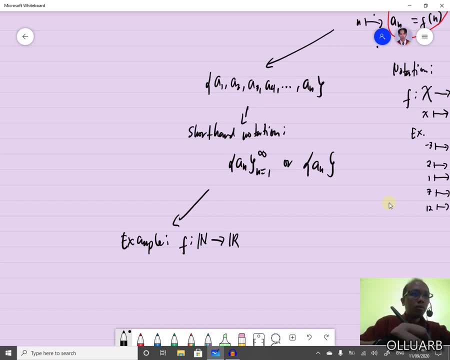 elements of the sequence before up to here. so this is now our sequence, okay and, as you notice here, I'm going to explain again here that we will be focusing all these elements of the sequence before up to here. so this is now our sequence, okay and, as you notice here, I'm going to explain again here that we will be focusing all these. 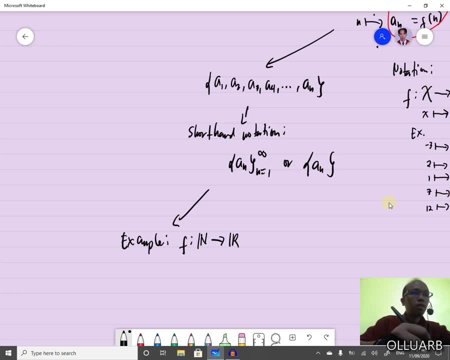 elements of the sequence before up to here. so this is now our sequence, okay and, as you notice here, I'm going to explain again here that we will be focusing all these elements of the sequence before up to here. so this is now our sequence, okay and, as you notice here, I'm going to explain again here that we will be focusing all these. 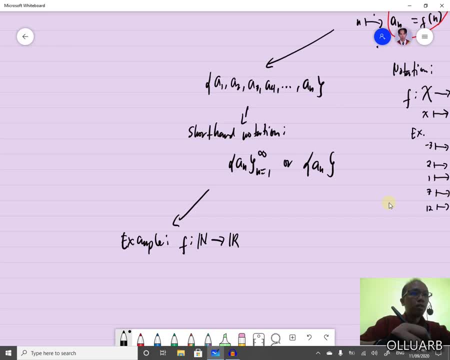 elements of the sequence before up to here. so this is now our sequence, okay and, as you notice here, I'm going to explain again here that we will be focusing all these elements of the sequence before up to here. so this is now our sequence, okay and, as you notice here, I'm going to explain again here that we will be focusing all these. 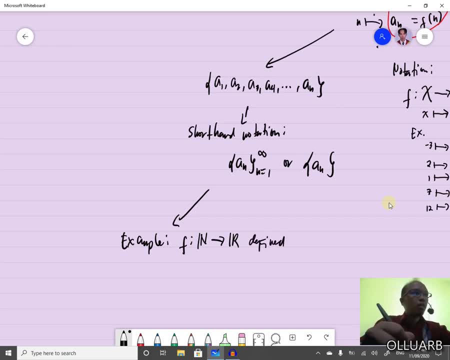 elements of the sequence before up to here. so this is now our sequence, okay and, as you notice here, I'm going to explain again here that we will be focusing all these elements of the sequence before up to here. so this is now our sequence, okay and, as you notice here, I'm going to explain again here that we will be focusing all these. 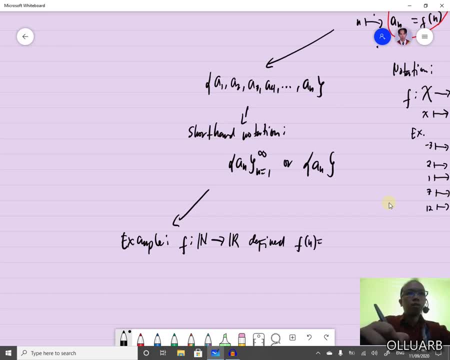 elements of the sequence before up to here. so this is now our sequence, okay and, as you notice here, I'm going to explain again here that we will be focusing all these elements of the sequence before up to here. so this is now our sequence, okay and, as you notice here, I'm going to explain again here that we will be focusing all these. 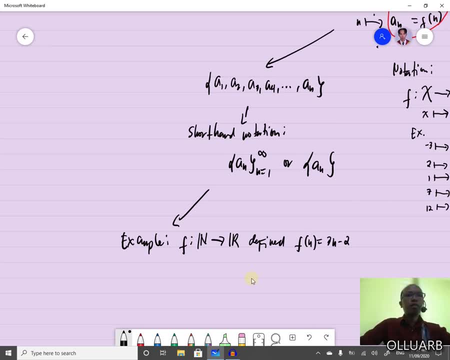 elements of the sequence before up to here. so this is now our sequence, okay and, as you notice here, I'm going to explain again here that we will be focusing all these elements of the sequence before up to here. so this is now our sequence, okay and, as you notice here, I'm going to explain again here that we will be focusing all these. 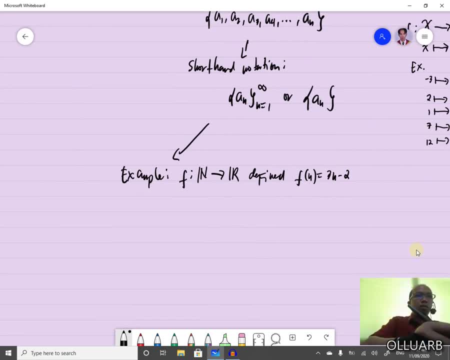 elements of the sequence before up to here. so this is now our sequence, okay and, as you notice here, I'm going to explain again here that we will be focusing all these elements of the sequence before up to here. so this is now our sequence, okay and, as you notice here, I'm going to explain again here that we will be focusing all these. 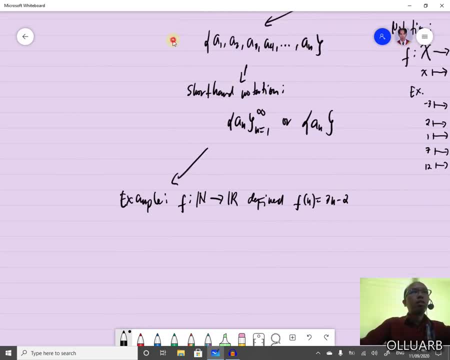 elements of the sequence before up to here. so this is now our sequence, okay and, as you notice here, I'm going to explain again here that we will be focusing all these elements of the sequence before up to here. so this is now our sequence, okay and, as you notice here, I'm going to explain again here that we will be focusing all these. 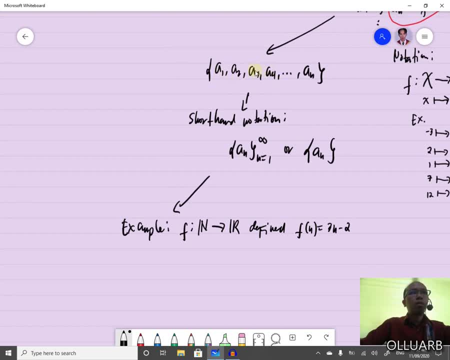 elements of the sequence before up to here. so this is now our sequence, okay and, as you notice here, I'm going to explain again here that we will be focusing all these elements of the sequence before up to here. so this is now our sequence, okay and, as you notice here, I'm going to explain again here that we will be focusing all these. 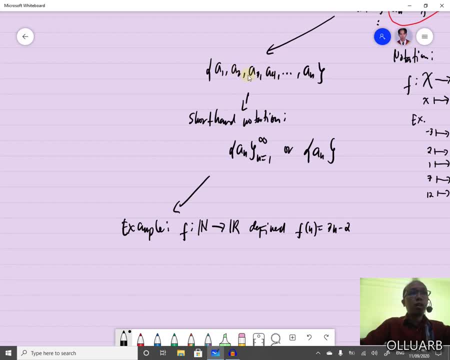 elements of the sequence before up to here. so this is now our sequence, okay and, as you notice here, I'm going to explain again here that we will be focusing all these elements of the sequence before up to here. so this is now our sequence, okay and, as you notice here, I'm going to explain again here that we will be focusing all these. 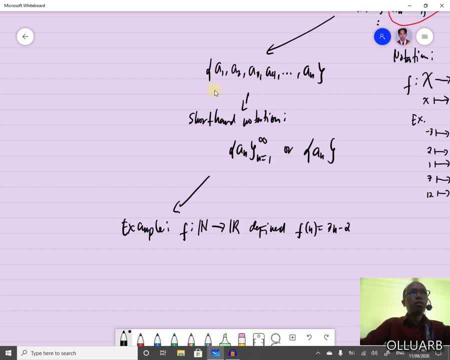 elements of the sequence before up to here. so this is now our sequence, okay and, as you notice here, I'm going to explain again here that we will be focusing all these elements of the sequence before up to here. so this is now our sequence, okay and, as you notice here, I'm going to explain again here that we will be focusing all these. 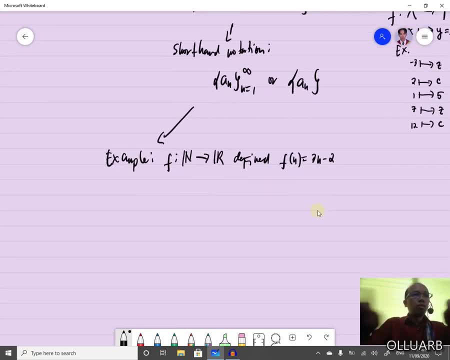 elements of the sequence before up to here. so this is now our sequence, okay and, as you notice here, I'm going to explain again here that we will be focusing all these elements of the sequence before up to here. so this is now our sequence, okay and, as you notice here, I'm going to explain again here that we will be focusing all these. 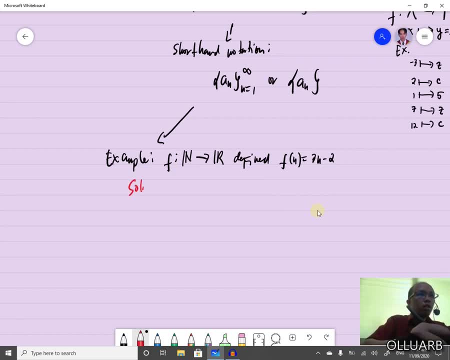 elements of the sequence before up to here. so this is now our sequence, okay and, as you notice here, I'm going to explain again here that we will be focusing all these elements of the sequence before up to here. so this is now our sequence, okay and, as you notice here, I'm going to explain again here that we will be focusing all these. 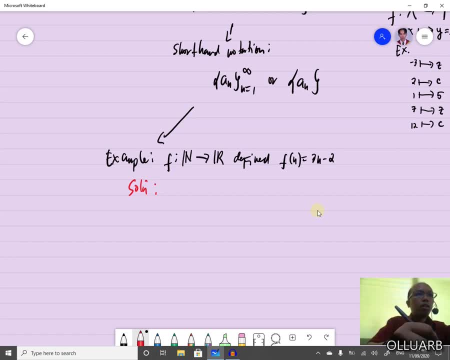 elements of the sequence before up to here. so this is now our sequence, okay and, as you notice here, I'm going to explain again here that we will be focusing all these elements of the sequence before up to here. so this is now our sequence, okay and, as you notice here, I'm going to explain again here that we will be focusing all these. 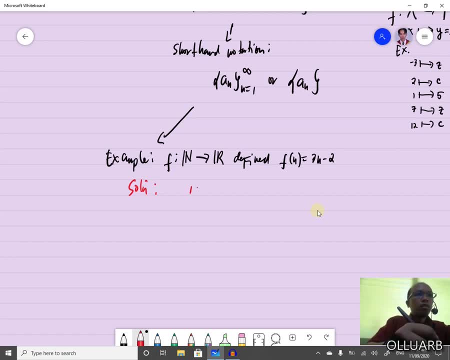 elements of the sequence before up to here. so this is now our sequence, okay and, as you notice here, I'm going to explain again here that we will be focusing all these elements of the sequence before up to here. so this is now our sequence, okay and, as you notice here, I'm going to explain again here that we will be focusing all these. 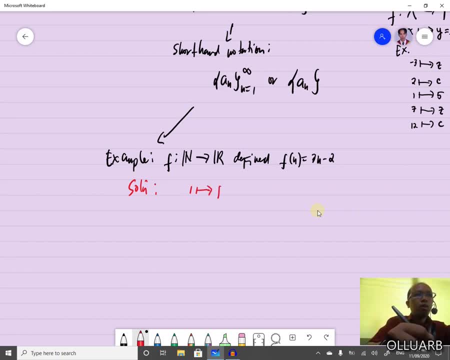 elements of the sequence before up to here. so this is now our sequence, okay and, as you notice here, I'm going to explain again here that we will be focusing all these elements of the sequence before up to here. so this is now our sequence, okay and, as you notice here, I'm going to explain again here that we will be focusing all these. 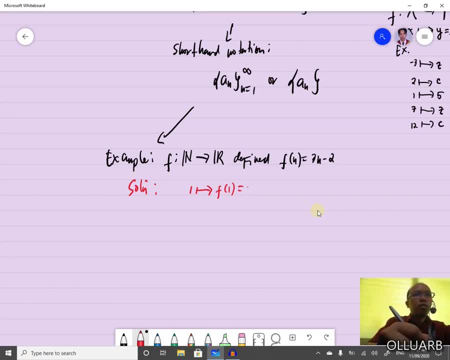 elements of the sequence before up to here. so this is now our sequence, okay and, as you notice here, I'm going to explain again here that we will be focusing all these elements of the sequence before up to here. so this is now our sequence, okay and, as you notice here, I'm going to explain again here that we will be focusing all these. 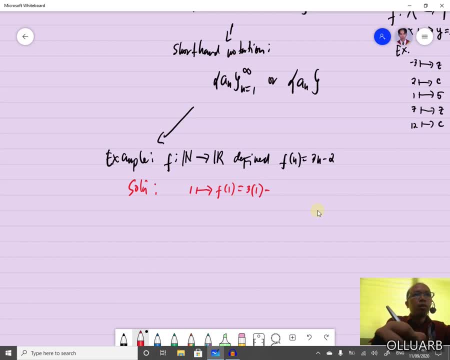 elements of the sequence before up to here. so this is now our sequence, okay and, as you notice here, I'm going to explain again here that we will be focusing all these elements of the sequence before up to here. so this is now our sequence, okay and, as you notice here, I'm going to explain again here that we will be focusing all these. 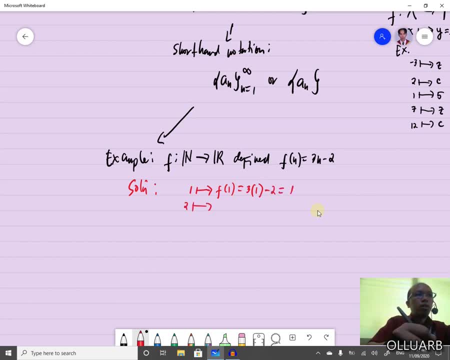 elements of the sequence before up to here. so this is now our sequence, okay and, as you notice here, I'm going to explain again here that we will be focusing all these elements of the sequence before up to here. so this is now our sequence, okay and, as you notice here, I'm going to explain again here that we will be focusing all these. 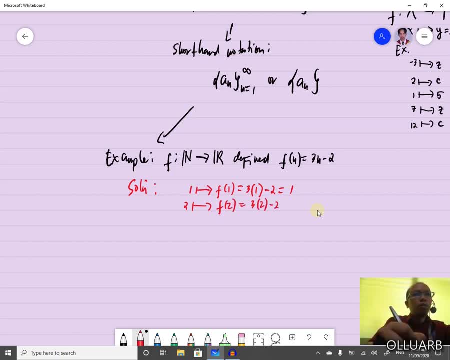 elements of the sequence before up to here. so this is now our sequence, okay and, as you notice here, I'm going to explain again here that we will be focusing all these elements of the sequence before up to here. so this is now our sequence, okay and, as you notice here, I'm going to explain again here that we will be focusing all these. 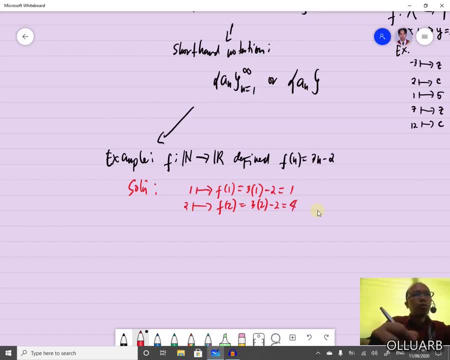 elements of the sequence before up to here. so this is now our sequence, okay and, as you notice here, I'm going to explain again here that we will be focusing all these elements of the sequence before up to here. so this is now our sequence, okay and, as you notice here, I'm going to explain again here that we will be focusing all these. 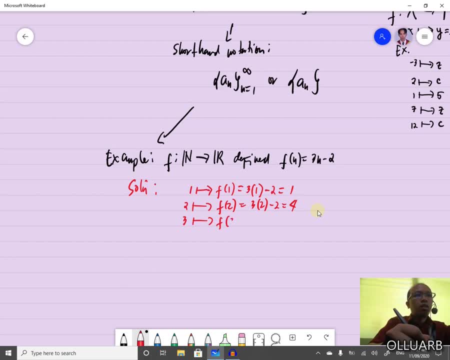 elements of the sequence before up to here. so this is now our sequence, okay and, as you notice here, I'm going to explain again here that we will be focusing all these elements of the sequence before up to here. so this is now our sequence, okay and, as you notice here, I'm going to explain again here that we will be focusing all these. 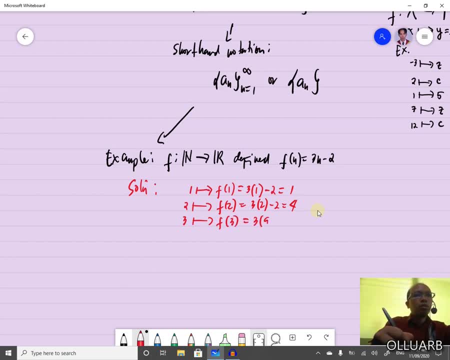 elements of the sequence before up to here. so this is now our sequence, okay and, as you notice here, I'm going to explain again here that we will be focusing all these elements of the sequence before up to here. so this is now our sequence, okay and, as you notice here, I'm going to explain again here that we will be focusing all these. 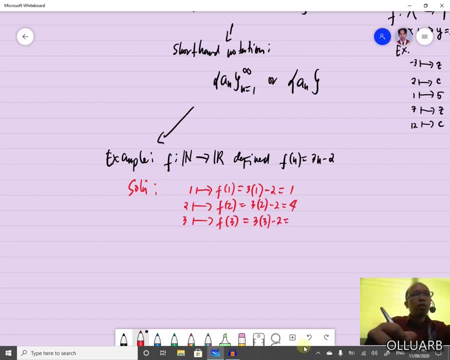 elements of the sequence before up to here. so this is now our sequence, okay and, as you notice here, I'm going to explain again here that we will be focusing all these elements of the sequence before up to here. so this is now our sequence, okay and, as you notice here, I'm going to explain again here that we will be focusing all these. 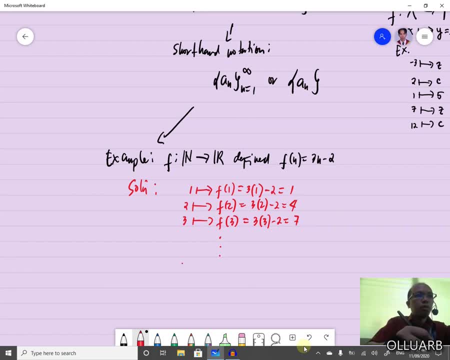 elements of the sequence before up to here. so this is now our sequence, okay and, as you notice here, I'm going to explain again here that we will be focusing all these elements of the sequence before up to here. so this is now our sequence, okay and, as you notice here, I'm going to explain again here that we will be focusing all these. 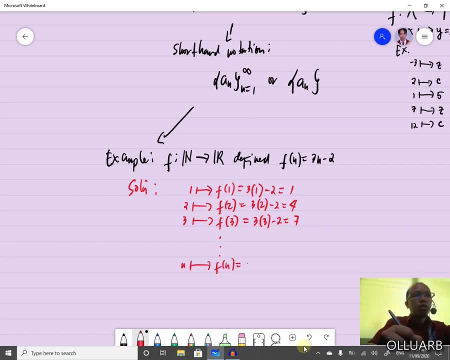 elements of the sequence before up to here. so this is now our sequence, okay and, as you notice here, I'm going to explain again here that we will be focusing all these elements of the sequence before up to here. so this is now our sequence, okay and, as you notice here, I'm going to explain again here that we will be focusing all these. 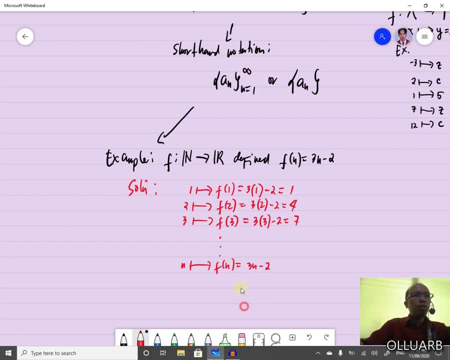 elements of the sequence before up to here. so this is now our sequence, okay and, as you notice here, I'm going to explain again here that we will be focusing all these elements of the sequence before up to here. so this is now our sequence, okay and, as you notice here, I'm going to explain again here that we will be focusing all these. 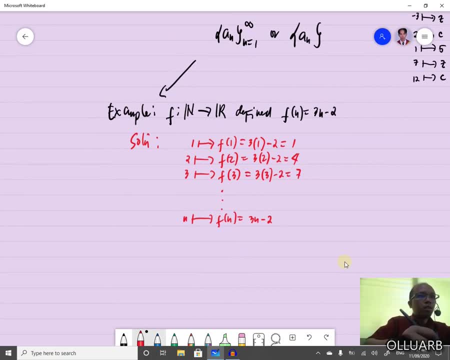 elements of the sequence before up to here. so this is now our sequence, okay and, as you notice here, I'm going to explain again here that we will be focusing all these elements of the sequence before up to here. so this is now our sequence, okay and, as you notice here, I'm going to explain again here that we will be focusing all these. 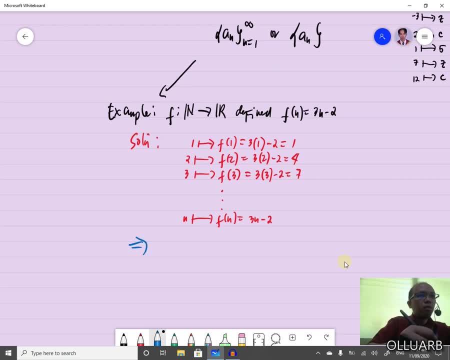 elements of the sequence before up to here. so this is now our sequence, okay and, as you notice here, I'm going to explain again here that we will be focusing all these elements of the sequence before up to here. so this is now our sequence, okay and, as you notice here, I'm going to explain again here that we will be focusing all these. 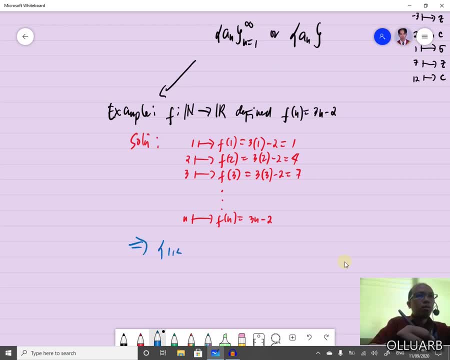 elements of the sequence before up to here. so this is now our sequence, okay and, as you notice here, I'm going to explain again here that we will be focusing all these elements of the sequence before up to here. so this is now our sequence, okay and, as you notice here, I'm going to explain again here that we will be focusing all these. 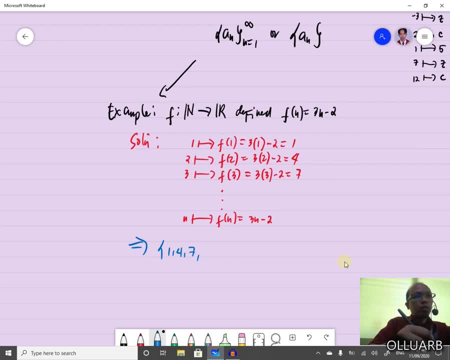 elements of the sequence before up to here. so this is now our sequence, okay and, as you notice here, I'm going to explain again here that we will be focusing all these elements of the sequence before up to here. so this is now our sequence, okay and, as you notice here, I'm going to explain again here that we will be focusing all these. 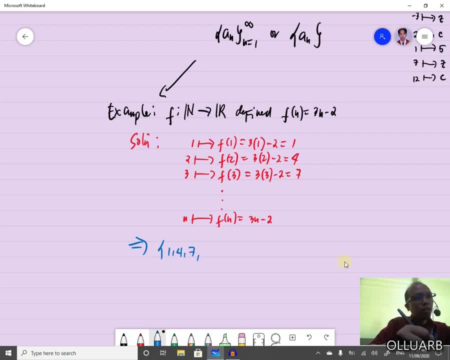 elements of the sequence before up to here. so this is now our sequence, okay and, as you notice here, I'm going to explain again here that we will be focusing all these elements of the sequence before up to here. so this is now our sequence, okay and, as you notice here, I'm going to explain again here that we will be focusing all these. 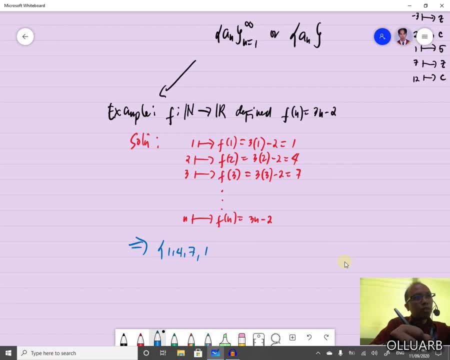 elements of the sequence before up to here. so this is now our sequence, okay and, as you notice here, I'm going to explain again here that we will be focusing all these elements of the sequence before up to here. so this is now our sequence, okay and, as you notice here, I'm going to explain again here that we will be focusing all these. 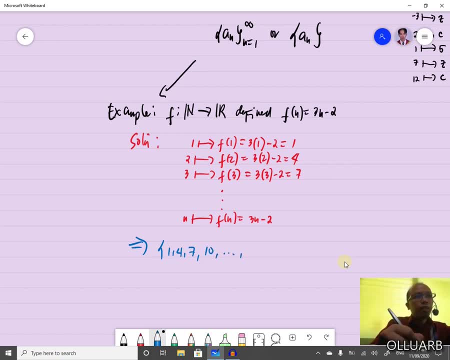 elements of the sequence before up to here. so this is now our sequence, okay and, as you notice here, I'm going to explain again here that we will be focusing all these elements of the sequence before up to here. so this is now our sequence, okay and, as you notice here, I'm going to explain again here that we will be focusing all these. 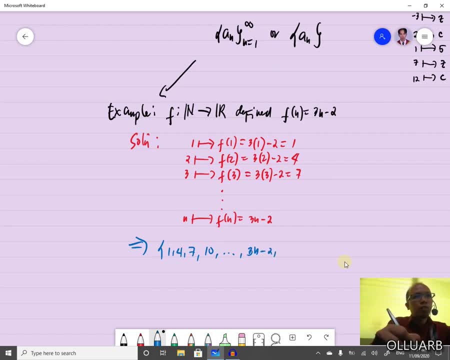 elements of the sequence before up to here. so this is now our sequence, okay and, as you notice here, I'm going to explain again here that we will be focusing all these elements of the sequence before up to here. so this is now our sequence, okay and, as you notice here, I'm going to explain again here that we will be focusing all these. 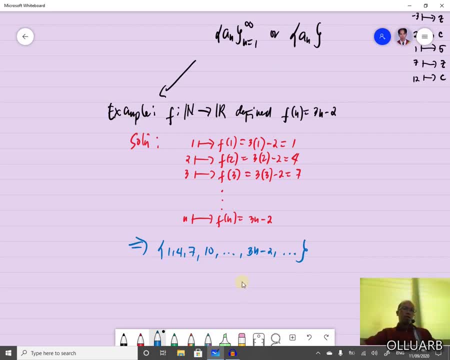 elements of the sequence before up to here. so this is now our sequence, okay and, as you notice here, I'm going to explain again here that we will be focusing all these elements of the sequence before up to here. so this is now our sequence, okay and, as you notice here, I'm going to explain again here that we will be focusing all these. 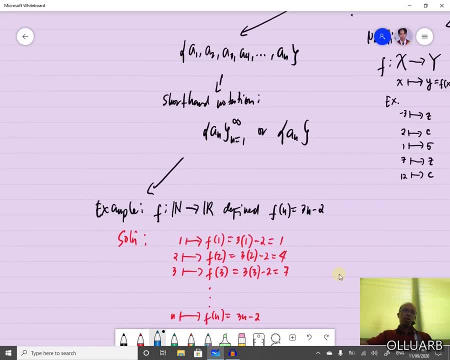 elements of the sequence before up to here. so this is now our sequence, okay and, as you notice here, I'm going to explain again here that we will be focusing all these elements of the sequence before up to here. so this is now our sequence, okay and, as you notice here, I'm going to explain again here that we will be focusing all these. 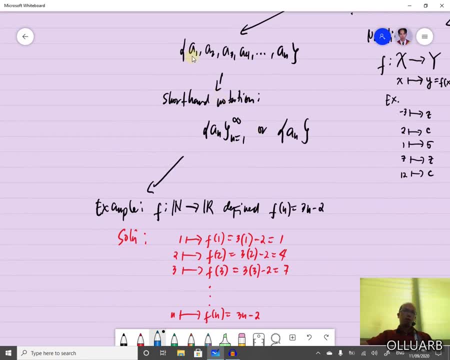 elements of the sequence before up to here. so this is now our sequence, okay and, as you notice here, I'm going to explain again here that we will be focusing all these elements of the sequence before up to here. so this is now our sequence, okay and, as you notice here, I'm going to explain again here that we will be focusing all these. 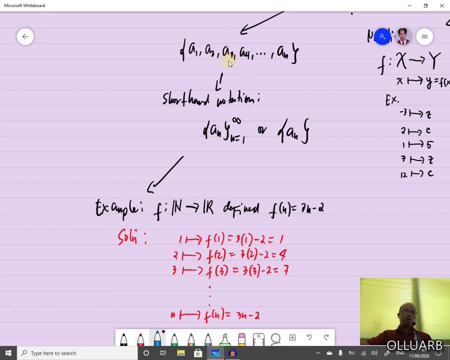 elements of the sequence before up to here. so this is now our sequence, okay and, as you notice here, I'm going to explain again here that we will be focusing all these elements of the sequence before up to here. so this is now our sequence, okay and, as you notice here, I'm going to explain again here that we will be focusing all these. 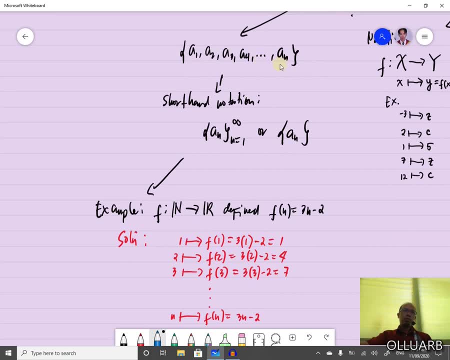 elements of the sequence before up to here. so this is now our sequence, okay and, as you notice here, I'm going to explain again here that we will be focusing all these elements of the sequence before up to here. so this is now our sequence, okay and, as you notice here, I'm going to explain again here that we will be focusing all these. 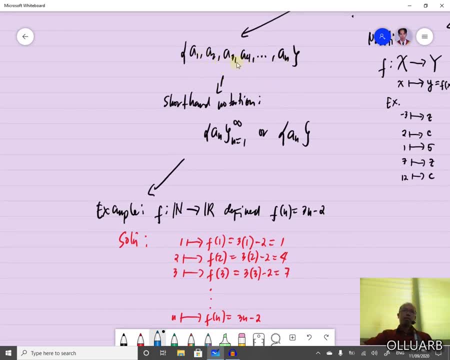 elements of the sequence before up to here. so this is now our sequence, okay and, as you notice here, I'm going to explain again here that we will be focusing all these elements of the sequence before up to here. so this is now our sequence, okay and, as you notice here, I'm going to explain again here that we will be focusing all these. 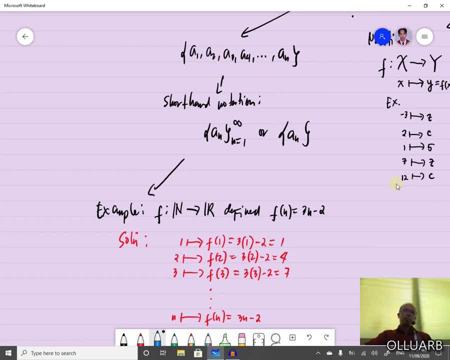 elements of the sequence before up to here. so this is now our sequence, okay and, as you notice here, I'm going to explain again here that we will be focusing all these elements of the sequence before up to here. so this is now our sequence, okay and, as you notice here, I'm going to explain again here that we will be focusing all these. 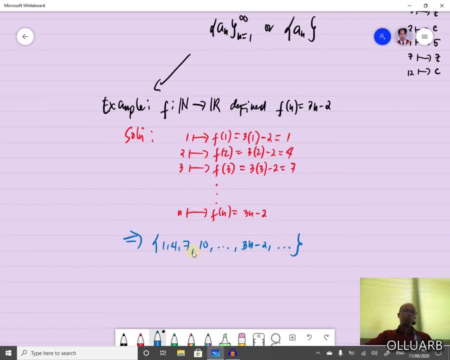 elements of the sequence before up to here. so this is now our sequence, okay and, as you notice here, I'm going to explain again here that we will be focusing all these elements of the sequence before up to here. so this is now our sequence, okay and, as you notice here, I'm going to explain again here that we will be focusing all these. 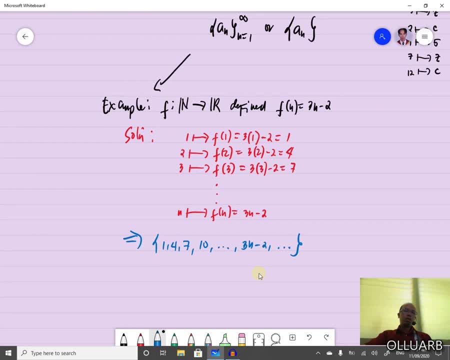 elements of the sequence before up to here. so this is now our sequence, okay and, as you notice here, I'm going to explain again here that we will be focusing all these elements of the sequence before up to here. so this is now our sequence, okay and, as you notice here, I'm going to explain again here that we will be focusing all these. 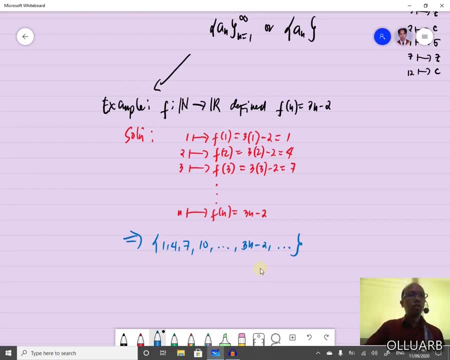 elements of the sequence before up to here. so this is now our sequence, okay and, as you notice here, I'm going to explain again here that we will be focusing all these elements of the sequence before up to here. so this is now our sequence, okay and, as you notice here, I'm going to explain again here that we will be focusing all these. 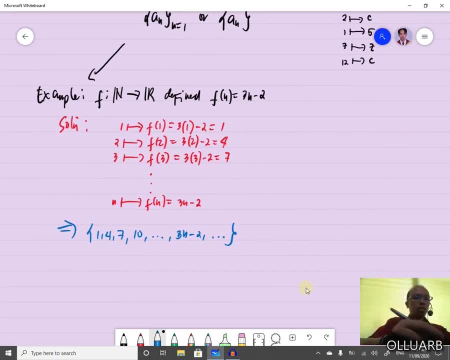 elements of the sequence before up to here. so this is now our sequence, okay and, as you notice here, I'm going to explain again here that we will be focusing all these elements of the sequence before up to here. so this is now our sequence, okay and, as you notice here, I'm going to explain again here that we will be focusing all these. 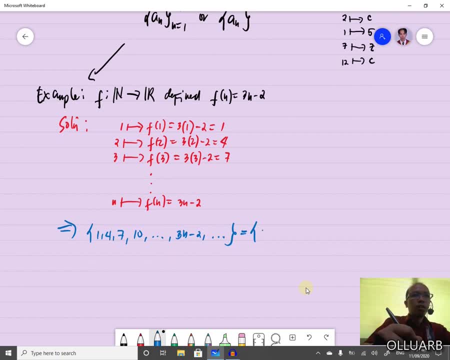 elements of the sequence before up to here. so this is now our sequence, okay and, as you notice here, I'm going to explain again here that we will be focusing all these elements of the sequence before up to here. so this is now our sequence, okay and, as you notice here, I'm going to explain again here that we will be focusing all these. 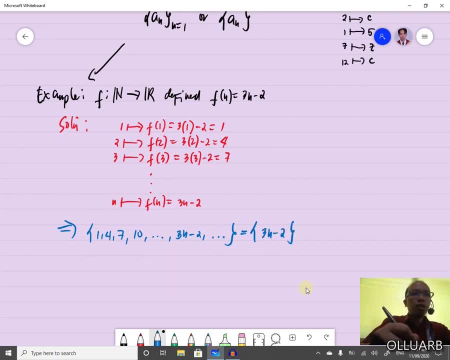 elements of the sequence before up to here. so this is now our sequence, okay and, as you notice here, I'm going to explain again here that we will be focusing all these elements of the sequence before up to here. so this is now our sequence, okay and, as you notice here, I'm going to explain again here that we will be focusing all these. 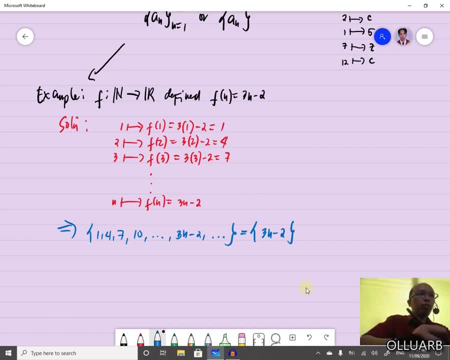 elements of the sequence before up to here. so this is now our sequence, okay and, as you notice here, I'm going to explain again here that we will be focusing all these elements of the sequence before up to here. so this is now our sequence, okay and, as you notice here, I'm going to explain again here that we will be focusing all these. 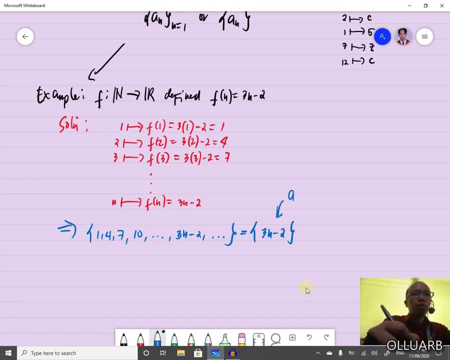 elements of the sequence before up to here. so this is now our sequence, okay and, as you notice here, I'm going to explain again here that we will be focusing all these elements of the sequence before up to here. so this is now our sequence, okay and, as you notice here, I'm going to explain again here that we will be focusing all these. 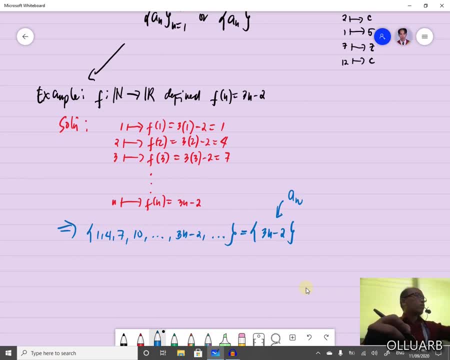 elements of the sequence before up to here. so this is now our sequence, okay and, as you notice here, I'm going to explain again here that we will be focusing all these elements of the sequence before up to here. so this is now our sequence, okay and, as you notice here, I'm going to explain again here that we will be focusing all these. 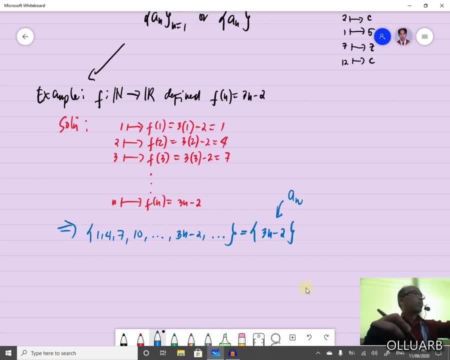 elements of the sequence before up to here. so this is now our sequence, okay and, as you notice here, I'm going to explain again here that we will be focusing all these elements of the sequence before up to here. so this is now our sequence, okay and, as you notice here, I'm going to explain again here that we will be focusing all these. 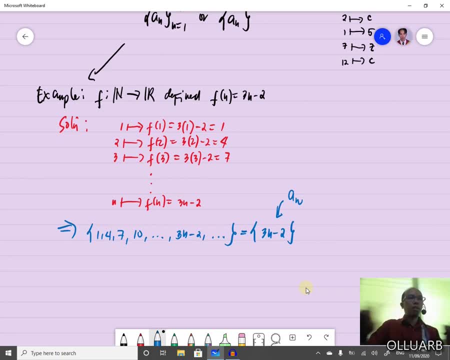 elements of the sequence before up to here. so this is now our sequence, okay and, as you notice here, I'm going to explain again here that we will be focusing all these elements of the sequence before up to here. so this is now our sequence, okay and, as you notice here, I'm going to explain again here that we will be focusing all these. 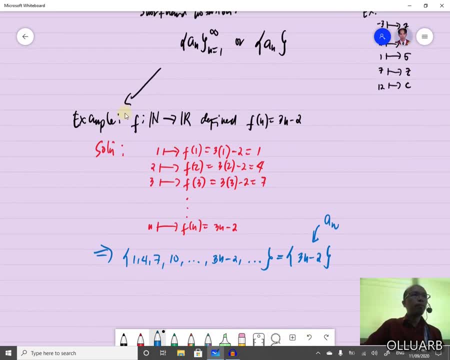 elements of the sequence before up to here. so this is now our sequence, okay and, as you notice here, I'm going to explain again here that we will be focusing all these elements of the sequence before up to here. so this is now our sequence, okay and, as you notice here, I'm going to explain again here that we will be focusing all these. 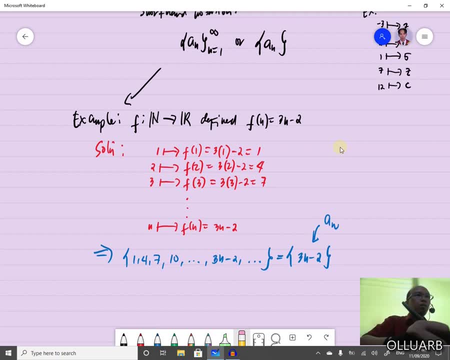 elements of the sequence before up to here. so this is now our sequence, okay and, as you notice here, I'm going to explain again here that we will be focusing all these elements of the sequence before up to here. so this is now our sequence, okay and, as you notice here, I'm going to explain again here that we will be focusing all these. 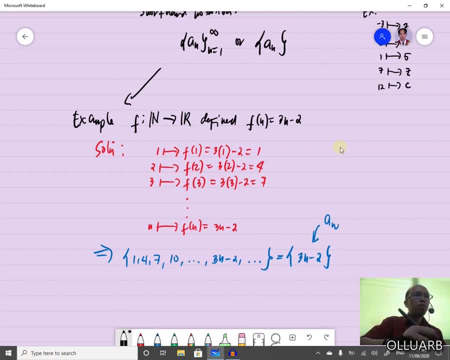 elements of the sequence before up to here. so this is now our sequence, okay and, as you notice here, I'm going to explain again here that we will be focusing all these elements of the sequence before up to here. so this is now our sequence, okay and, as you notice here, I'm going to explain again here that we will be focusing all these. 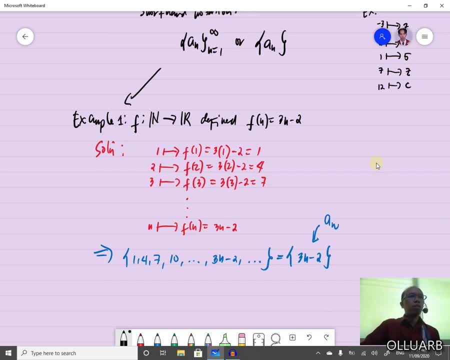 elements of the sequence before up to here. so this is now our sequence, okay and, as you notice here, I'm going to explain again here that we will be focusing all these elements of the sequence before up to here. so this is now our sequence, okay and, as you notice here, I'm going to explain again here that we will be focusing all these. 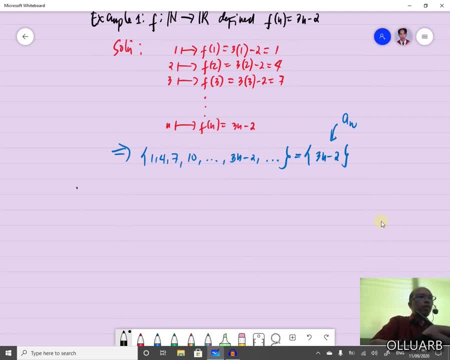 elements of the sequence before up to here. so this is now our sequence, okay and, as you notice here, I'm going to explain again here that we will be focusing all these elements of the sequence before up to here. so this is now our sequence, okay and, as you notice here, I'm going to explain again here that we will be focusing all these. 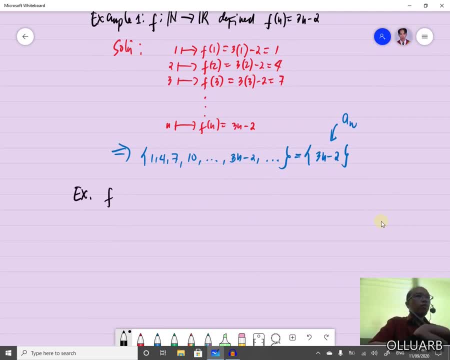 elements of the sequence before up to here. so this is now our sequence, okay and, as you notice here, I'm going to explain again here that we will be focusing all these elements of the sequence before up to here. so this is now our sequence, okay and, as you notice here, I'm going to explain again here that we will be focusing all these. 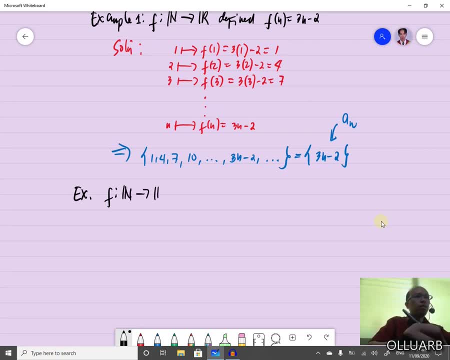 elements of the sequence before up to here. so this is now our sequence, okay and, as you notice here, I'm going to explain again here that we will be focusing all these elements of the sequence before up to here. so this is now our sequence, okay and, as you notice here, I'm going to explain again here that we will be focusing all these. 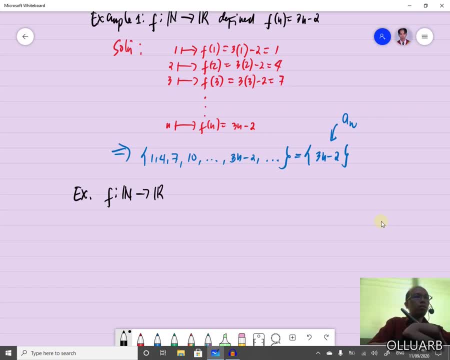 elements of the sequence before up to here. so this is now our sequence, okay and, as you notice here, I'm going to explain again here that we will be focusing all these elements of the sequence before up to here. so this is now our sequence, okay and, as you notice here, I'm going to explain again here that we will be focusing all these. 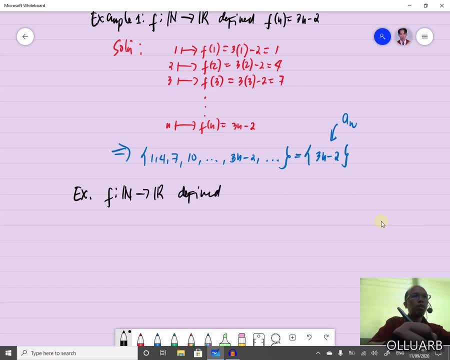 elements of the sequence before up to here. so this is now our sequence, okay and, as you notice here, I'm going to explain again here that we will be focusing all these elements of the sequence before up to here. so this is now our sequence, okay and, as you notice here, I'm going to explain again here that we will be focusing all these. 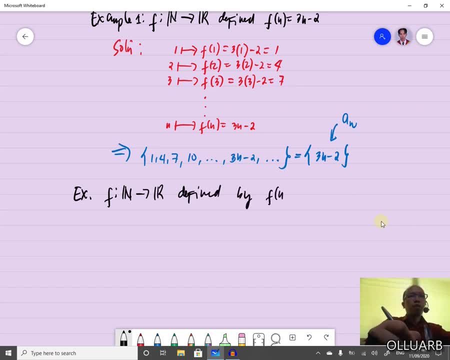 elements of the sequence before up to here. so this is now our sequence, okay and, as you notice here, I'm going to explain again here that we will be focusing all these elements of the sequence before up to here. so this is now our sequence, okay and, as you notice here, I'm going to explain again here that we will be focusing all these. 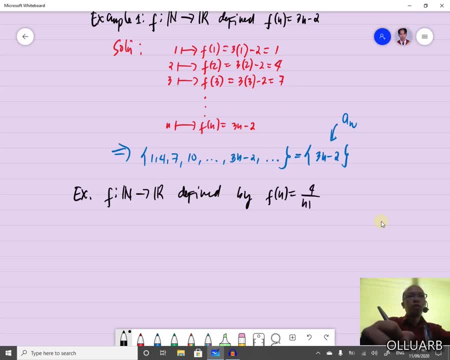 elements of the sequence before up to here. so this is now our sequence, okay and, as you notice here, I'm going to explain again here that we will be focusing all these elements of the sequence before up to here. so this is now our sequence, okay and, as you notice here, I'm going to explain again here that we will be focusing all these. 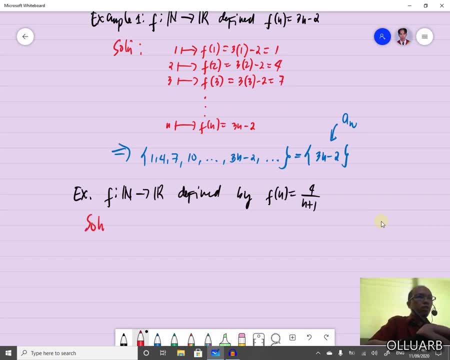 elements of the sequence before up to here. so this is now our sequence, okay and, as you notice here, I'm going to explain again here that we will be focusing all these elements of the sequence before up to here. so this is now our sequence, okay and, as you notice here, I'm going to explain again here that we will be focusing all these. 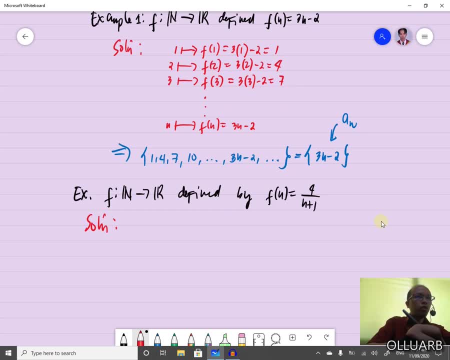 elements of the sequence before up to here. so this is now our sequence, okay and, as you notice here, I'm going to explain again here that we will be focusing all these elements of the sequence before up to here. so this is now our sequence, okay and, as you notice here, I'm going to explain again here that we will be focusing all these. 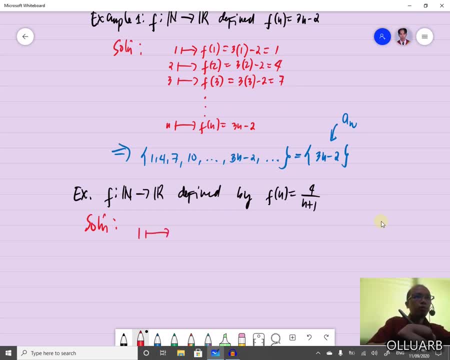 elements of the sequence before up to here. so this is now our sequence, okay and, as you notice here, I'm going to explain again here that we will be focusing all these elements of the sequence before up to here. so this is now our sequence, okay and, as you notice here, I'm going to explain again here that we will be focusing all these. 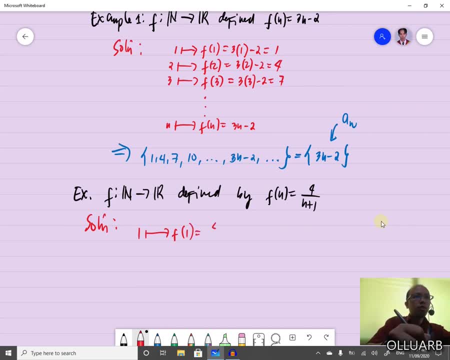 elements of the sequence before up to here. so this is now our sequence, okay and, as you notice here, I'm going to explain again here that we will be focusing all these elements of the sequence before up to here. so this is now our sequence, okay and, as you notice here, I'm going to explain again here that we will be focusing all these. 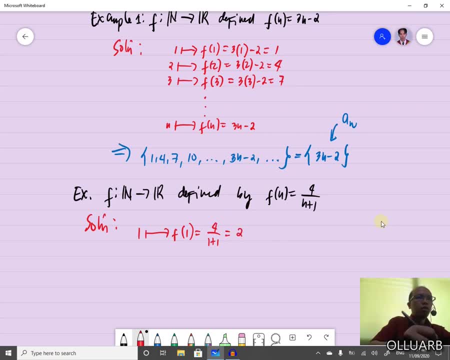 elements of the sequence before up to here. so this is now our sequence, okay and, as you notice here, I'm going to explain again here that we will be focusing all these elements of the sequence before up to here. so this is now our sequence, okay and, as you notice here, I'm going to explain again here that we will be focusing all these. 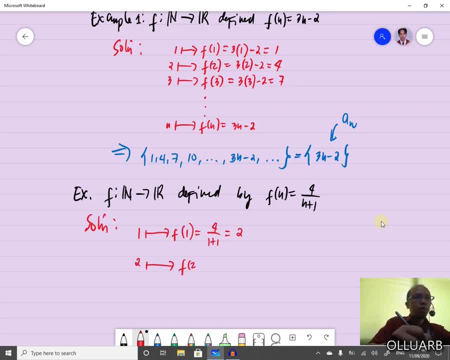 elements of the sequence before up to here. so this is now our sequence, okay and, as you notice here, I'm going to explain again here that we will be focusing all these elements of the sequence before up to here. so this is now our sequence, okay and, as you notice here, I'm going to explain again here that we will be focusing all these. 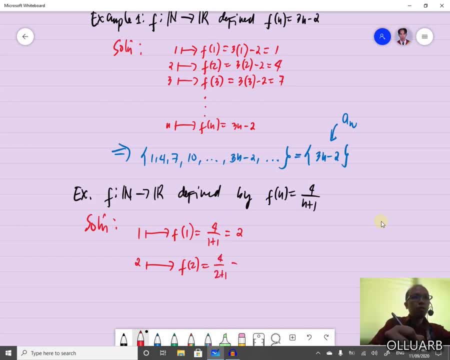 elements of the sequence before up to here. so this is now our sequence, okay and, as you notice here, I'm going to explain again here that we will be focusing all these elements of the sequence before up to here. so this is now our sequence, okay and, as you notice here, I'm going to explain again here that we will be focusing all these. 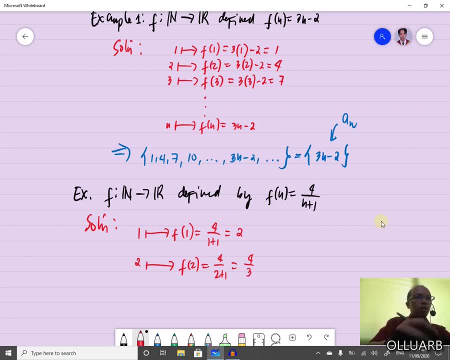 elements of the sequence before up to here. so this is now our sequence, okay and, as you notice here, I'm going to explain again here that we will be focusing all these elements of the sequence before up to here. so this is now our sequence, okay and, as you notice here, I'm going to explain again here that we will be focusing all these. 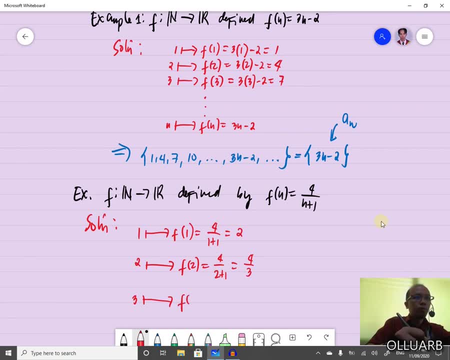 elements of the sequence before up to here. so this is now our sequence, okay and, as you notice here, I'm going to explain again here that we will be focusing all these elements of the sequence before up to here. so this is now our sequence, okay and, as you notice here, I'm going to explain again here that we will be focusing all these. 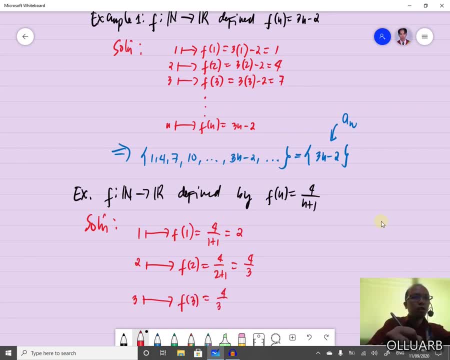 elements of the sequence before up to here. so this is now our sequence, okay and, as you notice here, I'm going to explain again here that we will be focusing all these elements of the sequence before up to here. so this is now our sequence, okay and, as you notice here, I'm going to explain again here that we will be focusing all these. 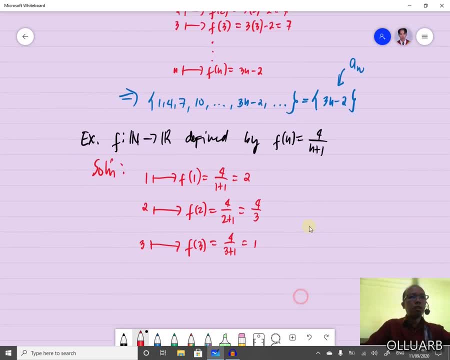 elements of the sequence before up to here. so this is now our sequence, okay and, as you notice here, I'm going to explain again here that we will be focusing all these elements of the sequence before up to here. so this is now our sequence, okay and, as you notice here, I'm going to explain again here that we will be focusing all these. 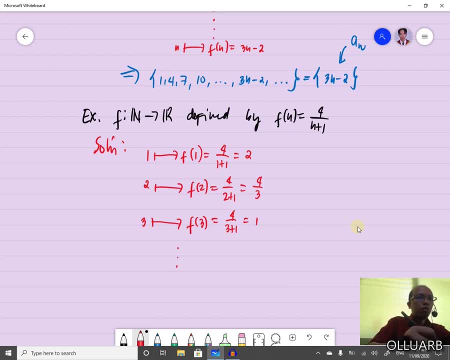 elements of the sequence before up to here. so this is now our sequence, okay and, as you notice here, I'm going to explain again here that we will be focusing all these elements of the sequence before up to here. so this is now our sequence, okay and, as you notice here, I'm going to explain again here that we will be focusing all these. 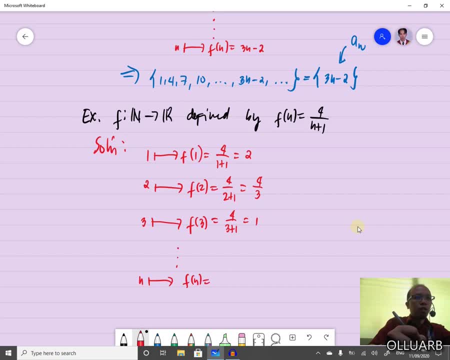 elements of the sequence before up to here. so this is now our sequence, okay and, as you notice here, I'm going to explain again here that we will be focusing all these elements of the sequence before up to here. so this is now our sequence, okay and, as you notice here, I'm going to explain again here that we will be focusing all these. 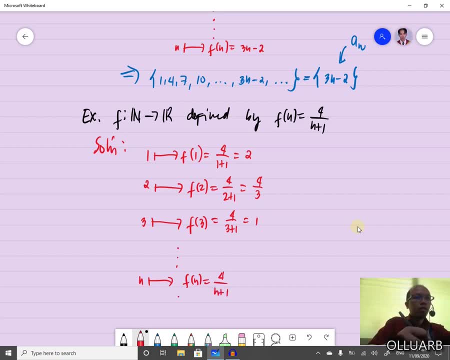 elements of the sequence before up to here. so this is now our sequence, okay and, as you notice here, I'm going to explain again here that we will be focusing all these elements of the sequence before up to here. so this is now our sequence, okay and, as you notice here, I'm going to explain again here that we will be focusing all these. 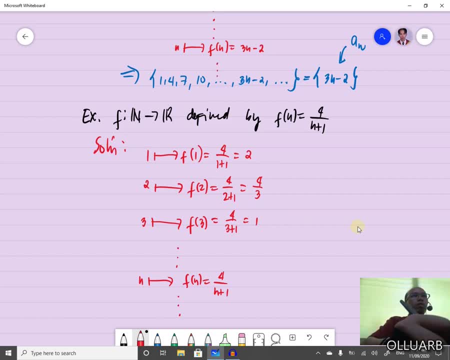 elements of the sequence before up to here. so this is now our sequence, okay and, as you notice here, I'm going to explain again here that we will be focusing all these elements of the sequence before up to here. so this is now our sequence, okay and, as you notice here, I'm going to explain again here that we will be focusing all these. 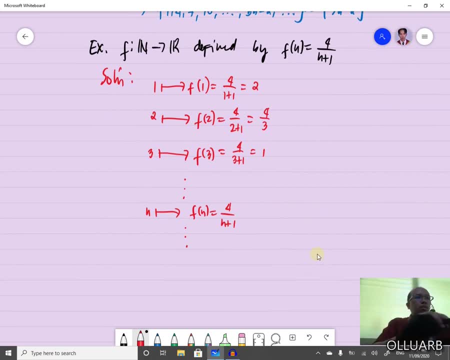 elements of the sequence before up to here. so this is now our sequence, okay and, as you notice here, I'm going to explain again here that we will be focusing all these elements of the sequence before up to here. so this is now our sequence, okay and, as you notice here, I'm going to explain again here that we will be focusing all these. 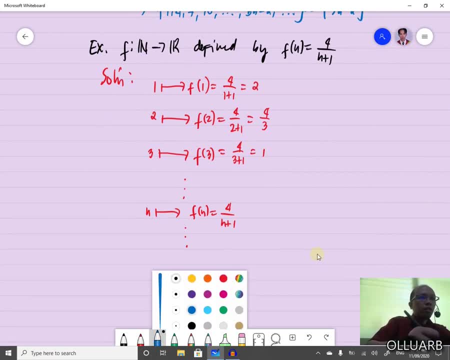 elements of the sequence before up to here. so this is now our sequence, okay and, as you notice here, I'm going to explain again here that we will be focusing all these elements of the sequence before up to here. so this is now our sequence, okay and, as you notice here, I'm going to explain again here that we will be focusing all these. 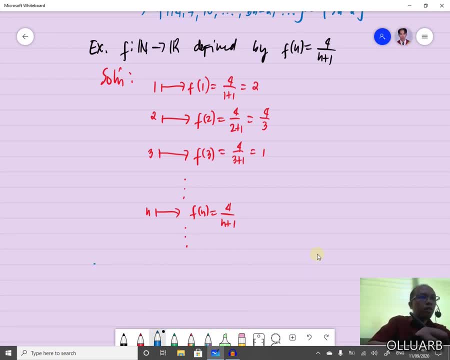 elements of the sequence before up to here. so this is now our sequence, okay and, as you notice here, I'm going to explain again here that we will be focusing all these elements of the sequence before up to here. so this is now our sequence, okay and, as you notice here, I'm going to explain again here that we will be focusing all these. 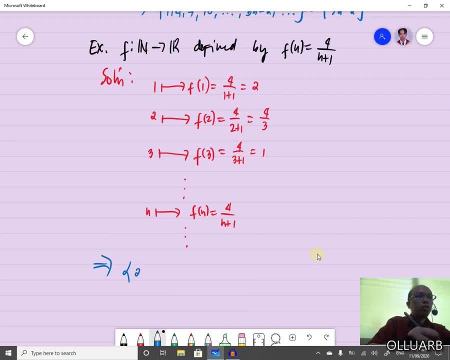 elements of the sequence before up to here. so this is now our sequence, okay and, as you notice here, I'm going to explain again here that we will be focusing all these elements of the sequence before up to here. so this is now our sequence, okay and, as you notice here, I'm going to explain again here that we will be focusing all these. 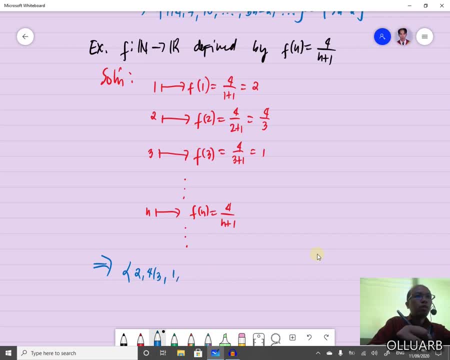 elements of the sequence before up to here. so this is now our sequence, okay and, as you notice here, I'm going to explain again here that we will be focusing all these elements of the sequence before up to here. so this is now our sequence, okay and, as you notice here, I'm going to explain again here that we will be focusing all these. 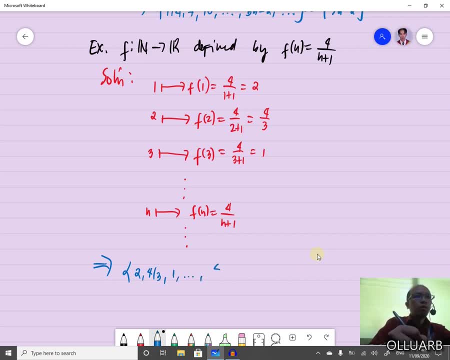 elements of the sequence before up to here. so this is now our sequence, okay and, as you notice here, I'm going to explain again here that we will be focusing all these elements of the sequence before up to here. so this is now our sequence, okay and, as you notice here, I'm going to explain again here that we will be focusing all these. 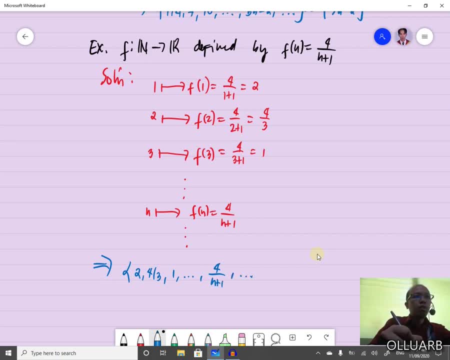 elements of the sequence before up to here. so this is now our sequence, okay and, as you notice here, I'm going to explain again here that we will be focusing all these elements of the sequence before up to here. so this is now our sequence, okay and, as you notice here, I'm going to explain again here that we will be focusing all these. 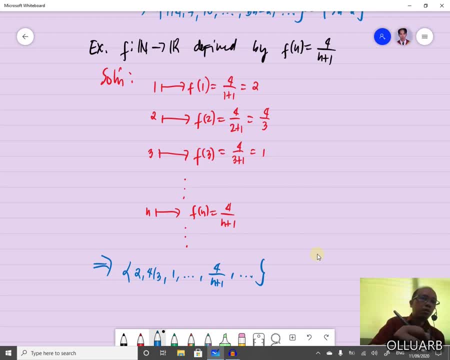 elements of the sequence before up to here. so this is now our sequence, okay and, as you notice here, I'm going to explain again here that we will be focusing all these elements of the sequence before up to here. so this is now our sequence, okay and, as you notice here, I'm going to explain again here that we will be focusing all these. 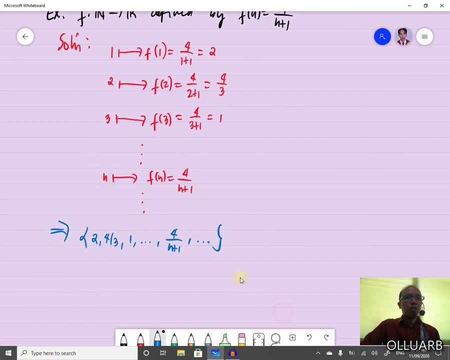 elements of the sequence before up to here. so this is now our sequence, okay and, as you notice here, I'm going to explain again here that we will be focusing all these elements of the sequence before up to here. so this is now our sequence, okay and, as you notice here, I'm going to explain again here that we will be focusing all these. 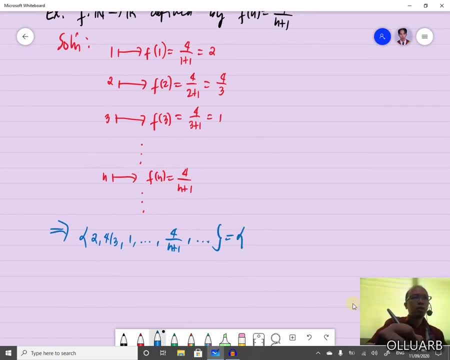 elements of the sequence before up to here. so this is now our sequence, okay and, as you notice here, I'm going to explain again here that we will be focusing all these elements of the sequence before up to here. so this is now our sequence, okay and, as you notice here, I'm going to explain again here that we will be focusing all these. 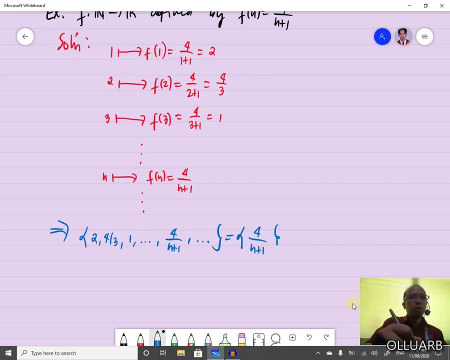 elements of the sequence before up to here. so this is now our sequence, okay and, as you notice here, I'm going to explain again here that we will be focusing all these elements of the sequence before up to here. so this is now our sequence, okay and, as you notice here, I'm going to explain again here that we will be focusing all these. 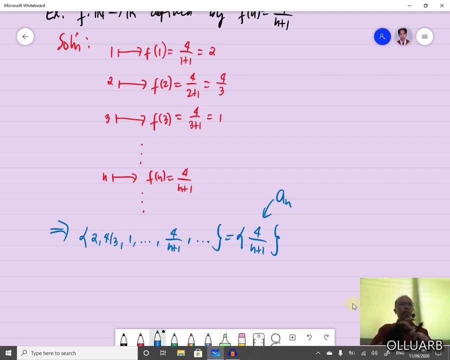 elements of the sequence before up to here. so this is now our sequence, okay and, as you notice here, I'm going to explain again here that we will be focusing all these elements of the sequence before up to here. so this is now our sequence, okay and, as you notice here, I'm going to explain again here that we will be focusing all these. 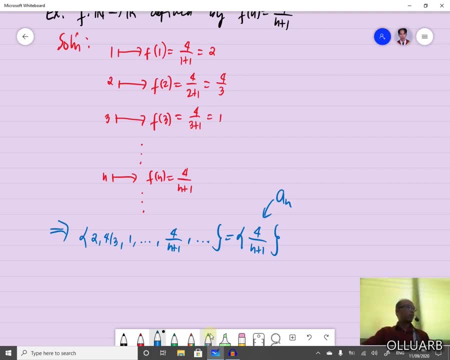 elements of the sequence before up to here. so this is now our sequence, okay and, as you notice here, I'm going to explain again here that we will be focusing all these elements of the sequence before up to here. so this is now our sequence, okay and, as you notice here, I'm going to explain again here that we will be focusing all these. 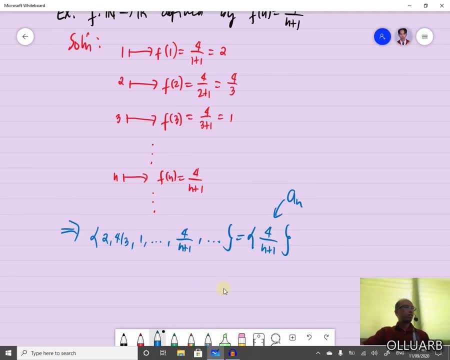 elements of the sequence before up to here. so this is now our sequence, okay and, as you notice here, I'm going to explain again here that we will be focusing all these elements of the sequence before up to here. so this is now our sequence, okay and, as you notice here, I'm going to explain again here that we will be focusing all these. 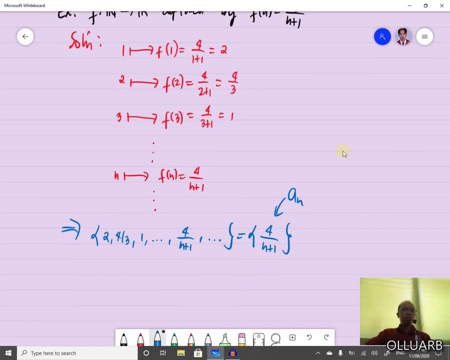 elements of the sequence before up to here. so this is now our sequence, okay and, as you notice here, I'm going to explain again here that we will be focusing all these elements of the sequence before up to here. so this is now our sequence, okay and, as you notice here, I'm going to explain again here that we will be focusing all these. 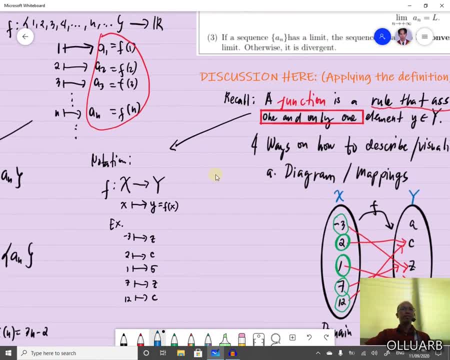 elements of the sequence before up to here. so this is now our sequence, okay and, as you notice here, I'm going to explain again here that we will be focusing all these elements of the sequence before up to here. so this is now our sequence, okay and, as you notice here, I'm going to explain again here that we will be focusing all these. 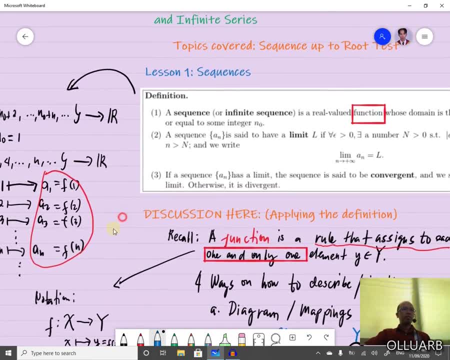 elements of the sequence before up to here. so this is now our sequence, okay and, as you notice here, I'm going to explain again here that we will be focusing all these elements of the sequence before up to here. so this is now our sequence, okay and, as you notice here, I'm going to explain again here that we will be focusing all these. 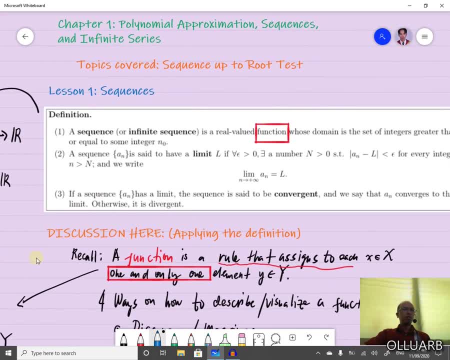 elements of the sequence before up to here. so this is now our sequence, okay and, as you notice here, I'm going to explain again here that we will be focusing all these elements of the sequence before up to here. so this is now our sequence, okay and, as you notice here, I'm going to explain again here that we will be focusing all these. 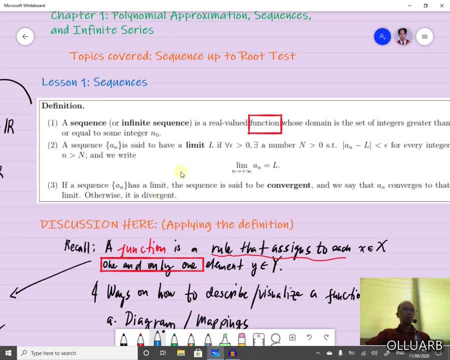 elements of the sequence before up to here. so this is now our sequence, okay and, as you notice here, I'm going to explain again here that we will be focusing all these elements of the sequence before up to here. so this is now our sequence, okay and, as you notice here, I'm going to explain again here that we will be focusing all these. 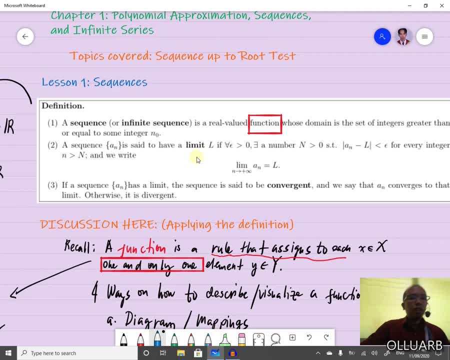 elements of the sequence before up to here. so this is now our sequence, okay and, as you notice here, I'm going to explain again here that we will be focusing all these elements of the sequence before up to here. so this is now our sequence, okay and, as you notice here, I'm going to explain again here that we will be focusing all these. 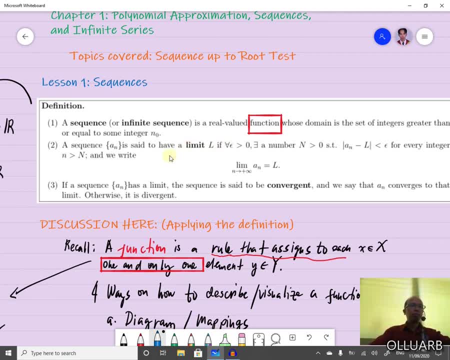 elements of the sequence before up to here. so this is now our sequence, okay and, as you notice here, I'm going to explain again here that we will be focusing all these elements of the sequence before up to here. so this is now our sequence, okay and, as you notice here, I'm going to explain again here that we will be focusing all these. 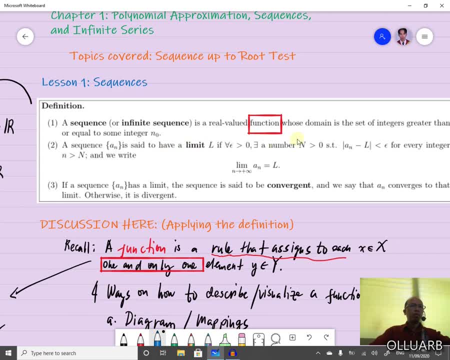 elements of the sequence before up to here. so this is now our sequence, okay and, as you notice here, I'm going to explain again here that we will be focusing all these elements of the sequence before up to here. so this is now our sequence, okay and, as you notice here, I'm going to explain again here that we will be focusing all these. 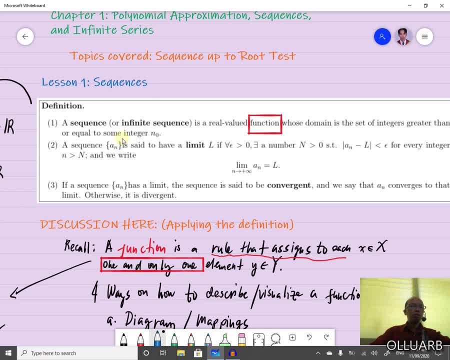 elements of the sequence before up to here. so this is now our sequence, okay and, as you notice here, I'm going to explain again here that we will be focusing all these elements of the sequence before up to here. so this is now our sequence, okay and, as you notice here, I'm going to explain again here that we will be focusing all these. 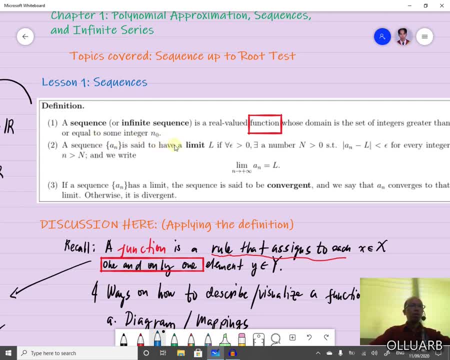 elements of the sequence before up to here. so this is now our sequence, okay and, as you notice here, I'm going to explain again here that we will be focusing all these elements of the sequence before up to here. so this is now our sequence, okay and, as you notice here, I'm going to explain again here that we will be focusing all these. 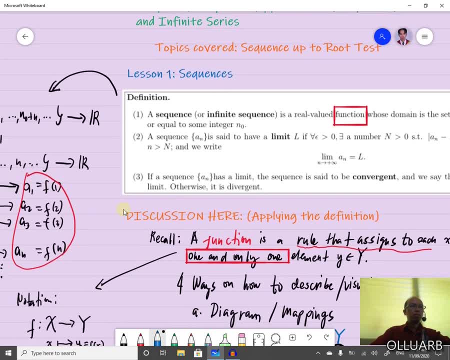 elements of the sequence before up to here. so this is now our sequence, okay and, as you notice here, I'm going to explain again here that we will be focusing all these elements of the sequence before up to here. so this is now our sequence, okay and, as you notice here, I'm going to explain again here that we will be focusing all these. 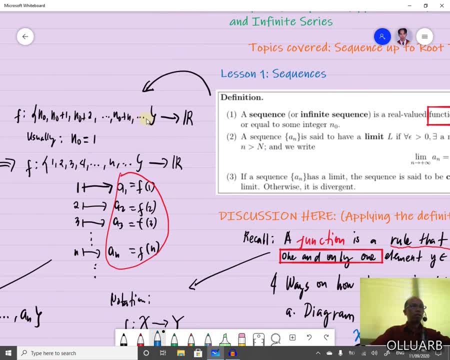 elements of the sequence before up to here. so this is now our sequence, okay and, as you notice here, I'm going to explain again here that we will be focusing all these elements of the sequence before up to here. so this is now our sequence, okay and, as you notice here, I'm going to explain again here that we will be focusing all these. 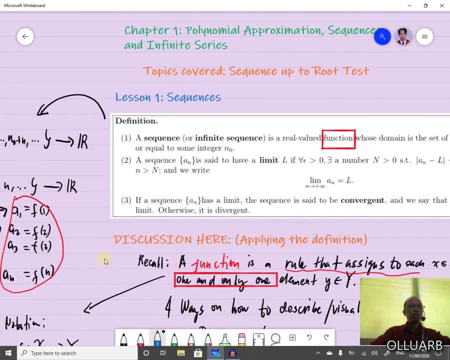 elements of the sequence before up to here. so this is now our sequence, okay and, as you notice here, I'm going to explain again here that we will be focusing all these elements of the sequence before up to here. so this is now our sequence, okay and, as you notice here, I'm going to explain again here that we will be focusing all these. 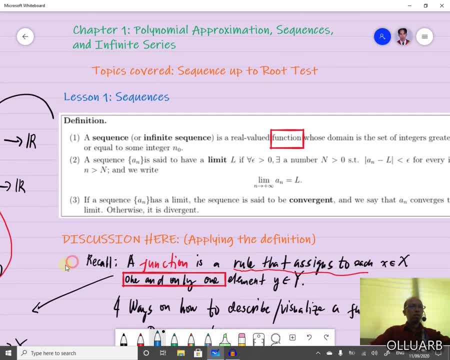 elements of the sequence before up to here. so this is now our sequence, okay and, as you notice here, I'm going to explain again here that we will be focusing all these elements of the sequence before up to here. so this is now our sequence, okay and, as you notice here, I'm going to explain again here that we will be focusing all these. 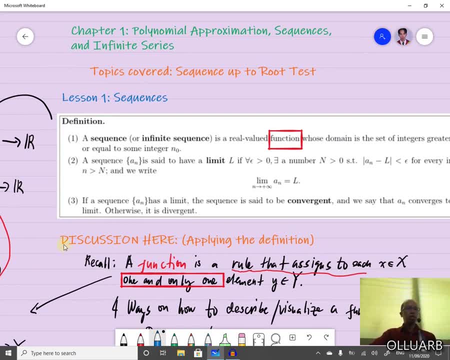 elements of the sequence before up to here. so this is now our sequence, okay and, as you notice here, I'm going to explain again here that we will be focusing all these elements of the sequence before up to here. so this is now our sequence, okay and, as you notice here, I'm going to explain again here that we will be focusing all these. 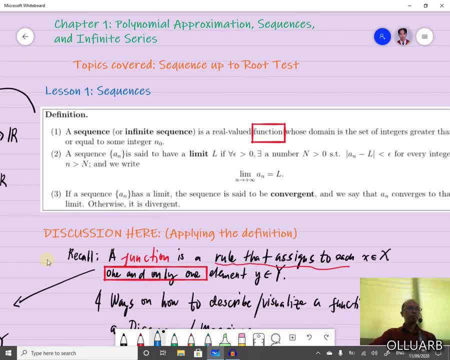 elements of the sequence before up to here. so this is now our sequence, okay and, as you notice here, I'm going to explain again here that we will be focusing all these elements of the sequence before up to here. so this is now our sequence, okay and, as you notice here, I'm going to explain again here that we will be focusing all these. 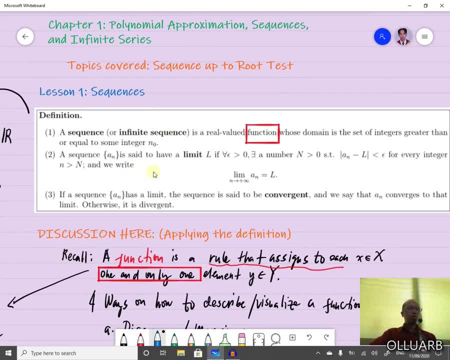 elements of the sequence before up to here. so this is now our sequence, okay and, as you notice here, I'm going to explain again here that we will be focusing all these elements of the sequence before up to here. so this is now our sequence, okay and, as you notice here, I'm going to explain again here that we will be focusing all these. 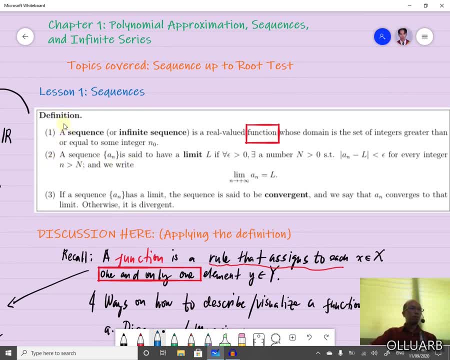 elements of the sequence before up to here. so this is now our sequence, okay and, as you notice here, I'm going to explain again here that we will be focusing all these elements of the sequence before up to here. so this is now our sequence, okay and, as you notice here, I'm going to explain again here that we will be focusing all these. 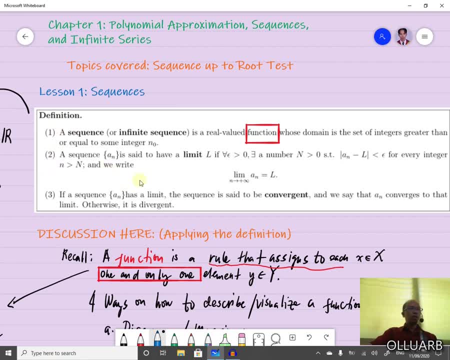 elements of the sequence before up to here. so this is now our sequence, okay and, as you notice here, I'm going to explain again here that we will be focusing all these elements of the sequence before up to here. so this is now our sequence, okay and, as you notice here, I'm going to explain again here that we will be focusing all these. 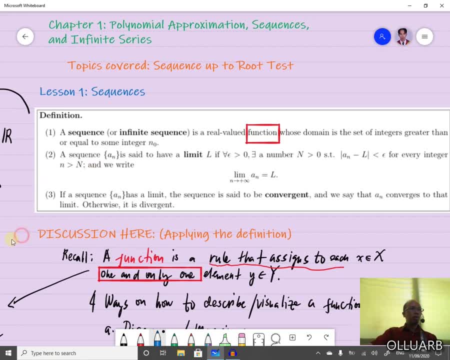 elements of the sequence before up to here. so this is now our sequence, okay and, as you notice here, I'm going to explain again here that we will be focusing all these elements of the sequence before up to here. so this is now our sequence, okay and, as you notice here, I'm going to explain again here that we will be focusing all these. 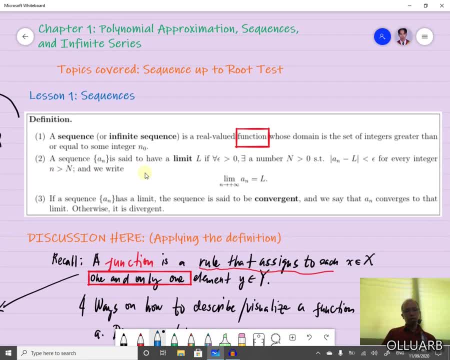 elements of the sequence before up to here. so this is now our sequence, okay and, as you notice here, I'm going to explain again here that we will be focusing all these elements of the sequence before up to here. so this is now our sequence, okay and, as you notice here, I'm going to explain again here that we will be focusing all these. 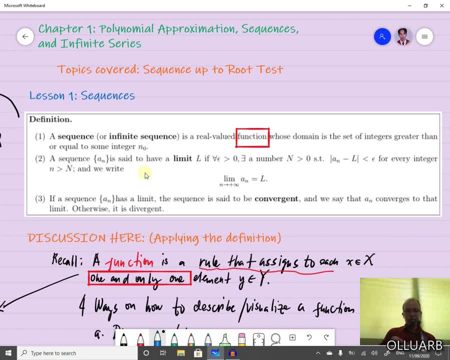 elements of the sequence before up to here. so this is now our sequence, okay and, as you notice here, I'm going to explain again here that we will be focusing all these elements of the sequence before up to here. so this is now our sequence, okay and, as you notice here, I'm going to explain again here that we will be focusing all these. 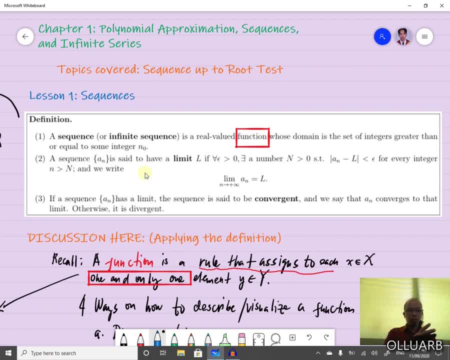 elements of the sequence before up to here. so this is now our sequence, okay and, as you notice here, I'm going to explain again here that we will be focusing all these elements of the sequence before up to here. so this is now our sequence, okay and, as you notice here, I'm going to explain again here that we will be focusing all these. 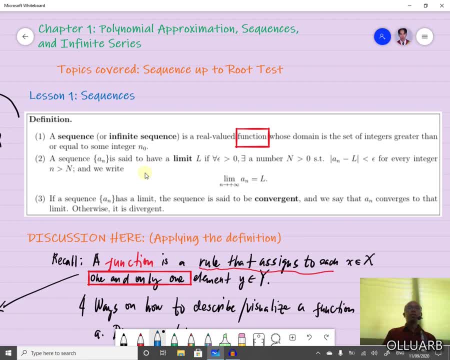 elements of the sequence before up to here. so this is now our sequence, okay and, as you notice here, I'm going to explain again here that we will be focusing all these elements of the sequence before up to here. so this is now our sequence, okay and, as you notice here, I'm going to explain again here that we will be focusing all these. 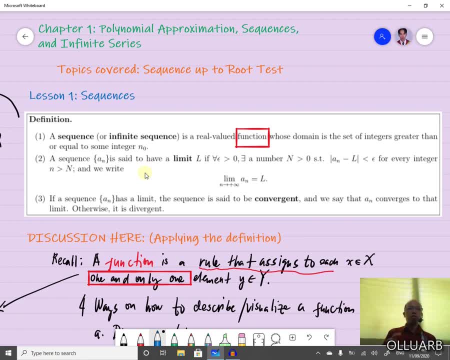 elements of the sequence before up to here. so this is now our sequence, okay and, as you notice here, I'm going to explain again here that we will be focusing all these elements of the sequence before up to here. so this is now our sequence, okay and, as you notice here, I'm going to explain again here that we will be focusing all these. 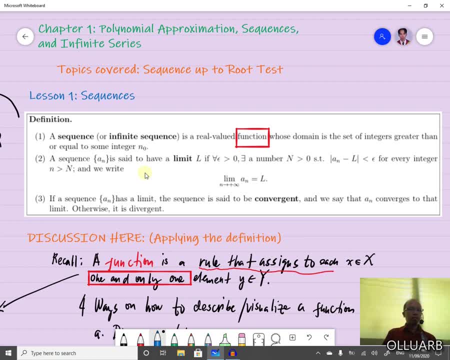 elements of the sequence before up to here. so this is now our sequence, okay and, as you notice here, I'm going to explain again here that we will be focusing all these elements of the sequence before up to here. so this is now our sequence, okay and, as you notice here, I'm going to explain again here that we will be focusing all these. 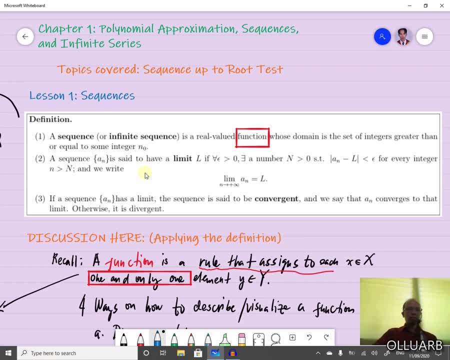 elements of the sequence before up to here. so this is now our sequence, okay and, as you notice here, I'm going to explain again here that we will be focusing all these elements of the sequence before up to here. so this is now our sequence, okay and, as you notice here, I'm going to explain again here that we will be focusing all these. 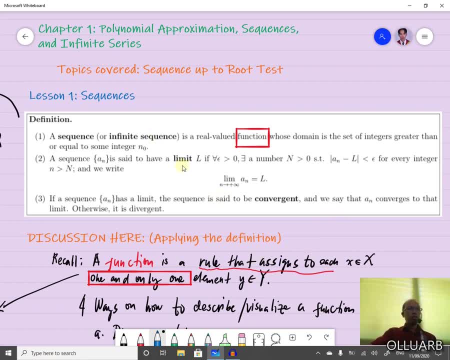 elements of the sequence before up to here. so this is now our sequence, okay and, as you notice here, I'm going to explain again here that we will be focusing all these elements of the sequence before up to here. so this is now our sequence, okay and, as you notice here, I'm going to explain again here that we will be focusing all these. 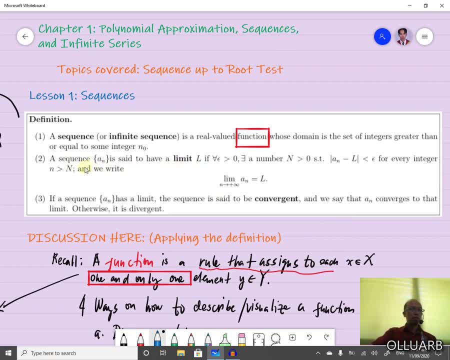 elements of the sequence before up to here. so this is now our sequence, okay and, as you notice here, I'm going to explain again here that we will be focusing all these elements of the sequence before up to here. so this is now our sequence, okay and, as you notice here, I'm going to explain again here that we will be focusing all these. 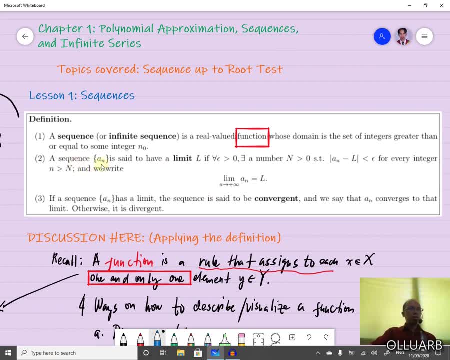 elements of the sequence before up to here. so this is now our sequence, okay and, as you notice here, I'm going to explain again here that we will be focusing all these elements of the sequence before up to here. so this is now our sequence, okay and, as you notice here, I'm going to explain again here that we will be focusing all these. 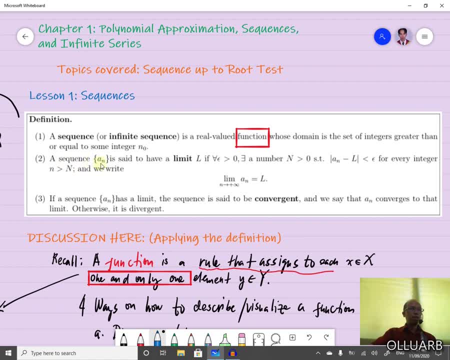 elements of the sequence before up to here. so this is now our sequence, okay and, as you notice here, I'm going to explain again here that we will be focusing all these elements of the sequence before up to here. so this is now our sequence, okay and, as you notice here, I'm going to explain again here that we will be focusing all these. 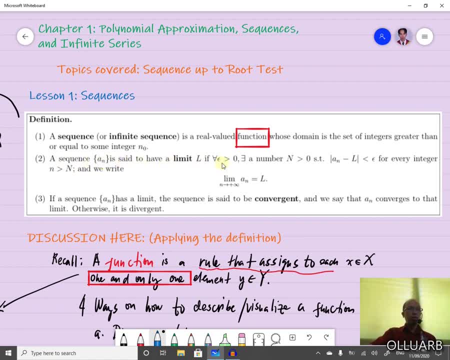 elements of the sequence before up to here. so this is now our sequence, okay and, as you notice here, I'm going to explain again here that we will be focusing all these elements of the sequence before up to here. so this is now our sequence, okay and, as you notice here, I'm going to explain again here that we will be focusing all these. 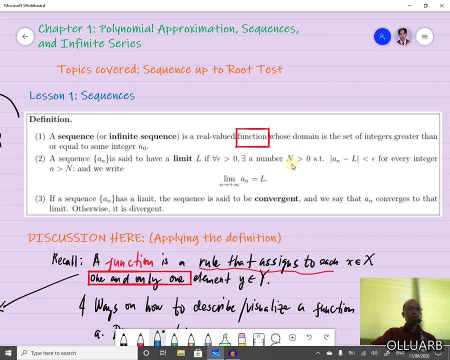 elements of the sequence before up to here. so this is now our sequence, okay and, as you notice here, I'm going to explain again here that we will be focusing all these elements of the sequence before up to here. so this is now our sequence, okay and, as you notice here, I'm going to explain again here that we will be focusing all these. 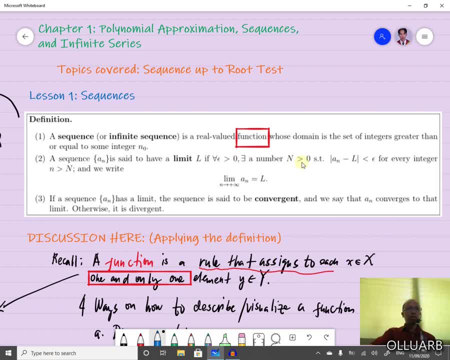 elements of the sequence before up to here. so this is now our sequence, okay and, as you notice here, I'm going to explain again here that we will be focusing all these elements of the sequence before up to here. so this is now our sequence, okay and, as you notice here, I'm going to explain again here that we will be focusing all these. 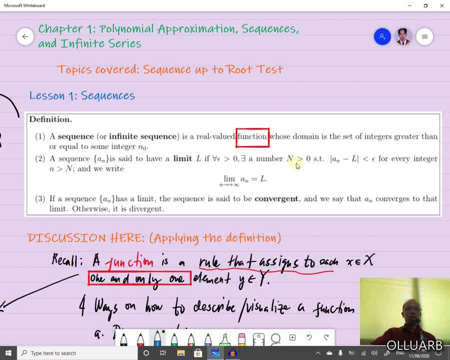 elements of the sequence before up to here. so this is now our sequence, okay and, as you notice here, I'm going to explain again here that we will be focusing all these elements of the sequence before up to here. so this is now our sequence, okay and, as you notice here, I'm going to explain again here that we will be focusing all these. 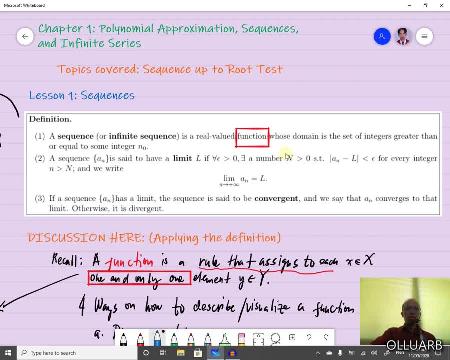 elements of the sequence before up to here. so this is now our sequence, okay and, as you notice here, I'm going to explain again here that we will be focusing all these elements of the sequence before up to here. so this is now our sequence, okay and, as you notice here, I'm going to explain again here that we will be focusing all these. 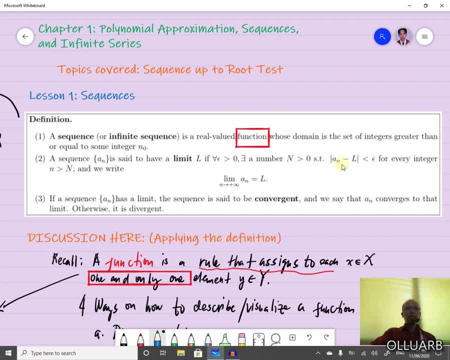 elements of the sequence before up to here. so this is now our sequence, okay and, as you notice here, I'm going to explain again here that we will be focusing all these elements of the sequence before up to here. so this is now our sequence, okay and, as you notice here, I'm going to explain again here that we will be focusing all these. 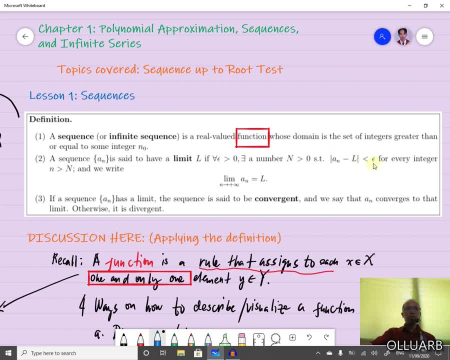 elements of the sequence before up to here. so this is now our sequence, okay and, as you notice here, I'm going to explain again here that we will be focusing all these elements of the sequence before up to here. so this is now our sequence, okay and, as you notice here, I'm going to explain again here that we will be focusing all these. 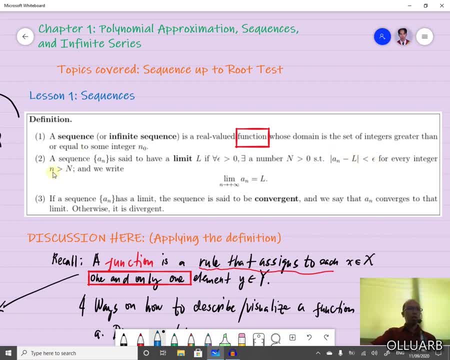 elements of the sequence before up to here. so this is now our sequence, okay and, as you notice here, I'm going to explain again here that we will be focusing all these elements of the sequence before up to here. so this is now our sequence, okay and, as you notice here, I'm going to explain again here that we will be focusing all these. 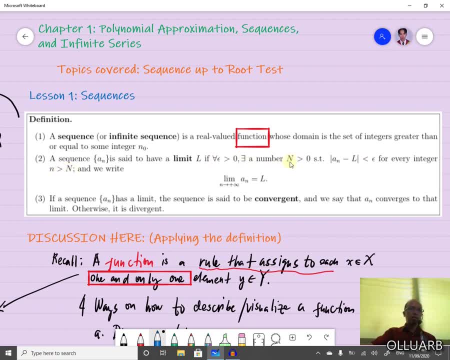 elements of the sequence before up to here. so this is now our sequence, okay and, as you notice here, I'm going to explain again here that we will be focusing all these elements of the sequence before up to here. so this is now our sequence, okay and, as you notice here, I'm going to explain again here that we will be focusing all these. 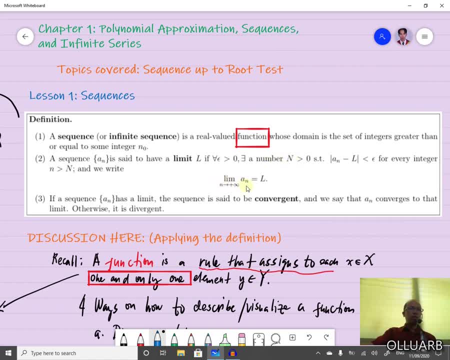 elements of the sequence before up to here. so this is now our sequence, okay and, as you notice here, I'm going to explain again here that we will be focusing all these elements of the sequence before up to here. so this is now our sequence, okay and, as you notice here, I'm going to explain again here that we will be focusing all these. 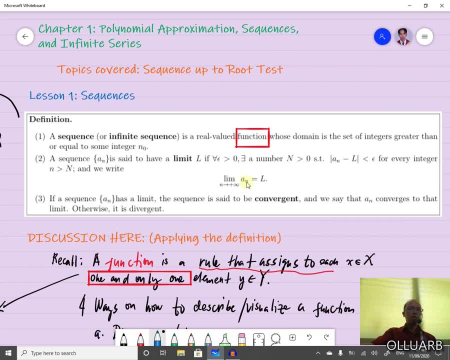 elements of the sequence before up to here. so this is now our sequence, okay and, as you notice here, I'm going to explain again here that we will be focusing all these elements of the sequence before up to here. so this is now our sequence, okay and, as you notice here, I'm going to explain again here that we will be focusing all these. 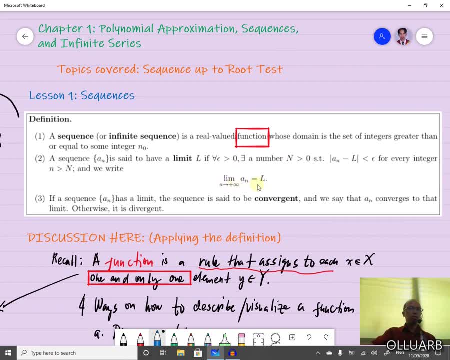 elements of the sequence before up to here. so this is now our sequence, okay and, as you notice here, I'm going to explain again here that we will be focusing all these elements of the sequence before up to here. so this is now our sequence, okay and, as you notice here, I'm going to explain again here that we will be focusing all these. 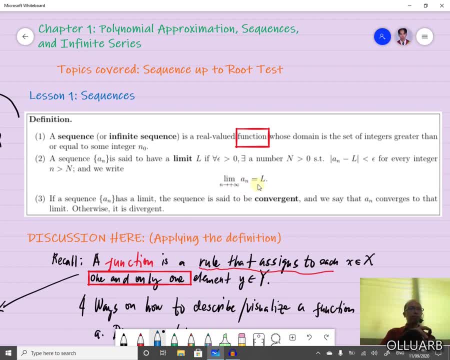 elements of the sequence before up to here. so this is now our sequence, okay and, as you notice here, I'm going to explain again here that we will be focusing all these elements of the sequence before up to here. so this is now our sequence, okay and, as you notice here, I'm going to explain again here that we will be focusing all these. 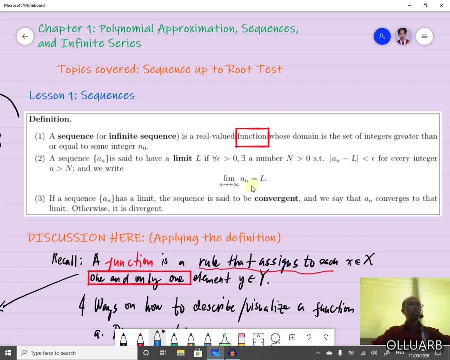 elements of the sequence before up to here. so this is now our sequence, okay and, as you notice here, I'm going to explain again here that we will be focusing all these elements of the sequence before up to here. so this is now our sequence, okay and, as you notice here, I'm going to explain again here that we will be focusing all these. 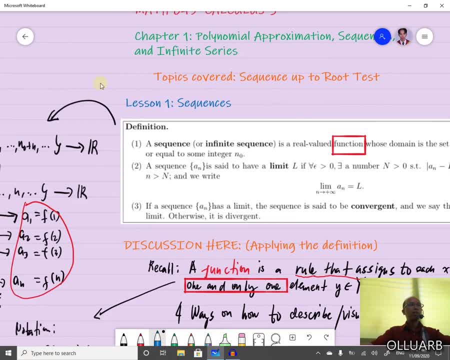 elements of the sequence before up to here. so this is now our sequence, okay and, as you notice here, I'm going to explain again here that we will be focusing all these elements of the sequence before up to here. so this is now our sequence, okay and, as you notice here, I'm going to explain again here that we will be focusing all these. 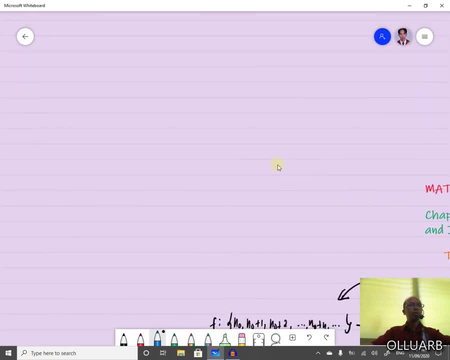 elements of the sequence before up to here. so this is now our sequence, okay and, as you notice here, I'm going to explain again here that we will be focusing all these elements of the sequence before up to here. so this is now our sequence, okay and, as you notice here, I'm going to explain again here that we will be focusing all these. 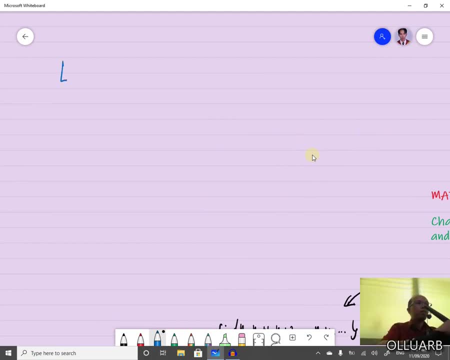 elements of the sequence before up to here. so this is now our sequence, okay and, as you notice here, I'm going to explain again here that we will be focusing all these elements of the sequence before up to here. so this is now our sequence, okay and, as you notice here, I'm going to explain again here that we will be focusing all these. 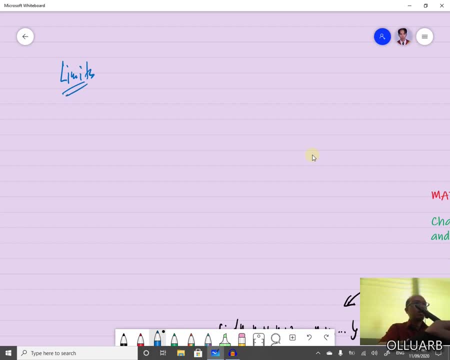 elements of the sequence before up to here. so this is now our sequence, okay and, as you notice here, I'm going to explain again here that we will be focusing all these elements of the sequence before up to here. so this is now our sequence, okay and, as you notice here, I'm going to explain again here that we will be focusing all these. 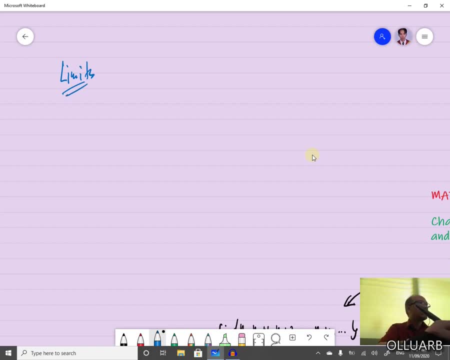 elements of the sequence before up to here. so this is now our sequence, okay and, as you notice here, I'm going to explain again here that we will be focusing all these elements of the sequence before up to here. so this is now our sequence, okay and, as you notice here, I'm going to explain again here that we will be focusing all these. 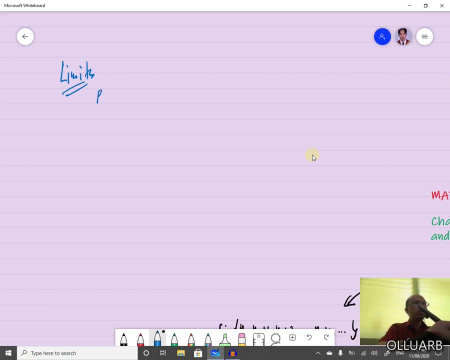 elements of the sequence before up to here. so this is now our sequence, okay and, as you notice here, I'm going to explain again here that we will be focusing all these elements of the sequence before up to here. so this is now our sequence, okay and, as you notice here, I'm going to explain again here that we will be focusing all these. 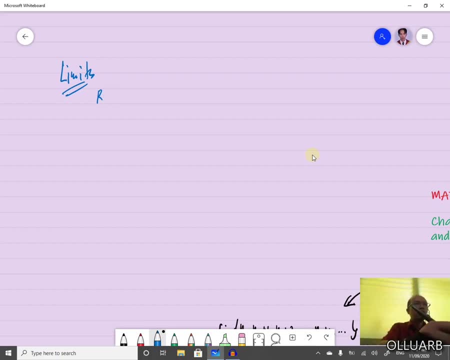 elements of the sequence before up to here. so this is now our sequence, okay and, as you notice here, I'm going to explain again here that we will be focusing all these elements of the sequence before up to here. so this is now our sequence, okay and, as you notice here, I'm going to explain again here that we will be focusing all these. 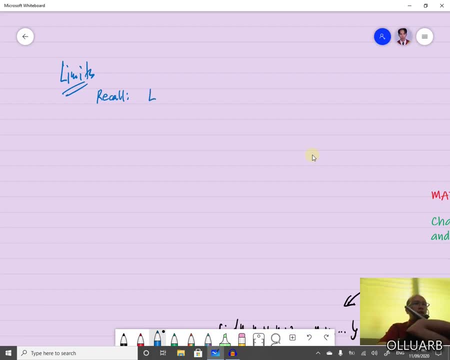 elements of the sequence before up to here. so this is now our sequence, okay and, as you notice here, I'm going to explain again here that we will be focusing all these elements of the sequence before up to here. so this is now our sequence, okay and, as you notice here, I'm going to explain again here that we will be focusing all these. 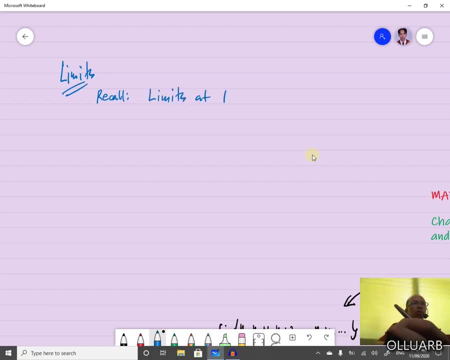 elements of the sequence before up to here. so this is now our sequence, okay and, as you notice here, I'm going to explain again here that we will be focusing all these elements of the sequence before up to here. so this is now our sequence, okay and, as you notice here, I'm going to explain again here that we will be focusing all these. 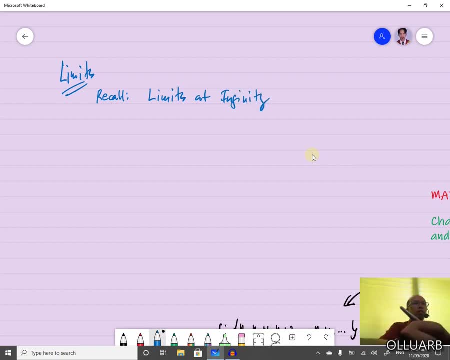 elements of the sequence before up to here. so this is now our sequence, okay and, as you notice here, I'm going to explain again here that we will be focusing all these elements of the sequence before up to here. so this is now our sequence, okay and, as you notice here, I'm going to explain again here that we will be focusing all these. 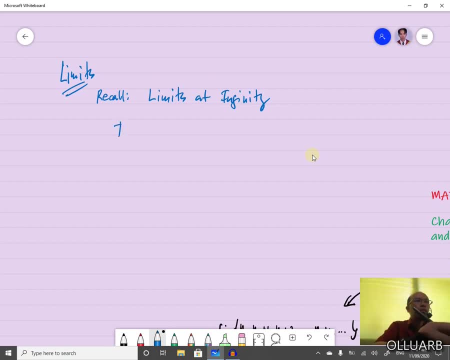 elements of the sequence before up to here. so this is now our sequence, okay and, as you notice here, I'm going to explain again here that we will be focusing all these elements of the sequence before up to here. so this is now our sequence, okay and, as you notice here, I'm going to explain again here that we will be focusing all these. 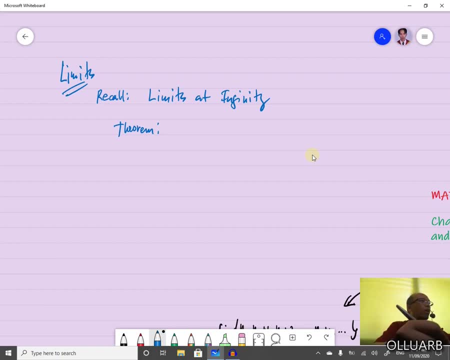 elements of the sequence before up to here. so this is now our sequence, okay and, as you notice here, I'm going to explain again here that we will be focusing all these elements of the sequence before up to here. so this is now our sequence, okay and, as you notice here, I'm going to explain again here that we will be focusing all these. 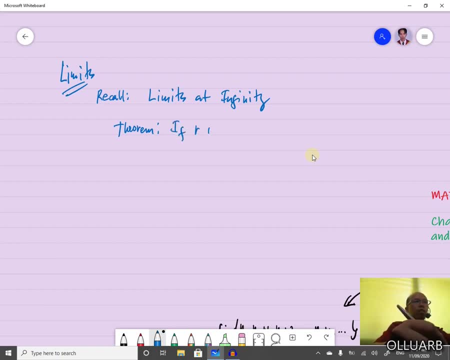 elements of the sequence before up to here. so this is now our sequence, okay and, as you notice here, I'm going to explain again here that we will be focusing all these elements of the sequence before up to here. so this is now our sequence, okay and, as you notice here, I'm going to explain again here that we will be focusing all these. 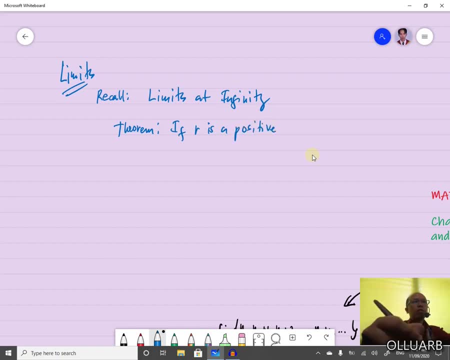 elements of the sequence before up to here. so this is now our sequence, okay and, as you notice here, I'm going to explain again here that we will be focusing all these elements of the sequence before up to here. so this is now our sequence, okay and, as you notice here, I'm going to explain again here that we will be focusing all these. 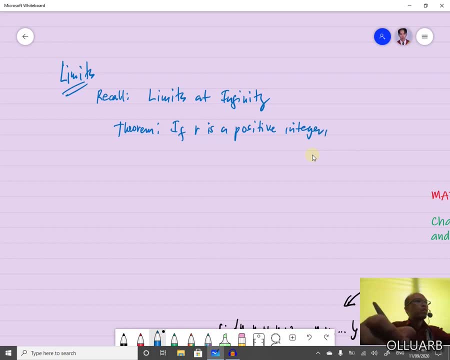 elements of the sequence before up to here. so this is now our sequence, okay and, as you notice here, I'm going to explain again here that we will be focusing all these elements of the sequence before up to here. so this is now our sequence, okay and, as you notice here, I'm going to explain again here that we will be focusing all these. 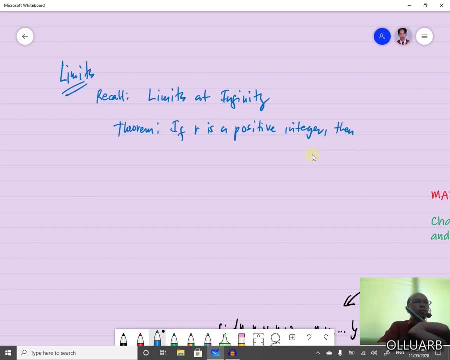 elements of the sequence before up to here. so this is now our sequence, okay and, as you notice here, I'm going to explain again here that we will be focusing all these elements of the sequence before up to here. so this is now our sequence, okay and, as you notice here, I'm going to explain again here that we will be focusing all these. 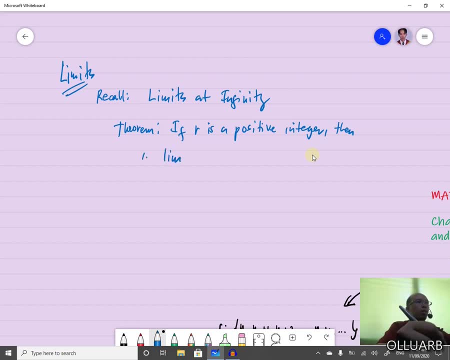 elements of the sequence before up to here. so this is now our sequence, okay and, as you notice here, I'm going to explain again here that we will be focusing all these elements of the sequence before up to here. so this is now our sequence, okay and, as you notice here, I'm going to explain again here that we will be focusing all these. 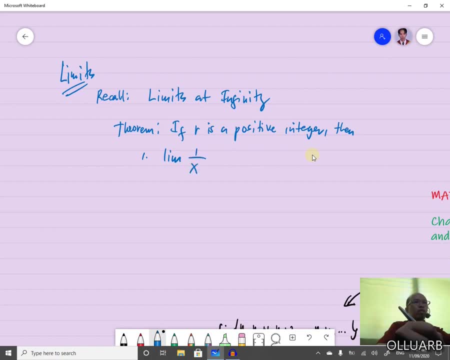 elements of the sequence before up to here. so this is now our sequence, okay and, as you notice here, I'm going to explain again here that we will be focusing all these elements of the sequence before up to here. so this is now our sequence, okay and, as you notice here, I'm going to explain again here that we will be focusing all these. 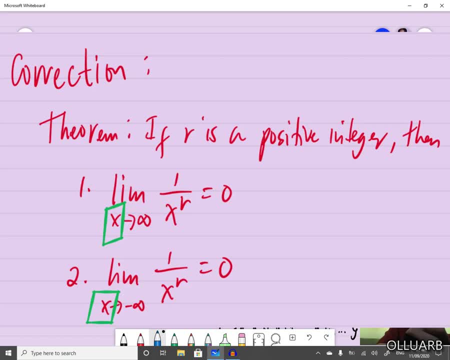 elements of the sequence before up to here. so this is now our sequence, okay and, as you notice here, I'm going to explain again here that we will be focusing all these elements of the sequence before up to here. so this is now our sequence, okay and, as you notice here, I'm going to explain again here that we will be focusing all these. 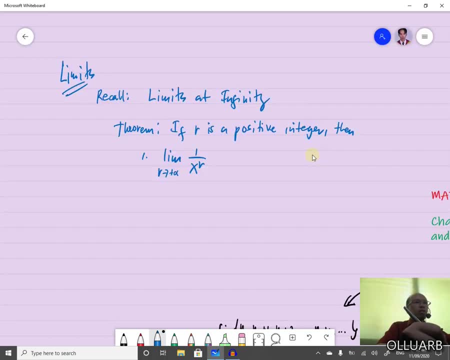 elements of the sequence before up to here. so this is now our sequence, okay and, as you notice here, I'm going to explain again here that we will be focusing all these elements of the sequence before up to here. so this is now our sequence, okay and, as you notice here, I'm going to explain again here that we will be focusing all these. 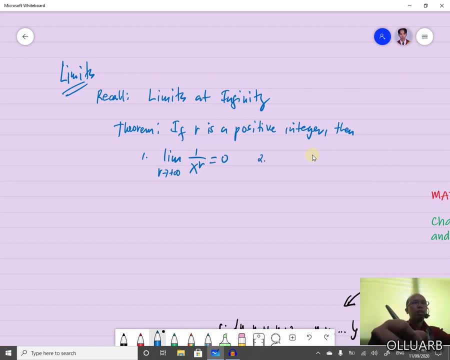 elements of the sequence before up to here. so this is now our sequence, okay and, as you notice here, I'm going to explain again here that we will be focusing all these elements of the sequence before up to here. so this is now our sequence, okay and, as you notice here, I'm going to explain again here that we will be focusing all these. 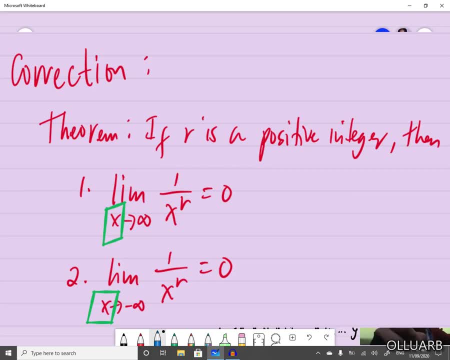 elements of the sequence before up to here. so this is now our sequence, okay and, as you notice here, I'm going to explain again here that we will be focusing all these elements of the sequence before up to here. so this is now our sequence, okay and, as you notice here, I'm going to explain again here that we will be focusing all these. 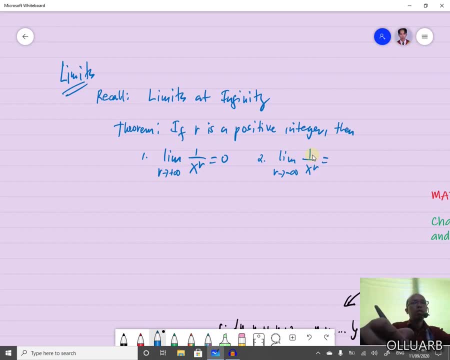 elements of the sequence before up to here. so this is now our sequence, okay and, as you notice here, I'm going to explain again here that we will be focusing all these elements of the sequence before up to here. so this is now our sequence, okay and, as you notice here, I'm going to explain again here that we will be focusing all these. 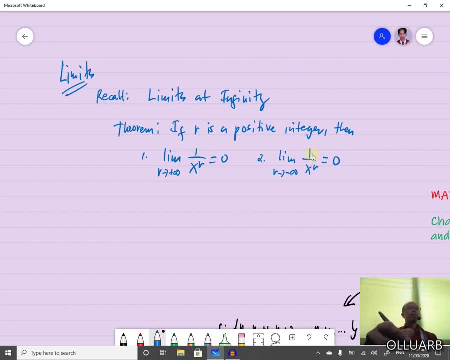 elements of the sequence before up to here. so this is now our sequence, okay and, as you notice here, I'm going to explain again here that we will be focusing all these elements of the sequence before up to here. so this is now our sequence, okay and, as you notice here, I'm going to explain again here that we will be focusing all these. 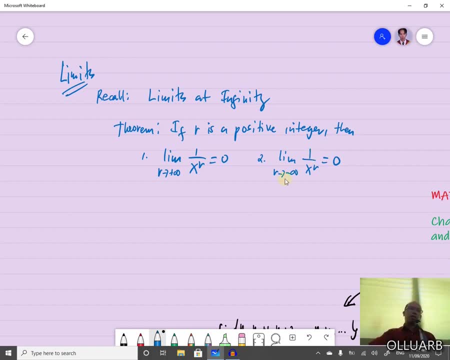 elements of the sequence before up to here. so this is now our sequence, okay and, as you notice here, I'm going to explain again here that we will be focusing all these elements of the sequence before up to here. so this is now our sequence, okay and, as you notice here, I'm going to explain again here that we will be focusing all these. 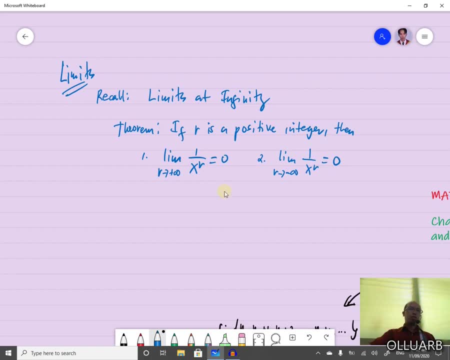 elements of the sequence before up to here. so this is now our sequence, okay and, as you notice here, I'm going to explain again here that we will be focusing all these elements of the sequence before up to here. so this is now our sequence, okay and, as you notice here, I'm going to explain again here that we will be focusing all these. 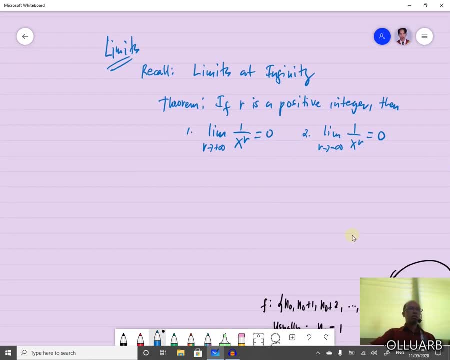 elements of the sequence before up to here. so this is now our sequence, okay and, as you notice here, I'm going to explain again here that we will be focusing all these elements of the sequence before up to here. so this is now our sequence, okay and, as you notice here, I'm going to explain again here that we will be focusing all these. 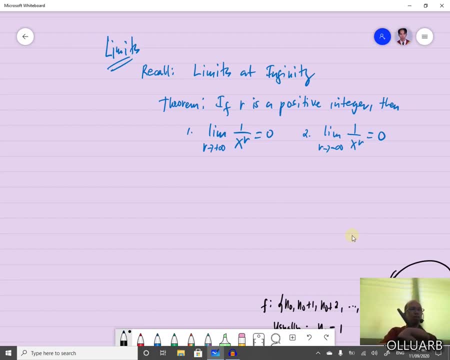 elements of the sequence before up to here. so this is now our sequence, okay and, as you notice here, I'm going to explain again here that we will be focusing all these elements of the sequence before up to here. so this is now our sequence, okay and, as you notice here, I'm going to explain again here that we will be focusing all these. 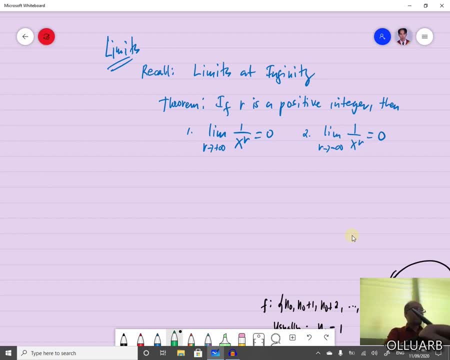 elements of the sequence before up to here. so this is now our sequence, okay and, as you notice here, I'm going to explain again here that we will be focusing all these elements of the sequence before up to here. so this is now our sequence, okay and, as you notice here, I'm going to explain again here that we will be focusing all these. 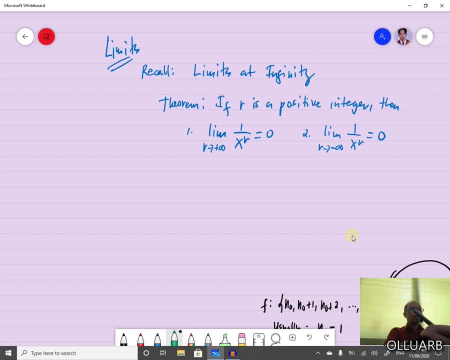 elements of the sequence before up to here. so this is now our sequence, okay and, as you notice here, I'm going to explain again here that we will be focusing all these elements of the sequence before up to here. so this is now our sequence, okay and, as you notice here, I'm going to explain again here that we will be focusing all these. 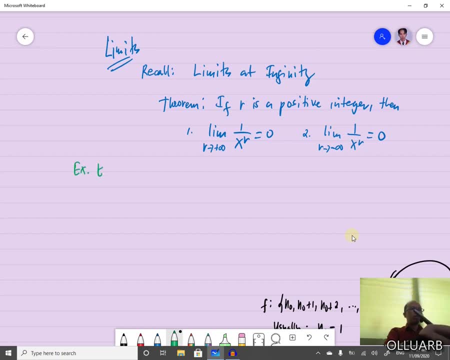 elements of the sequence before up to here. so this is now our sequence, okay and, as you notice here, I'm going to explain again here that we will be focusing all these elements of the sequence before up to here. so this is now our sequence, okay and, as you notice here, I'm going to explain again here that we will be focusing all these. 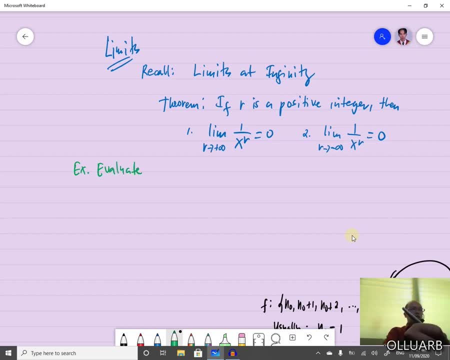 elements of the sequence before up to here. so this is now our sequence, okay and, as you notice here, I'm going to explain again here that we will be focusing all these elements of the sequence before up to here. so this is now our sequence, okay and, as you notice here, I'm going to explain again here that we will be focusing all these. 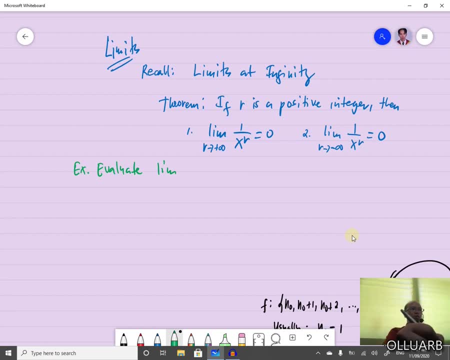 elements of the sequence before up to here. so this is now our sequence, okay and, as you notice here, I'm going to explain again here that we will be focusing all these elements of the sequence before up to here. so this is now our sequence, okay and, as you notice here, I'm going to explain again here that we will be focusing all these. 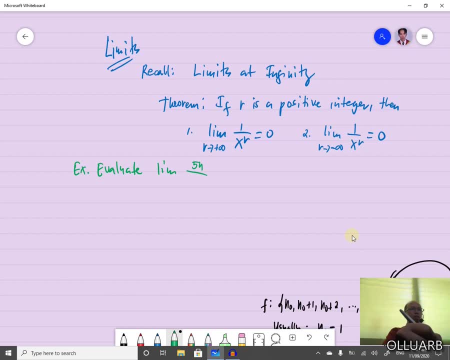 elements of the sequence before up to here. so this is now our sequence, okay and, as you notice here, I'm going to explain again here that we will be focusing all these elements of the sequence before up to here. so this is now our sequence, okay and, as you notice here, I'm going to explain again here that we will be focusing all these. 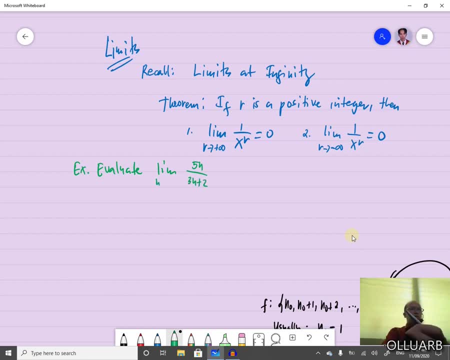 elements of the sequence before up to here. so this is now our sequence, okay and, as you notice here, I'm going to explain again here that we will be focusing all these elements of the sequence before up to here. so this is now our sequence, okay and, as you notice here, I'm going to explain again here that we will be focusing all these. 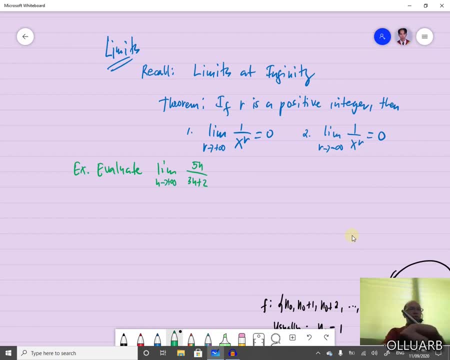 elements of the sequence before up to here. so this is now our sequence, okay and, as you notice here, I'm going to explain again here that we will be focusing all these elements of the sequence before up to here. so this is now our sequence, okay and, as you notice here, I'm going to explain again here that we will be focusing all these. 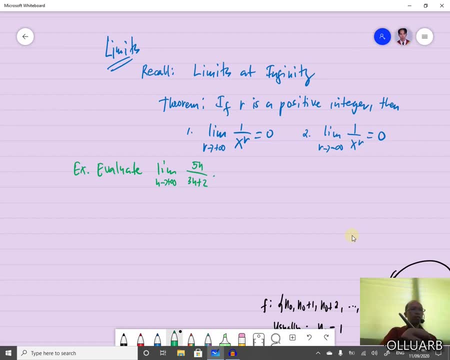 elements of the sequence before up to here. so this is now our sequence, okay and, as you notice here, I'm going to explain again here that we will be focusing all these elements of the sequence before up to here. so this is now our sequence, okay and, as you notice here, I'm going to explain again here that we will be focusing all these. 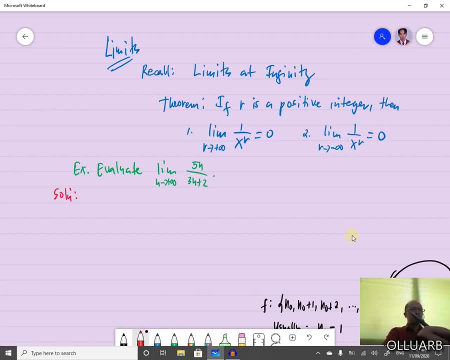 elements of the sequence before up to here. so this is now our sequence, okay and, as you notice here, I'm going to explain again here that we will be focusing all these elements of the sequence before up to here. so this is now our sequence, okay and, as you notice here, I'm going to explain again here that we will be focusing all these. 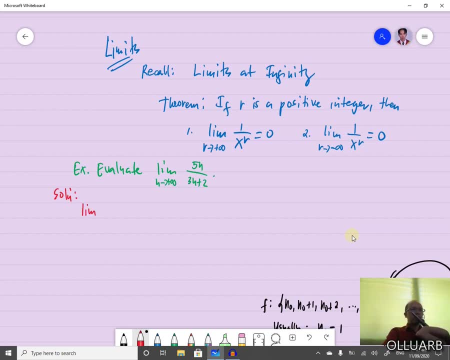 elements of the sequence before up to here. so this is now our sequence, okay and, as you notice here, I'm going to explain again here that we will be focusing all these elements of the sequence before up to here. so this is now our sequence, okay and, as you notice here, I'm going to explain again here that we will be focusing all these. 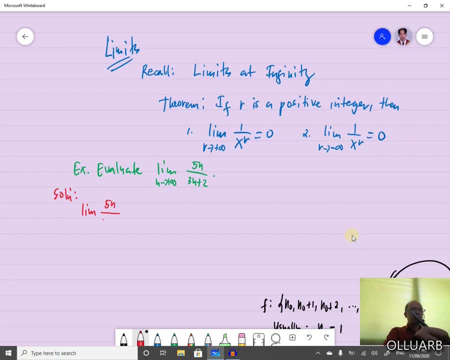 elements of the sequence before up to here. so this is now our sequence, okay and, as you notice here, I'm going to explain again here that we will be focusing all these elements of the sequence before up to here. so this is now our sequence, okay and, as you notice here, I'm going to explain again here that we will be focusing all these. 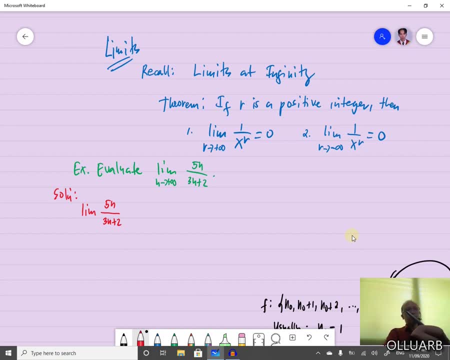 elements of the sequence before up to here. so this is now our sequence, okay and, as you notice here, I'm going to explain again here that we will be focusing all these elements of the sequence before up to here. so this is now our sequence, okay and, as you notice here, I'm going to explain again here that we will be focusing all these. 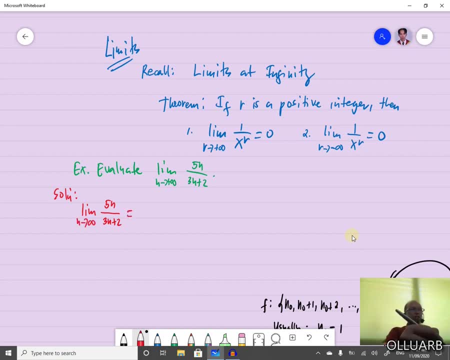 elements of the sequence before up to here. so this is now our sequence, okay and, as you notice here, I'm going to explain again here that we will be focusing all these elements of the sequence before up to here. so this is now our sequence, okay and, as you notice here, I'm going to explain again here that we will be focusing all these. 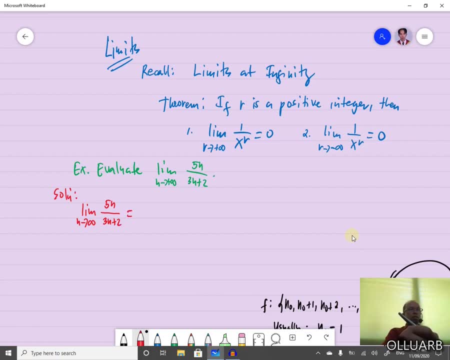 elements of the sequence before up to here. so this is now our sequence, okay and, as you notice here, I'm going to explain again here that we will be focusing all these elements of the sequence before up to here. so this is now our sequence, okay and, as you notice here, I'm going to explain again here that we will be focusing all these. 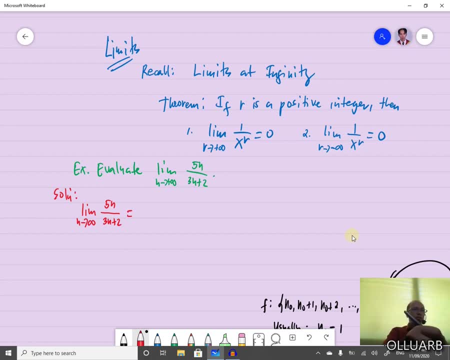 elements of the sequence before up to here. so this is now our sequence, okay and, as you notice here, I'm going to explain again here that we will be focusing all these elements of the sequence before up to here. so this is now our sequence, okay and, as you notice here, I'm going to explain again here that we will be focusing all these. 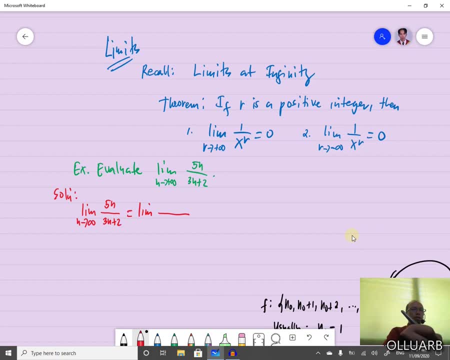 elements of the sequence before up to here. so this is now our sequence, okay and, as you notice here, I'm going to explain again here that we will be focusing all these elements of the sequence before up to here. so this is now our sequence, okay and, as you notice here, I'm going to explain again here that we will be focusing all these. 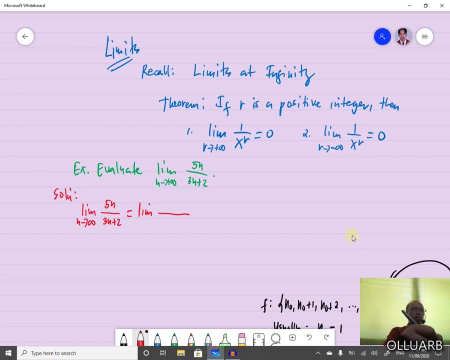 elements of the sequence before up to here. so this is now our sequence, okay and, as you notice here, I'm going to explain again here that we will be focusing all these elements of the sequence before up to here. so this is now our sequence, okay and, as you notice here, I'm going to explain again here that we will be focusing all these. 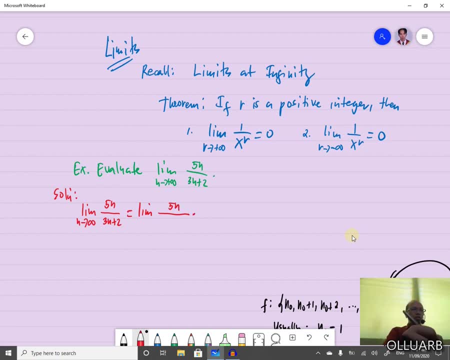 elements of the sequence before up to here. so this is now our sequence, okay and, as you notice here, I'm going to explain again here that we will be focusing all these elements of the sequence before up to here. so this is now our sequence, okay and, as you notice here, I'm going to explain again here that we will be focusing all these. 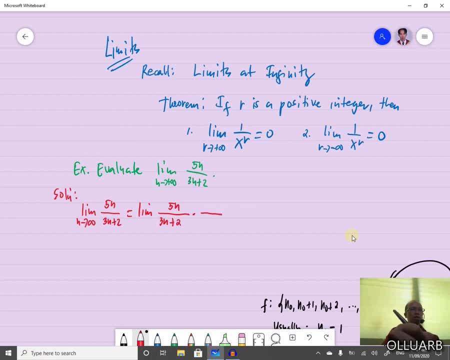 elements of the sequence before up to here. so this is now our sequence, okay and, as you notice here, I'm going to explain again here that we will be focusing all these elements of the sequence before up to here. so this is now our sequence, okay and, as you notice here, I'm going to explain again here that we will be focusing all these. 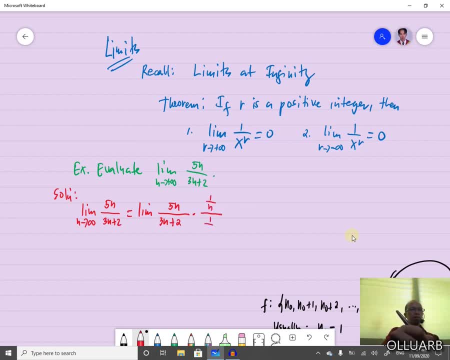 elements of the sequence before up to here. so this is now our sequence, okay and, as you notice here, I'm going to explain again here that we will be focusing all these elements of the sequence before up to here. so this is now our sequence, okay and, as you notice here, I'm going to explain again here that we will be focusing all these. 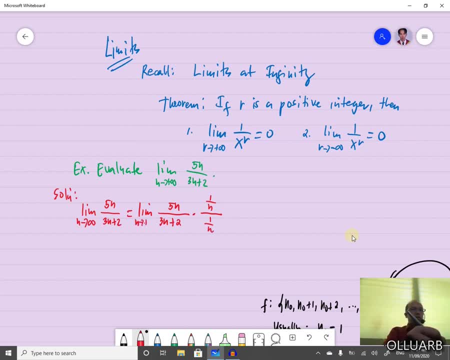 elements of the sequence before up to here. so this is now our sequence, okay and, as you notice here, I'm going to explain again here that we will be focusing all these elements of the sequence before up to here. so this is now our sequence, okay and, as you notice here, I'm going to explain again here that we will be focusing all these. 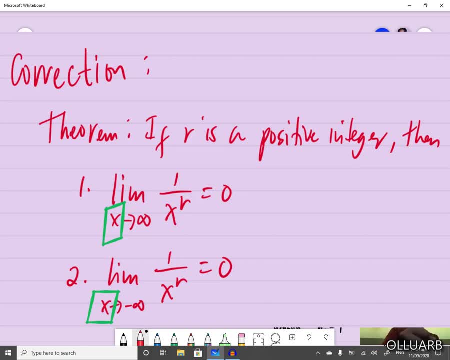 elements of the sequence before up to here. so this is now our sequence, okay and, as you notice here, I'm going to explain again here that we will be focusing all these elements of the sequence before up to here. so this is now our sequence, okay and, as you notice here, I'm going to explain again here that we will be focusing all these. 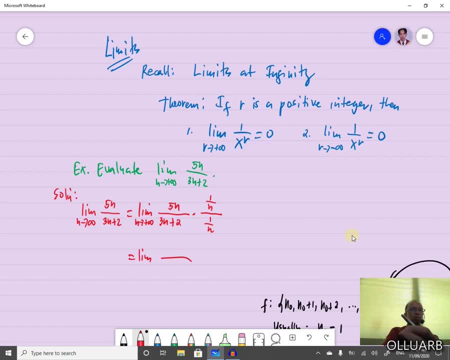 elements of the sequence before up to here. so this is now our sequence, okay and, as you notice here, I'm going to explain again here that we will be focusing all these elements of the sequence before up to here. so this is now our sequence, okay and, as you notice here, I'm going to explain again here that we will be focusing all these. 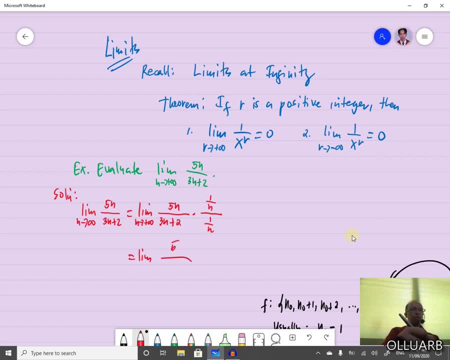 elements of the sequence before up to here. so this is now our sequence, okay and, as you notice here, I'm going to explain again here that we will be focusing all these elements of the sequence before up to here. so this is now our sequence, okay and, as you notice here, I'm going to explain again here that we will be focusing all these. 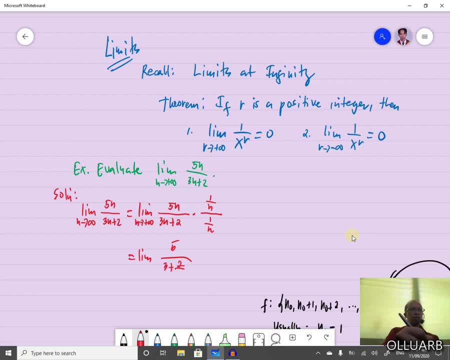 elements of the sequence before up to here. so this is now our sequence, okay and, as you notice here, I'm going to explain again here that we will be focusing all these elements of the sequence before up to here. so this is now our sequence, okay and, as you notice here, I'm going to explain again here that we will be focusing all these. 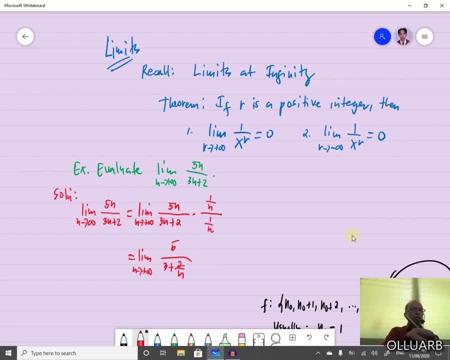 elements of the sequence before up to here. so this is now our sequence, okay and, as you notice here, I'm going to explain again here that we will be focusing all these elements of the sequence before up to here. so this is now our sequence, okay and, as you notice here, I'm going to explain again here that we will be focusing all these. 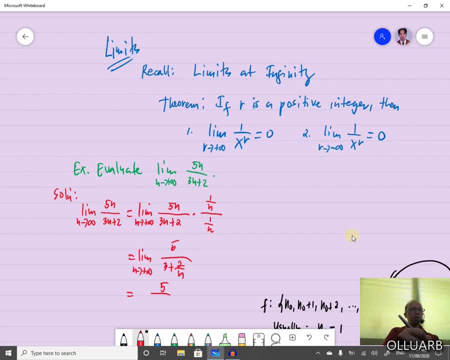 elements of the sequence before up to here. so this is now our sequence, okay and, as you notice here, I'm going to explain again here that we will be focusing all these elements of the sequence before up to here. so this is now our sequence, okay and, as you notice here, I'm going to explain again here that we will be focusing all these. 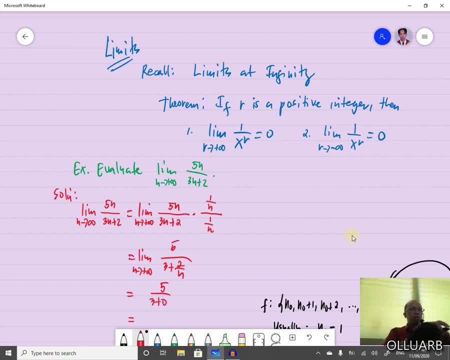 elements of the sequence before up to here. so this is now our sequence, okay and, as you notice here, I'm going to explain again here that we will be focusing all these elements of the sequence before up to here. so this is now our sequence, okay and, as you notice here, I'm going to explain again here that we will be focusing all these. 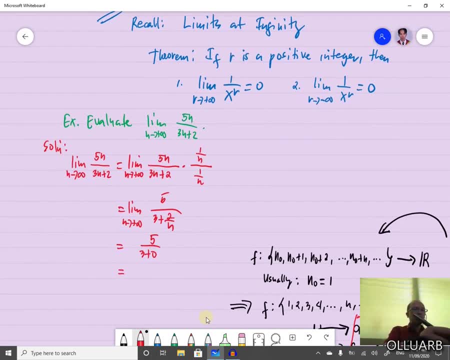 elements of the sequence before up to here. so this is now our sequence, okay and, as you notice here, I'm going to explain again here that we will be focusing all these elements of the sequence before up to here. so this is now our sequence, okay and, as you notice here, I'm going to explain again here that we will be focusing all these. 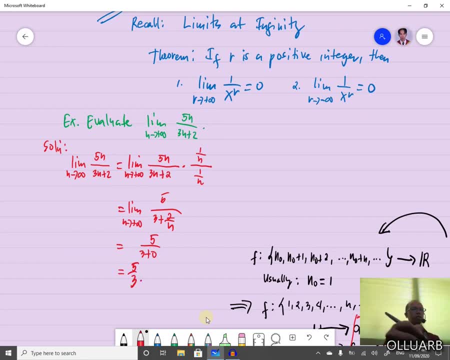 elements of the sequence before up to here. so this is now our sequence, okay and, as you notice here, I'm going to explain again here that we will be focusing all these elements of the sequence before up to here. so this is now our sequence, okay and, as you notice here, I'm going to explain again here that we will be focusing all these. 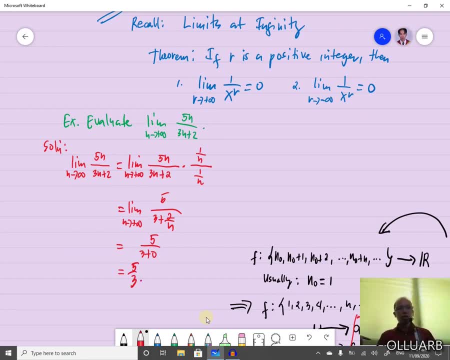 elements of the sequence before up to here. so this is now our sequence, okay and, as you notice here, I'm going to explain again here that we will be focusing all these elements of the sequence before up to here. so this is now our sequence, okay and, as you notice here, I'm going to explain again here that we will be focusing all these. 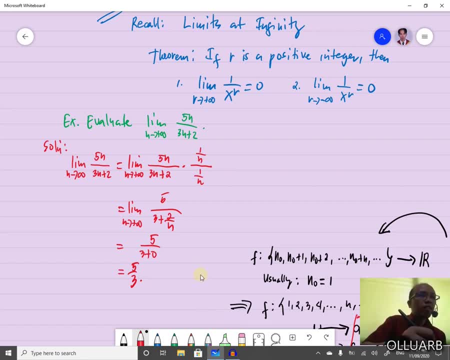 elements of the sequence before up to here. so this is now our sequence, okay and, as you notice here, I'm going to explain again here that we will be focusing all these elements of the sequence before up to here. so this is now our sequence, okay and, as you notice here, I'm going to explain again here that we will be focusing all these. 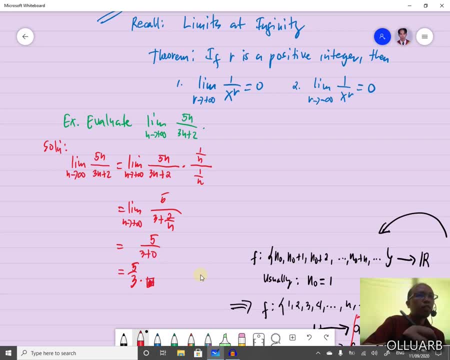 elements of the sequence before up to here. so this is now our sequence, okay and, as you notice here, I'm going to explain again here that we will be focusing all these elements of the sequence before up to here. so this is now our sequence, okay and, as you notice here, I'm going to explain again here that we will be focusing all these. 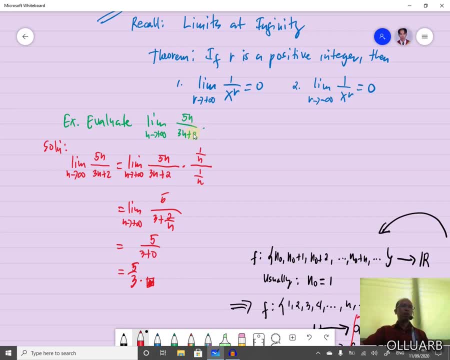 elements of the sequence before up to here. so this is now our sequence, okay and, as you notice here, I'm going to explain again here that we will be focusing all these elements of the sequence before up to here. so this is now our sequence, okay and, as you notice here, I'm going to explain again here that we will be focusing all these. 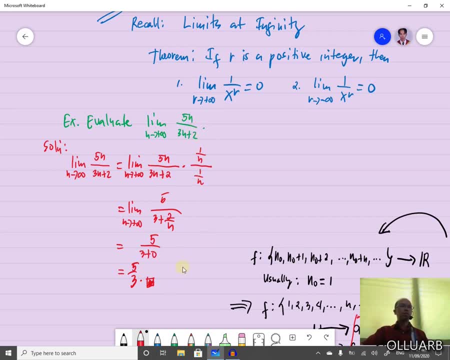 elements of the sequence before up to here. so this is now our sequence, okay and, as you notice here, I'm going to explain again here that we will be focusing all these elements of the sequence before up to here. so this is now our sequence, okay and, as you notice here, I'm going to explain again here that we will be focusing all these. 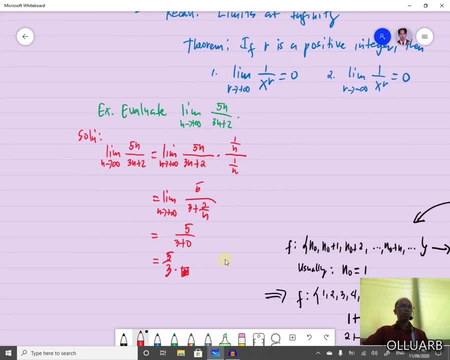 elements of the sequence before up to here. so this is now our sequence, okay and, as you notice here, I'm going to explain again here that we will be focusing all these elements of the sequence before up to here. so this is now our sequence, okay and, as you notice here, I'm going to explain again here that we will be focusing all these. 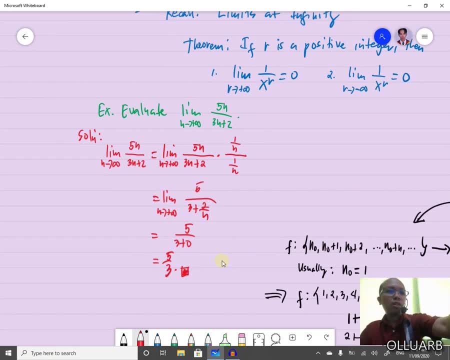 elements of the sequence before up to here. so this is now our sequence, okay and, as you notice here, I'm going to explain again here that we will be focusing all these elements of the sequence before up to here. so this is now our sequence, okay and, as you notice here, I'm going to explain again here that we will be focusing all these. 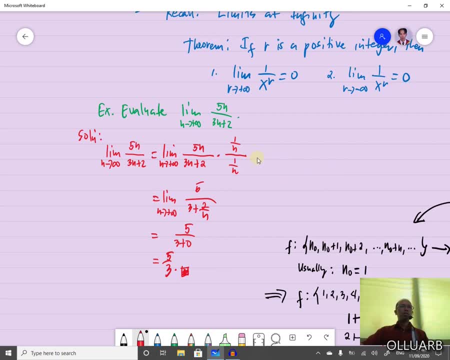 elements of the sequence before up to here. so this is now our sequence, okay and, as you notice here, I'm going to explain again here that we will be focusing all these elements of the sequence before up to here. so this is now our sequence, okay and, as you notice here, I'm going to explain again here that we will be focusing all these. 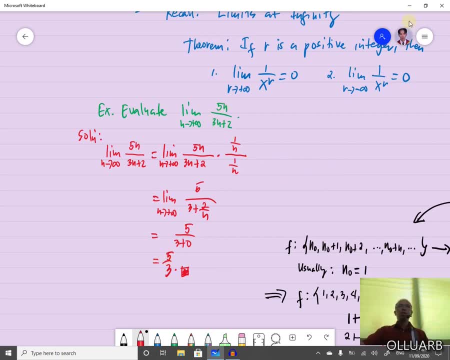 elements of the sequence before up to here. so this is now our sequence, okay and, as you notice here, I'm going to explain again here that we will be focusing all these elements of the sequence before up to here. so this is now our sequence, okay and, as you notice here, I'm going to explain again here that we will be focusing all these. 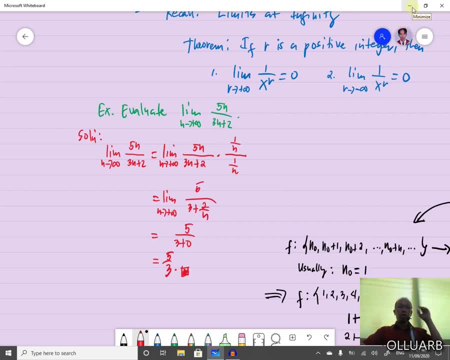 elements of the sequence before up to here. so this is now our sequence, okay and, as you notice here, I'm going to explain again here that we will be focusing all these elements of the sequence before up to here. so this is now our sequence, okay and, as you notice here, I'm going to explain again here that we will be focusing all these. 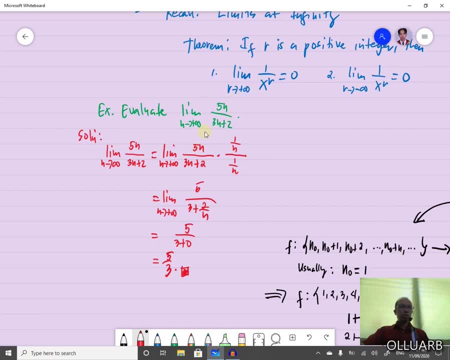 elements of the sequence before up to here. so this is now our sequence, okay and, as you notice here, I'm going to explain again here that we will be focusing all these elements of the sequence before up to here. so this is now our sequence, okay and, as you notice here, I'm going to explain again here that we will be focusing all these. 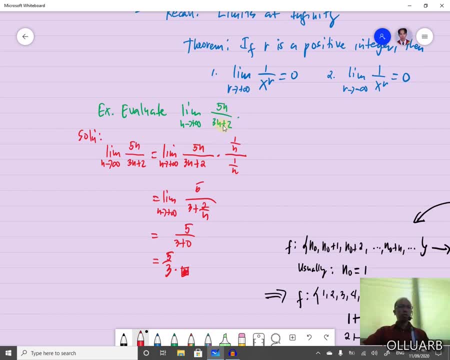 elements of the sequence before up to here. so this is now our sequence, okay and, as you notice here, I'm going to explain again here that we will be focusing all these elements of the sequence before up to here. so this is now our sequence, okay and, as you notice here, I'm going to explain again here that we will be focusing all these. 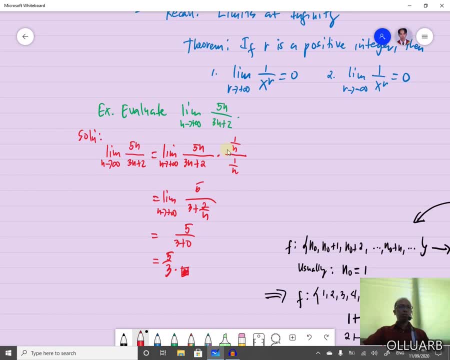 elements of the sequence before up to here. so this is now our sequence, okay and, as you notice here, I'm going to explain again here that we will be focusing all these elements of the sequence before up to here. so this is now our sequence, okay and, as you notice here, I'm going to explain again here that we will be focusing all these. 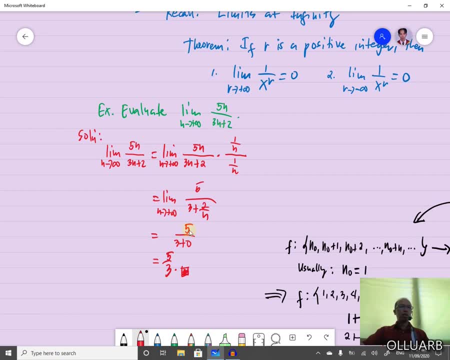 elements of the sequence before up to here. so this is now our sequence, okay and, as you notice here, I'm going to explain again here that we will be focusing all these elements of the sequence before up to here. so this is now our sequence, okay and, as you notice here, I'm going to explain again here that we will be focusing all these. 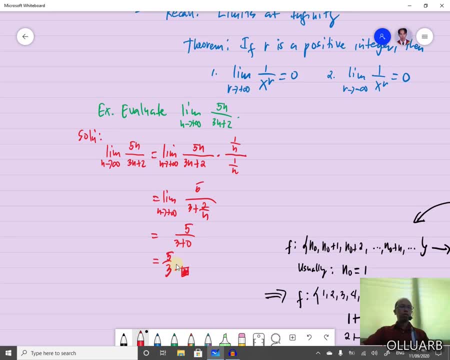 elements of the sequence before up to here. so this is now our sequence, okay and, as you notice here, I'm going to explain again here that we will be focusing all these elements of the sequence before up to here. so this is now our sequence, okay and, as you notice here, I'm going to explain again here that we will be focusing all these. 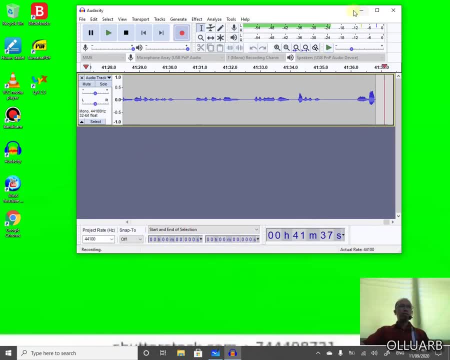 elements of the sequence before up to here. so this is now our sequence, okay and, as you notice here, I'm going to explain again here that we will be focusing all these elements of the sequence before up to here. so this is now our sequence, okay and, as you notice here, I'm going to explain again here that we will be focusing all these. 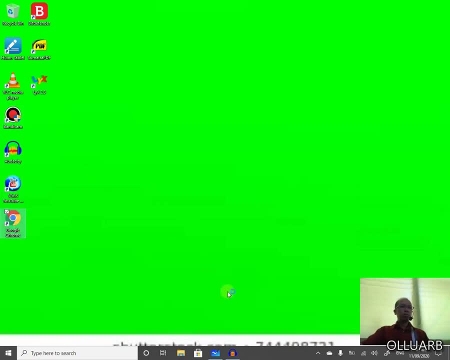 elements of the sequence before up to here. so this is now our sequence, okay and, as you notice here, I'm going to explain again here that we will be focusing all these elements of the sequence before up to here. so this is now our sequence, okay and, as you notice here, I'm going to explain again here that we will be focusing all these. 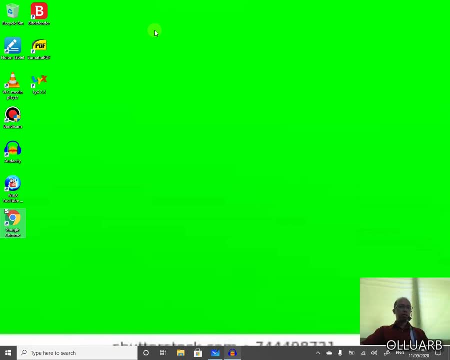 elements of the sequence before up to here. so this is now our sequence, okay and, as you notice here, I'm going to explain again here that we will be focusing all these elements of the sequence before up to here. so this is now our sequence, okay and, as you notice here, I'm going to explain again here that we will be focusing all these. 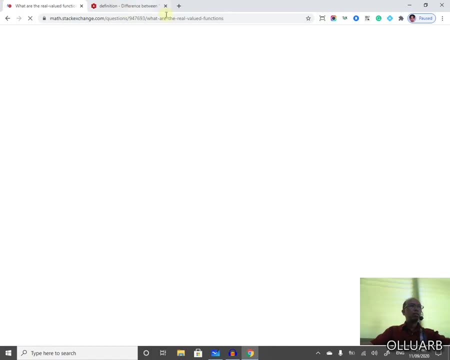 elements of the sequence before up to here. so this is now our sequence, okay and, as you notice here, I'm going to explain again here that we will be focusing all these elements of the sequence before up to here. so this is now our sequence, okay and, as you notice here, I'm going to explain again here that we will be focusing all these. 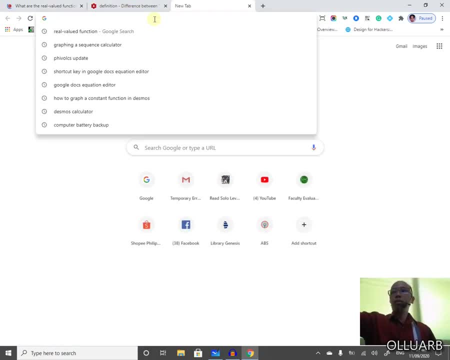 elements of the sequence before up to here. so this is now our sequence, okay and, as you notice here, I'm going to explain again here that we will be focusing all these elements of the sequence before up to here. so this is now our sequence, okay and, as you notice here, I'm going to explain again here that we will be focusing all these. 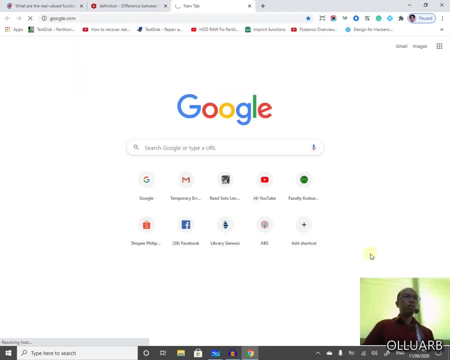 elements of the sequence before up to here. so this is now our sequence, okay and, as you notice here, I'm going to explain again here that we will be focusing all these elements of the sequence before up to here. so this is now our sequence, okay and, as you notice here, I'm going to explain again here that we will be focusing all these. 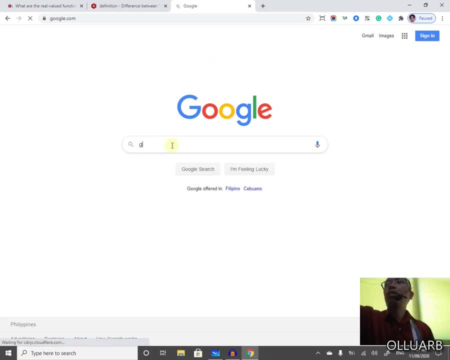 elements of the sequence before up to here. so this is now our sequence, okay and, as you notice here, I'm going to explain again here that we will be focusing all these elements of the sequence before up to here. so this is now our sequence, okay and, as you notice here, I'm going to explain again here that we will be focusing all these. 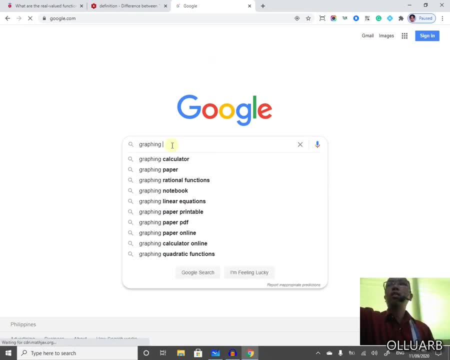 elements of the sequence before up to here. so this is now our sequence, okay and, as you notice here, I'm going to explain again here that we will be focusing all these elements of the sequence before up to here. so this is now our sequence, okay and, as you notice here, I'm going to explain again here that we will be focusing all these. 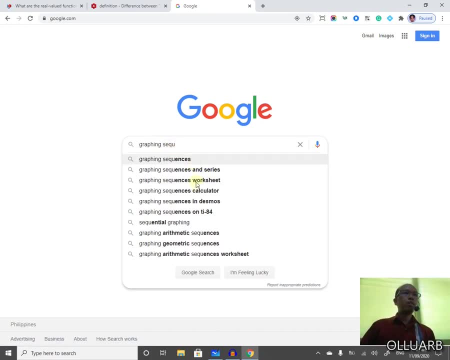 elements of the sequence before up to here. so this is now our sequence, okay and, as you notice here, I'm going to explain again here that we will be focusing all these elements of the sequence before up to here. so this is now our sequence, okay and, as you notice here, I'm going to explain again here that we will be focusing all these. 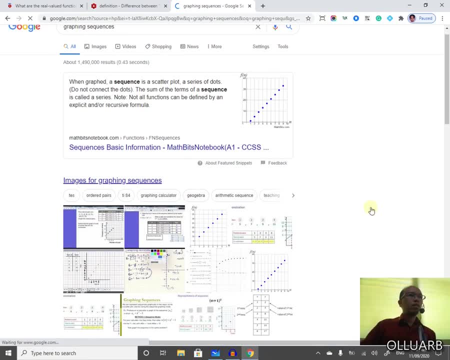 elements of the sequence before up to here. so this is now our sequence, okay and, as you notice here, I'm going to explain again here that we will be focusing all these elements of the sequence before up to here. so this is now our sequence, okay and, as you notice here, I'm going to explain again here that we will be focusing all these. 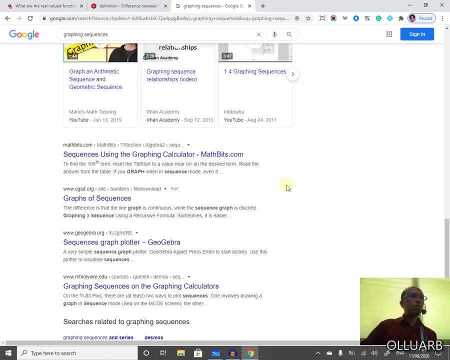 elements of the sequence before up to here. so this is now our sequence, okay and, as you notice here, I'm going to explain again here that we will be focusing all these elements of the sequence before up to here. so this is now our sequence, okay and, as you notice here, I'm going to explain again here that we will be focusing all these. 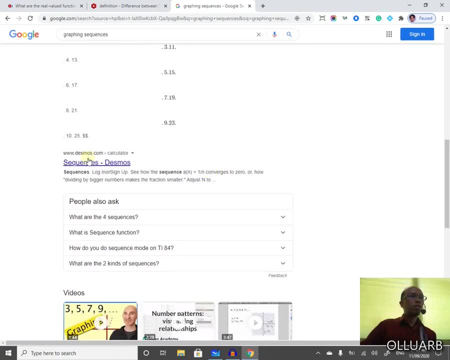 elements of the sequence before up to here. so this is now our sequence, okay and, as you notice here, I'm going to explain again here that we will be focusing all these elements of the sequence before up to here. so this is now our sequence, okay and, as you notice here, I'm going to explain again here that we will be focusing all these. 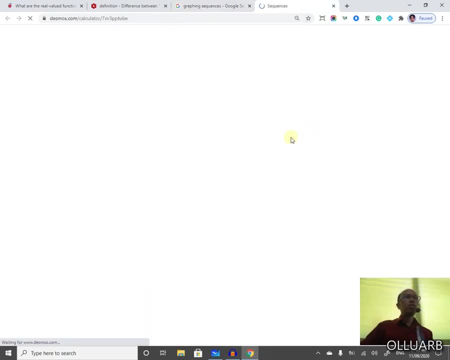 elements of the sequence before up to here. so this is now our sequence, okay and, as you notice here, I'm going to explain again here that we will be focusing all these elements of the sequence before up to here. so this is now our sequence, okay and, as you notice here, I'm going to explain again here that we will be focusing all these. 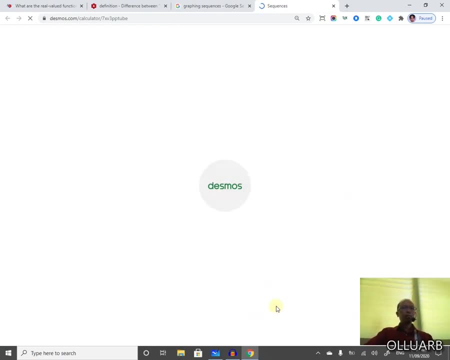 elements of the sequence before up to here. so this is now our sequence, okay and, as you notice here, I'm going to explain again here that we will be focusing all these elements of the sequence before up to here. so this is now our sequence, okay and, as you notice here, I'm going to explain again here that we will be focusing all these. 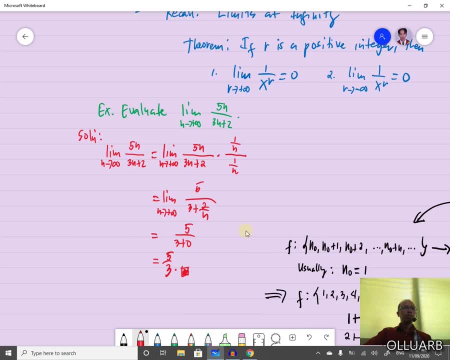 elements of the sequence before up to here. so this is now our sequence, okay and, as you notice here, I'm going to explain again here that we will be focusing all these elements of the sequence before up to here. so this is now our sequence, okay and, as you notice here, I'm going to explain again here that we will be focusing all these. 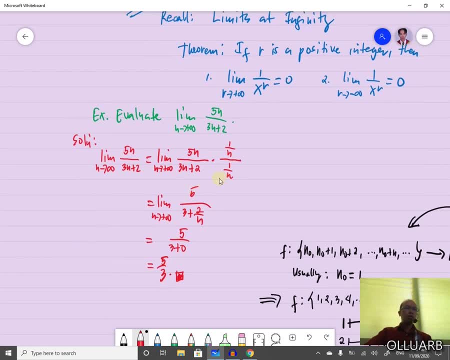 elements of the sequence before up to here. so this is now our sequence, okay and, as you notice here, I'm going to explain again here that we will be focusing all these elements of the sequence before up to here. so this is now our sequence, okay and, as you notice here, I'm going to explain again here that we will be focusing all these. 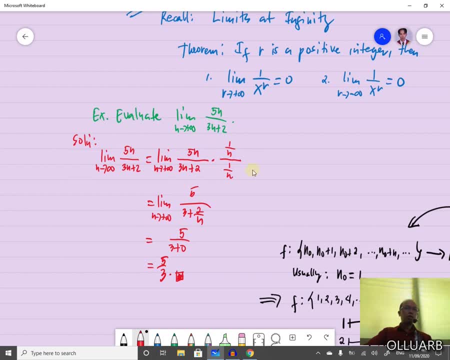 elements of the sequence before up to here. so this is now our sequence, okay and, as you notice here, I'm going to explain again here that we will be focusing all these elements of the sequence before up to here. so this is now our sequence, okay and, as you notice here, I'm going to explain again here that we will be focusing all these. 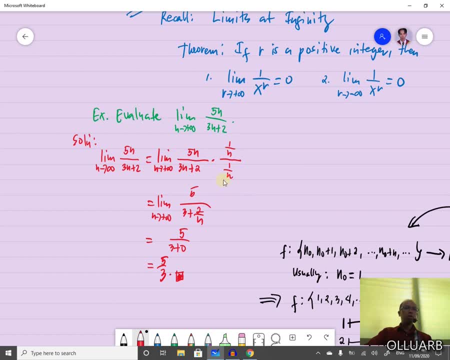 elements of the sequence before up to here. so this is now our sequence, okay and, as you notice here, I'm going to explain again here that we will be focusing all these elements of the sequence before up to here. so this is now our sequence, okay and, as you notice here, I'm going to explain again here that we will be focusing all these. 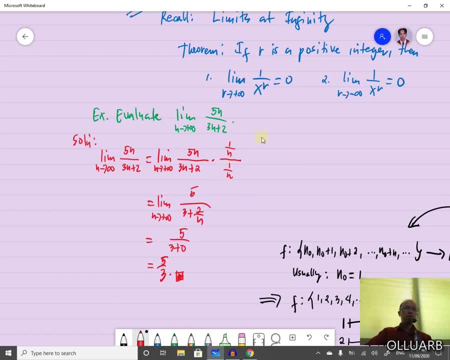 elements of the sequence before up to here. so this is now our sequence, okay and, as you notice here, I'm going to explain again here that we will be focusing all these elements of the sequence before up to here. so this is now our sequence, okay and, as you notice here, I'm going to explain again here that we will be focusing all these. 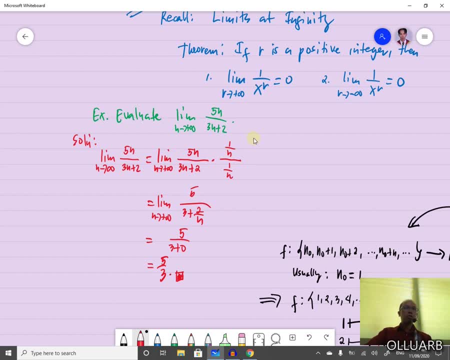 elements of the sequence before up to here. so this is now our sequence, okay and, as you notice here, I'm going to explain again here that we will be focusing all these elements of the sequence before up to here. so this is now our sequence, okay and, as you notice here, I'm going to explain again here that we will be focusing all these. 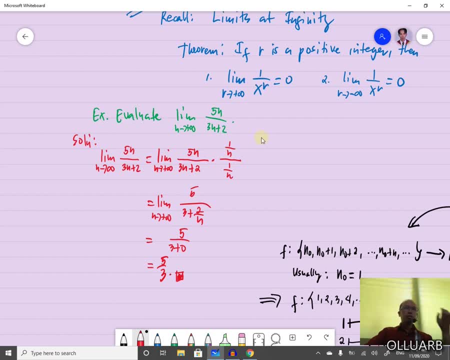 elements of the sequence before up to here. so this is now our sequence, okay and, as you notice here, I'm going to explain again here that we will be focusing all these elements of the sequence before up to here. so this is now our sequence, okay and, as you notice here, I'm going to explain again here that we will be focusing all these. 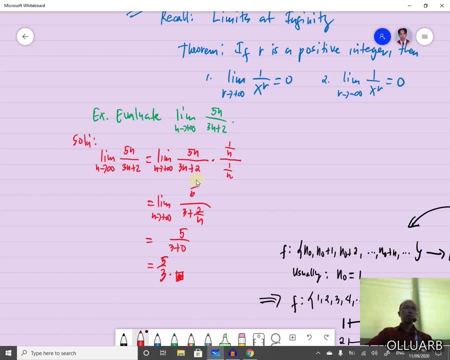 elements of the sequence before up to here. so this is now our sequence, okay and, as you notice here, I'm going to explain again here that we will be focusing all these elements of the sequence before up to here. so this is now our sequence, okay and, as you notice here, I'm going to explain again here that we will be focusing all these. 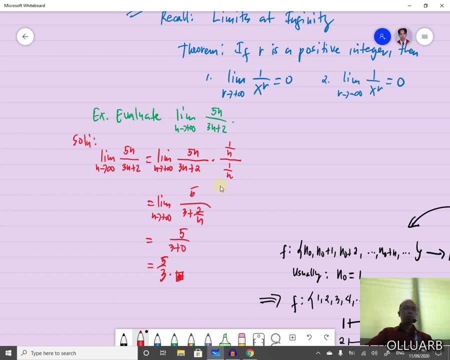 elements of the sequence before up to here. so this is now our sequence, okay and, as you notice here, I'm going to explain again here that we will be focusing all these elements of the sequence before up to here. so this is now our sequence, okay and, as you notice here, I'm going to explain again here that we will be focusing all these. 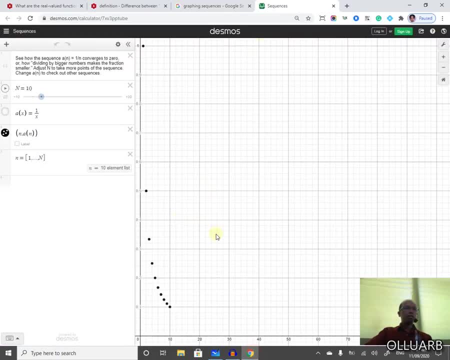 elements of the sequence before up to here. so this is now our sequence, okay and, as you notice here, I'm going to explain again here that we will be focusing all these elements of the sequence before up to here. so this is now our sequence, okay and, as you notice here, I'm going to explain again here that we will be focusing all these. 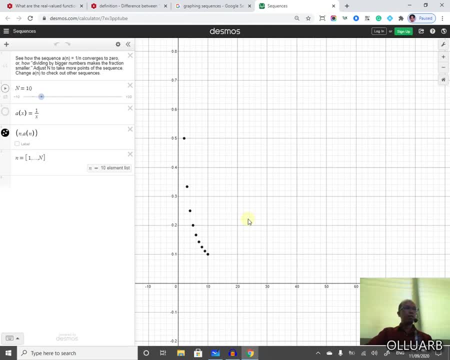 elements of the sequence before up to here. so this is now our sequence, okay and, as you notice here, I'm going to explain again here that we will be focusing all these elements of the sequence before up to here. so this is now our sequence, okay and, as you notice here, I'm going to explain again here that we will be focusing all these. 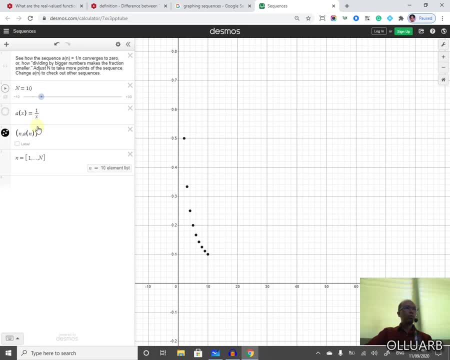 elements of the sequence before up to here. so this is now our sequence, okay and, as you notice here, I'm going to explain again here that we will be focusing all these elements of the sequence before up to here. so this is now our sequence, okay and, as you notice here, I'm going to explain again here that we will be focusing all these. 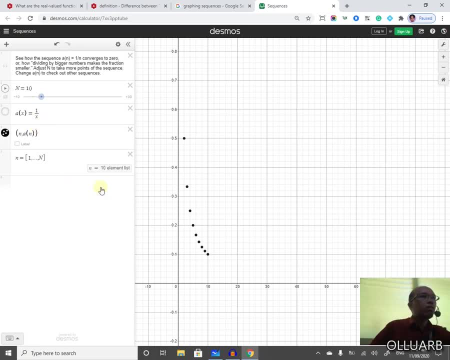 elements of the sequence before up to here. so this is now our sequence, okay and, as you notice here, I'm going to explain again here that we will be focusing all these elements of the sequence before up to here. so this is now our sequence, okay and, as you notice here, I'm going to explain again here that we will be focusing all these. 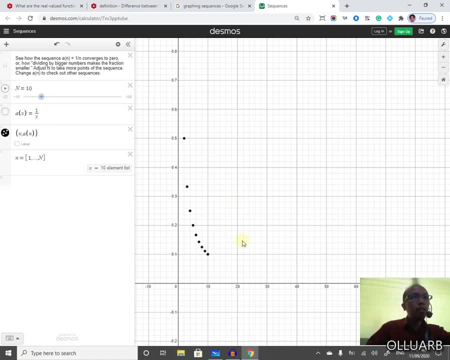 elements of the sequence before up to here. so this is now our sequence, okay and, as you notice here, I'm going to explain again here that we will be focusing all these elements of the sequence before up to here. so this is now our sequence, okay and, as you notice here, I'm going to explain again here that we will be focusing all these. 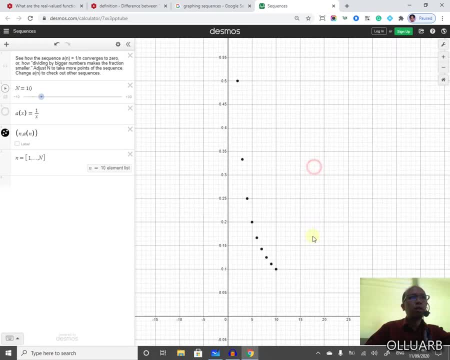 elements of the sequence before up to here. so this is now our sequence, okay and, as you notice here, I'm going to explain again here that we will be focusing all these elements of the sequence before up to here. so this is now our sequence, okay and, as you notice here, I'm going to explain again here that we will be focusing all these. 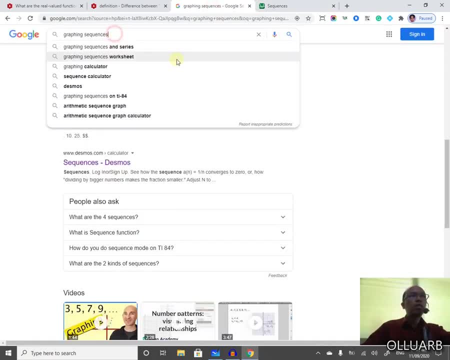 elements of the sequence before up to here. so this is now our sequence, okay and, as you notice here, I'm going to explain again here that we will be focusing all these elements of the sequence before up to here. so this is now our sequence, okay and, as you notice here, I'm going to explain again here that we will be focusing all these. 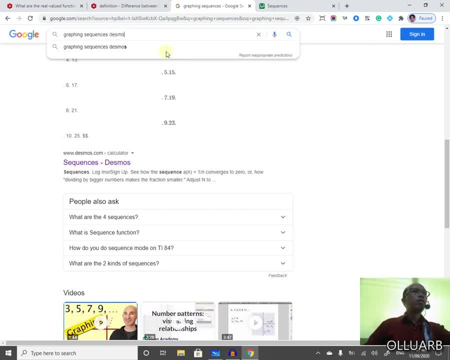 elements of the sequence before up to here. so this is now our sequence, okay and, as you notice here, I'm going to explain again here that we will be focusing all these elements of the sequence before up to here. so this is now our sequence, okay and, as you notice here, I'm going to explain again here that we will be focusing all these. 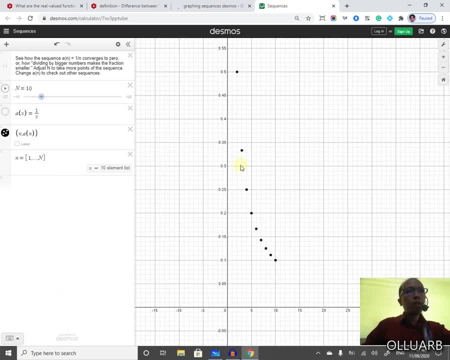 elements of the sequence before up to here. so this is now our sequence, okay and, as you notice here, I'm going to explain again here that we will be focusing all these elements of the sequence before up to here. so this is now our sequence, okay and, as you notice here, I'm going to explain again here that we will be focusing all these. 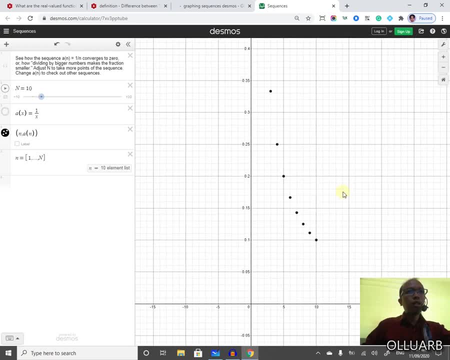 elements of the sequence before up to here. so this is now our sequence, okay and, as you notice here, I'm going to explain again here that we will be focusing all these elements of the sequence before up to here. so this is now our sequence, okay and, as you notice here, I'm going to explain again here that we will be focusing all these. 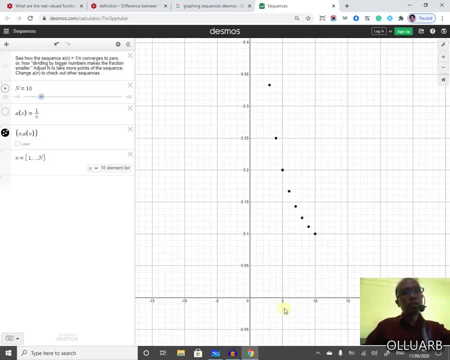 elements of the sequence before up to here. so this is now our sequence, okay and, as you notice here, I'm going to explain again here that we will be focusing all these elements of the sequence before up to here. so this is now our sequence, okay and, as you notice here, I'm going to explain again here that we will be focusing all these. 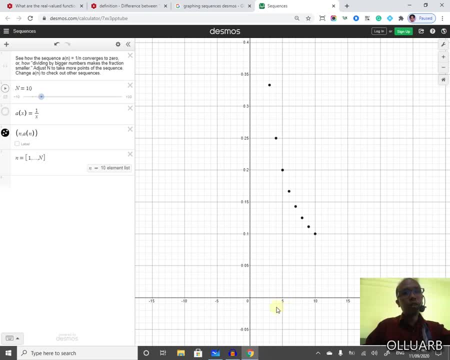 elements of the sequence before up to here. so this is now our sequence, okay and, as you notice here, I'm going to explain again here that we will be focusing all these elements of the sequence before up to here. so this is now our sequence, okay and, as you notice here, I'm going to explain again here that we will be focusing all these. 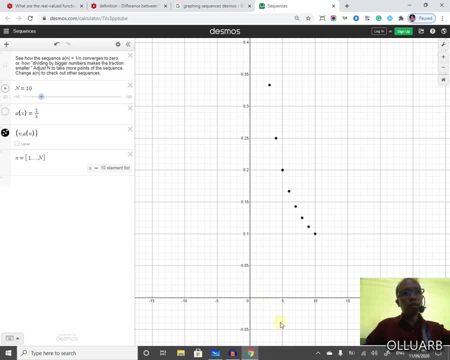 elements of the sequence before up to here. so this is now our sequence, okay and, as you notice here, I'm going to explain again here that we will be focusing all these elements of the sequence before up to here. so this is now our sequence, okay and, as you notice here, I'm going to explain again here that we will be focusing all these. 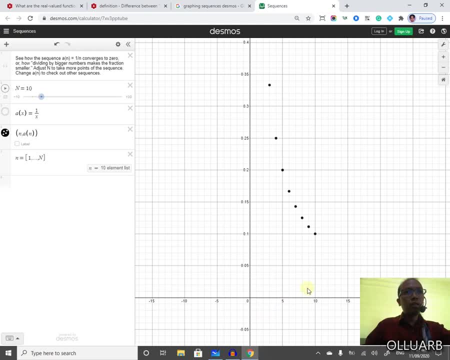 elements of the sequence before up to here. so this is now our sequence, okay and, as you notice here, I'm going to explain again here that we will be focusing all these elements of the sequence before up to here. so this is now our sequence, okay and, as you notice here, I'm going to explain again here that we will be focusing all these. 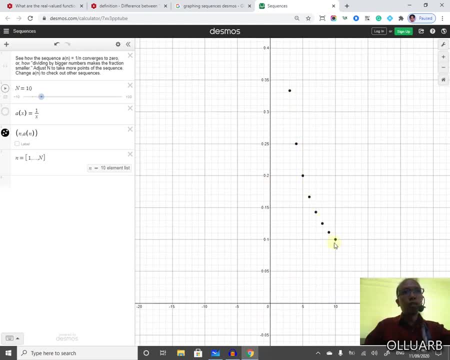 elements of the sequence before up to here. so this is now our sequence, okay and, as you notice here, I'm going to explain again here that we will be focusing all these elements of the sequence before up to here. so this is now our sequence, okay and, as you notice here, I'm going to explain again here that we will be focusing all these. 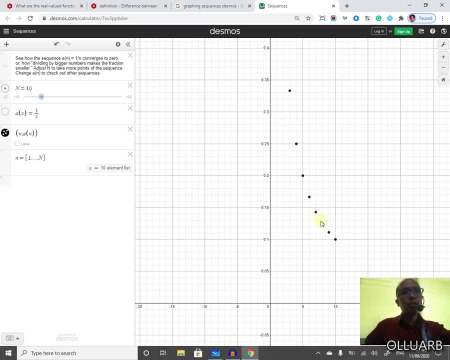 elements of the sequence before up to here. so this is now our sequence, okay and, as you notice here, I'm going to explain again here that we will be focusing all these elements of the sequence before up to here. so this is now our sequence, okay and, as you notice here, I'm going to explain again here that we will be focusing all these. 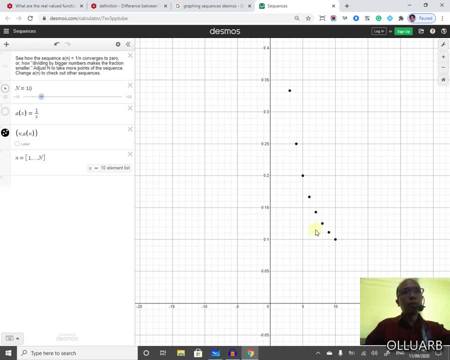 elements of the sequence before up to here. so this is now our sequence, okay and, as you notice here, I'm going to explain again here that we will be focusing all these elements of the sequence before up to here. so this is now our sequence, okay and, as you notice here, I'm going to explain again here that we will be focusing all these. 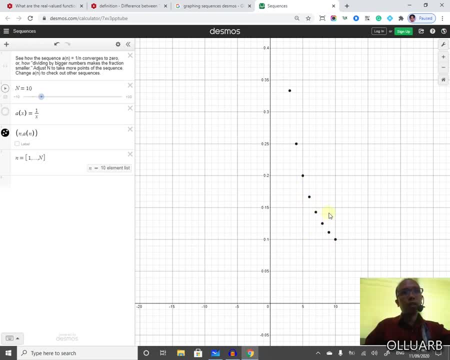 elements of the sequence before up to here. so this is now our sequence, okay and, as you notice here, I'm going to explain again here that we will be focusing all these elements of the sequence before up to here. so this is now our sequence, okay and, as you notice here, I'm going to explain again here that we will be focusing all these. 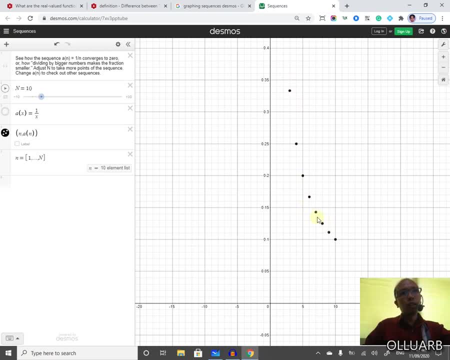 elements of the sequence before up to here. so this is now our sequence, okay and, as you notice here, I'm going to explain again here that we will be focusing all these elements of the sequence before up to here. so this is now our sequence, okay and, as you notice here, I'm going to explain again here that we will be focusing all these. 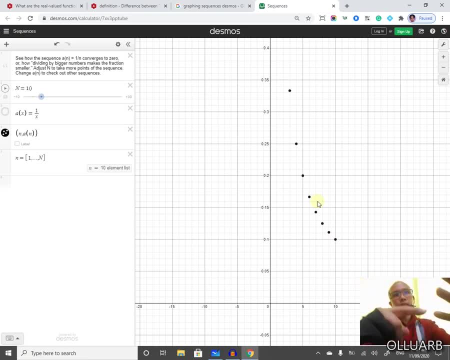 elements of the sequence before up to here. so this is now our sequence, okay and, as you notice here, I'm going to explain again here that we will be focusing all these elements of the sequence before up to here. so this is now our sequence, okay and, as you notice here, I'm going to explain again here that we will be focusing all these. 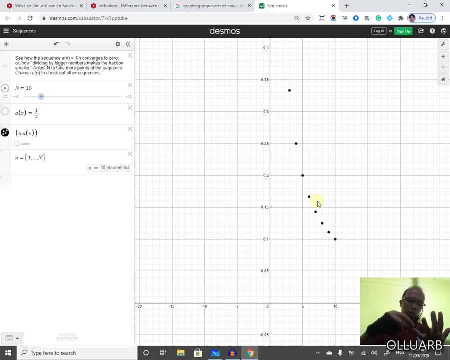 elements of the sequence before up to here. so this is now our sequence, okay and, as you notice here, I'm going to explain again here that we will be focusing all these elements of the sequence before up to here. so this is now our sequence, okay and, as you notice here, I'm going to explain again here that we will be focusing all these. 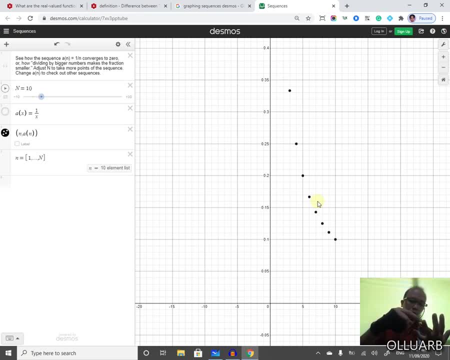 elements of the sequence before up to here. so this is now our sequence, okay and, as you notice here, I'm going to explain again here that we will be focusing all these elements of the sequence before up to here. so this is now our sequence, okay and, as you notice here, I'm going to explain again here that we will be focusing all these. 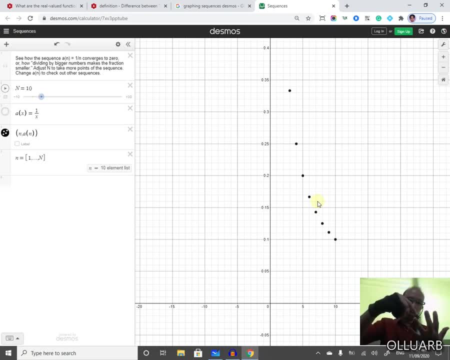 elements of the sequence before up to here. so this is now our sequence, okay and, as you notice here, I'm going to explain again here that we will be focusing all these elements of the sequence before up to here. so this is now our sequence, okay and, as you notice here, I'm going to explain again here that we will be focusing all these. 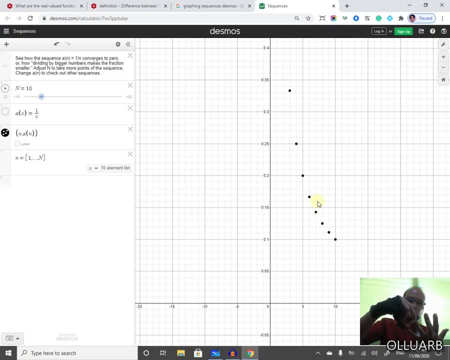 elements of the sequence before up to here. so this is now our sequence, okay and, as you notice here, I'm going to explain again here that we will be focusing all these elements of the sequence before up to here. so this is now our sequence, okay and, as you notice here, I'm going to explain again here that we will be focusing all these. 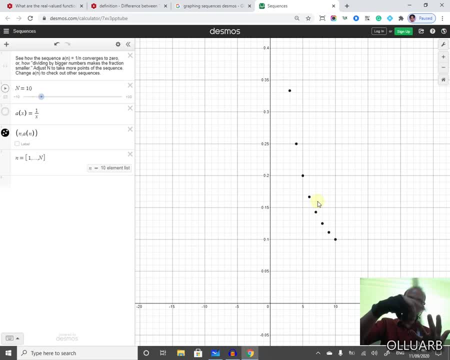 elements of the sequence before up to here. so this is now our sequence, okay and, as you notice here, I'm going to explain again here that we will be focusing all these elements of the sequence before up to here. so this is now our sequence, okay and, as you notice here, I'm going to explain again here that we will be focusing all these. 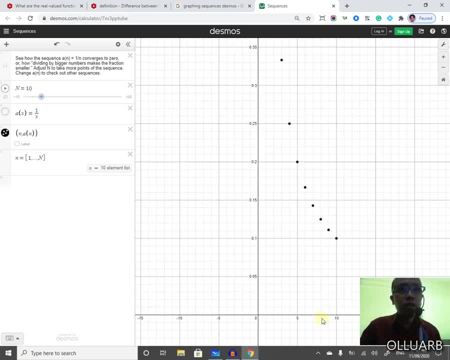 elements of the sequence before up to here. so this is now our sequence, okay and, as you notice here, I'm going to explain again here that we will be focusing all these elements of the sequence before up to here. so this is now our sequence, okay and, as you notice here, I'm going to explain again here that we will be focusing all these. 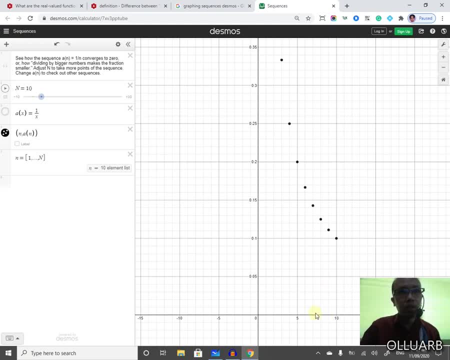 elements of the sequence before up to here. so this is now our sequence, okay and, as you notice here, I'm going to explain again here that we will be focusing all these elements of the sequence before up to here. so this is now our sequence, okay and, as you notice here, I'm going to explain again here that we will be focusing all these. 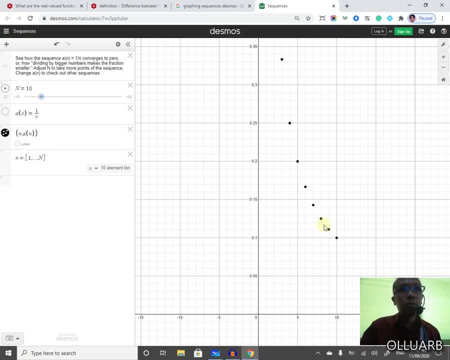 elements of the sequence before up to here. so this is now our sequence, okay and, as you notice here, I'm going to explain again here that we will be focusing all these elements of the sequence before up to here. so this is now our sequence, okay and, as you notice here, I'm going to explain again here that we will be focusing all these. 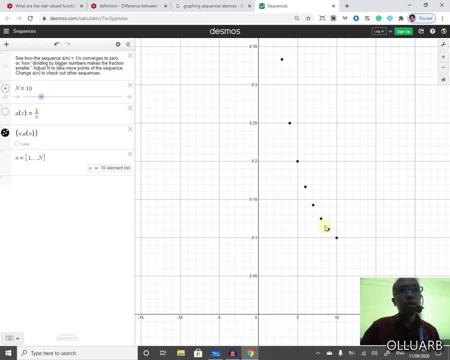 elements of the sequence before up to here. so this is now our sequence, okay and, as you notice here, I'm going to explain again here that we will be focusing all these elements of the sequence before up to here. so this is now our sequence, okay and, as you notice here, I'm going to explain again here that we will be focusing all these. 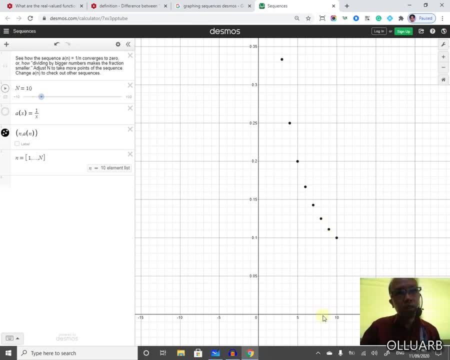 elements of the sequence before up to here. so this is now our sequence, okay and, as you notice here, I'm going to explain again here that we will be focusing all these elements of the sequence before up to here. so this is now our sequence, okay and, as you notice here, I'm going to explain again here that we will be focusing all these. 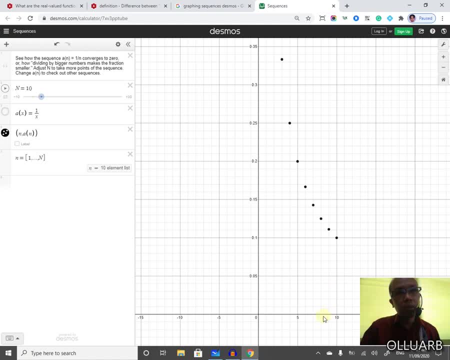 elements of the sequence before up to here. so this is now our sequence, okay and, as you notice here, I'm going to explain again here that we will be focusing all these elements of the sequence before up to here. so this is now our sequence, okay and, as you notice here, I'm going to explain again here that we will be focusing all these. 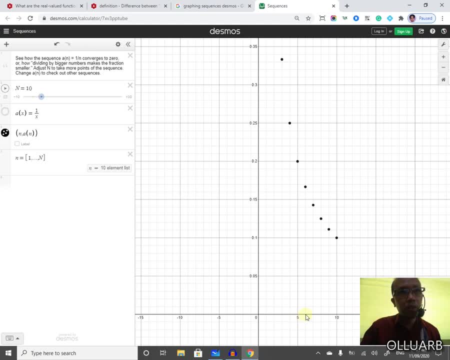 elements of the sequence before up to here. so this is now our sequence, okay and, as you notice here, I'm going to explain again here that we will be focusing all these elements of the sequence before up to here. so this is now our sequence, okay and, as you notice here, I'm going to explain again here that we will be focusing all these. 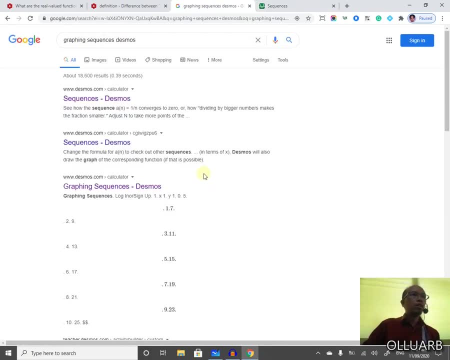 elements of the sequence before up to here. so this is now our sequence, okay and, as you notice here, I'm going to explain again here that we will be focusing all these elements of the sequence before up to here. so this is now our sequence, okay and, as you notice here, I'm going to explain again here that we will be focusing all these. 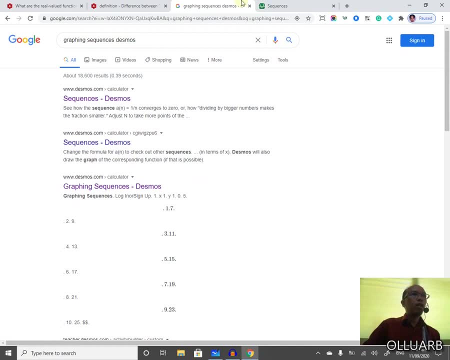 elements of the sequence before up to here. so this is now our sequence, okay and, as you notice here, I'm going to explain again here that we will be focusing all these elements of the sequence before up to here. so this is now our sequence, okay and, as you notice here, I'm going to explain again here that we will be focusing all these. 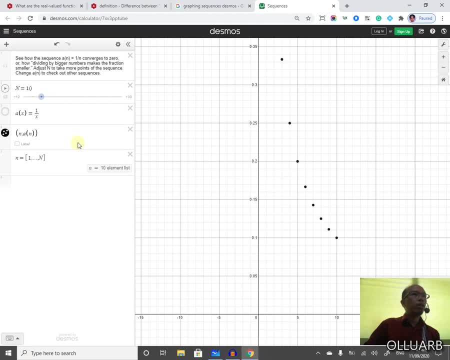 elements of the sequence before up to here. so this is now our sequence, okay and, as you notice here, I'm going to explain again here that we will be focusing all these elements of the sequence before up to here. so this is now our sequence, okay and, as you notice here, I'm going to explain again here that we will be focusing all these. 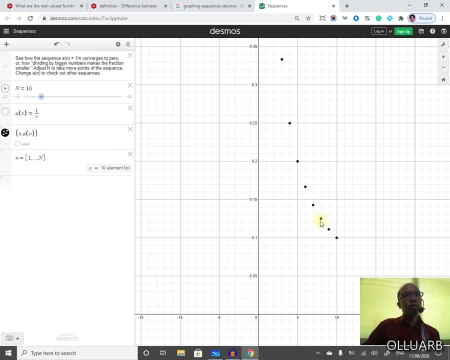 elements of the sequence before up to here. so this is now our sequence, okay and, as you notice here, I'm going to explain again here that we will be focusing all these elements of the sequence before up to here. so this is now our sequence, okay and, as you notice here, I'm going to explain again here that we will be focusing all these. 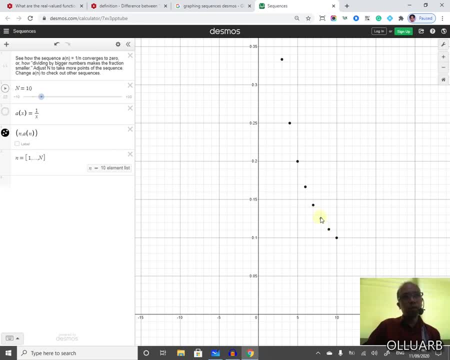 elements of the sequence before up to here. so this is now our sequence, okay and, as you notice here, I'm going to explain again here that we will be focusing all these elements of the sequence before up to here. so this is now our sequence, okay and, as you notice here, I'm going to explain again here that we will be focusing all these. 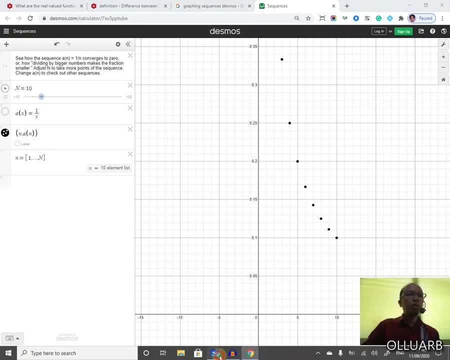 elements of the sequence before up to here. so this is now our sequence, okay and, as you notice here, I'm going to explain again here that we will be focusing all these elements of the sequence before up to here. so this is now our sequence, okay and, as you notice here, I'm going to explain again here that we will be focusing all these. 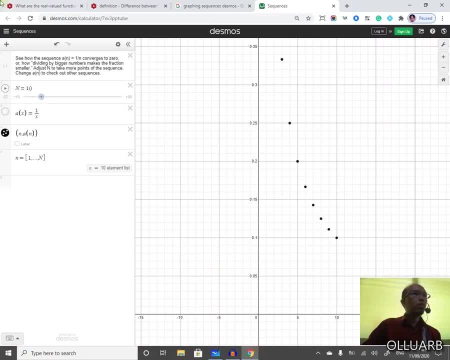 elements of the sequence before up to here. so this is now our sequence, okay and, as you notice here, I'm going to explain again here that we will be focusing all these elements of the sequence before up to here. so this is now our sequence, okay and, as you notice here, I'm going to explain again here that we will be focusing all these. 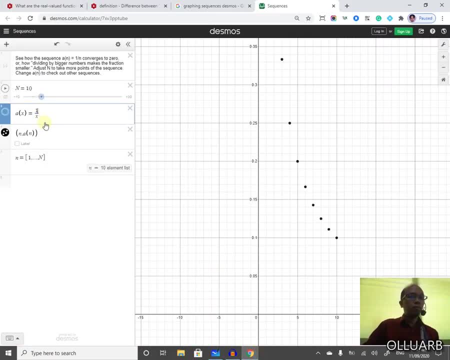 elements of the sequence before up to here. so this is now our sequence, okay and, as you notice here, I'm going to explain again here that we will be focusing all these elements of the sequence before up to here. so this is now our sequence, okay and, as you notice here, I'm going to explain again here that we will be focusing all these. 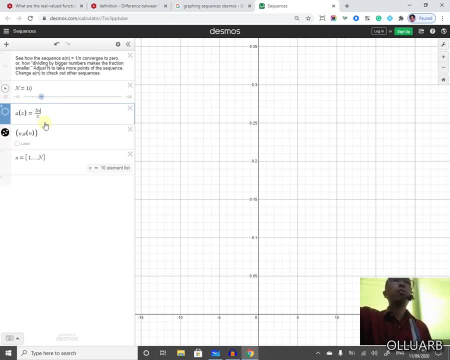 elements of the sequence before up to here. so this is now our sequence, okay and, as you notice here, I'm going to explain again here that we will be focusing all these elements of the sequence before up to here. so this is now our sequence, okay and, as you notice here, I'm going to explain again here that we will be focusing all these. 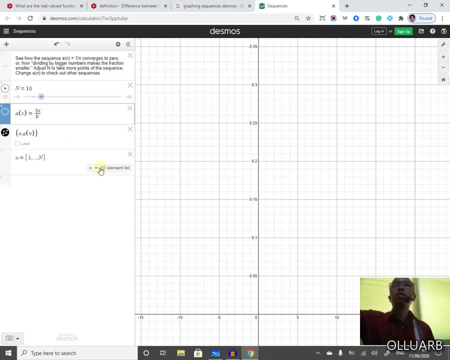 elements of the sequence before up to here. so this is now our sequence, okay and, as you notice here, I'm going to explain again here that we will be focusing all these elements of the sequence before up to here. so this is now our sequence, okay and, as you notice here, I'm going to explain again here that we will be focusing all these. 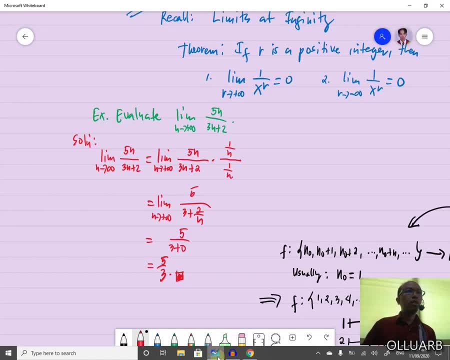 elements of the sequence before up to here. so this is now our sequence, okay and, as you notice here, I'm going to explain again here that we will be focusing all these elements of the sequence before up to here. so this is now our sequence, okay and, as you notice here, I'm going to explain again here that we will be focusing all these. 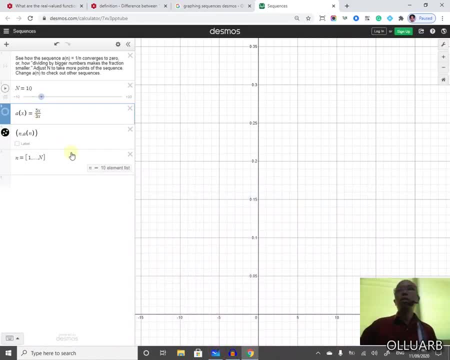 elements of the sequence before up to here. so this is now our sequence, okay and, as you notice here, I'm going to explain again here that we will be focusing all these elements of the sequence before up to here. so this is now our sequence, okay and, as you notice here, I'm going to explain again here that we will be focusing all these. 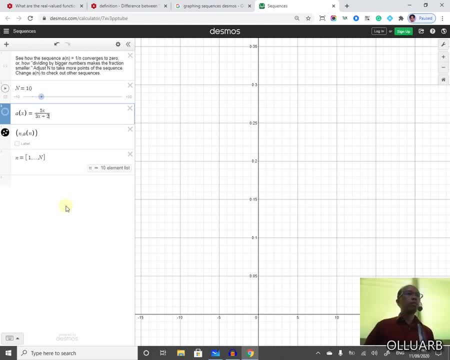 elements of the sequence before up to here. so this is now our sequence, okay and, as you notice here, I'm going to explain again here that we will be focusing all these elements of the sequence before up to here. so this is now our sequence, okay and, as you notice here, I'm going to explain again here that we will be focusing all these. 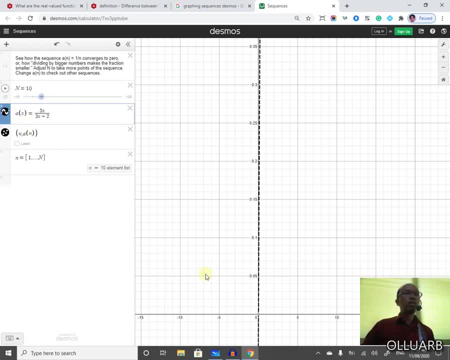 elements of the sequence before up to here. so this is now our sequence, okay and, as you notice here, I'm going to explain again here that we will be focusing all these elements of the sequence before up to here. so this is now our sequence, okay and, as you notice here, I'm going to explain again here that we will be focusing all these. 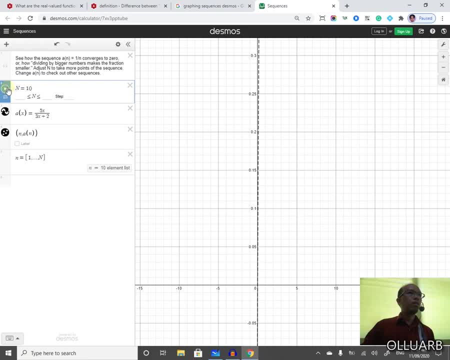 elements of the sequence before up to here. so this is now our sequence, okay and, as you notice here, I'm going to explain again here that we will be focusing all these elements of the sequence before up to here. so this is now our sequence, okay and, as you notice here, I'm going to explain again here that we will be focusing all these. 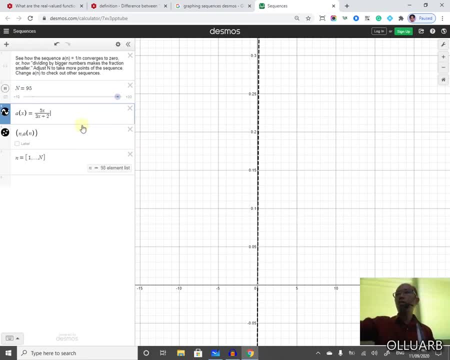 elements of the sequence before up to here. so this is now our sequence, okay and, as you notice here, I'm going to explain again here that we will be focusing all these elements of the sequence before up to here. so this is now our sequence, okay and, as you notice here, I'm going to explain again here that we will be focusing all these. 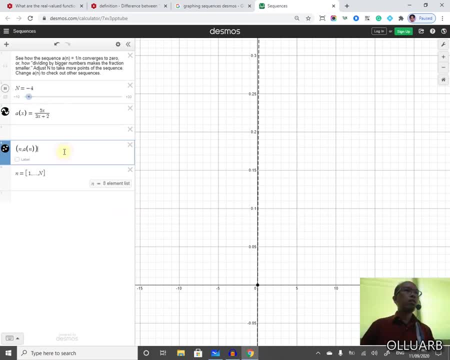 elements of the sequence before up to here. so this is now our sequence, okay and, as you notice here, I'm going to explain again here that we will be focusing all these elements of the sequence before up to here. so this is now our sequence, okay and, as you notice here, I'm going to explain again here that we will be focusing all these. 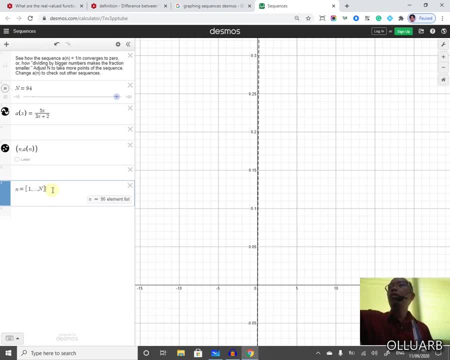 elements of the sequence before up to here. so this is now our sequence, okay and, as you notice here, I'm going to explain again here that we will be focusing all these elements of the sequence before up to here. so this is now our sequence, okay and, as you notice here, I'm going to explain again here that we will be focusing all these. 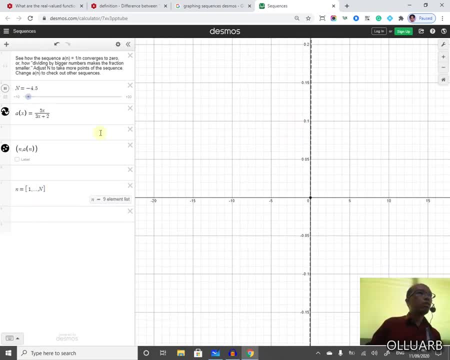 elements of the sequence before up to here. so this is now our sequence, okay and, as you notice here, I'm going to explain again here that we will be focusing all these elements of the sequence before up to here. so this is now our sequence, okay and, as you notice here, I'm going to explain again here that we will be focusing all these. 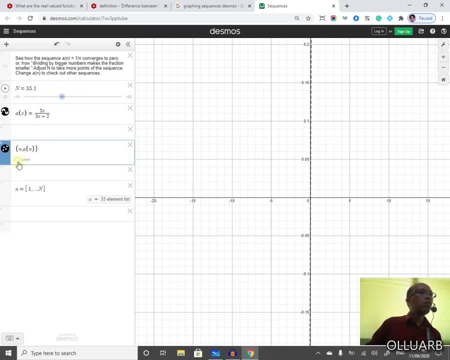 elements of the sequence before up to here. so this is now our sequence, okay and, as you notice here, I'm going to explain again here that we will be focusing all these elements of the sequence before up to here. so this is now our sequence, okay and, as you notice here, I'm going to explain again here that we will be focusing all these. 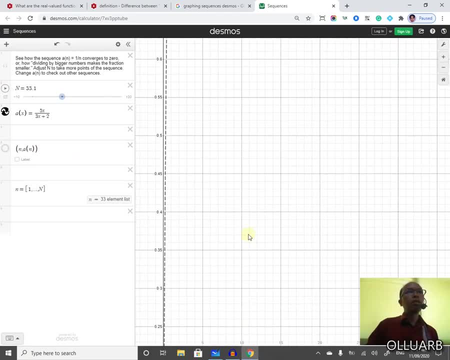 elements of the sequence before up to here. so this is now our sequence, okay and, as you notice here, I'm going to explain again here that we will be focusing all these elements of the sequence before up to here. so this is now our sequence, okay and, as you notice here, I'm going to explain again here that we will be focusing all these. 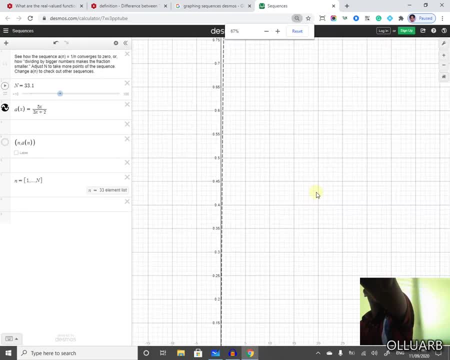 elements of the sequence before up to here. so this is now our sequence, okay and, as you notice here, I'm going to explain again here that we will be focusing all these elements of the sequence before up to here. so this is now our sequence, okay and, as you notice here, I'm going to explain again here that we will be focusing all these. 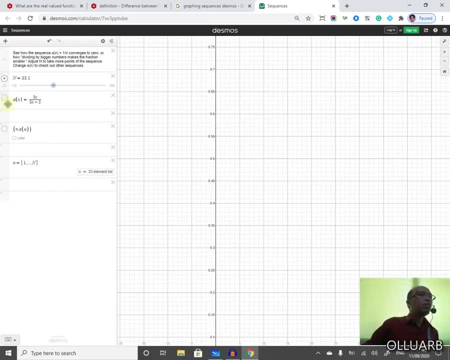 elements of the sequence before up to here. so this is now our sequence, okay and, as you notice here, I'm going to explain again here that we will be focusing all these elements of the sequence before up to here. so this is now our sequence, okay and, as you notice here, I'm going to explain again here that we will be focusing all these. 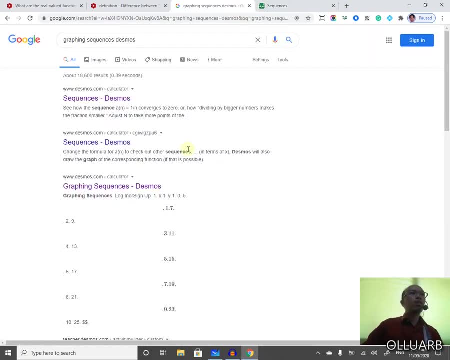 elements of the sequence before up to here. so this is now our sequence, okay and, as you notice here, I'm going to explain again here that we will be focusing all these elements of the sequence before up to here. so this is now our sequence, okay and, as you notice here, I'm going to explain again here that we will be focusing all these. 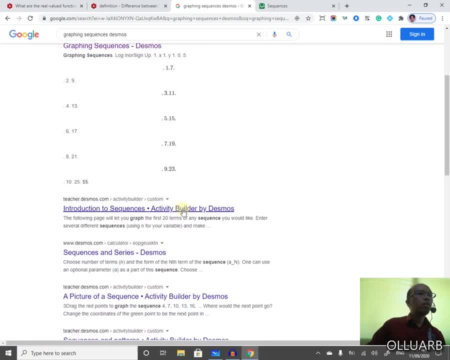 elements of the sequence before up to here. so this is now our sequence, okay and, as you notice here, I'm going to explain again here that we will be focusing all these elements of the sequence before up to here. so this is now our sequence, okay and, as you notice here, I'm going to explain again here that we will be focusing all these. 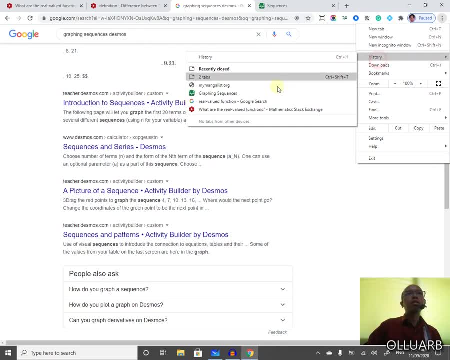 elements of the sequence before up to here. so this is now our sequence, okay and, as you notice here, I'm going to explain again here that we will be focusing all these elements of the sequence before up to here. so this is now our sequence, okay and, as you notice here, I'm going to explain again here that we will be focusing all these. 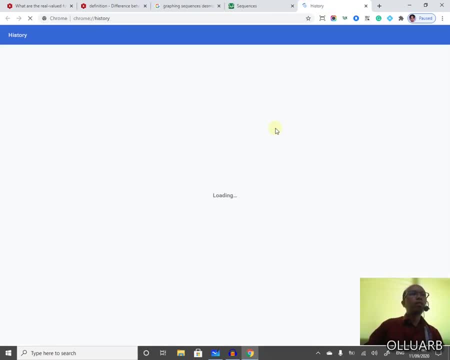 elements of the sequence before up to here. so this is now our sequence, okay and, as you notice here, I'm going to explain again here that we will be focusing all these elements of the sequence before up to here. so this is now our sequence, okay and, as you notice here, I'm going to explain again here that we will be focusing all these. 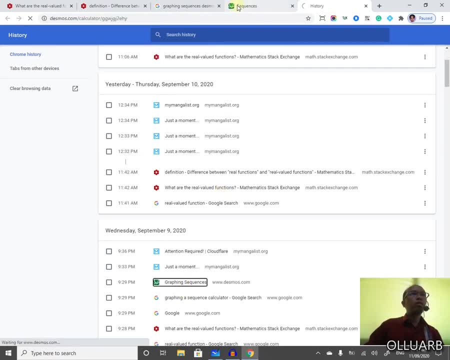 elements of the sequence before up to here. so this is now our sequence, okay and, as you notice here, I'm going to explain again here that we will be focusing all these elements of the sequence before up to here. so this is now our sequence, okay and, as you notice here, I'm going to explain again here that we will be focusing all these. 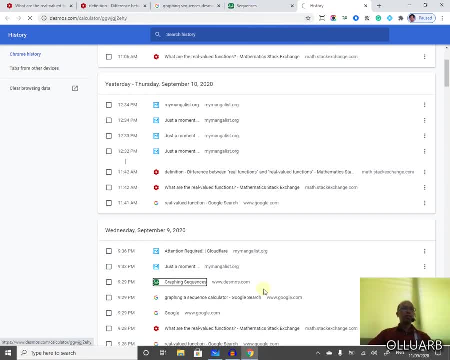 elements of the sequence before up to here. so this is now our sequence, okay and, as you notice here, I'm going to explain again here that we will be focusing all these elements of the sequence before up to here. so this is now our sequence, okay and, as you notice here, I'm going to explain again here that we will be focusing all these. 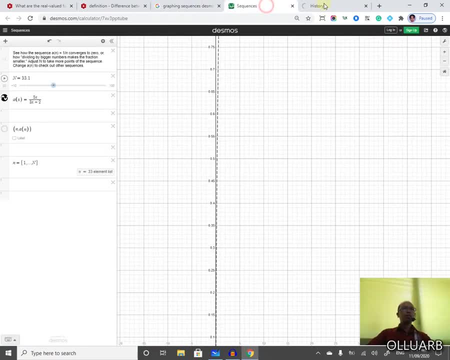 elements of the sequence before up to here. so this is now our sequence, okay and, as you notice here, I'm going to explain again here that we will be focusing all these elements of the sequence before up to here. so this is now our sequence, okay and, as you notice here, I'm going to explain again here that we will be focusing all these. 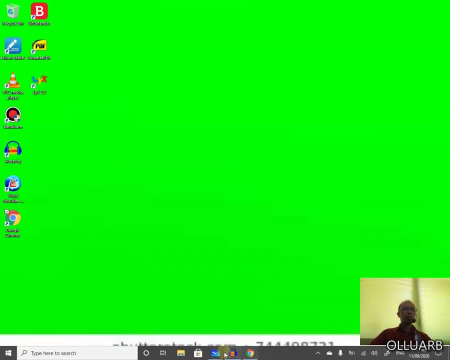 elements of the sequence before up to here. so this is now our sequence, okay and, as you notice here, I'm going to explain again here that we will be focusing all these elements of the sequence before up to here. so this is now our sequence, okay and, as you notice here, I'm going to explain again here that we will be focusing all these. 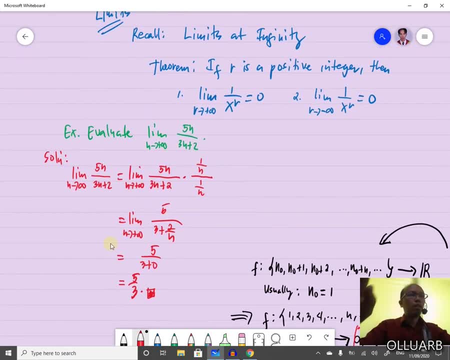 elements of the sequence before up to here. so this is now our sequence, okay and, as you notice here, I'm going to explain again here that we will be focusing all these elements of the sequence before up to here. so this is now our sequence, okay and, as you notice here, I'm going to explain again here that we will be focusing all these. 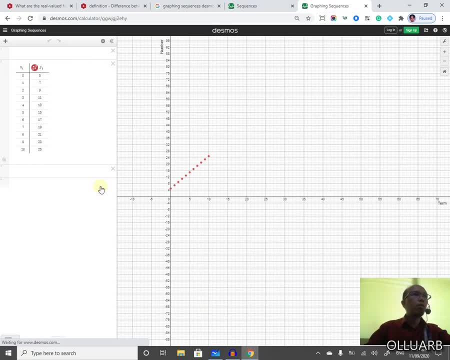 elements of the sequence before up to here. so this is now our sequence, okay and, as you notice here, I'm going to explain again here that we will be focusing all these elements of the sequence before up to here. so this is now our sequence, okay and, as you notice here, I'm going to explain again here that we will be focusing all these. 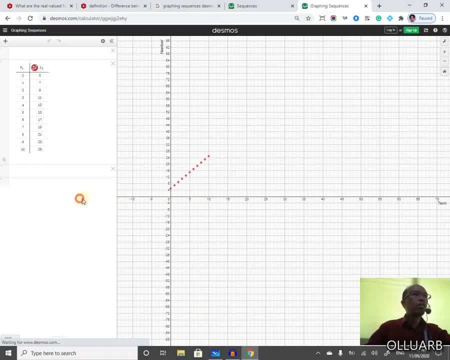 elements of the sequence before up to here. so this is now our sequence, okay and, as you notice here, I'm going to explain again here that we will be focusing all these elements of the sequence before up to here. so this is now our sequence, okay and, as you notice here, I'm going to explain again here that we will be focusing all these. 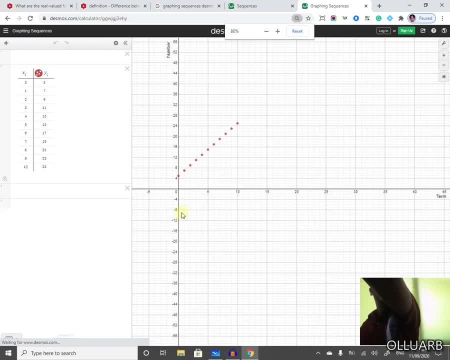 elements of the sequence before up to here. so this is now our sequence, okay and, as you notice here, I'm going to explain again here that we will be focusing all these elements of the sequence before up to here. so this is now our sequence, okay and, as you notice here, I'm going to explain again here that we will be focusing all these. 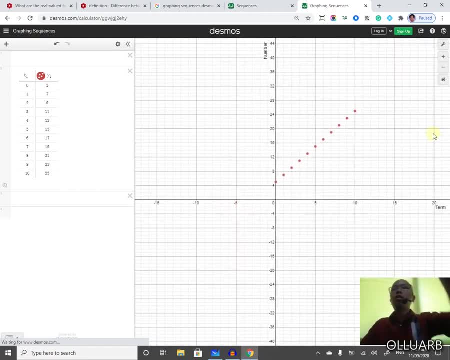 elements of the sequence before up to here. so this is now our sequence, okay and, as you notice here, I'm going to explain again here that we will be focusing all these elements of the sequence before up to here. so this is now our sequence, okay and, as you notice here, I'm going to explain again here that we will be focusing all these. 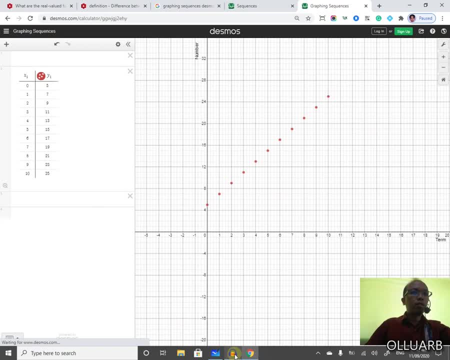 elements of the sequence before up to here. so this is now our sequence, okay and, as you notice here, I'm going to explain again here that we will be focusing all these elements of the sequence before up to here. so this is now our sequence, okay and, as you notice here, I'm going to explain again here that we will be focusing all these. 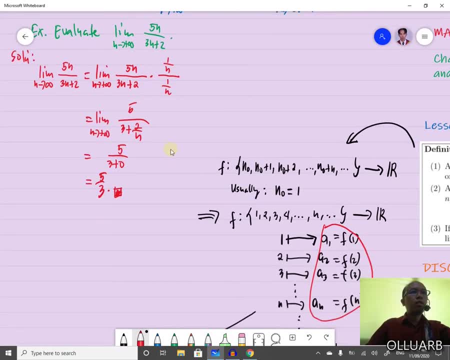 elements of the sequence before up to here. so this is now our sequence, okay and, as you notice here, I'm going to explain again here that we will be focusing all these elements of the sequence before up to here. so this is now our sequence, okay and, as you notice here, I'm going to explain again here that we will be focusing all these. 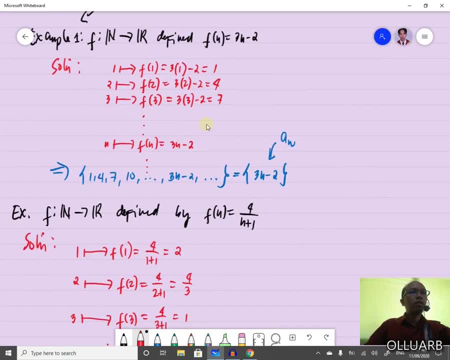 elements of the sequence before up to here. so this is now our sequence, okay and, as you notice here, I'm going to explain again here that we will be focusing all these elements of the sequence before up to here. so this is now our sequence, okay and, as you notice here, I'm going to explain again here that we will be focusing all these. 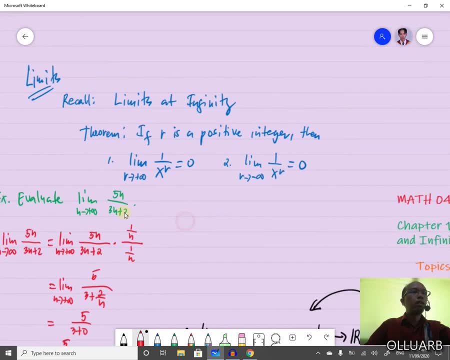 elements of the sequence before up to here. so this is now our sequence, okay and, as you notice here, I'm going to explain again here that we will be focusing all these elements of the sequence before up to here. so this is now our sequence, okay and, as you notice here, I'm going to explain again here that we will be focusing all these. 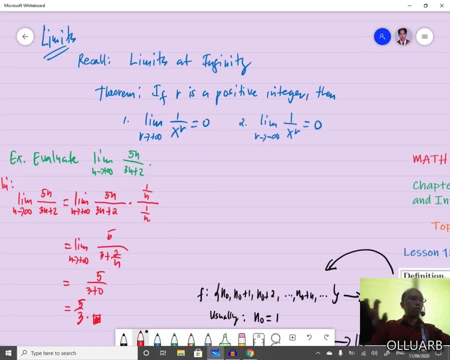 elements of the sequence before up to here. so this is now our sequence, okay and, as you notice here, I'm going to explain again here that we will be focusing all these elements of the sequence before up to here. so this is now our sequence, okay and, as you notice here, I'm going to explain again here that we will be focusing all these. 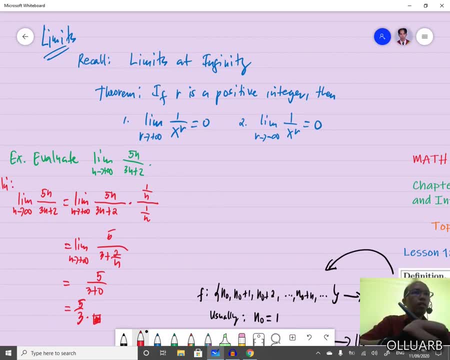 elements of the sequence before up to here. so this is now our sequence, okay and, as you notice here, I'm going to explain again here that we will be focusing all these elements of the sequence before up to here. so this is now our sequence, okay and, as you notice here, I'm going to explain again here that we will be focusing all these. 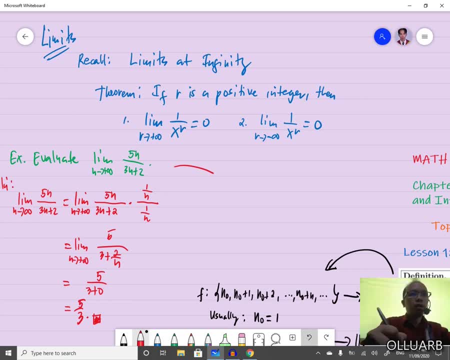 elements of the sequence before up to here. so this is now our sequence, okay and, as you notice here, I'm going to explain again here that we will be focusing all these elements of the sequence before up to here. so this is now our sequence, okay and, as you notice here, I'm going to explain again here that we will be focusing all these. 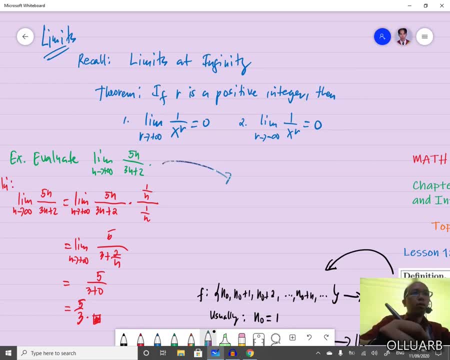 elements of the sequence before up to here. so this is now our sequence, okay and, as you notice here, I'm going to explain again here that we will be focusing all these elements of the sequence before up to here. so this is now our sequence, okay and, as you notice here, I'm going to explain again here that we will be focusing all these. 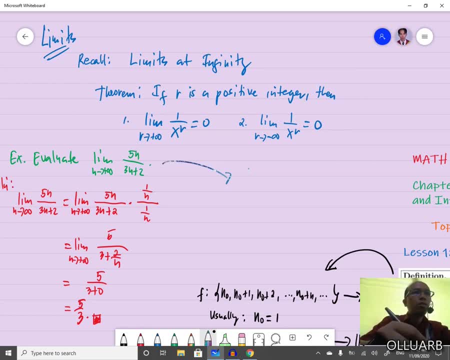 elements of the sequence before up to here. so this is now our sequence, okay and, as you notice here, I'm going to explain again here that we will be focusing all these elements of the sequence before up to here. so this is now our sequence, okay and, as you notice here, I'm going to explain again here that we will be focusing all these. 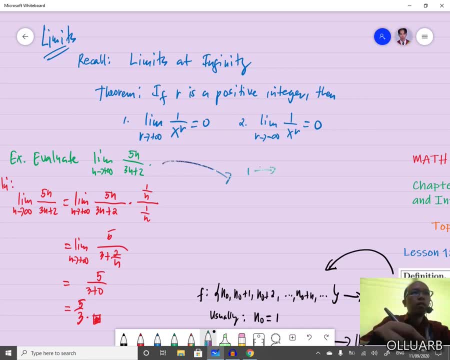 elements of the sequence before up to here. so this is now our sequence, okay and, as you notice here, I'm going to explain again here that we will be focusing all these elements of the sequence before up to here. so this is now our sequence, okay and, as you notice here, I'm going to explain again here that we will be focusing all these. 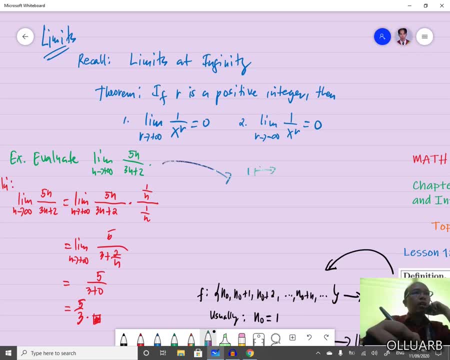 elements of the sequence before up to here. so this is now our sequence, okay and, as you notice here, I'm going to explain again here that we will be focusing all these elements of the sequence before up to here. so this is now our sequence, okay and, as you notice here, I'm going to explain again here that we will be focusing all these. 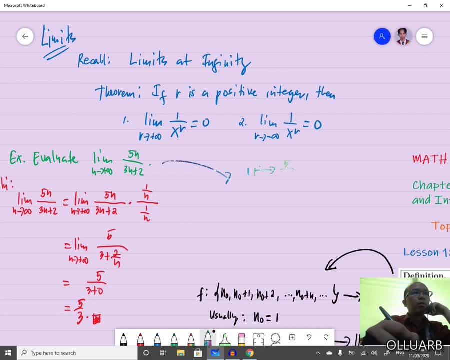 elements of the sequence before up to here. so this is now our sequence, okay and, as you notice here, I'm going to explain again here that we will be focusing all these elements of the sequence before up to here. so this is now our sequence, okay and, as you notice here, I'm going to explain again here that we will be focusing all these. 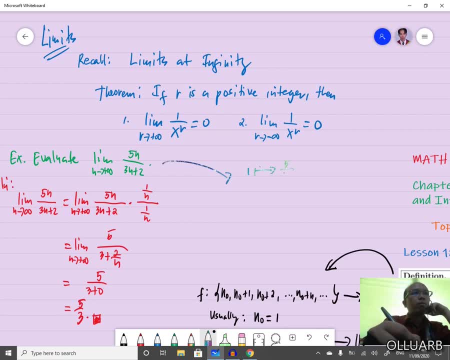 elements of the sequence before up to here. so this is now our sequence, okay and, as you notice here, I'm going to explain again here that we will be focusing all these elements of the sequence before up to here. so this is now our sequence, okay and, as you notice here, I'm going to explain again here that we will be focusing all these. 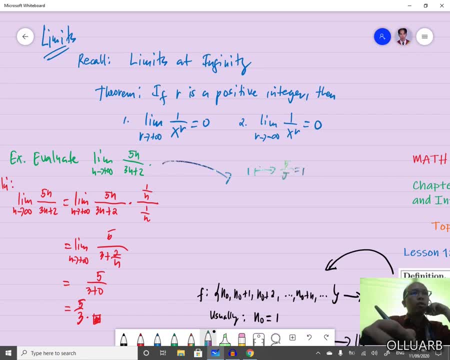 elements of the sequence before up to here. so this is now our sequence, okay and, as you notice here, I'm going to explain again here that we will be focusing all these elements of the sequence before up to here. so this is now our sequence, okay and, as you notice here, I'm going to explain again here that we will be focusing all these. 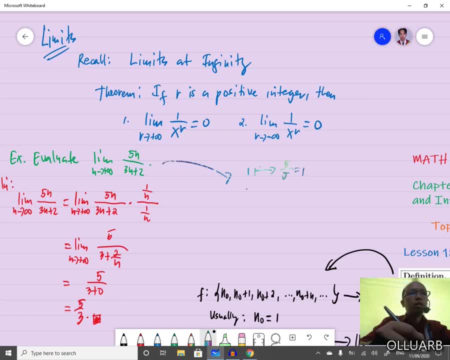 elements of the sequence before up to here. so this is now our sequence, okay and, as you notice here, I'm going to explain again here that we will be focusing all these elements of the sequence before up to here. so this is now our sequence, okay and, as you notice here, I'm going to explain again here that we will be focusing all these. 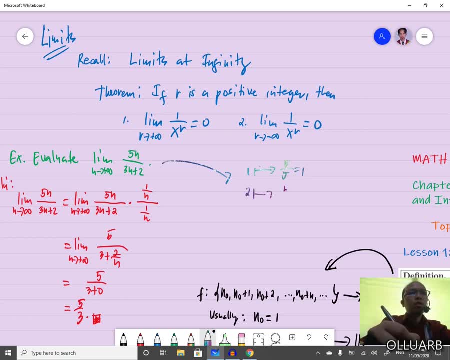 elements of the sequence before up to here. so this is now our sequence, okay and, as you notice here, I'm going to explain again here that we will be focusing all these elements of the sequence before up to here. so this is now our sequence, okay and, as you notice here, I'm going to explain again here that we will be focusing all these. 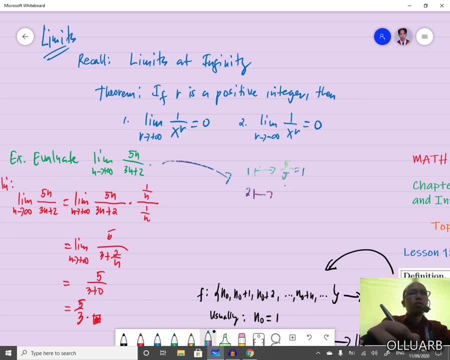 elements of the sequence before up to here. so this is now our sequence, okay and, as you notice here, I'm going to explain again here that we will be focusing all these elements of the sequence before up to here. so this is now our sequence, okay and, as you notice here, I'm going to explain again here that we will be focusing all these. 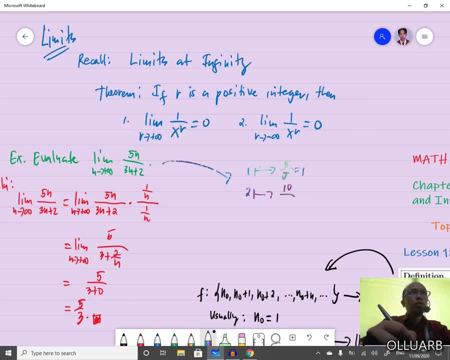 elements of the sequence before up to here. so this is now our sequence, okay and, as you notice here, I'm going to explain again here that we will be focusing all these elements of the sequence before up to here. so this is now our sequence, okay and, as you notice here, I'm going to explain again here that we will be focusing all these. 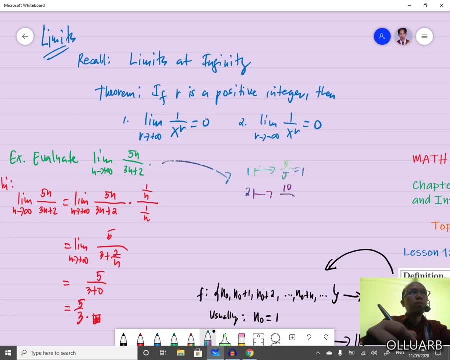 elements of the sequence before up to here. so this is now our sequence, okay and, as you notice here, I'm going to explain again here that we will be focusing all these elements of the sequence before up to here. so this is now our sequence, okay and, as you notice here, I'm going to explain again here that we will be focusing all these. 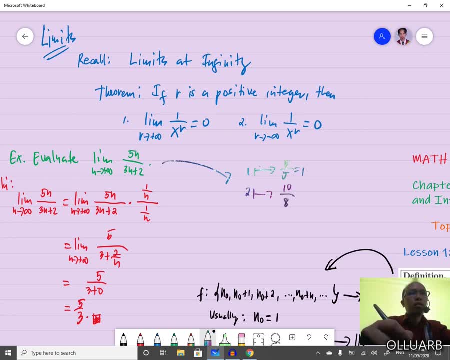 elements of the sequence before up to here. so this is now our sequence. okay, and as you notice here, I'm going to explain again here that we will be focusing all these elements of the sequence before up to here. so this is now our sequence. eight, or this is divide two, five, I think it's. let's try to use another five, four when n. 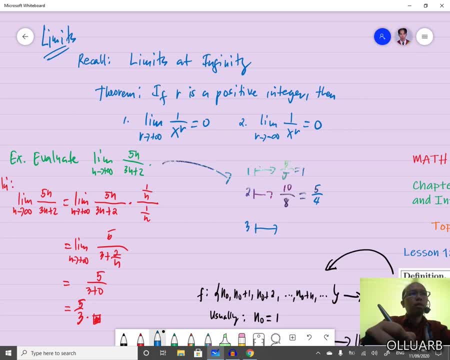 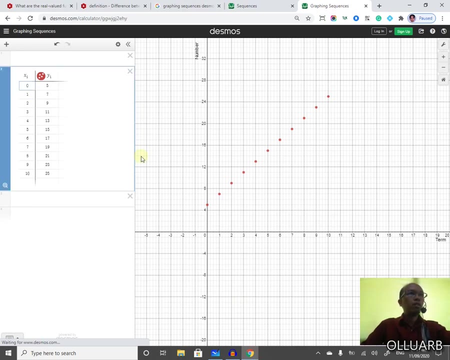 is equal to three. we have three times 5, 15, 3 times 3, 9 plus 2, 11, that one. so let's try to drop this one. when it is one, then it is map to one. okay, one when it is two. as you can see, I'm trying to delete that one. when it is two, it is. 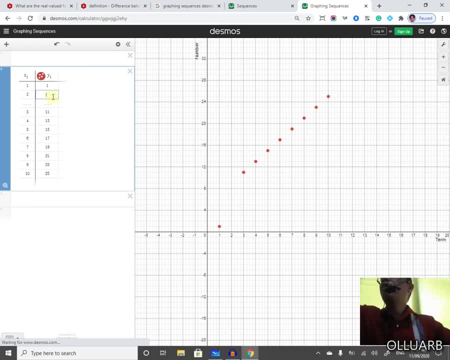 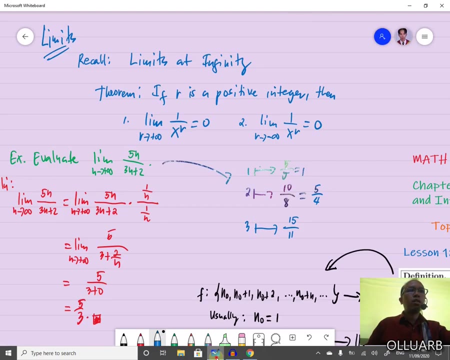 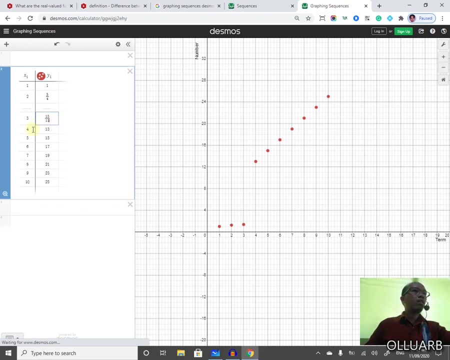 equivalent to five over four. five over four: okay. so when it is 3, 3, not three, I like 15 over 11, 15 over 11, okay. so as you can see, here, we forget about this. point C, okay, points in. as you can see, this approaches. 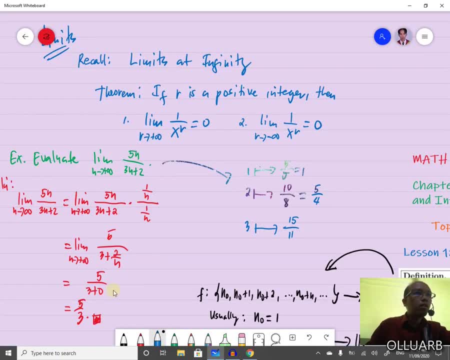 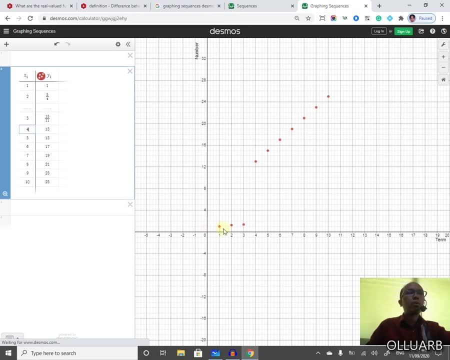 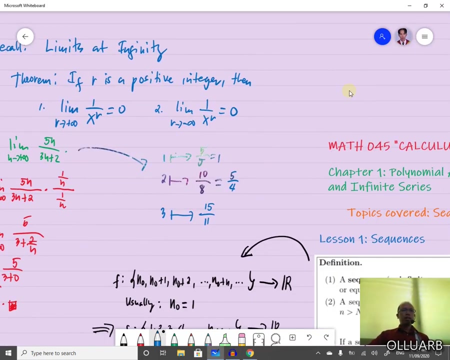 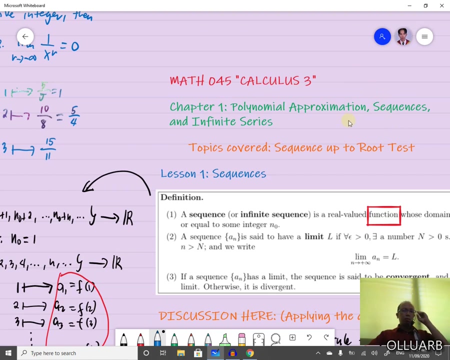 to 5 over 3. okay, which is the 5 over? what is the value? 5 over 3? so check your calculator. I guess that there will be a limit here which is equal to 5 over 3. so that's definition number two. but if you try to solve to prove that the limit is, 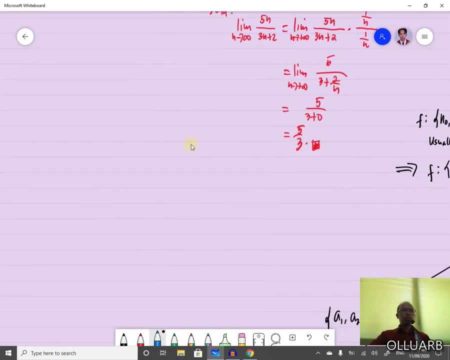 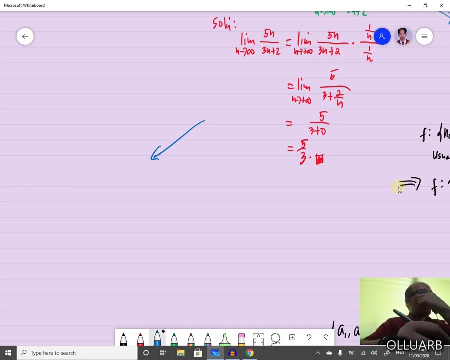 really equal to two using the definition. so let's try to answer this one. so if you recall your calculus again, okay this one. so if you recall your calculus again, okay this one. so if you recall your calculus again, okay this one. it's prov. musical, its status, prove, prove using definition. so meaning to say: 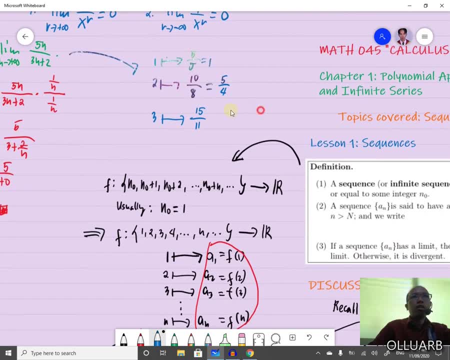 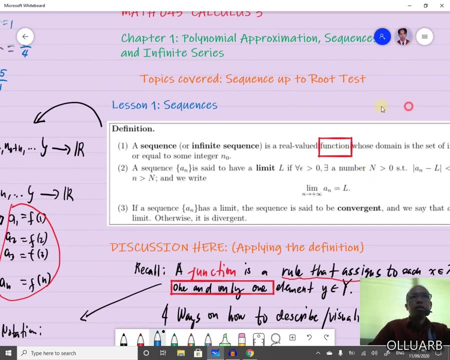 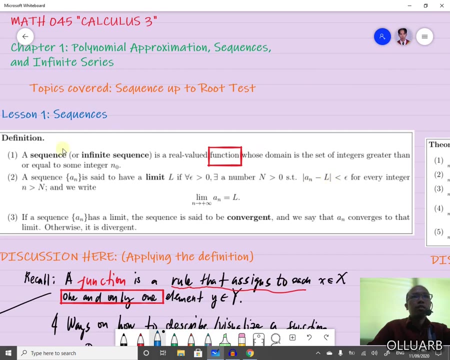 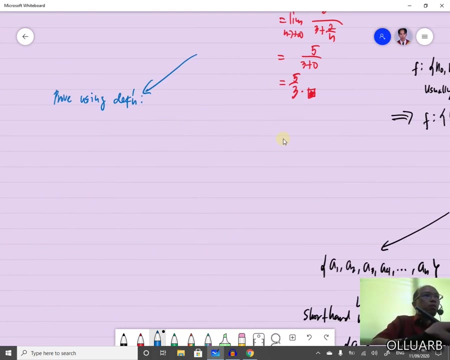 we have to find a, we have to find, we begin, you have to find, begin by solving this one, hoping this one. okay, so we have to get an epsilon. so let epsilon be greater than zero. then let's try to solve a n minus n. so, as you can see, our limit is five thirds. so we have: our function is 5 n over 3 n. 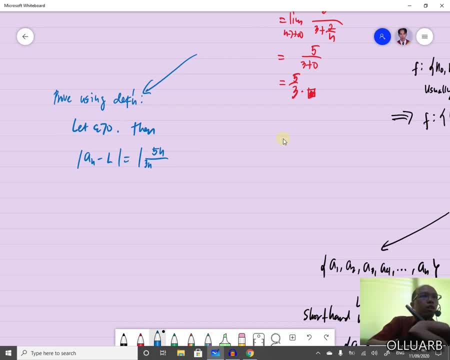 sorry, 3 n plus 2 minus 5 over 3. so let's try to simplify this. get the lcd. our lcd is 3 and 3 n plus 2, sorry. so divide times. so we have 3 times 5 n is 15. 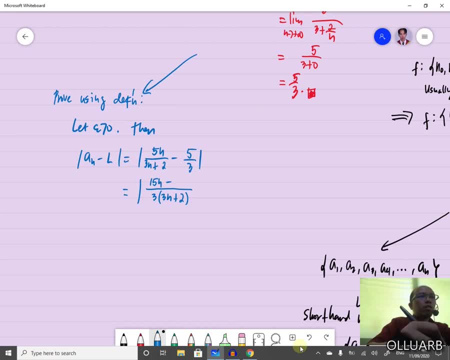 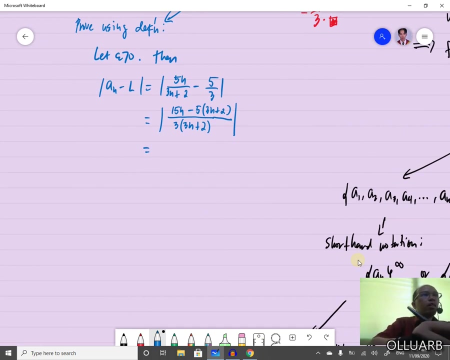 sorry, and minus uh, 5 times 3 n plus 2. okay, let's move this up then. if you further simplify this, this will become 3, 3 n plus 2, so we have 15 n minus 15 on my right. so we have to add that one. this becomes zero. 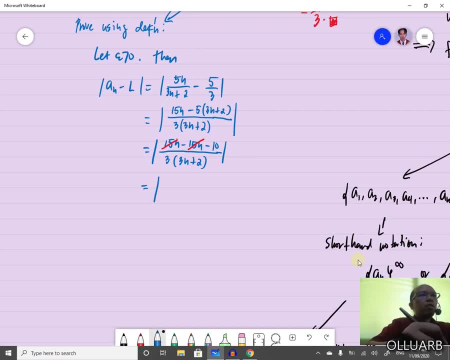 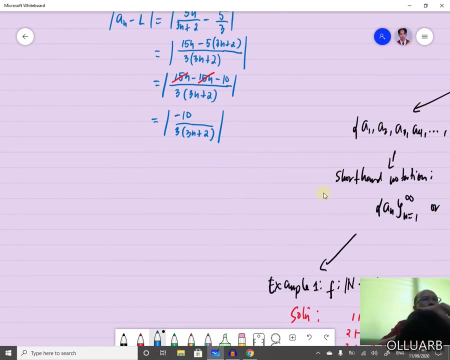 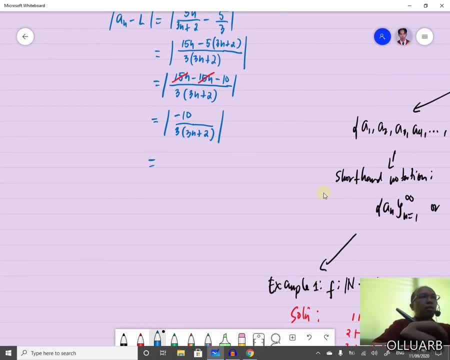 notice that since our n are positive integers, then we can remove the absolute value, which is 3 times 3 n plus 2.. remove the absolute value, which is 3 times 3 n plus 2.. sorry, sorry, let's try to remove this one. 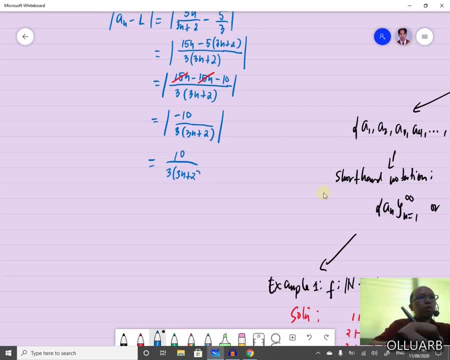 let's try to remove this one and go. okay, so let's try to see if we can do this. okay, so what should we do here? so this will become 10 over 3 times 3 n plus two less than epsilon, because if you look at the definition, this will be less than epsilon, because 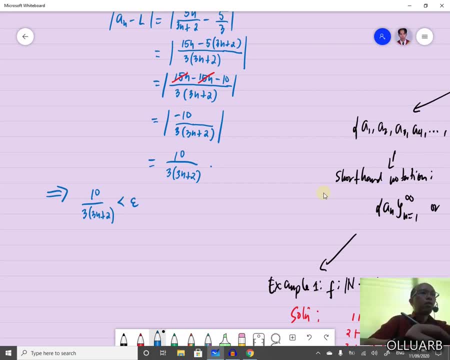 if you look at the definition, this will be less than epsilon. because this is less than epsilon, we are trying to solve this by separating epsilon and n, so cross multiplying, we have 10. it's time 3 epsilon, 3 n plus 2. so divide both sides by 3 epsilon. 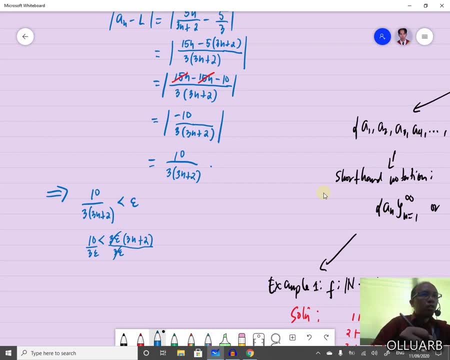 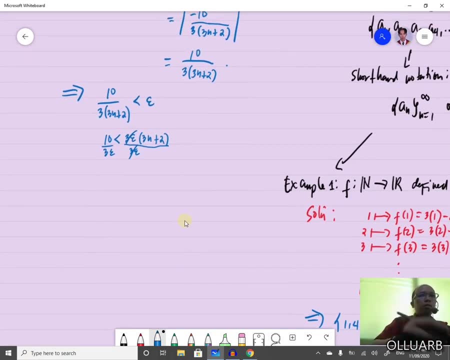 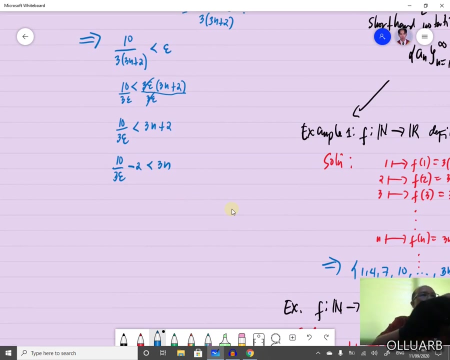 and then we can cancel out that one because our epsilon is greater than zero, so epsilon is not equal to zero. so we have 10 over 3 epsilon less than 3, n plus 2. so you can, you can transfer on the other side our 2 and then try to combine okay. 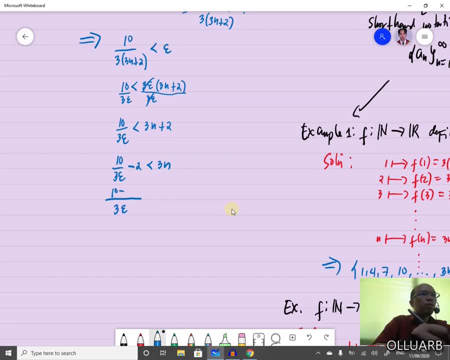 this is 10 minus 3 epsilon times 2 is 6, epsilon 3: n. so again can you? can multiply both sides by 1 third. multiply both sides by 1 third and you can cancel out. so this will become: lets change this to this one. 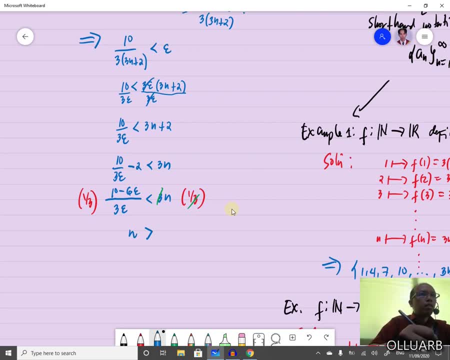 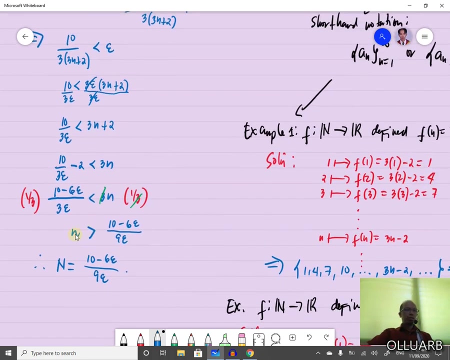 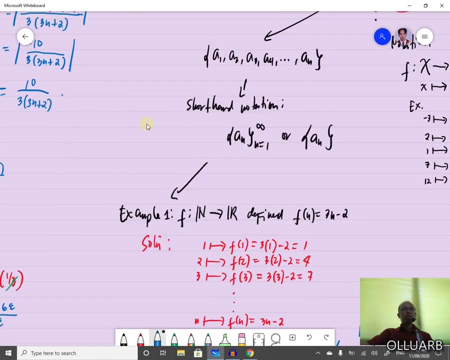 notice the sign. this is 10 minus 6 epsilon over 9 epsilon. so therefore, our big N is 10 minus 6 epsilon over 9 epsilon. okay, why? as you have notice, notice this one- that it must be n small. n must be greater than this one. so let's recall our definition where. 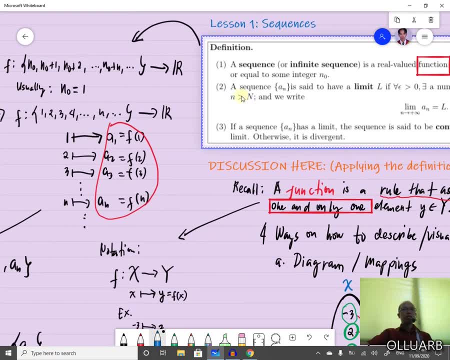 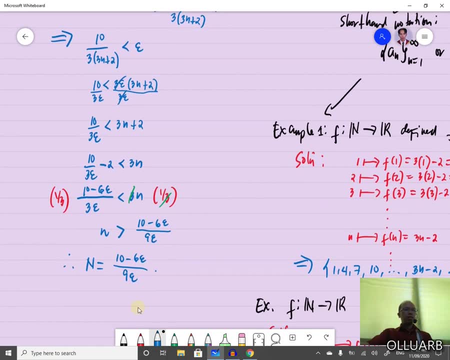 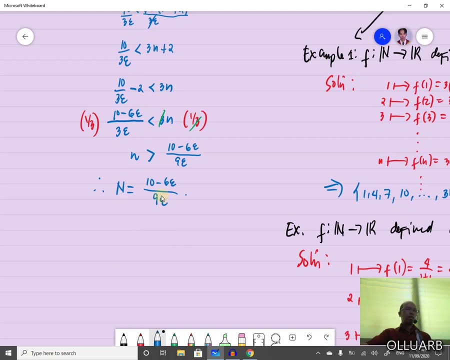 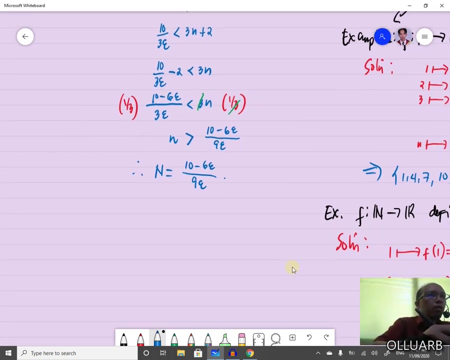 is our definition. yeah, okay, so meaning to say, if your n is this one, then the absolute value of the sequence a7 minus n is less than epsilon. so, in particular, so in particular, in particular, if you have epsilon, epsilon, epsilon, epsilon, which is, let's say, 0.1, 0.1, then our n is what let's try to solve. 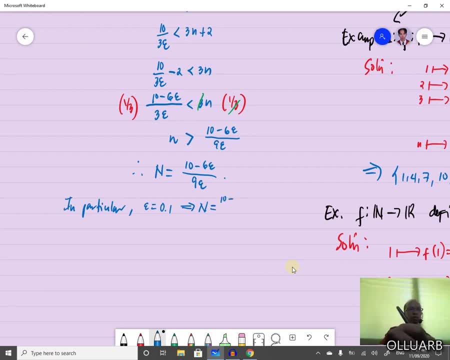 that one. for example, we have 10 minus 6 times 0.1 and then 9 to times 0.1. so what is the value of our personal calculator, then my calculator, and minus 6 times 0.1 and minus 6 times 0.1 and then 9 to. 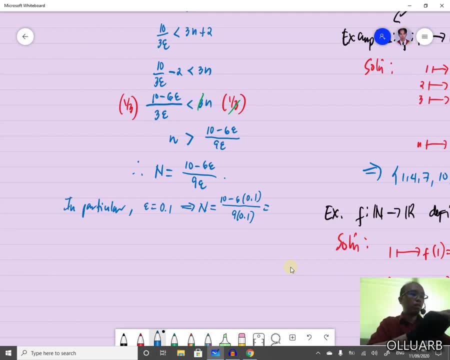 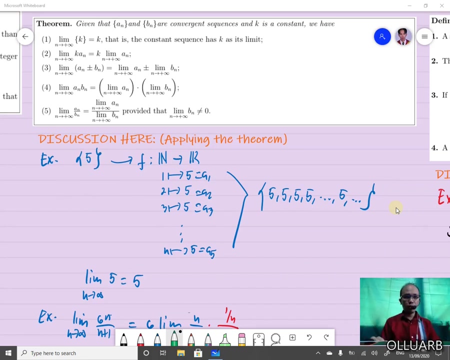 over 9 times 0.1. so our answer is 10.44. so this is 10.44. so meaning to say we can choose our small n to be 11 or 12, so pixel of 1 OFF. then when n is equal to lunch n or 12, then the absolute value of the sequence a7 minus l is less than epsilon. okay, hello everyone. I'm sorry I have to insert this video in the whole video tutorial because I have an instrument which is more important than epsilon. 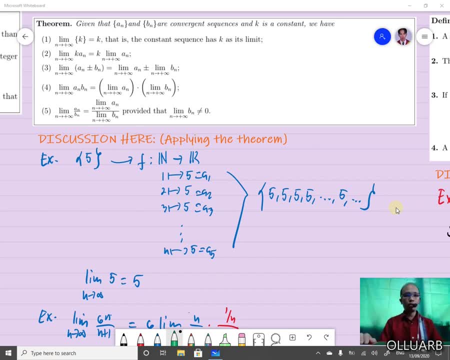 have some minor corrections. actually, there are two minor corrections that I have to point out, for example, this one: I write it as a sub five, so I guess this is correct. this is a sub n. yes, I have to erase this one, and then I will write as: 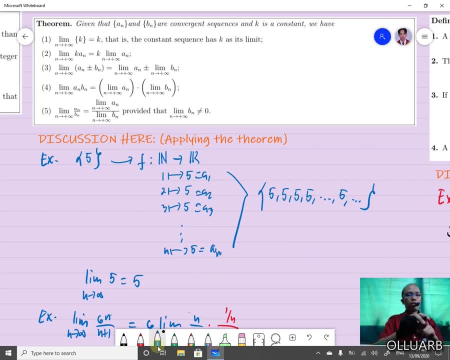 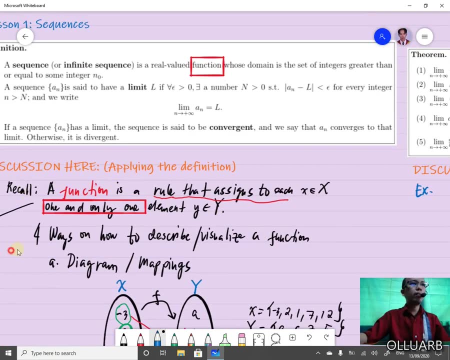 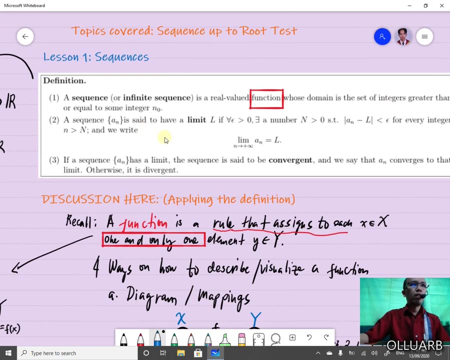 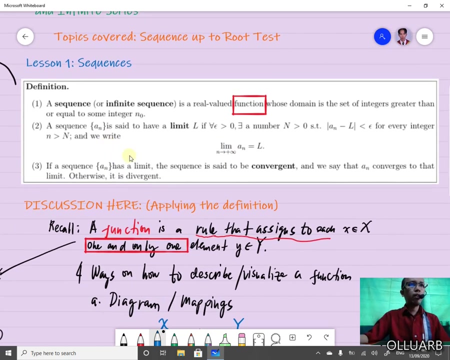 a sub n. okay, that's only the minor correction. and also, and also, as you can see here, in the definition of the second definition. I did not elaborate this as much when I, when I try to prove the limit of the of an example, I did not write it in a graceful manner, but I what I, just they did last, last, last. 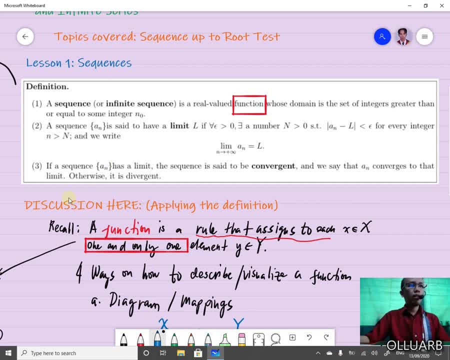 night is that I only try to find the value of the big N in terms of the epsilon. okay, so you can see here in the definition of the sub n. that's only the sketch of proof. but if you want a thesis like proof then you should have to refer some books. 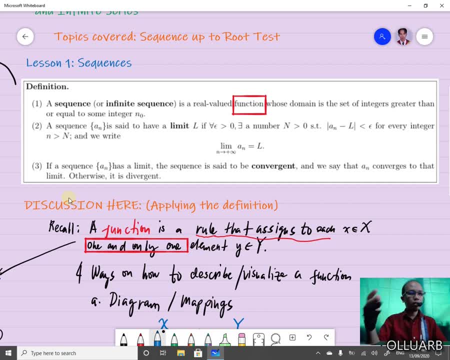 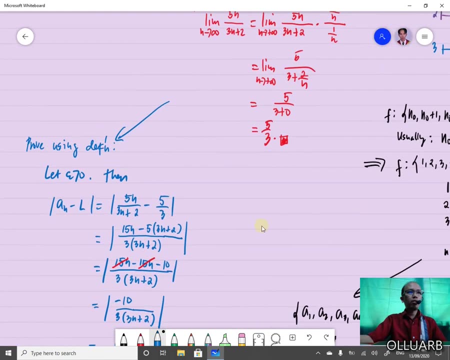 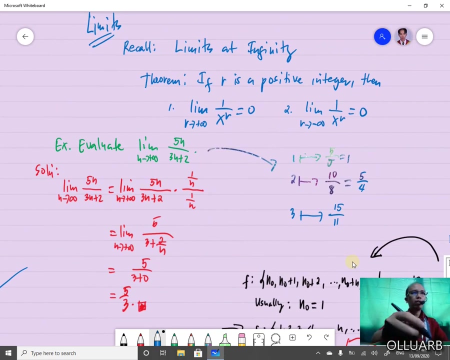 maybe light hold or Larson. you can look at the reference in this at the end of this video. okay, but anyway, I have to elaborate that more by showing that this one also, this one, this is not our, this is not our, this one, this is not our, but this is X as X approaches to. 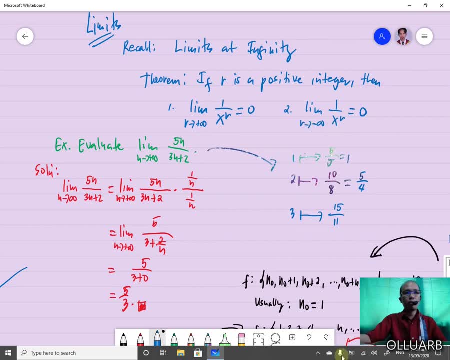 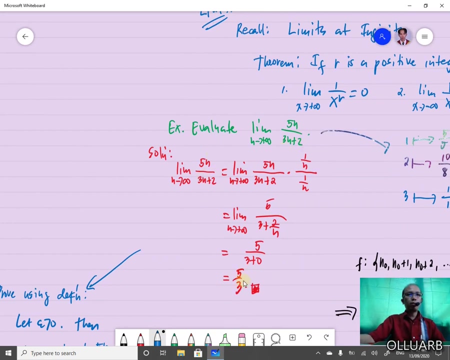 positive infinity and this is also X. okay, I have to correct this, this one by, but this one also. this one is esta limit, which is 5 over 3. it should be as X approaches the positive infinity. okay, what I will show you is to showыеン Sample. okay, It should be as X approaches to positive infinity. What will show you is to show this example. Example: if two limit, why is it the limit is five over 3? by using the thanked, what they call this one may be something I cannot do. I hear nothing but functions, complex точки that calculate the ml. one which means2 is negative the limit, what Started From? negative 2 is an inch horizontal value, So make even the difference clean. 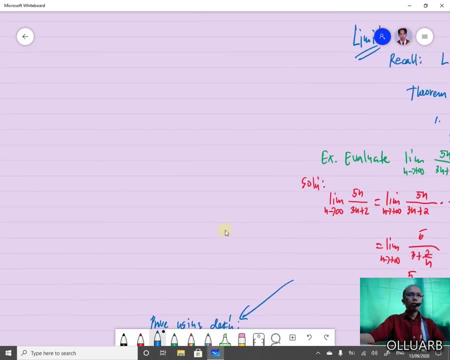 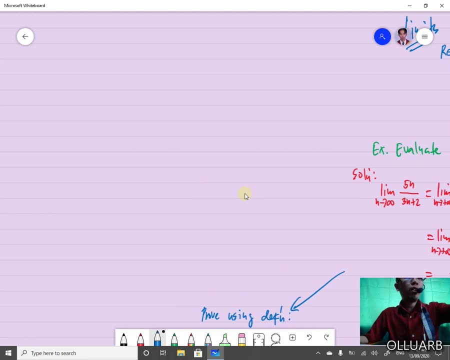 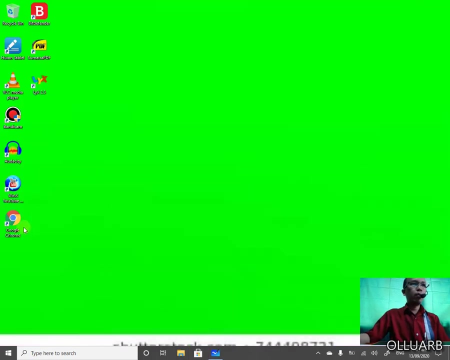 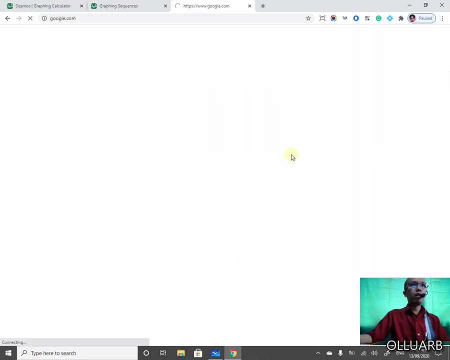 definition. okay. so, as you can see, if this is the, if you look at the graph of the sequence 5 n over 3, n plus 2, for example, if you will go to the article, this one, this most, this most graphing calculator, if you look at the, this most. 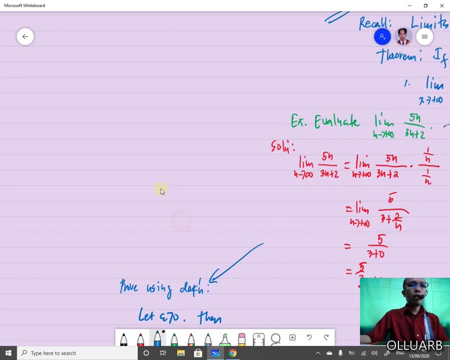 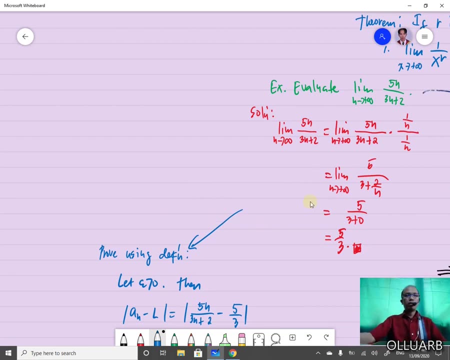 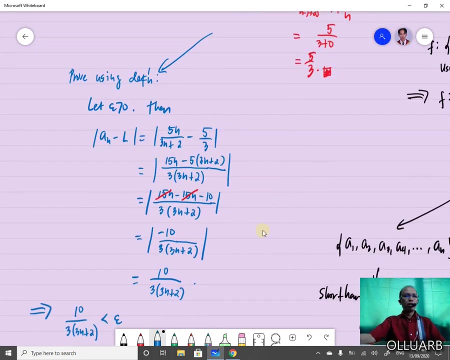 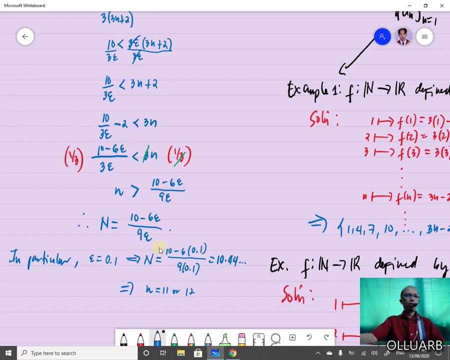 graphing calculator, you will see that. why is it? why is it that the vertical, this one, the, the limit of this function is 5 over 3? by using the definition, I prove it here. and then we we saw that our bigger n is 10 minus 6 epsilon over 9 epsilon. and in particular, if your epsilon is: 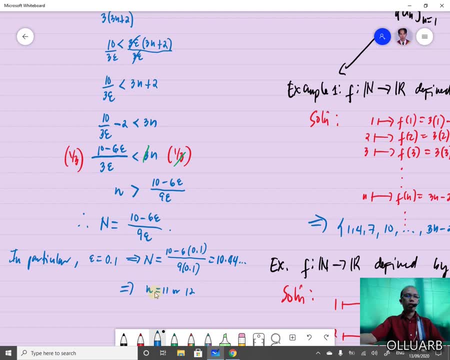 0.1. you have your n will start. you start at a small end, which is equal to 11, and you stay starting point. and if epsilon is point 1, what if epsilon is point 2? then you have an undervalue of n. so what does what does it mean? okay, what does it? 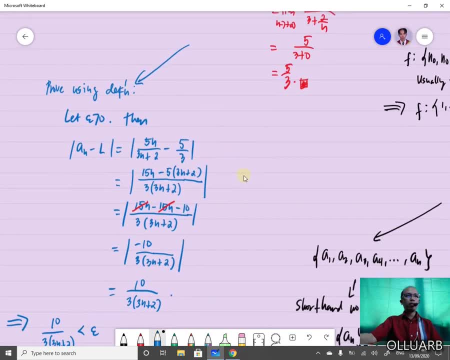 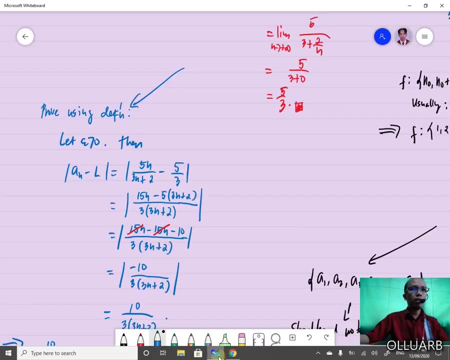 mean. so let's try to analyze that using the a graph. so, using a graph. so if you have this one uh, notice that our function is a sequence is 5n over 3 and plus 2, but we have to replace it by x, uh, and then imagine that there's a uh, the, the, the graph is is, is only a dot. okay, it's just a dot. 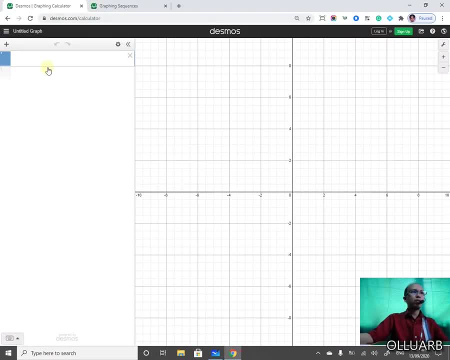 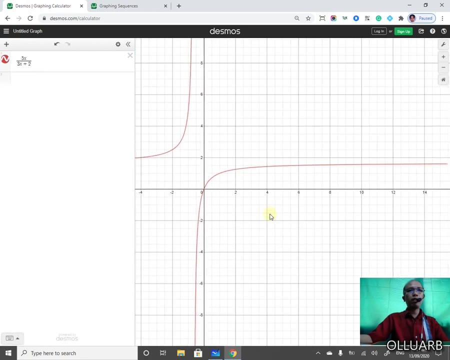 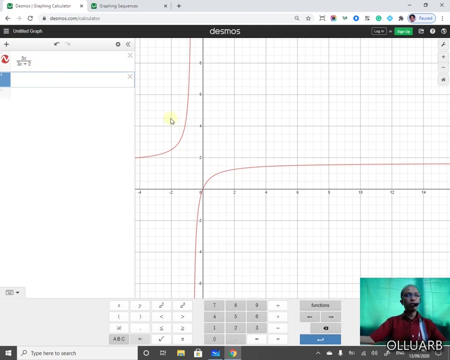 okay, so 5x over 3x plus 2.. so let's try to graph that: 5x over, uh, 3 x plus 2, okay, so this is the graph of the. this is the graph of the equation. uh, the the function. okay, and notice that the limit is. 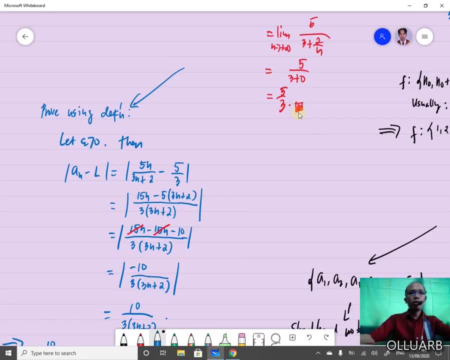 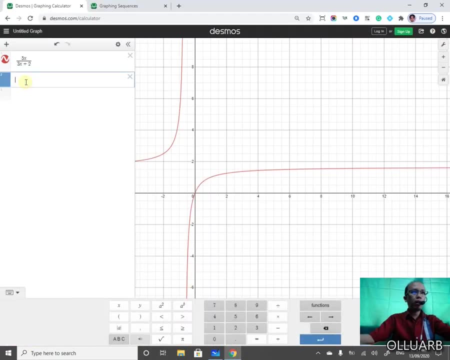 5 over 3. the limit is 5 over 3, is 5 over 3, so, as you can see here. so let's try to show if the limit is really 5 over 3 as n approaches to infinity, so let's try. i'm sorry, uh is equal to 5 over 3, okay, so enter, let's, let's uh. 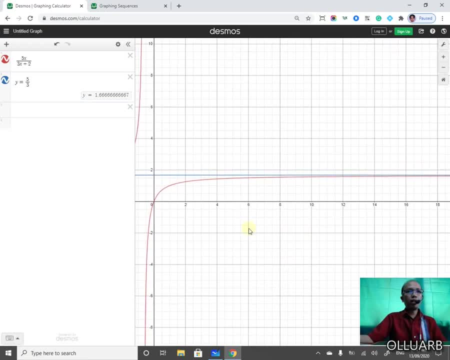 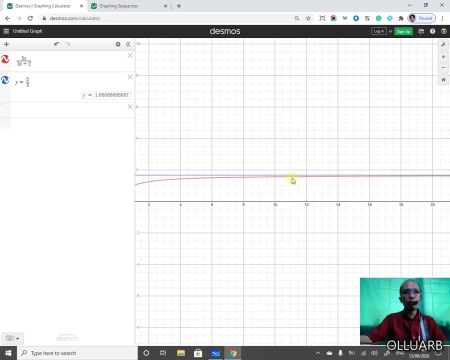 hit the function, enter, and then, as you'll notice, here in the graph you have one, two, three, as n approaches to infinity here. as you can see, here the graph never touches uh to. the line y is equal to 5 over 3. so it's clearly: if you extend that one it never touches. 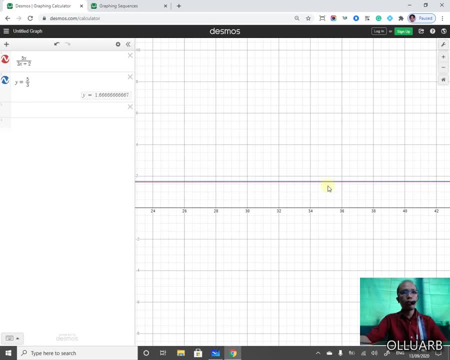 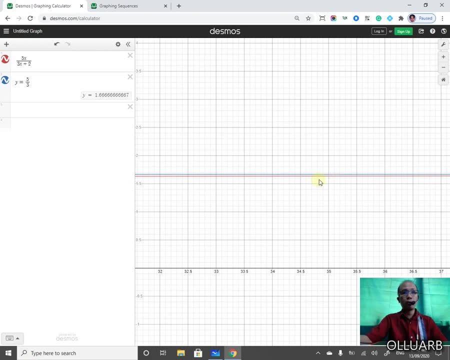 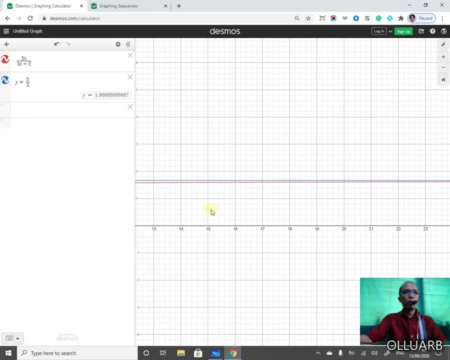 even if you expand, if you expand, that, if you expand, as you can see, it never touches to the line y is equal to 5 over 3, so that is why the reason is that the limit is this is 5 over 3. so what does it mean by? 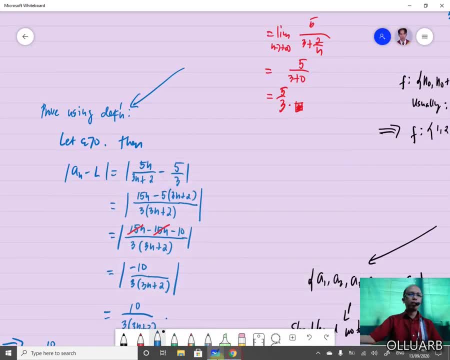 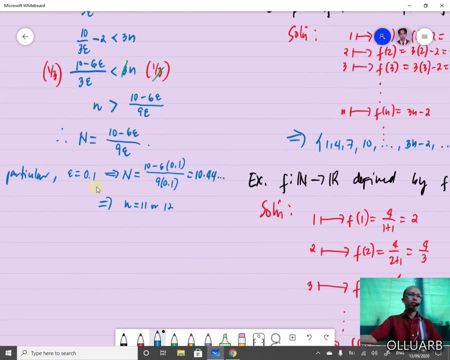 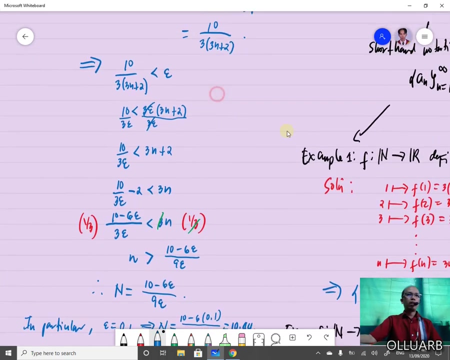 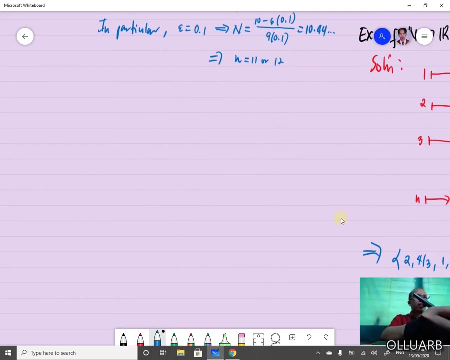 what does this, what does it mean by? by choosing an epsilon which is 0.1 and the value of n is: why is it that? is it uh? is it 11? okay, so i will try to. let's try to analyze that one. notice that uh illustration uh, further, further, uh, let's. 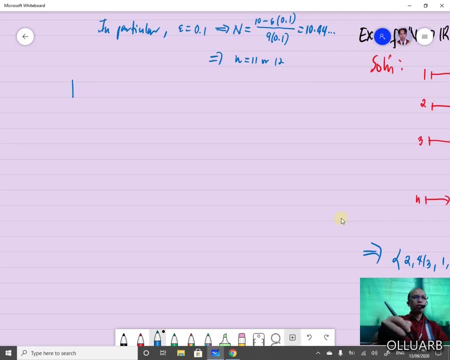 let's try another color. let's say red. okay, uh, further, uh, explanation, explanation: okay, notice that this is uh familiar in definition number two: okay, uh, in your algebra class, algebra and trigonometric class. this means that this is equal, if you recall, if you recall, uh, if you recall it in 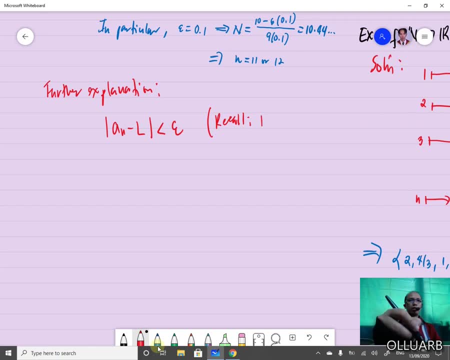 algebra class this uh. we know that absolute value of x, which is less than to a number, a uh is equivalent to negative a less than x, less than a. so i know that you remember this. we will apply this uh, this uh, property of the absolute value, to this inequality. so our x. 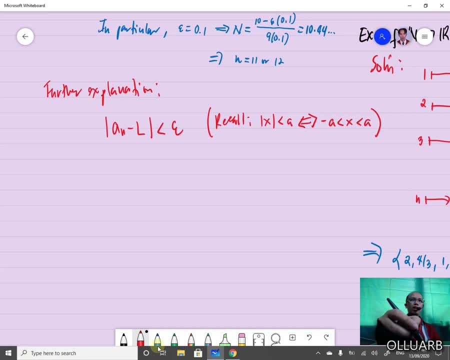 here is a sub n minus l and our a here is epsilon. so this is negative. epsilon less than l. Less than a sub n minus n less than Epsilon. Okay, but this is if we simplify this. this can be expressed as: l minus epsilon less than a sub n less than. 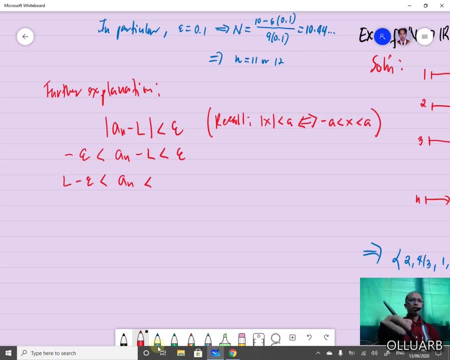 Epsilon No less than l plus epsilon. Okay, so since our l No, let's have a note here That our l is 5 thirds and Our epsilon is 0.1. our big n is 10, point 44- and Our small n is. it will start from 10- 11. 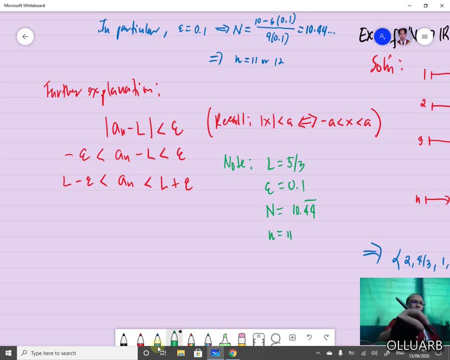 Okay. So if you substitute all these values, example 5 thirds is 5, thirds is 1 point, 1 point 6, 6, 7. so let's try to truncate that one: 1 point 6, 6, 7 minus 0.1, less than a sub n. 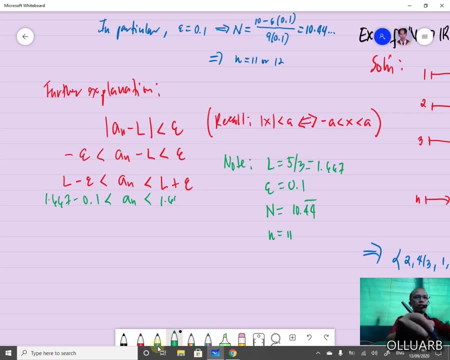 less than 1 point 6, 6, 7 plus 0 point 1, this is equal to: On the right side we have one point seven, six, seven, and on the left side, this is one point five, six, seven. Okay, so if you will try to make a table, 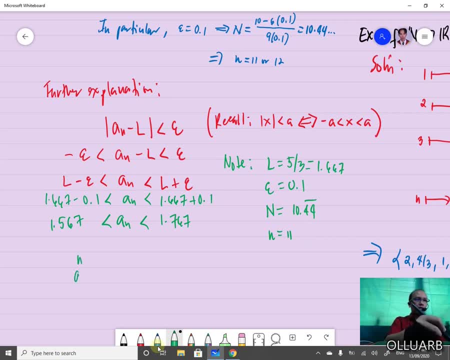 Okay, so this is your n and this is your a sub. n. Okay, sample that one. Okay, It's one. two, three, four, Five. so this is one. then if you substitute our our a sub and note that our a sub, and where should I put this? 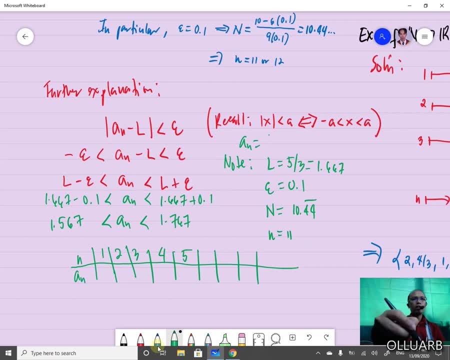 This one, a sub n, is three, five n over three, n plus two. Notice that our n, if you substitute n, is equal to one to this. see today's equation of the sequence. We have five times one over three times one plus two. This is one. if n is equal to two, you will have: 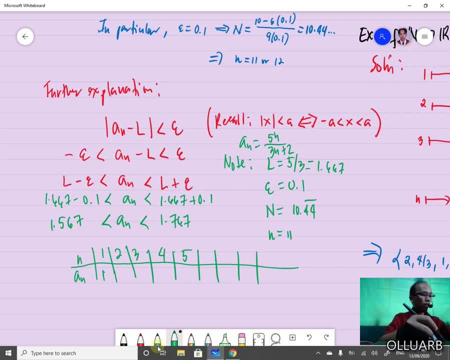 one point. I Already, I I think all this one. so this, This is five over four, or this is one point twenty five. If n is equal to three, this is one point three. six, three, four is one point four, three, and so on and so forth. as you have notice, if your, 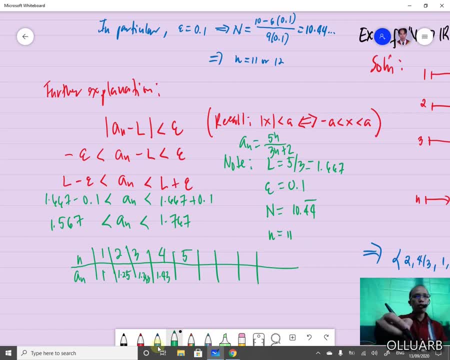 Epsilon is point zero one and you? this means that your big n is ten point forty four. notice that when N is equal to one, two, three, the values, This D, the value of a sub n, will not satisfy this in equality. Okay, so we know that. one point five. 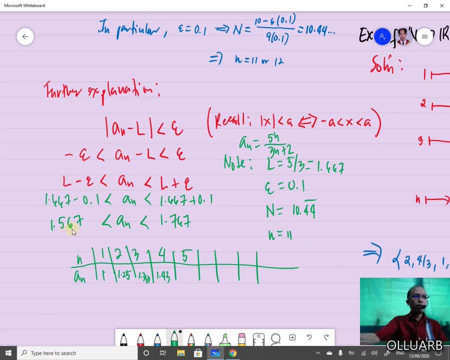 We know that this one one point, five, six, seven is not less than one, But through in the other side, okay, so meaning to say for all values of n, from 1 up to 10. okay, sample, if you have here, um, if you have 10 here, then the. 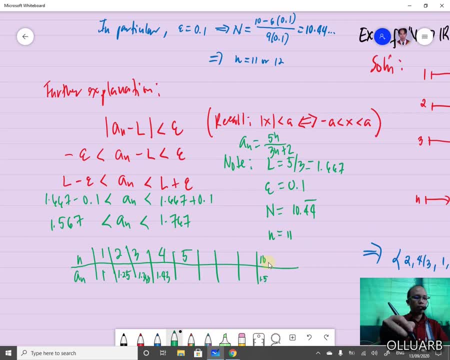 value is 1.5625. again, as you have noticed, 1.625 is not greater than 1.567, but less than 1.767. okay, if your n is 11, then the value of uh, a sub n, is 1.571. okay, 1.571, and, as you have noticed, 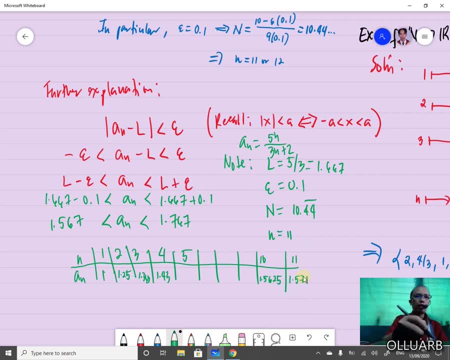 if this, if our n is 11, then this statement, okay, this statement here is true onwards for all values of n greater than or equal to 11. okay, for epsilon is 0.7. for for epsilon which is equal to 0.1. okay, so what does it mean? if you look at the graph? okay, if you look at the graph. 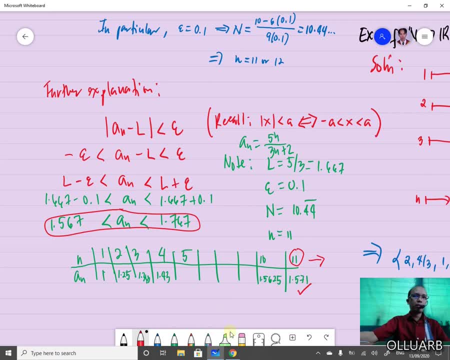 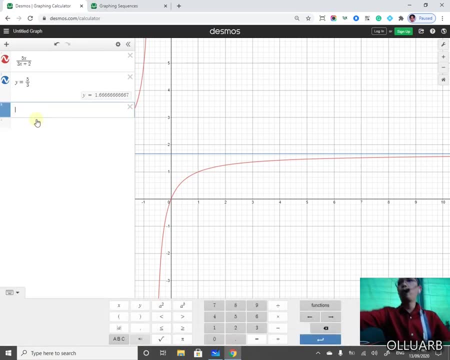 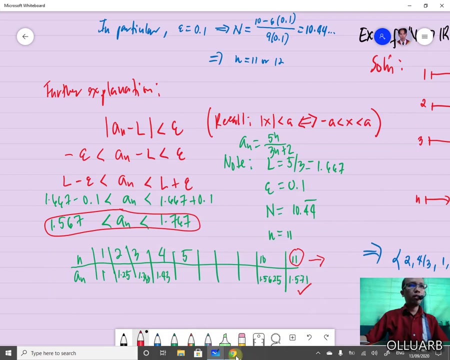 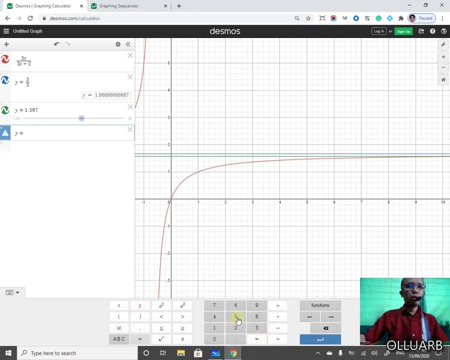 so again. so so this value 1.567 and 1.767. so if you try to substitute that one, 1.567, so if your Y is yy, y is equal to one point five, six, seven. okay, that's the green one and also enter. if your another is one point seven, six, seven, Y is equal to seven. 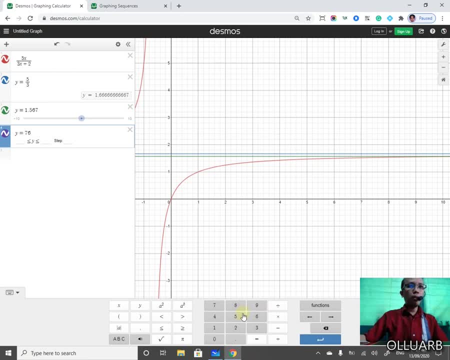 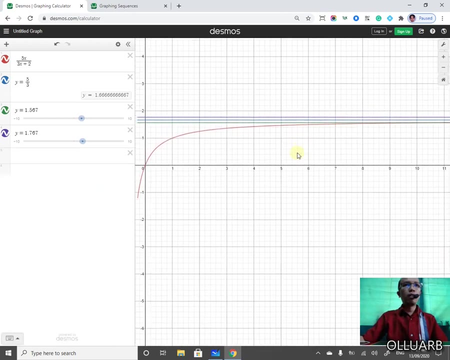 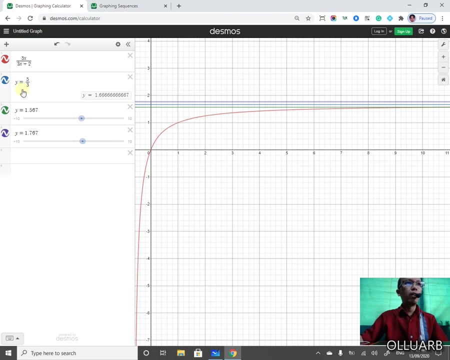 sixteen, no, no, no, no, no, one point back. one point seven, six, seven, okay, enter, hit, enter and, as you have notice here, as you have noticed, forget the, the blue one, I don't know the blue one, but consider on the green one, this one green green one, and 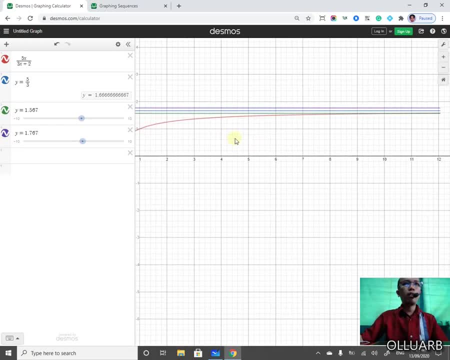 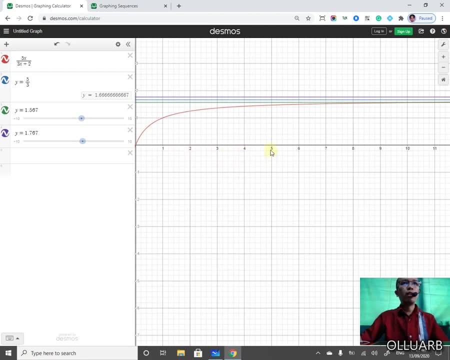 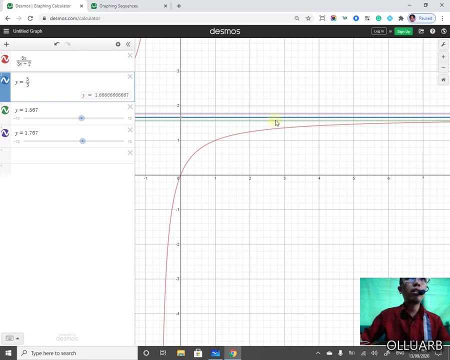 the violet one line, the light that line, as you have noticed, when it's got one to one, two, three, four, it is outside of the tube. okay, consider this, this, this one, this one here, that one, this is a tube. okay, then, these points here, this point here, these points here are outside of the tube. when epsilon is point one, 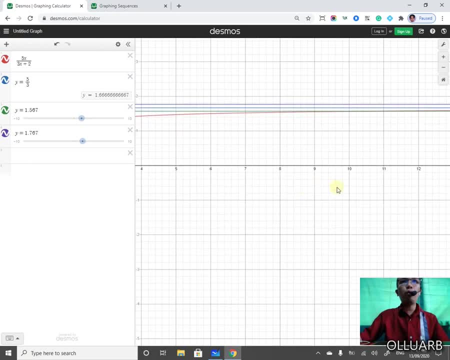 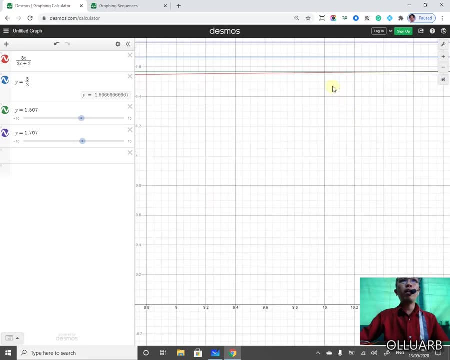 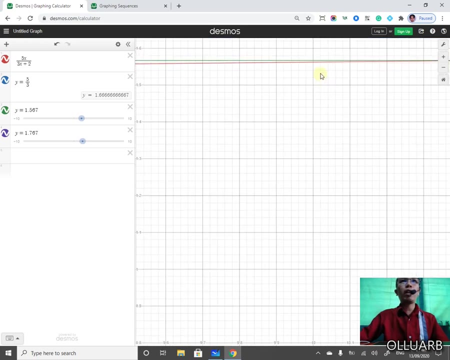 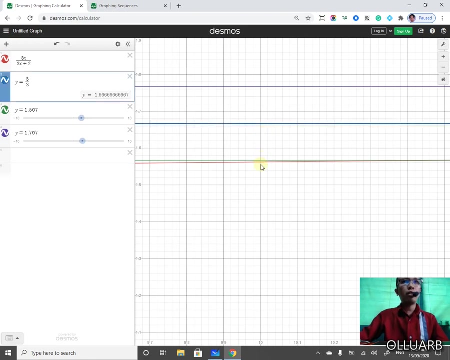 however, if you go up to, let's say, 10, and it's called to 10, let's zoom in. if you zoom in again, the value of n, which is equal to 10, is also outside notice. it is outside of the the tube. the tube from this one, blue one and the green one, it's. 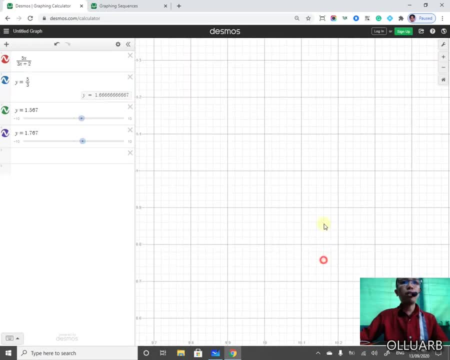 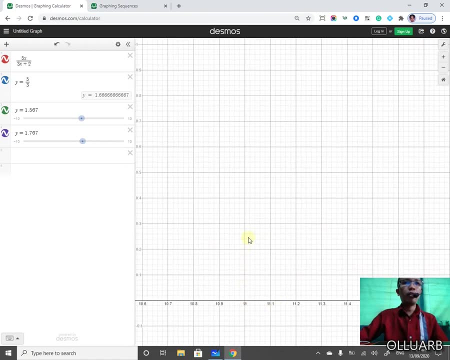 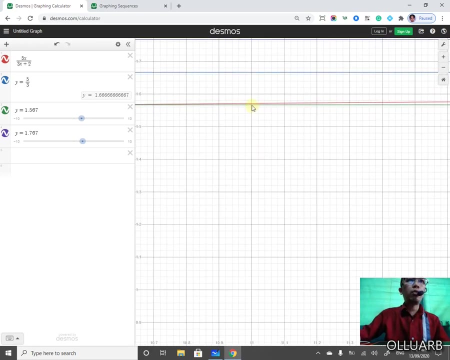 outside, but if it is what they call this one, if you look at 11, this one, 11, 11. okay, look at 11. this is 11. notice that it is inside the tube, inside at, or for all and up to. can you see the the vertical difference? red color, red color here. this is the graph of the this. 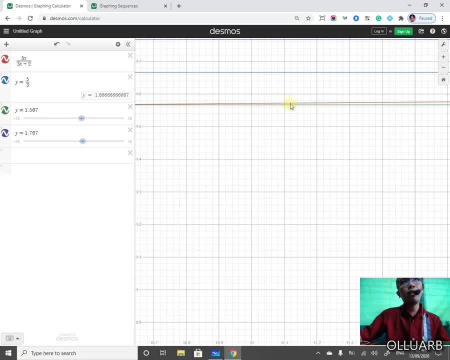 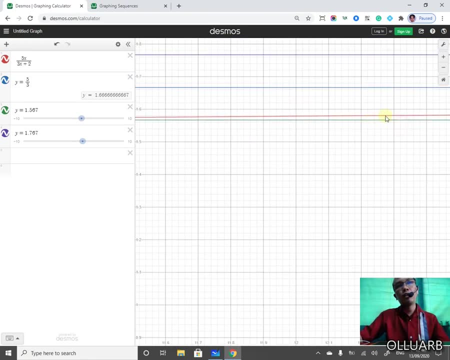 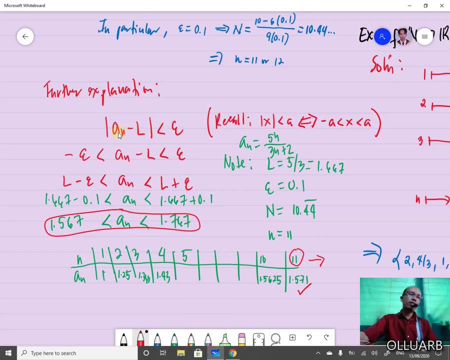 is the graph of the sequence: five e over 3n plus 2. okay, it is inside all throughout up to infinity. that is the meaning of the this one. the distance between the function values and with the difference between the function values and its limit is less than epsilon. 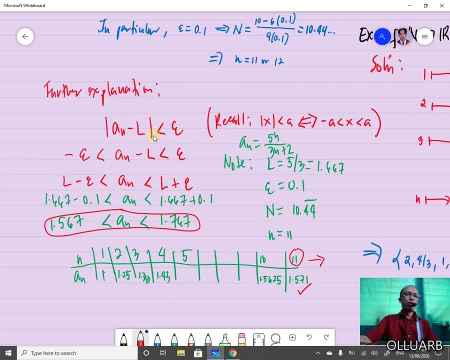 that's the meaning of it. okay, so that's the reason. if you look at the definition 2, that is the mainly the explanation. why is it that if the limit is correct, then you don't have a problem in the graph, but if your limit is not? 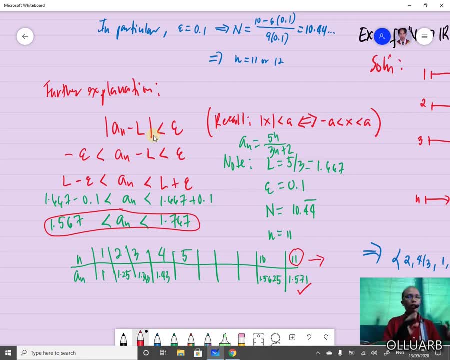 correct if the limit does not exist and you cannot find, I give the value. a big end: there is. it says there there is exists a number in big, in a number in vish greater than zero, which is not necessarily a positive norm, a positive integer, but it is a positive number okay. 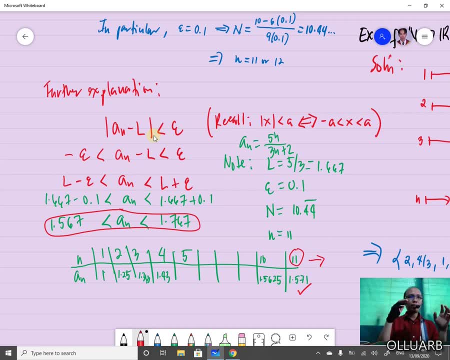 so that's I've missed in in the previous video, so that. so I have to insert this, to be careful that you have to analyze this all throughout, because this: you are a mathematics student, okay, you are a B A math student. if you are a physics student, you are a chemistry student or engineering student, then 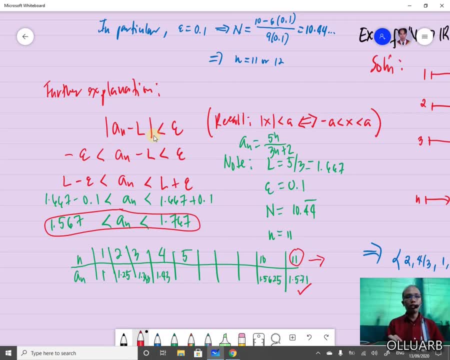 you have to analyze these uh things, okay, so i hope you understand this. if, if, if you did not, then repeat it again, again, again, again, until you understand, and then uh, do not focus on the on, on the on, this uh in this example, but you have to uh make another example. try it to uh with another. 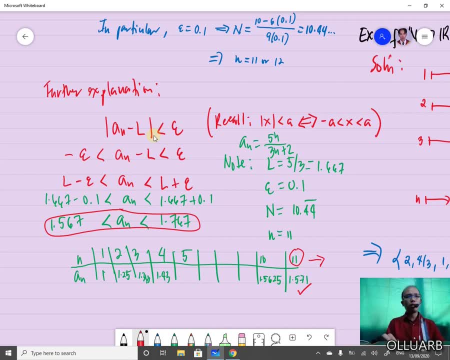 epsilon or another example. uh, then you will find that definition, that the definition of the, of the limit uh will will works if, yeah, if all will uh takes in in place, of course, okay, so i hope you enjoy learning. thank you so much for uh watching this. i'm going to insert this one to 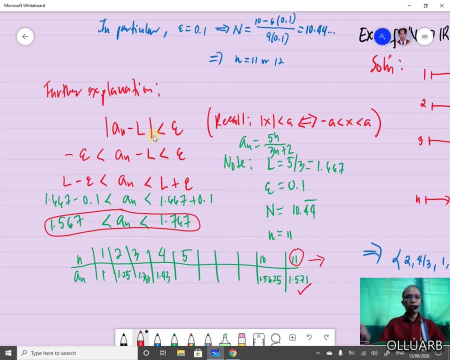 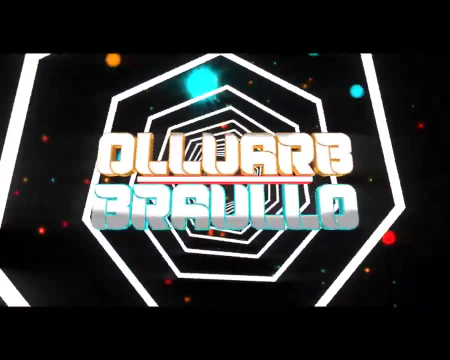 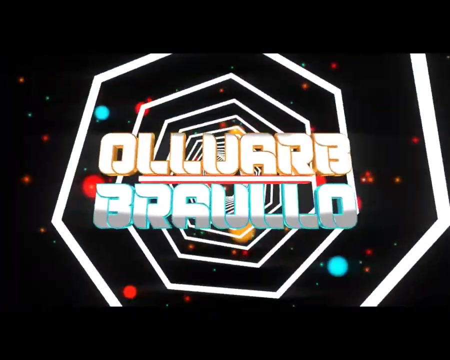 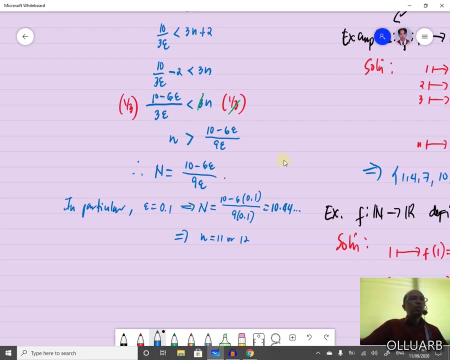 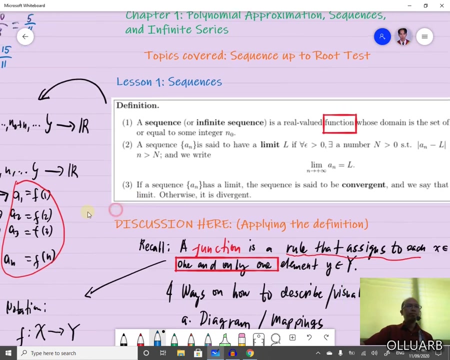 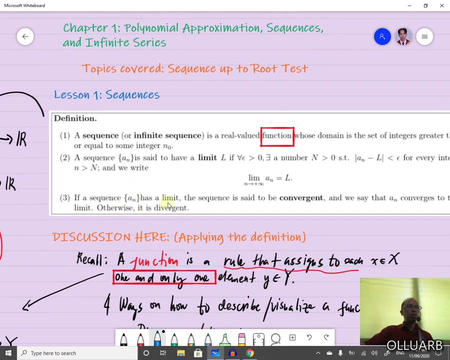 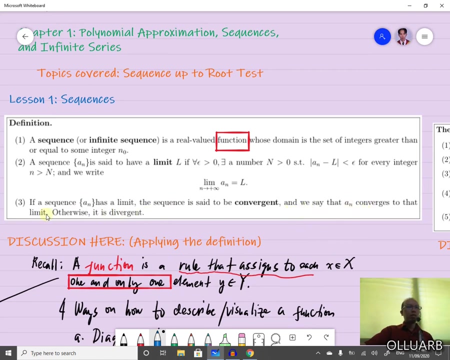 our uh, with, uh, our series of of videos. okay, god bless everyone. okay, god bless you. so that's uh, definition number two. okay, for definition number three. if a sequence, a sub n, has a limit, the sequence is said to be convergent and we say that a sub n converges to that limit. otherwise, 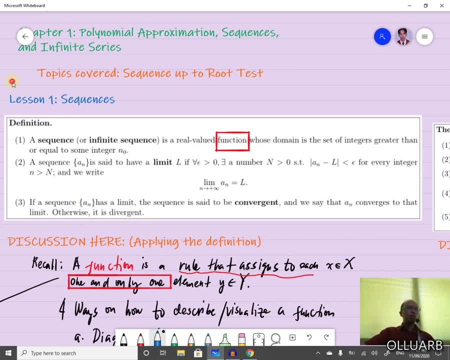 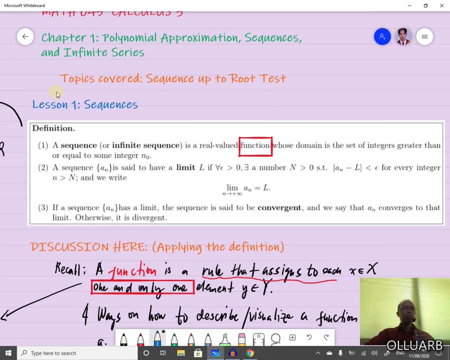 it is divergent. so, as you can see in the definition, if the sequence has a limit, then that sequence is said to be convergent, but if doesn't have a limit then the sequence is divergent. okay, that's very easy. it's file. it follows from the definition number two. 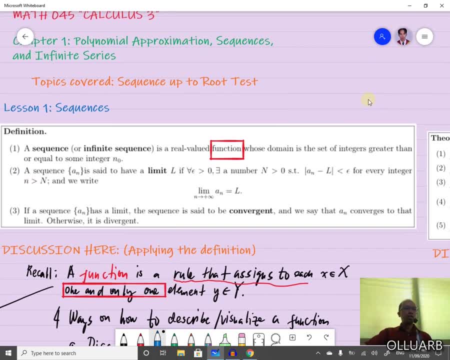 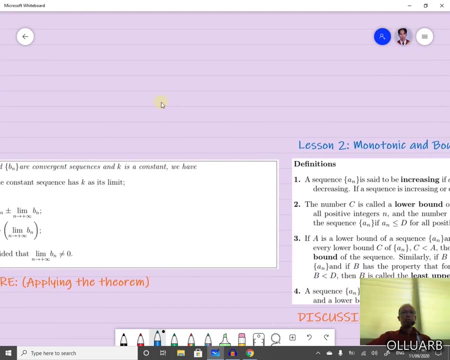 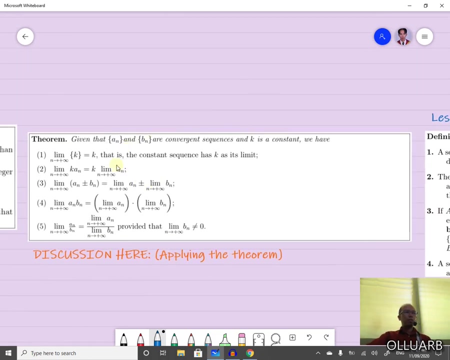 okay, so for our second lesson. that's all for today. uh, for for this. uh, lesson lesson one. uh, for the second lesson, we will be talking about monotonic in this one, monotonic and bounded sequences. but before that, if you remember this theorem, this is true also in your calculus. one subject: the limit of a constant. 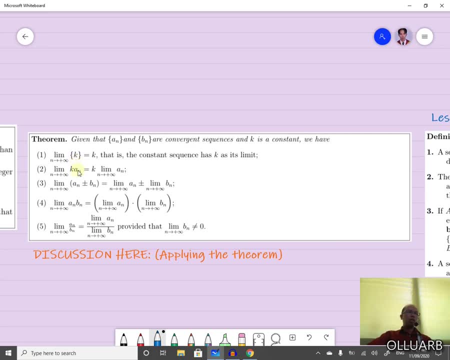 is a constant. sequence is a constant, the limit of the constant times. the sequence is: you can factor out the constant from that sequence- the limit of a sum and difference, you can distribute as you can see here. you can distribute. the limit of a product is the same. the limit of a quotient is the same as in calculus 1. 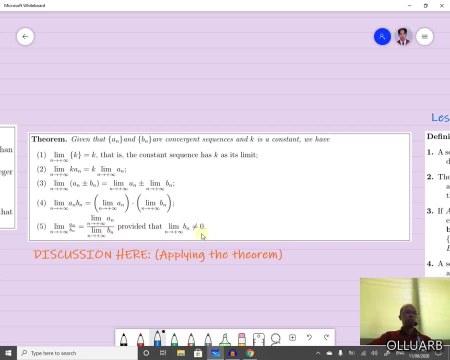 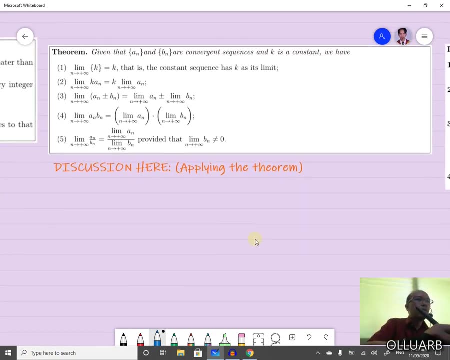 provided that the denominator must not be equal to 0. so, for example, let's have an example, sample number 1: you have the limit of a constant. let's say if you have a sequence, which is this one, okay, I mean to say if you will try to explain. 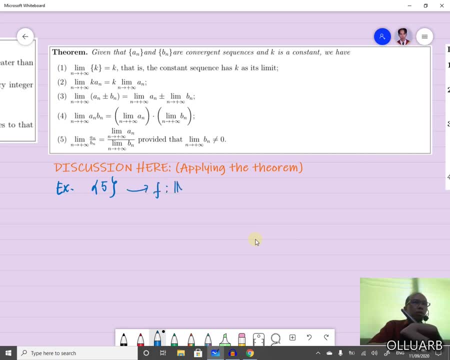 this is our sequence example. it starts from: n is equal to 1, so we need to say: 1 is map to 5, 2 is map to 5, 3 is map to 5. so this is our a1, a2, a3 and so on and up to. 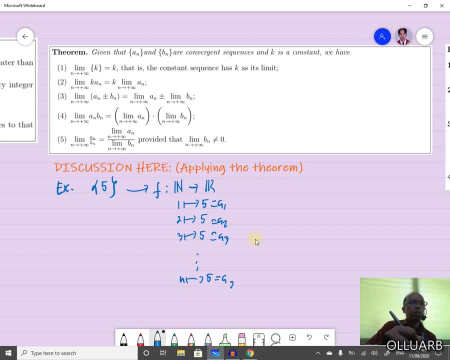 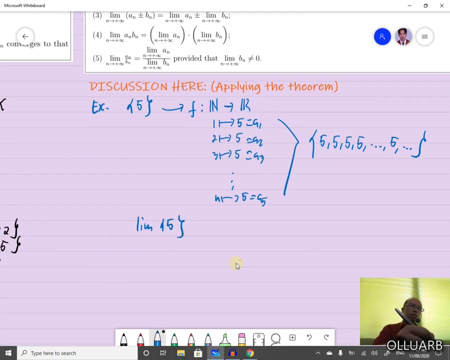 5. this is so then. so this is 5. so we need to say this is: this sequence is denoted as 5, 5, 5, 5, sorry, okay. so the limit of this sequence, the limit of the sequence we will have to equalize, so this: 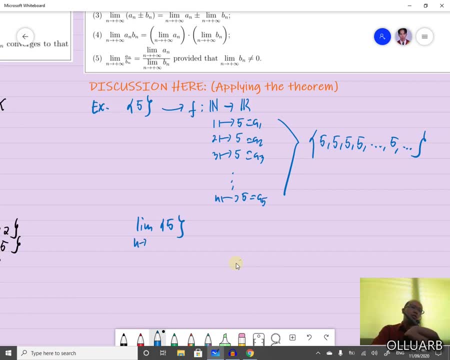 is as n approaches to Infinity. I'm sorry, this is. I think this is No. let's erase this one and limit Trans Над Él kriegen. think tgr me about pa- is 5, 3, 4 e truq e r-. 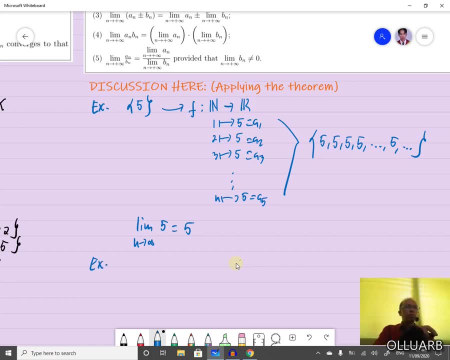 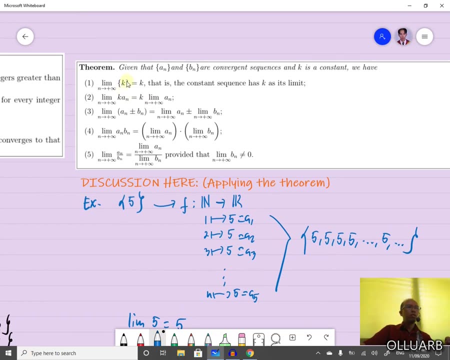 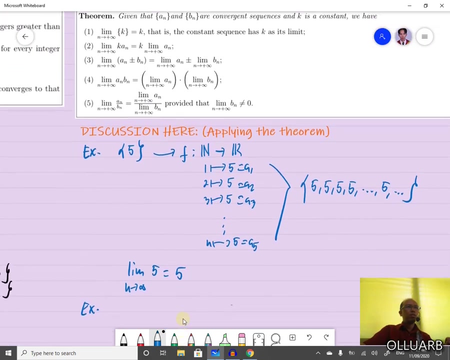 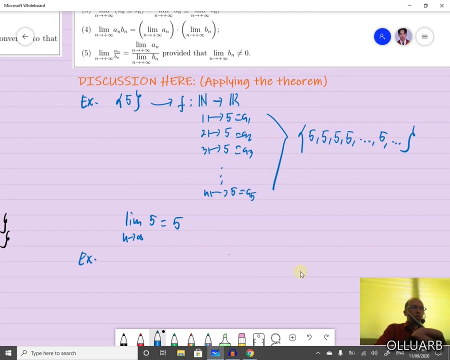 vi- I don't see but lead al- another example. I'm sorry, I think this notation is. I say yes, yes, this is correct, our an is fine, ok, so for the second Vm example, if you have the limit of, let's say, 6 and over and past one, 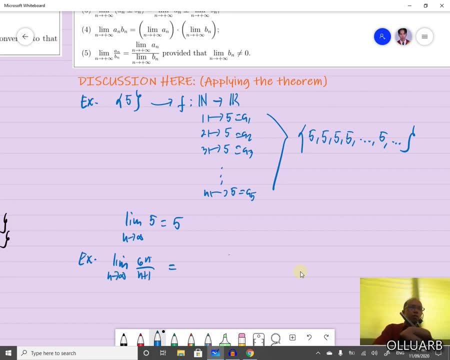 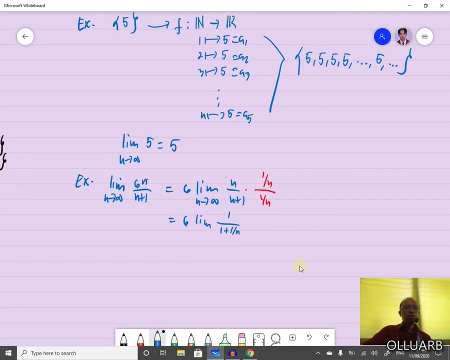 us. an approaches conventionally and buffer out six came over and that's all okay as n approaches to infinity. see we have, we can multiply by 1 over n. so this is 1 plus 1 over 1 over n. sorry, 1 over n. 6. we can evaluate now: this is 1 over 1 plus 0. the answer is 6. 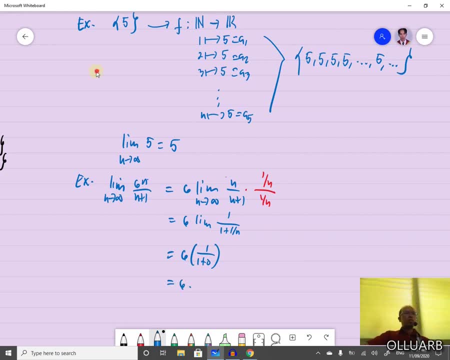 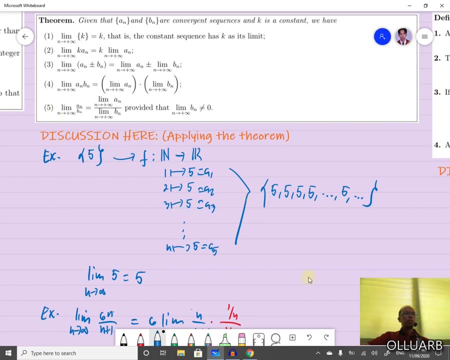 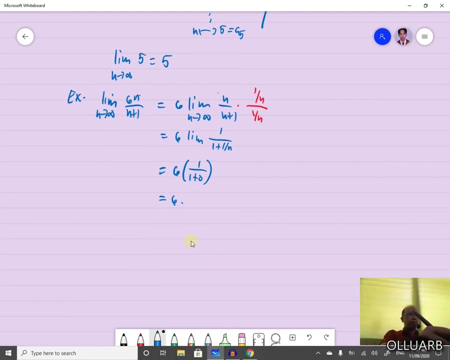 ok, and same is true for number 3, number 4 and so on and so forth. for example, we have this one limit of 3n minus 2. as n approaches to infinity, we can distribute the limit minus the limit of the constant: n approaches to n. notice that this is the answer, this one. 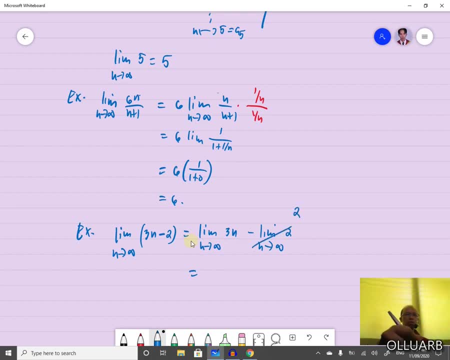 is 2, this is 2, but this one is infinity. so this one, our answer, is infinity minus a number, is infinity. okay, so you will have an answer which is creepy, or maybe it's not, does not exist. it doesn't exist, doesn't you? you don't have an. 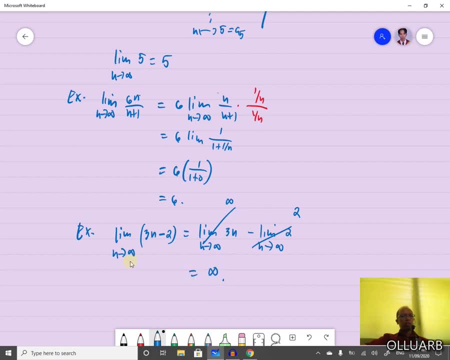 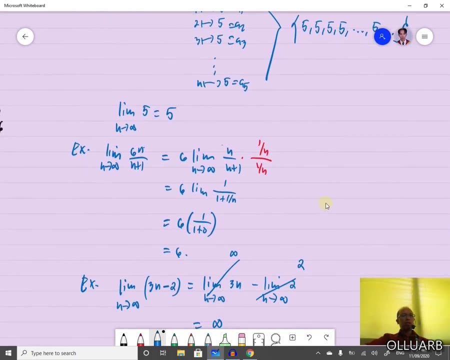 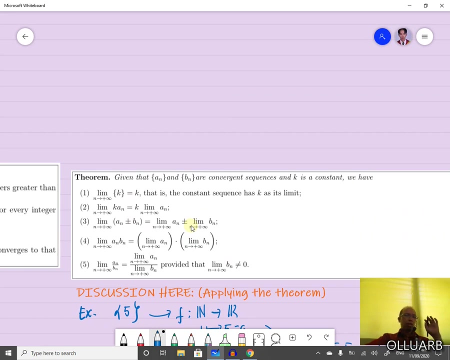 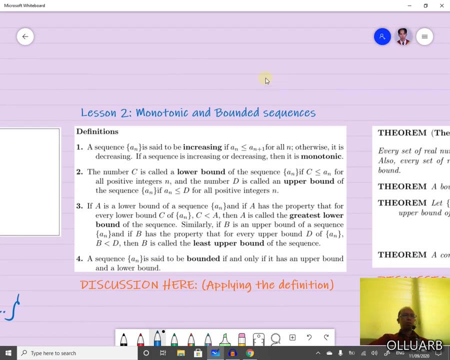 answer does not exist in in limits at infinity topic. okay, so that's how it works. if you have, if you will use this theorem, this is the same as your, your calculus, one subject. so again, don't forget. our next topic will be. you be discussing about monotonic and bounded sequences. okay, God bless. 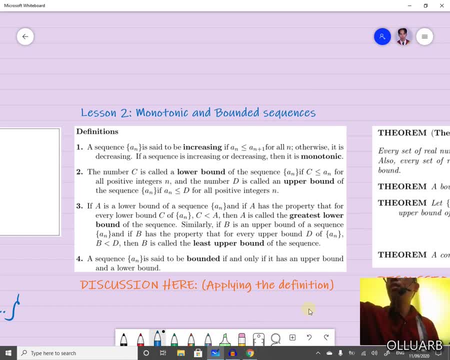 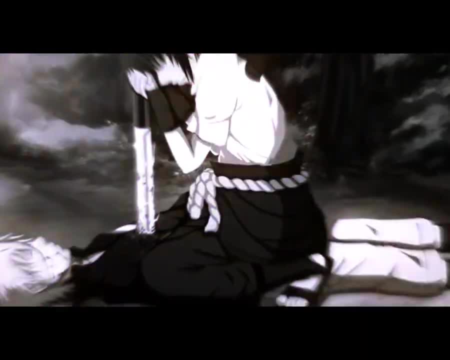 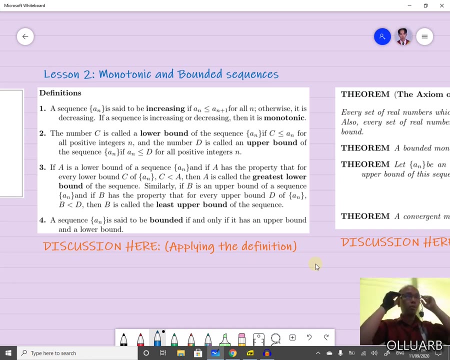 everyone. before we proceed to our lesson number two, which is monotonic, here are勘awia commands, which first two, which are the sampling method, preparation. monotonic and bounded sequences, wind sequence, Caleb. here are勘, finances and bounded sequences. let me have some examples in further examples in lesson number one. okay, so, 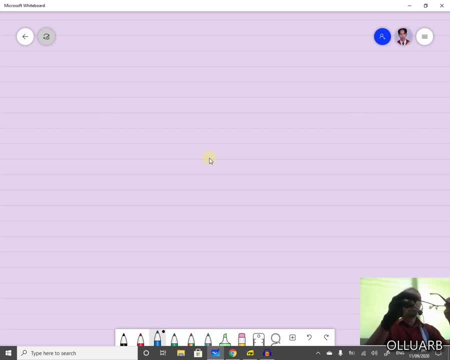 let's create a- sorry, let's create a new whiteboard. now let's have further examples in lesson number one. so example example in lesson one. so for the following problems: determine if the sequence is convergent or divergent. to me say we have to find the 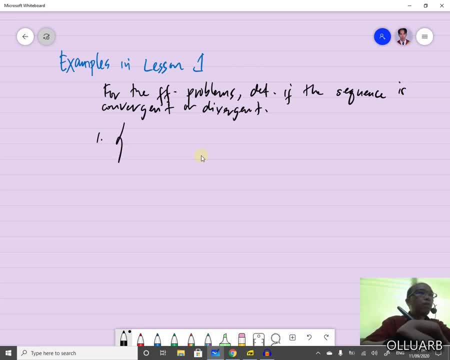 limit. so for problem number one, we have three n squared plus one over two n squared minus n. so let's have a solution. so first is, we will evaluate the limit. copy the problem first. by the way, before I forget again, I made a mistake in the first lesson since. 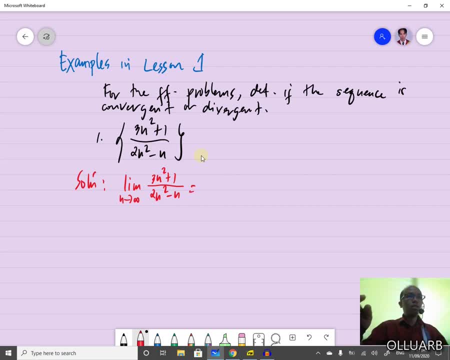 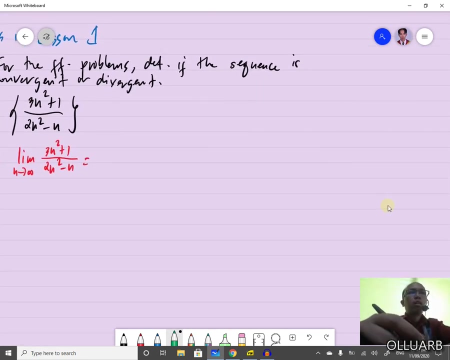 the very lengthy recording. so let me remind you that I made a mistake about the theorem of limits of infinity. so just like this one, this theorem, you remember it, this theorem, if R is a positive, then number one, the limit of 1 over X to the R. as before I write this, I write it. 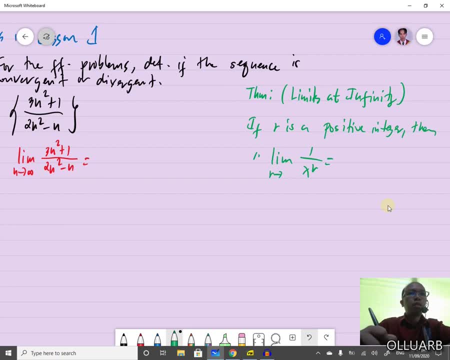 as R approaches to positive infinity. but I made a mistake, I forgot also this is: as X approaches to positive infinity, this is zero. and the same is true for number two, one over X to the R. if our X approaches to negative infinity, it's also zero, anyway that's. I know you are familiar with it. so 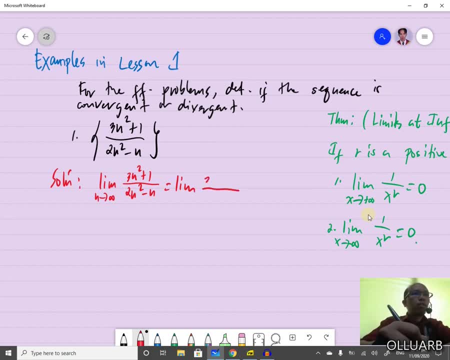 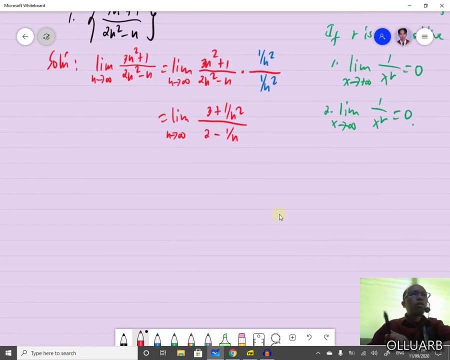 let's continue solving this: 2n squared minus n. so we have to multiply by 1 over n squared as n approaches to positive infinity, and this will become 3 plus 1 over n squared 2. the denominator is 2 minus 1 over n, plus n approaches to infinity. am I right? okay, so. 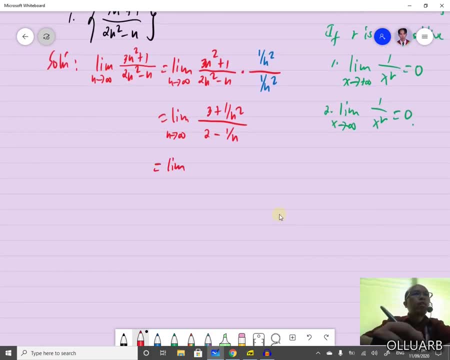 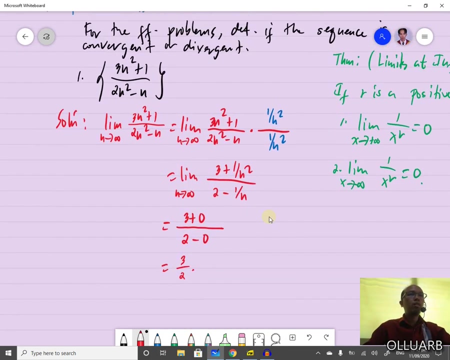 this will become okay. see, we can evaluate now the limit. let's go back. okay, this is 3 plus 0 over 2 minus 0 and this is 3 halves. okay, 3 halves and this one 3 halves. sorry if you will try to grab it in real line, not in a sequence, so you replace this as your X, replace it. 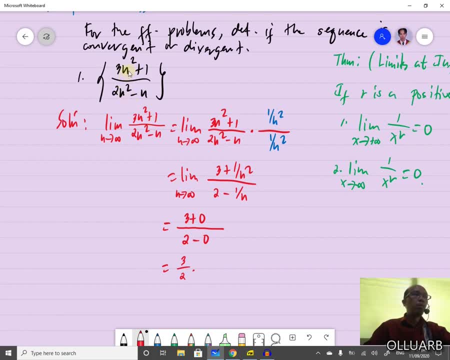 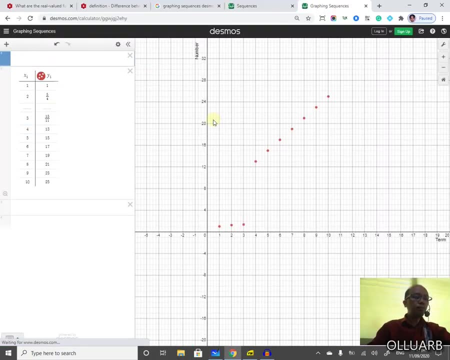 as X, your, your, your n. replace it as X. so let's try to grab this in this most. we have three. sorry shift. we have 3x squared, sorry, X squared, oops, shift. what happened? 3? what happened to all this moves? what happened to all this moves? 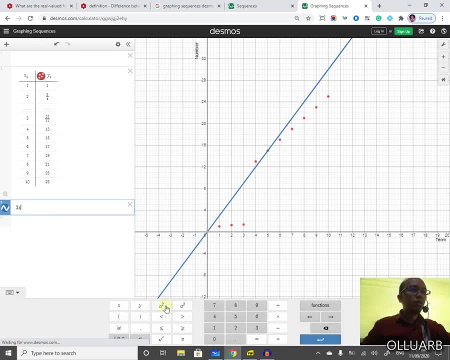 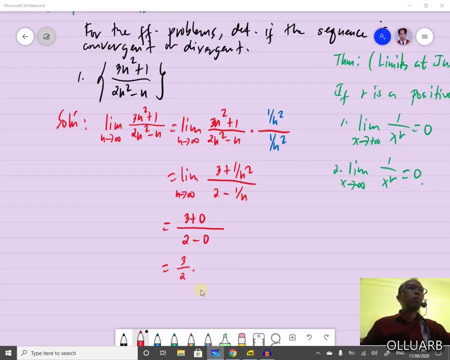 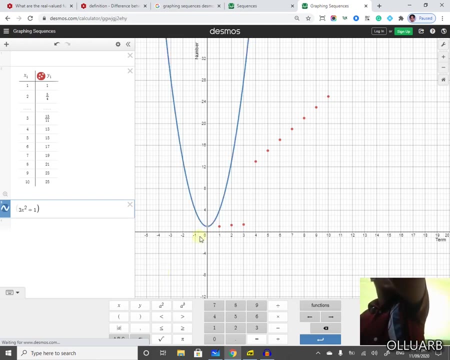 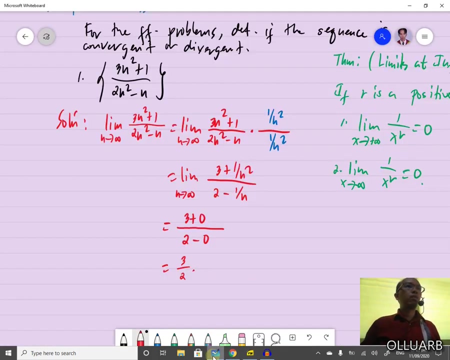 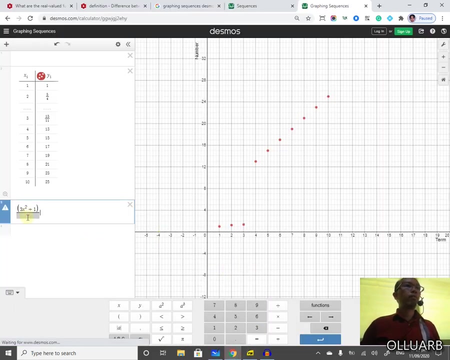 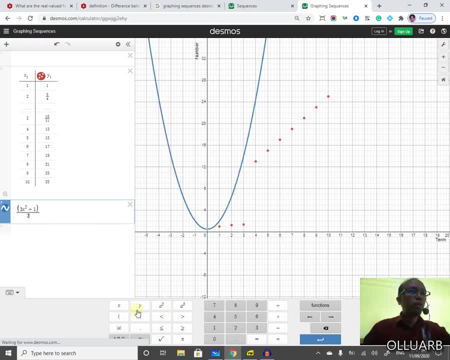 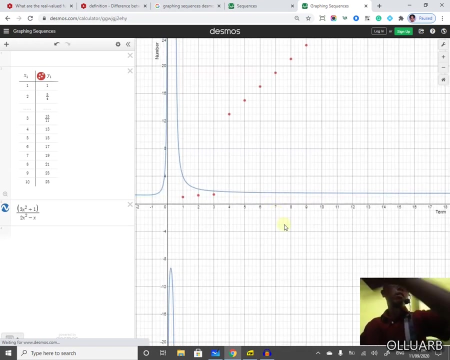 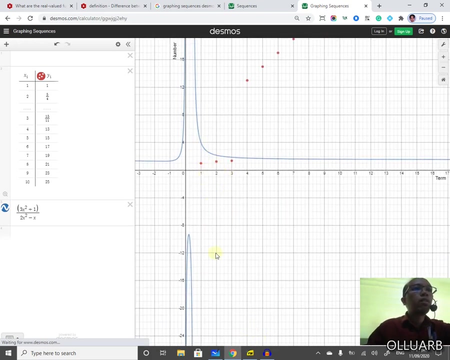 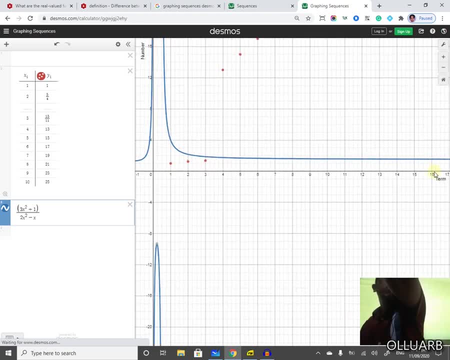 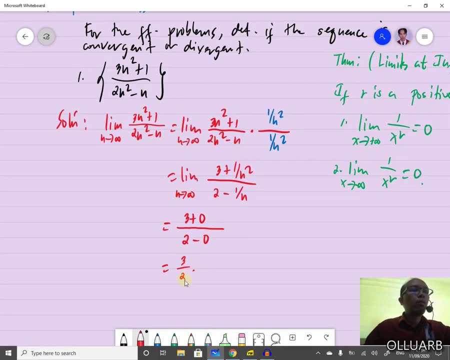 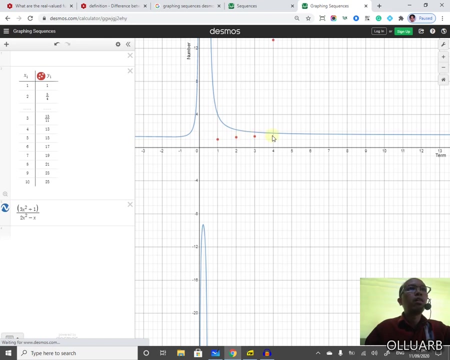 Frederic z anduzu, 3ivas y tenantsингles approaches to what is our limit, 3 and 3 over 2, meaning to say this is 1 and 1 half, 1 and 1 half, so 1 and 1 half. so clearly there is a you notice here graph. 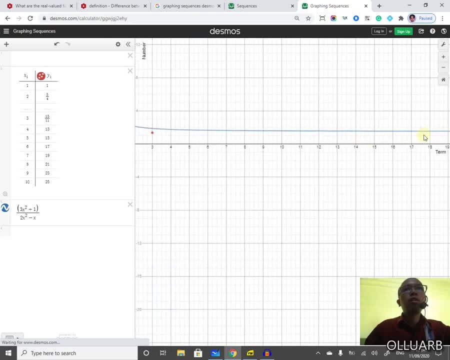 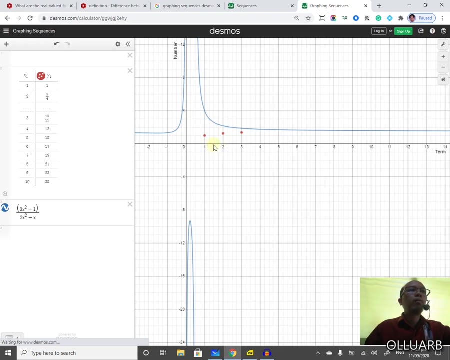 here, as X approaches to infinity, as n approaches to infinity. so we replace our end to be a real number and it's just the same. all you have to do is to not include the points here between 1 and 2. okay, there is. there must be a dot here. 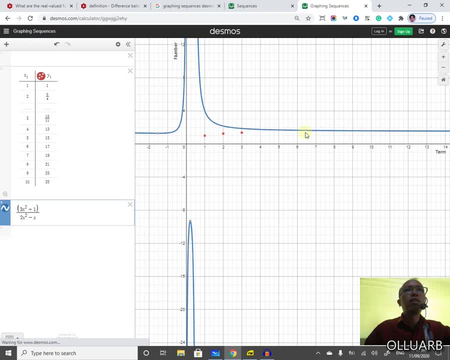 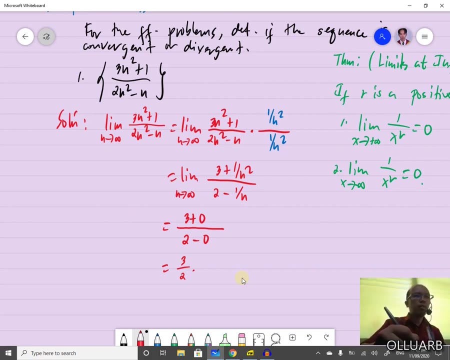 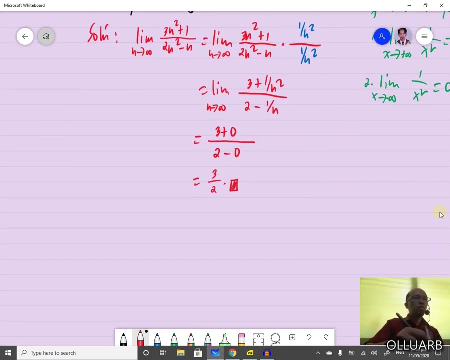 and so on and so forth. okay, there must be a dot there. so, as you have noticed, it approaches to three halves, or one and one half, so it verifies our result. okay, so this is correct for number one. this is correct for number two. let's try number two. we have 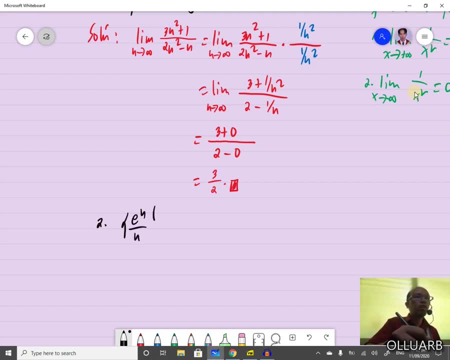 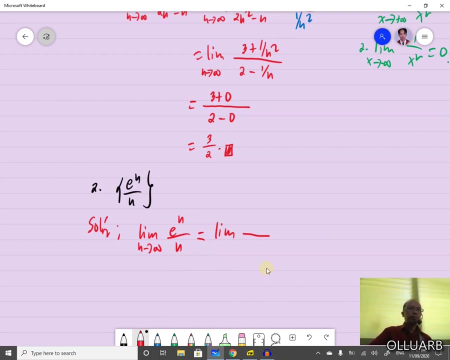 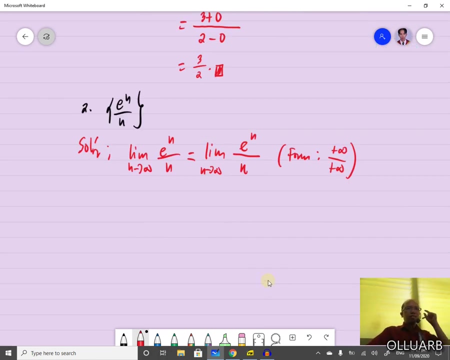 e to the n over n. so solution: give: the limit approaches to infinity. so what is the value of this problem as n approaches to infinity? so notice that this problem is not really as worded, but we know the value of the plane perspective is as the limit of fate is. 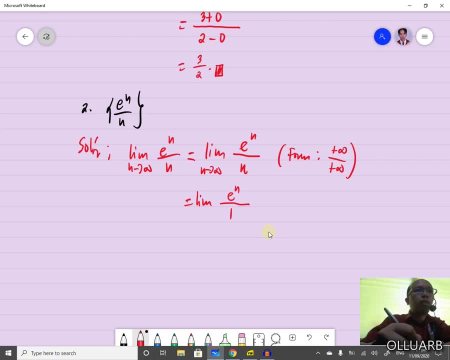 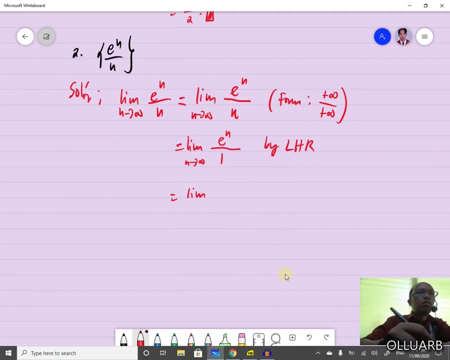 is e to the n over 1 as n approaches to infinity. So this is by LHR, but the limit of e to the x is e to the x, okay. so simplify, as n approaches to infinity and, as you have noticed, we have positive infinity, okay. so if you try to graph, 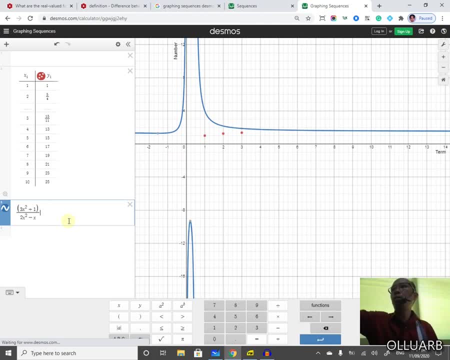 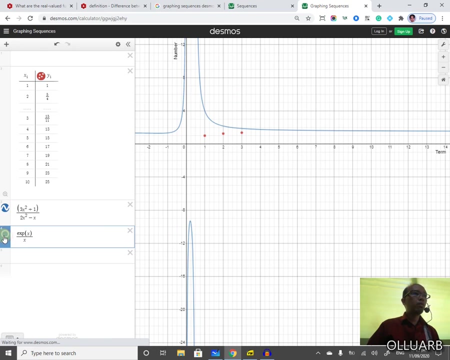 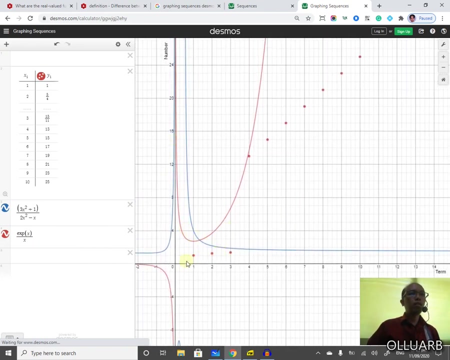 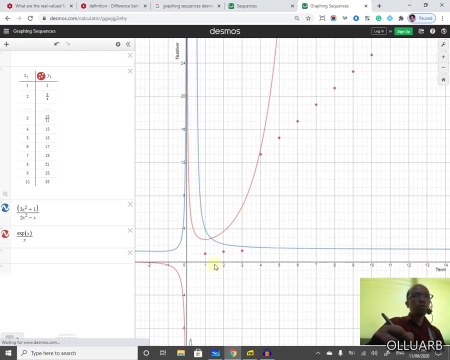 this problem. replace place n by X. where's the exponential, exponential? exponential, this one, sorry. X over divided by X? I think I have to replace the color to. I'm going to replace the color to red, okay, so if you have noticed the red one as X approaches to infinity in this setting, this is clear as X approaches X. 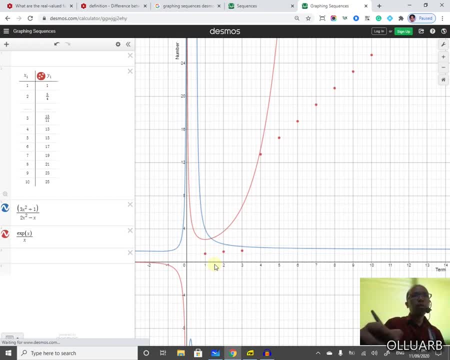 as you end up with infinity 1, 2, 3, 4, 5, up to infinity. the graph, as you have noticed here, x approaches to infinity. two, 0 come back, it's set. so x approaches to infinity. one, two, three, four, five of to infinity de graph. 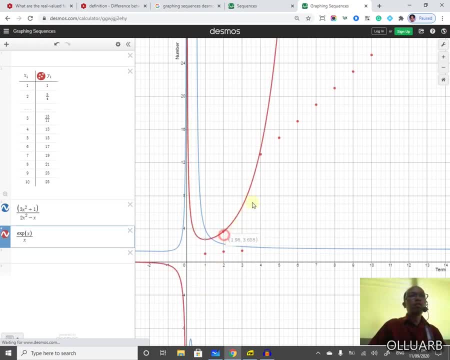 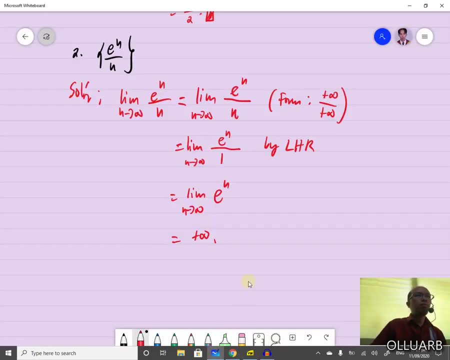 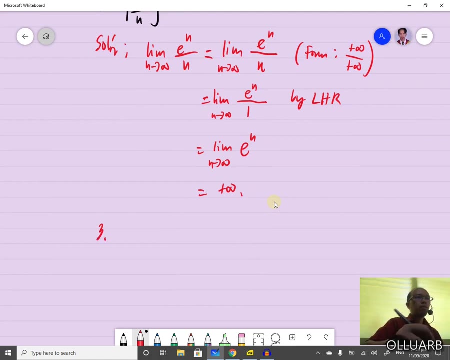 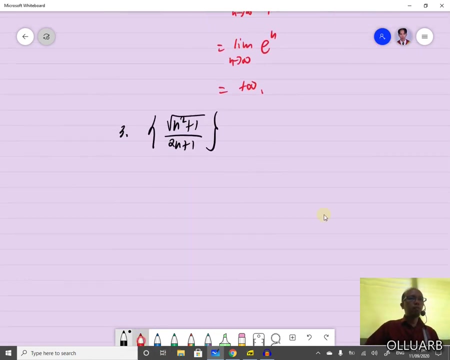 you have noticed here, this one gets bigger and bigger. so the answer is positive: infinity. and that's verifies our result for our third problem. sorry, third problem. our third problem is this: one: what if you are given n squared plus one, two n plus one? so this is our sequence solution. 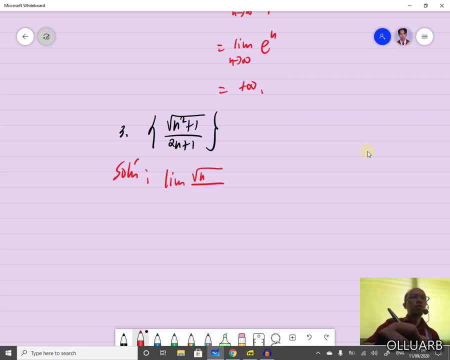 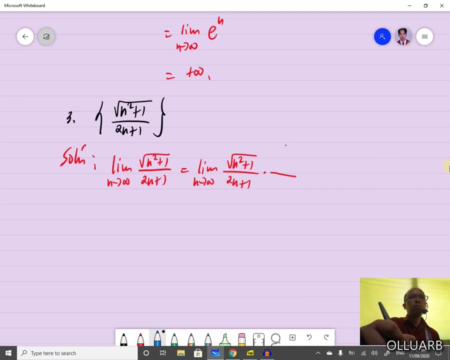 limit. copy the problem first. so what should we multiply both side of this equation? so I guess we are going to multiply one over square root of n squared, one over square root of n squared, so that we can combine the this one and you try to distribute limit of this will become n squared. 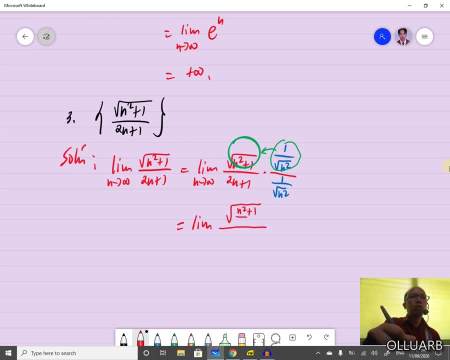 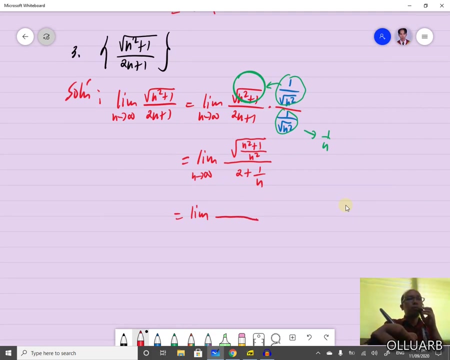 plus one over n, squared in denominator. as you have noticed, this is one over n, since our end approaches two positive infinities. so and approaches to последing p thing, and this is two plus one over n. so further simplify this to the result: this will become square root of 1 plus 1 over n, squared 2 plus. 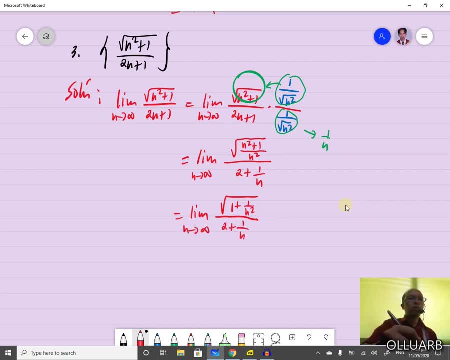 1 over n plus n approaches to infinity and this will become the limit is. you can evaluate now square root of 1 plus 0, 2 plus 7, and this is 1 half. so our answer is 1 half. so let's verify this problem again in a graph. replace n by X. okay, so it must be square root. 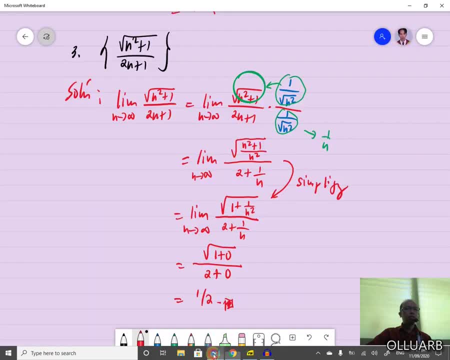 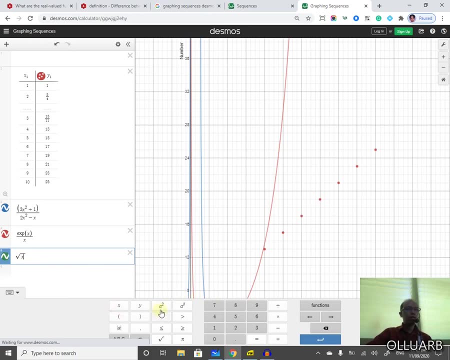 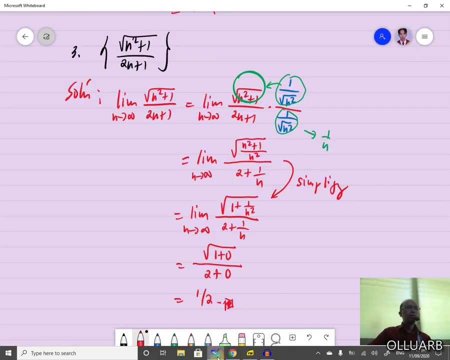 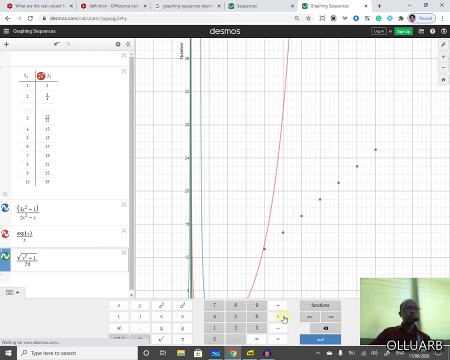 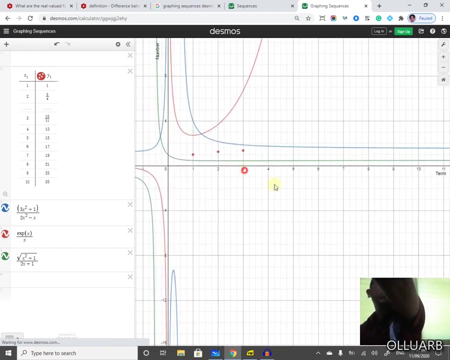 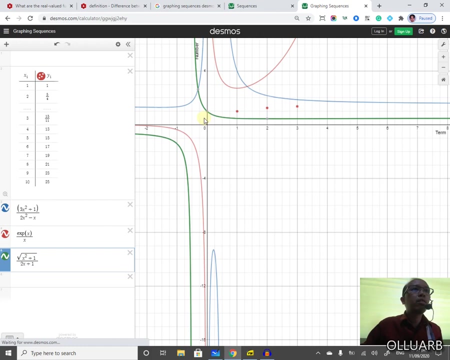 square root of where's that? one X squared plus 1 X squared plus 1, divided by 2x plus 1 to X plus 1, and the color graph is the green one. first the green one, so let's try to zoom. so this is one here, so one half is here and, as you have noticed, as n approaches to, 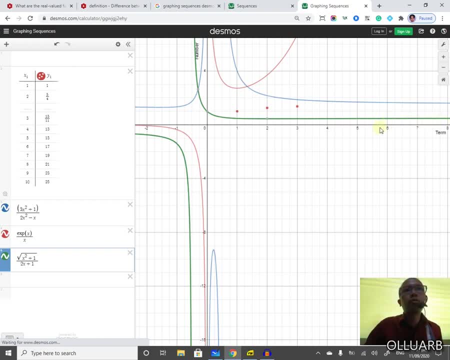 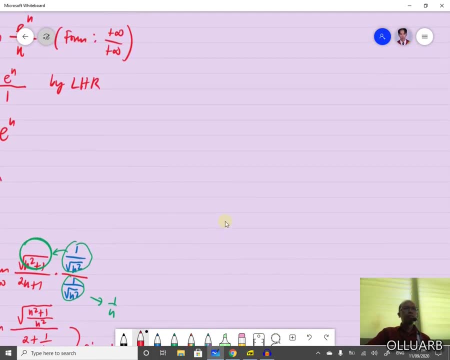 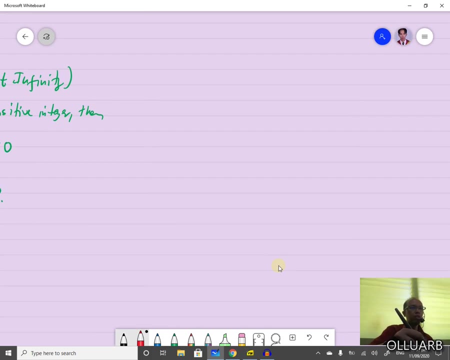 infinity. the limit is clearly one half. okay, so that's verifies our result. so how about number four, the last problem, number four, that's problem. what is the limit of this sequence over to the end? so solution again. get the copy the problem first. this is one plus three over n to the n as n approaches infinity. so how are we going to solve? 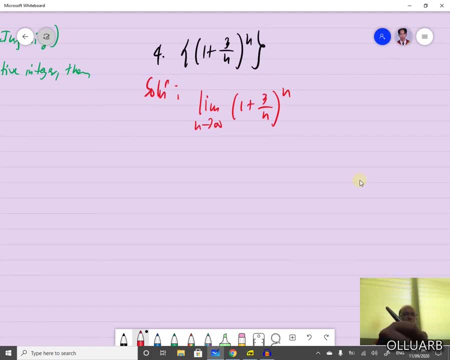 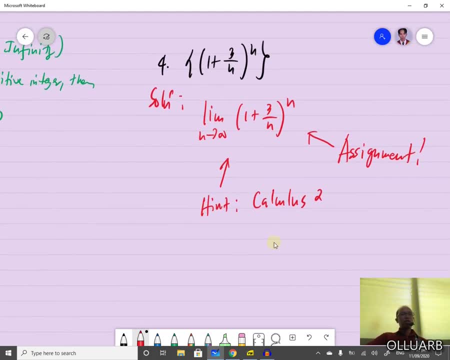 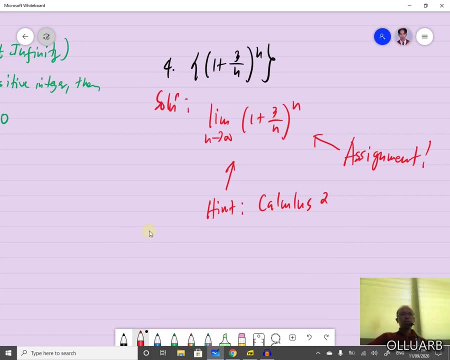 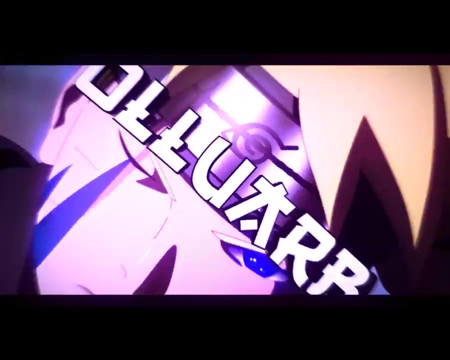 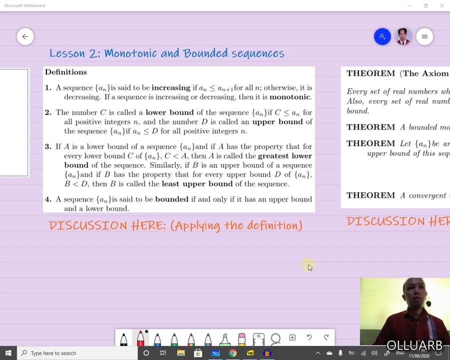 sorry, I forgot. okay, so that's all. thank you so much for listening. now we can proceed to lesson number two, which is all about monotonic and bounded sequences. everyone for our second lesson, which is entitled monotonic and bounded sequences. let me remind you that you have to familiar yourselves about what I told. 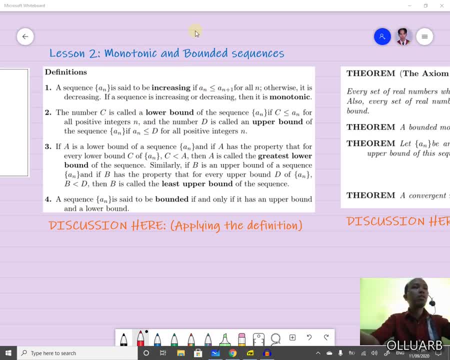 you before in lesson number one about sequence, you have to really try to understand our first topic. so since you are, I assume that you are familiar not with the first part of the lesson, then you have to try to understand our first topic. so, since you are, I assume that you are familiar not. 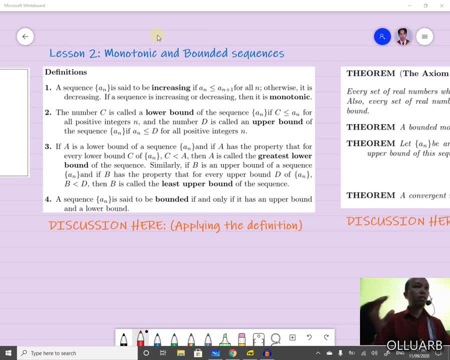 now the idea of a sequence. so let's proceed to lesson number two. okay, definition one. this is all about increasing and decreasing sequence. a sequence, a sub n, is said to be increasing if this condition satisfies for all n. otherwise the sequence is called decreasing. okay, so before we discuss what is monotonic, let me give you 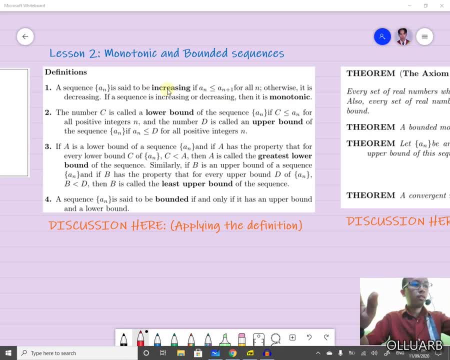 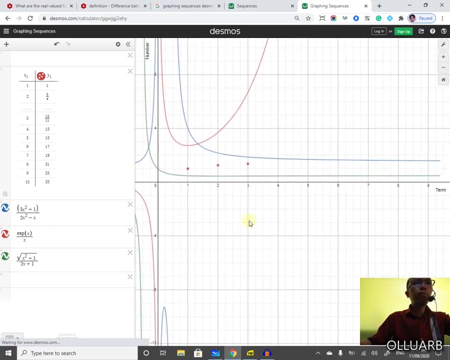 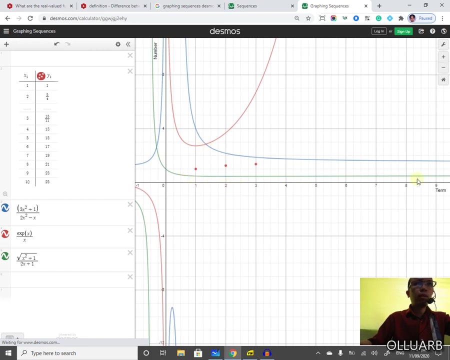 a brief, a simple explanation of about increasing and decreasing function. if you graph the function in the graphing calculator in this moss, as you can see, as if your n is, if your example, if this one is blue, one notice that as this one, as n, approaches to positive infinity, one 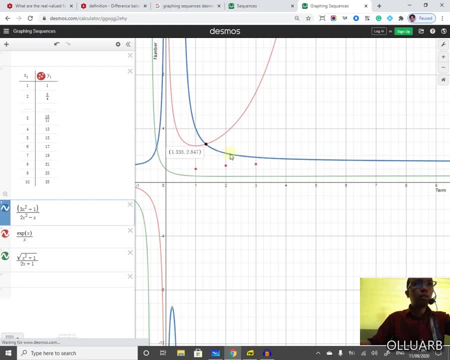 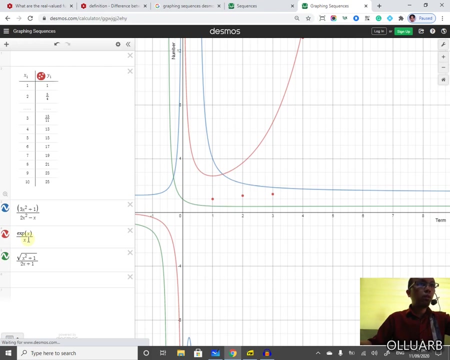 two, three, four. clearly, the graph is decreasing, okay, the things you mean to say. this function is decreasing 3n squared plus 1 over 2x squared minus X. how about the red one? this is an example of a sequence which is an increasing sequence. so you have noticed here, as when n is, 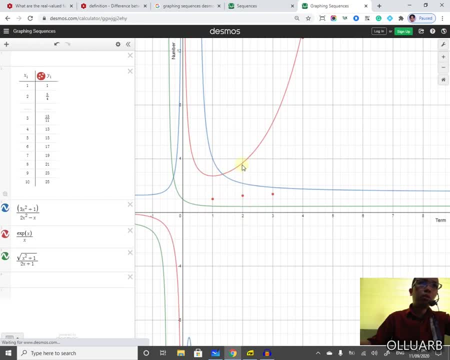 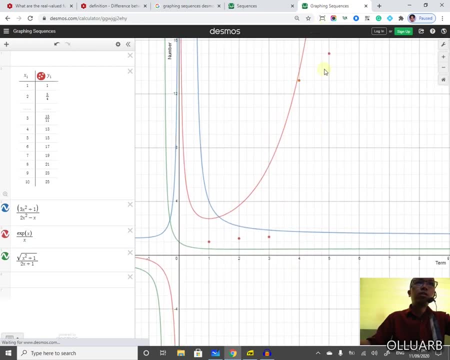 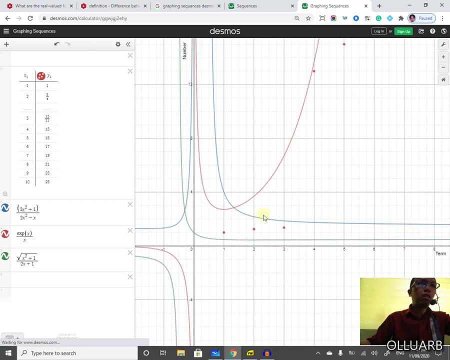 equal to 1, we have a dot here. when n is equal to 2, we have a dot here. n is equal to 3, a dot here, and so on, 4 and so on and so forth. so, as you have noticed, it is increasing. so that's basically the definition comes. how about? 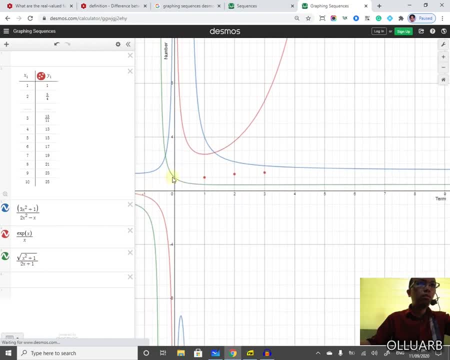 this function, the green one. do not include this one graph here, because our sequence starts from 0, or 1, or 2, and so on, so forth. okay, so for all n. remember that for all n, as n approaches to infinity and, as you can see, approaches to. 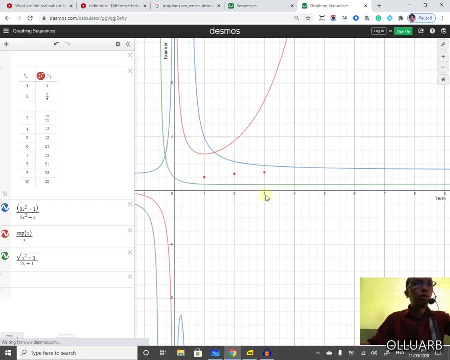 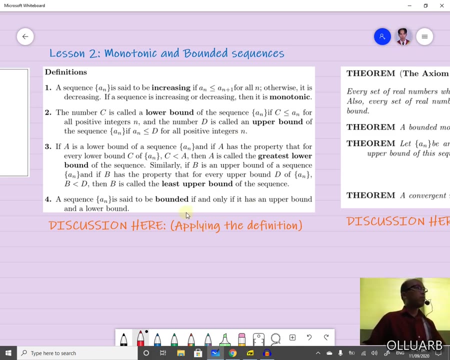 the limit, which is 1 half, just like before the answers before. so this is example of decreasing function sequence. okay, so as an example, very simple example, we have. how about this one? where's my pen? so, example: if you have this sequence: 4 over n plus 1. 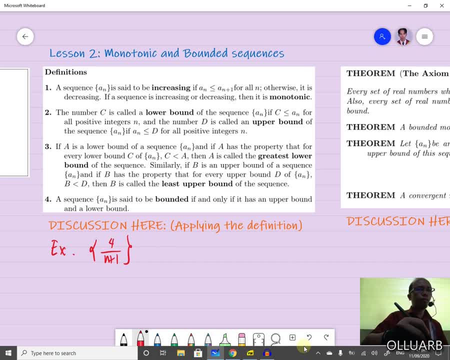 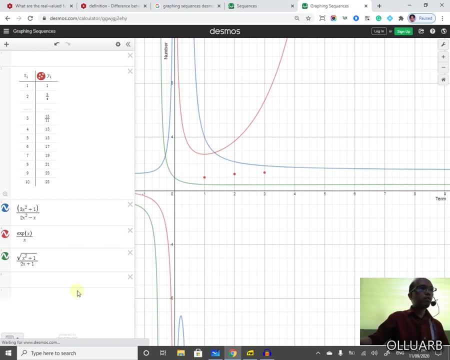 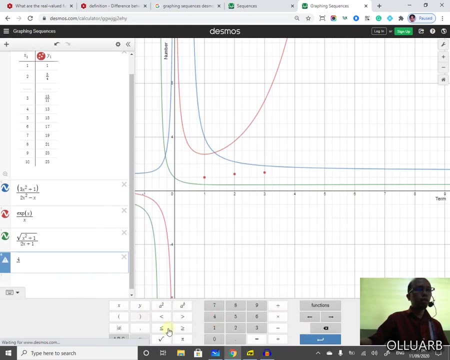 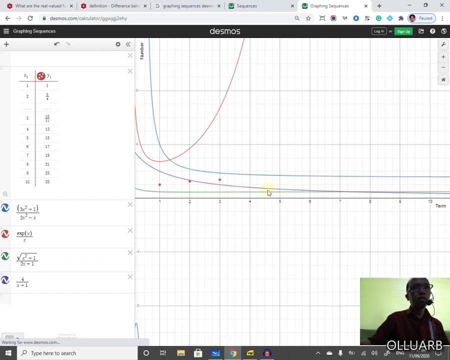 okay. so, as you can see, if we graph this one using this moth again, 4 over n plus 1, 4 divided by n, X plus 1, X plus 1, the violate. okay, as you can see, this one is decreasing. okay, so we expect that it is decreasing. so meaning to say: notice the. 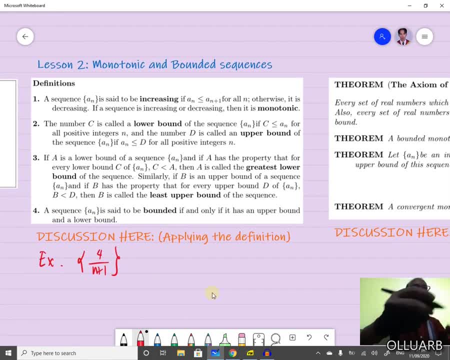 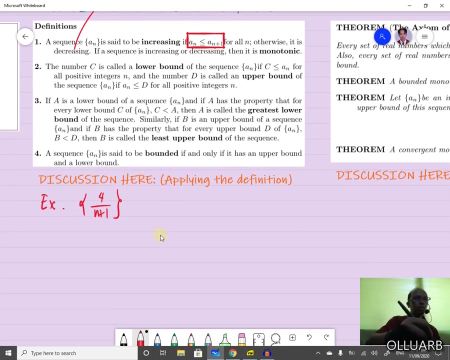 down the definition of increasing function. this one I'm going to. no, sorry. Y こちら es para tab track. how about? if this one is decreasing, okay, so it's reverse. okay, this is the. this is for decreasing. okay, so, since it is decreasing based on the graph, the violet one, so let's try to solve this, okay? solution. 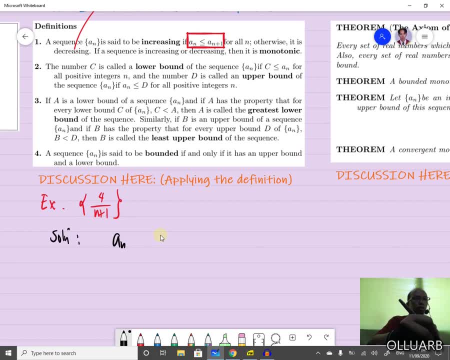 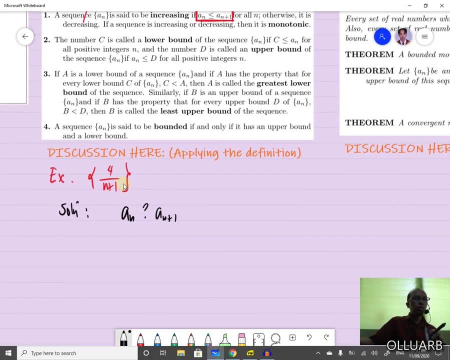 we have an we don't know, but in the graph we know that it is decreasing. so we don't know. and this one and plug in. so this is our an, this is our an, this is our en. an is four over n plus one. so this is four over n plus one question mark. 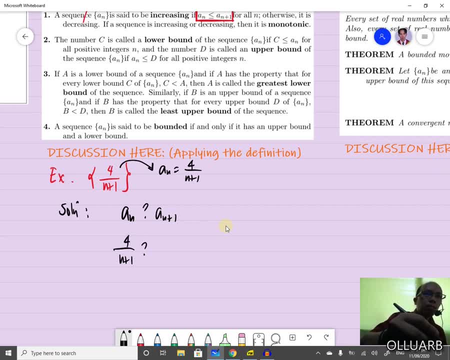 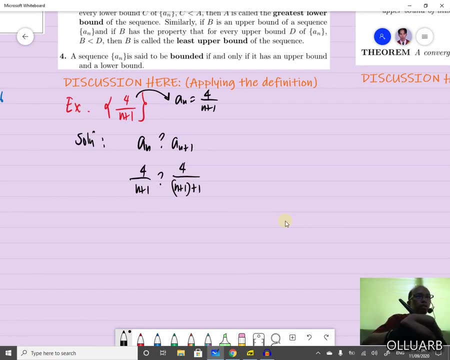 so remember that if n, if we replace, if we replace n by n plus one, we have four over n plus one plus one. okay, and then cross multiply. we have simplify: first n plus one, four over n plus two, so cross multiply one, cross multiply, so we have four. 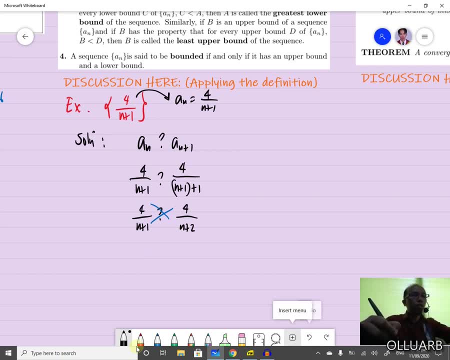 Stat hela N plus four, sorry, N plus two. Question Mark four n plus one. this is four n plus eight, four n plus four. so if you have a number we can pencil out this one. we have eight question mark four and clearly, of course, whenronof3d was set to zero. 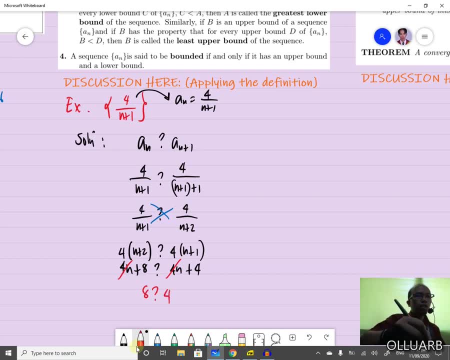 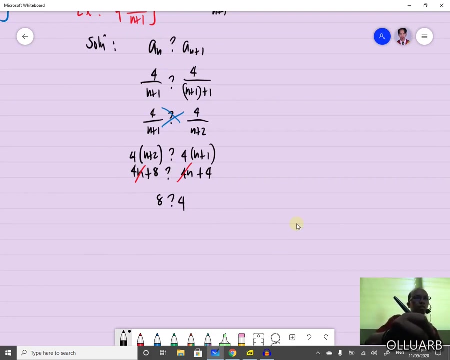 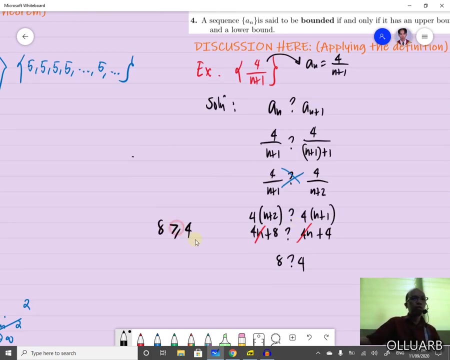 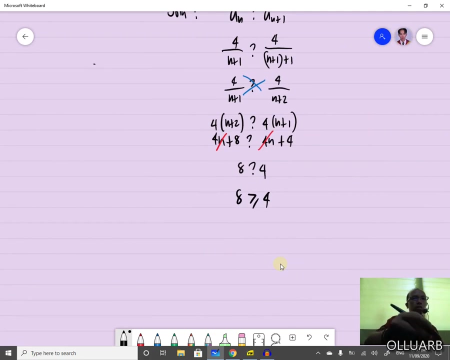 so you notice, we can cancel out this one. we have eight question mark four and clearly 8 question mark and clearly 8 is greater than 4. okay, so this is therefore a n is greater than a n plus 1, therefore the sequence 4 over n. 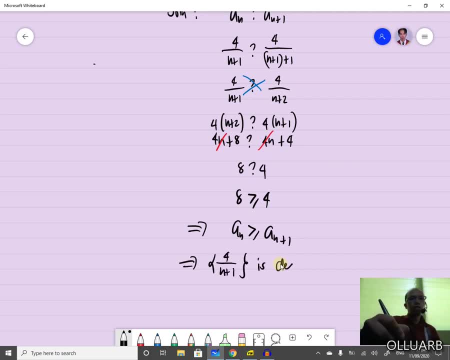 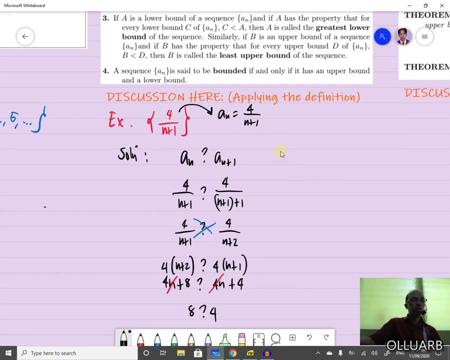 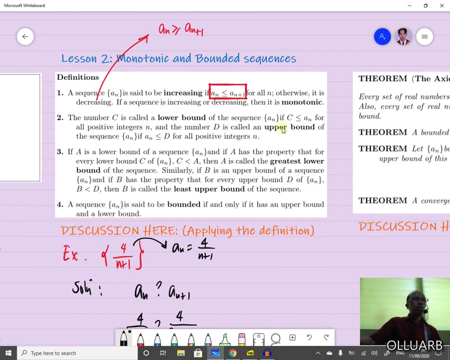 plus 1 is decreasing. okay, oops, okay. so the function 4 over n plus 1 is a example of a decreasing function. so what do we mean by a monotonic sequence? it says here: if a function is increasing or decreasing- so remember the conjunction here- or so either. so if it is increasing, either increasing or. 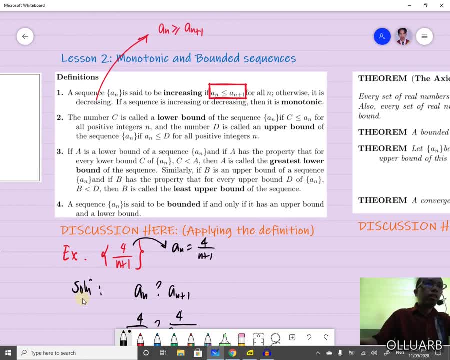 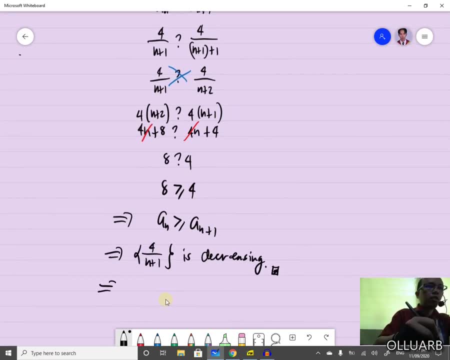 decreasing, then it is monotonic. so, meaning to say this example for the sequence four over n plus one is a monotonic. therefore, four over n plus one is a monotonic, monotonic sequence since my definition. if the function is increasing or decreasing, then it is a monotonic sequence. 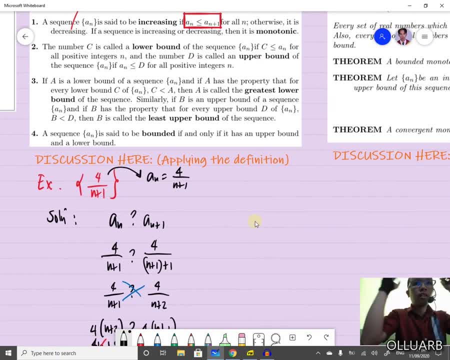 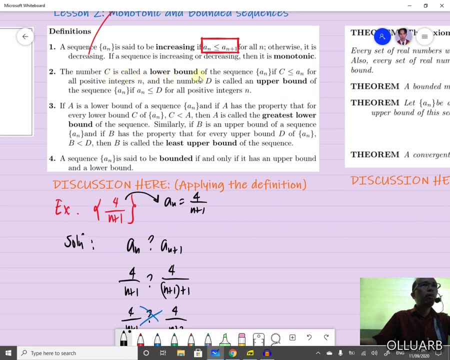 then it is monotonic, okay. so number two definition. number two, uh, definition about lower bound and upper bound, which is very easy to understand. the number c is called a lower bound of the sequence a- n if all of its term is this number. here you have to pick this number. 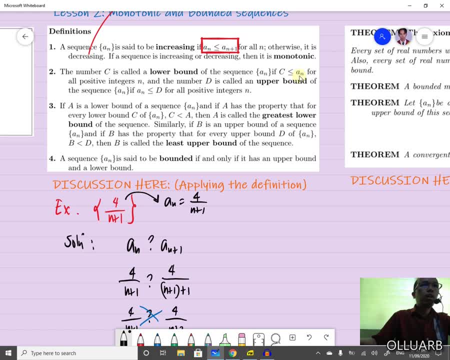 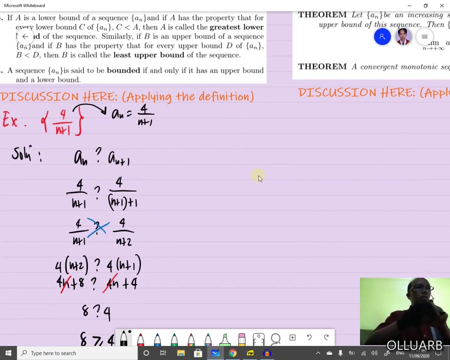 isotherm, equal to every elements of the sequence, for all positive integer n. and the number d is called the lower bar, upper bound. sorry of the sequence if it is bounded above, this number d is greater than all the elements of the sequence, for all positive integers n. so, for example, this one, the sequence as you can. 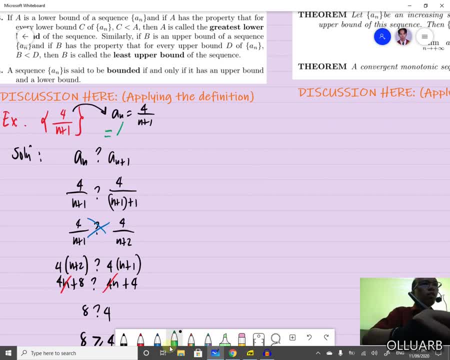 see. so our first element is 1, 2, 2 and then 4 divided by 2. how about 2 is 3, 4. thirds, if 3, 1, 1, 2, 3, 4, 4 over 5, my right, yes. if 6, if 1, 2, 3, 4, 5, 4 over 6, 4 over 6 is 2. 3rd and so: 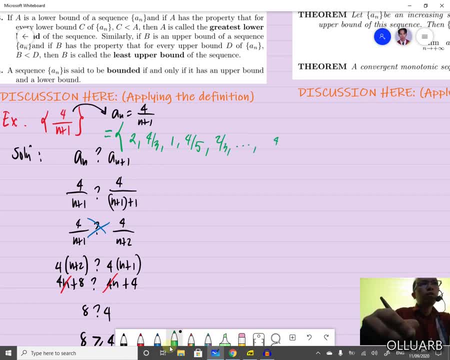 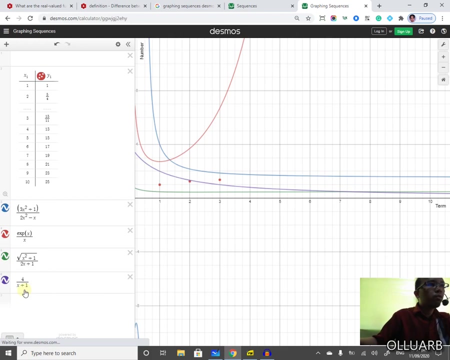 on so forth. this is 4 over n plus 1 and, as you can see, this sequence has a limit and it is decreasing, and the limit of this sequence is 1 half my right one half. let's look at the graph. I remember it correct: 1, 2, 3. 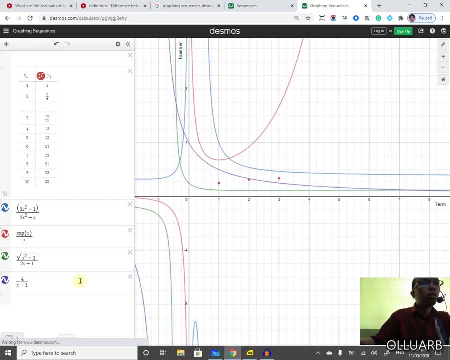 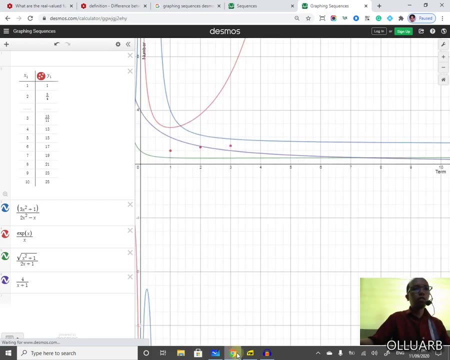 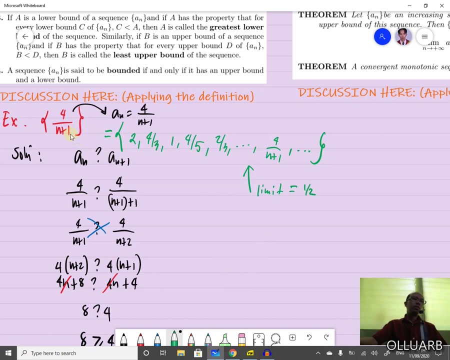 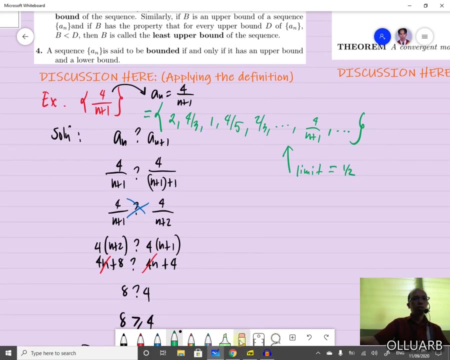 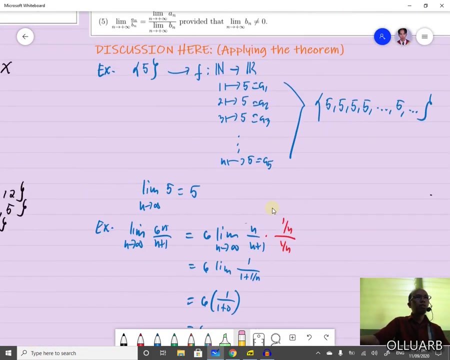 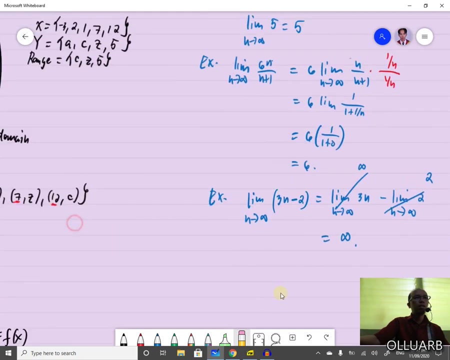 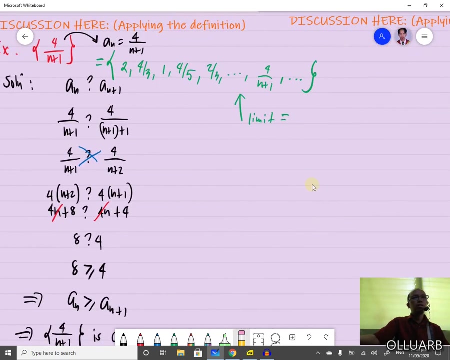 0 0 0 0 0 0. ok, is it one half? yes, 1 0 0 0. is it zero? I'm sorry, did we solve this problem before? where is that? where is that? where is that? anyway? I forgot, so let's try to solve it. 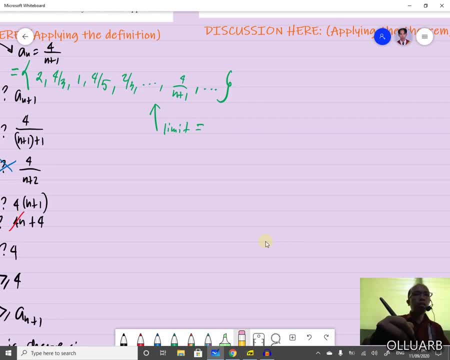 what is the limit? the limit of this function n approaches to infinity. so i said: n approaches to infinity, so n approaches to infinity. so so you have 4 limit of 1 over n plus 1, so this is zero, i guess. okay, zero. so, as you have noticed, 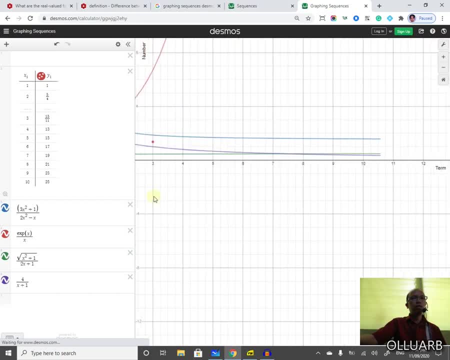 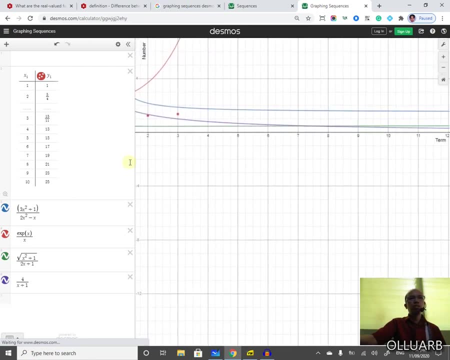 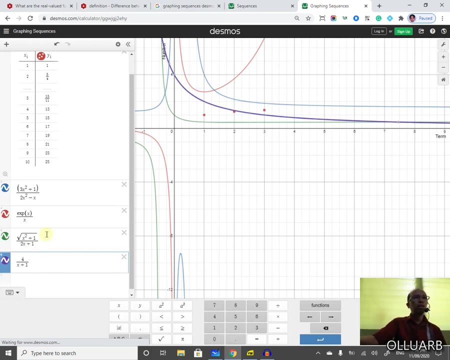 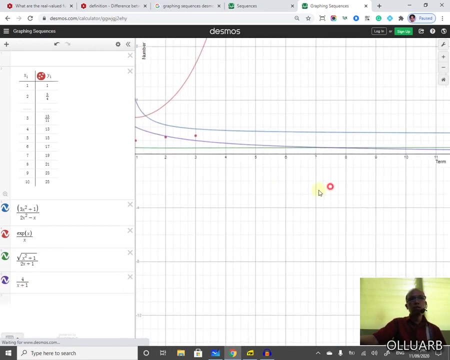 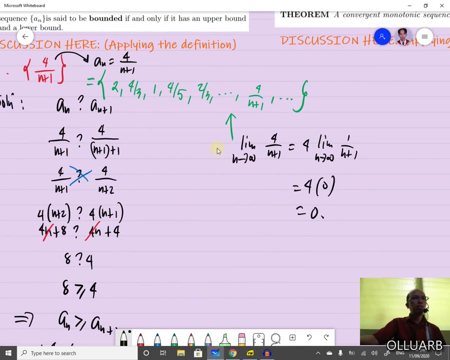 if you look at the graph, it approaches to zero, as i said, and approaches to infinity. okay, i'm sorry, i mistaken before. i thought it was the green one, but i think it is the violet one, that's why i mistaken. okay, so the limit is zero. so it is decreasing and the limit is zero. 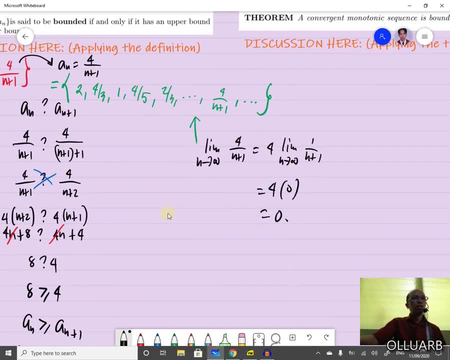 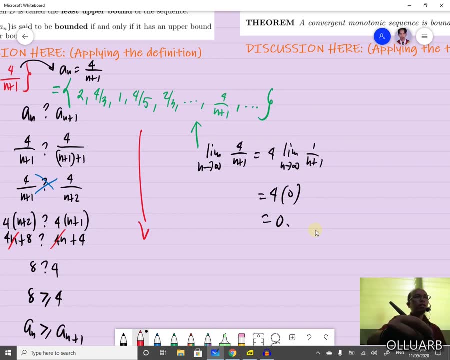 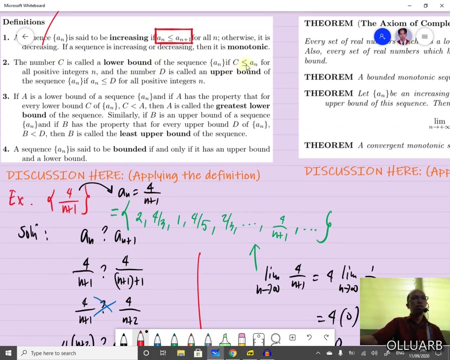 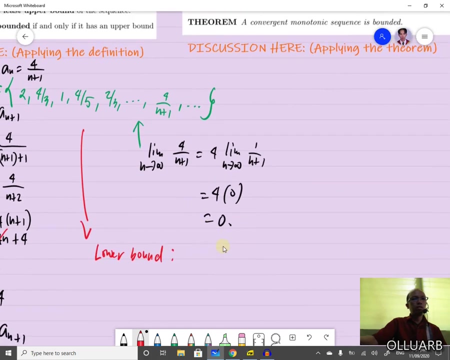 so meaning to say, for this sequence: okay, these are the lower bound. lower bound is c's here. c's here that the lower bound is a number c. it could be less than or equal to the element. so you can. you can. it could be zero, it could be negative one or negative two, and so on and so forth. 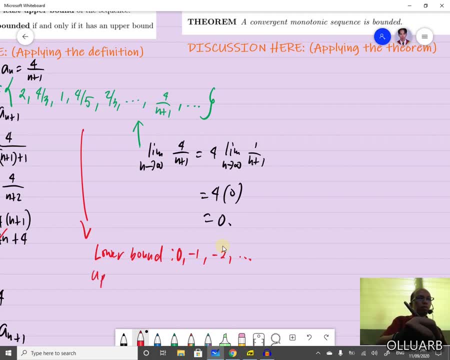 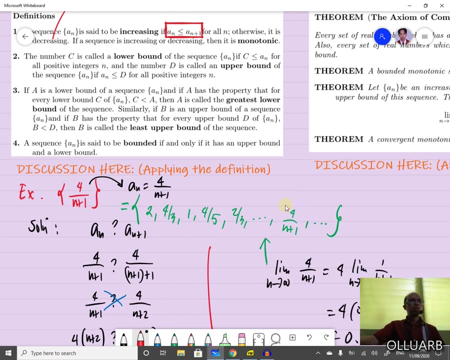 okay, but the upper bound, upper bound is here, as you can see, you can have two, three, four and so on and so forth. okay, so there can be, there can have two, three, four and so forth. you know, okay, their numbers. they refer to a, for an example. 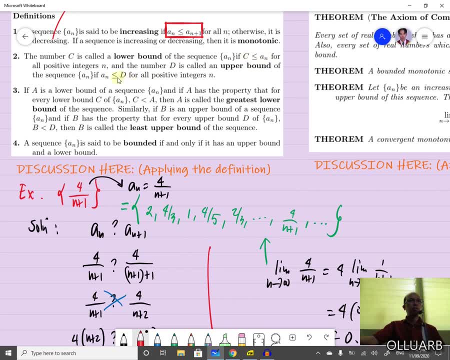 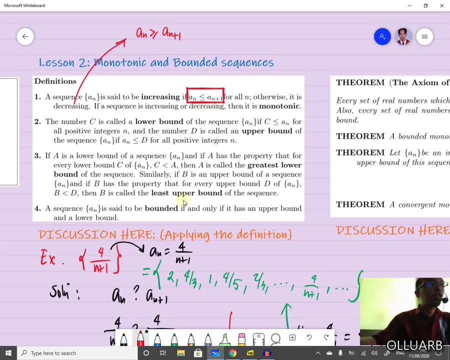 if it is higher bound or lower bound. so again you can choose a number because, yeah, there is no difference in terms of strength if it is hessian. so a can be mais stable for number. but for the number three, maybe a is unhappy. Comme là that for every lower bound c of the sequence this inequality is true, then a is called the. 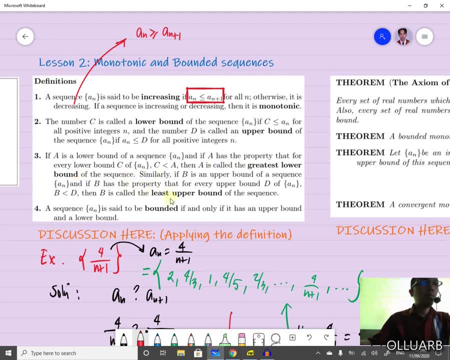 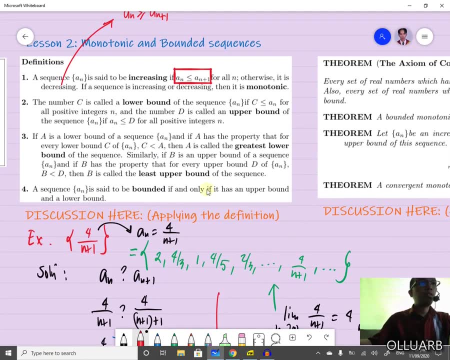 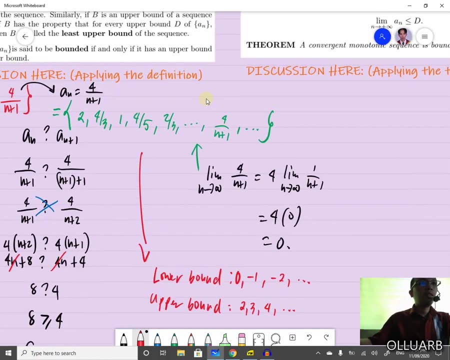 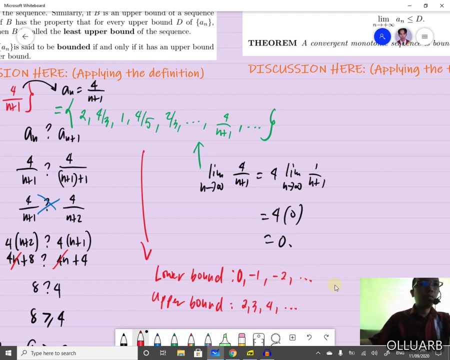 greatest lower bound and similarly the upper bound is defined as that. so meaning to say: if, uh, example this one, these are a's, our a's, these are the lower bounds- zero, negative one, negative two and so negative three could be our lower bound. it says here: if that, if that's our a. 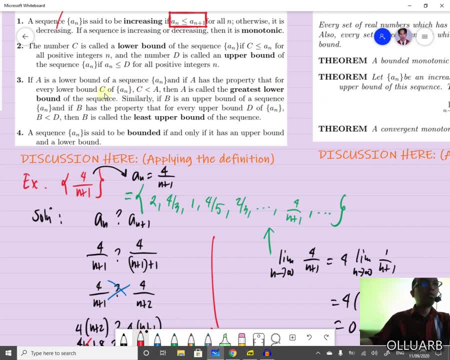 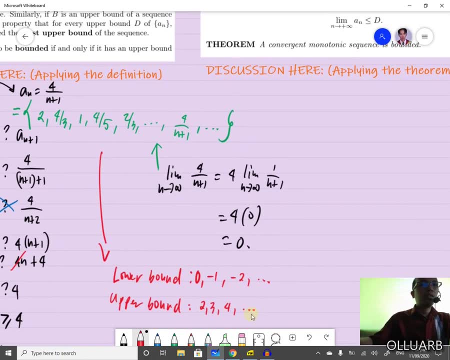 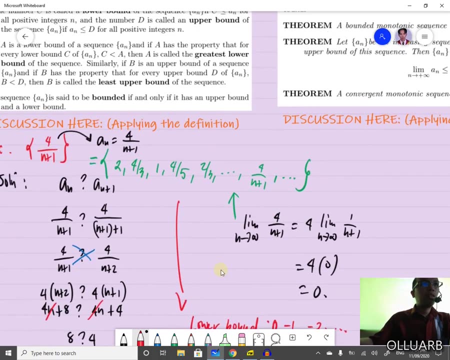 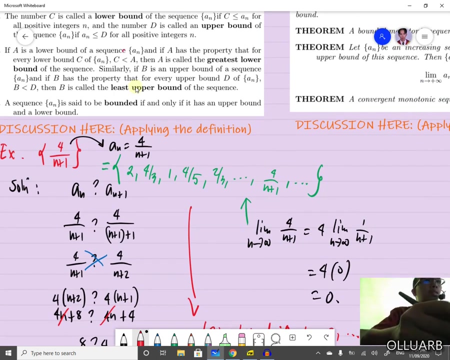 and if a has the property that every lower bound c. okay, so you can choose a or c here to be this one, but what is the exact uh inequality here is that this will follow. it must be. i'm sorry, but this is less than or equal, and also this one less than or equal. 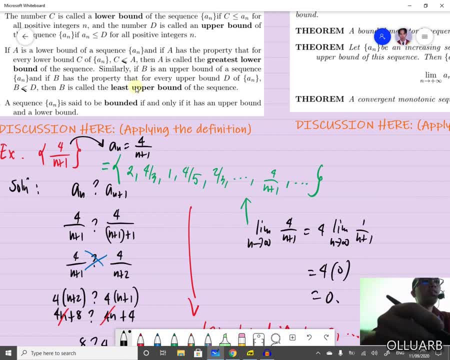 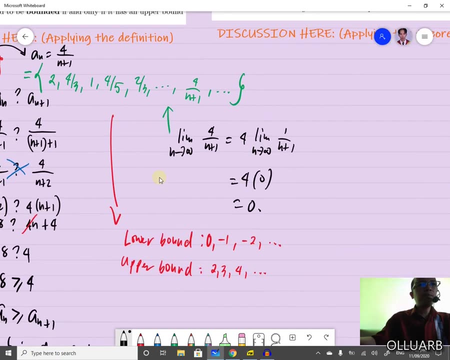 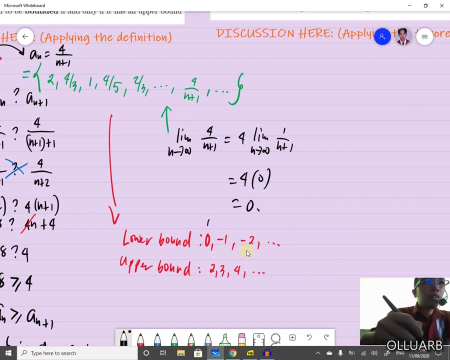 okay. so when you say there are many lower bounds, but the greatest of all those, uh, lower bounds is what we call the greatest lower bound, then that a will be our greatest lower bound. for example, this one: the greatest of this lower bound is this one. our greatest is this one: zero. so this is our greatest lower bound. or g m b. okay, because if this 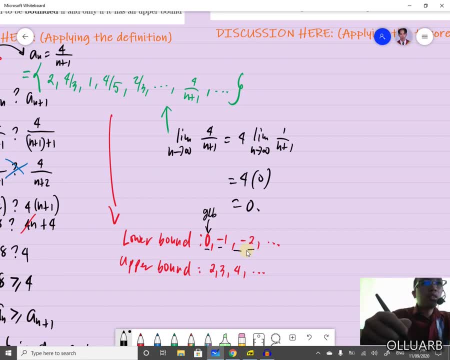 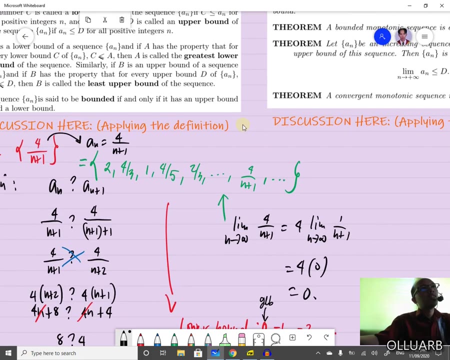 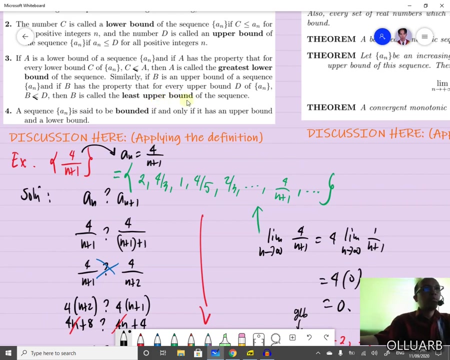 is our c- c. there are many c's here. this is the greatest of all the lower bounds. similarly for the upper bound. um, okay, for the upper bound, there are many upper bounds, but the least of those upper bounds is what we call the least upper bound. so, for example, 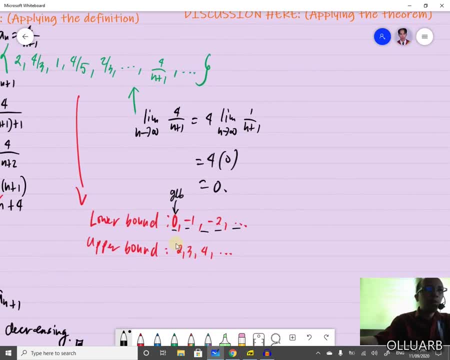 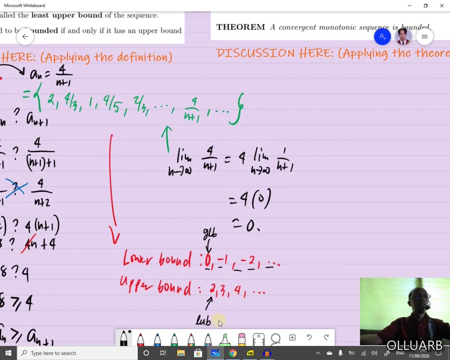 this one. these are our upper bound, but the least is to this one, so this is our least upper bound, okay, so notice that the upper bound and lower bound could be an element of the set, but for this example, the lower bound, zero, is not an element of this set. again example, and: 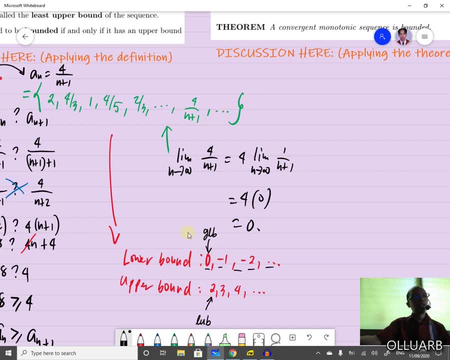 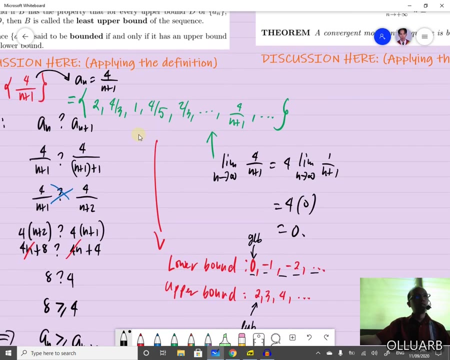 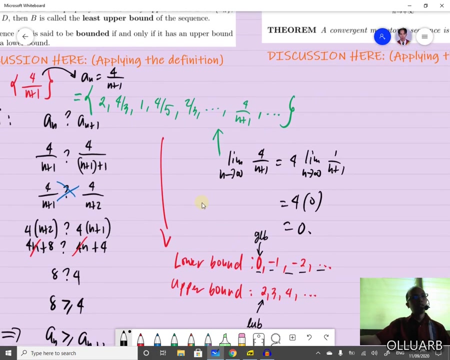 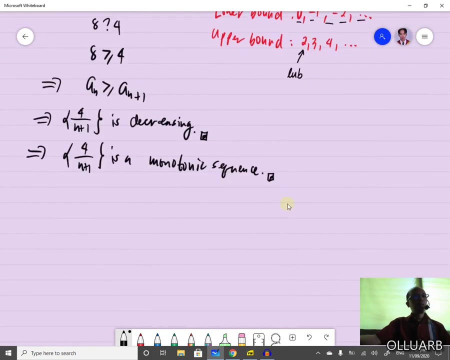 the example zero is not an element of this set. okay, the example zero is a greatest lower bound of this set, of this sequence: 4 over n plus 1. okay, that's the meaning of the lower bound and the upper bound. so another example, if you have, how about? 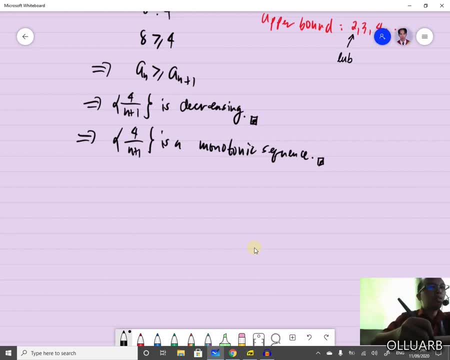 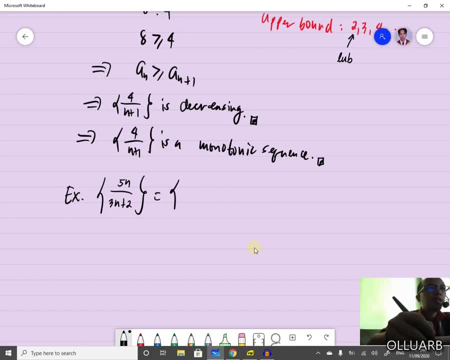 sequence 5n over 3n. the elements of the sequence are the following: so 5- 1. so of the sequence 5n over 3n, the elements of the sequence are the following: so 5, 1. so of the sequence 5n over 3n. the elements of the sequence are the following: so 5, 1. so this is 1. the first limit is 1. 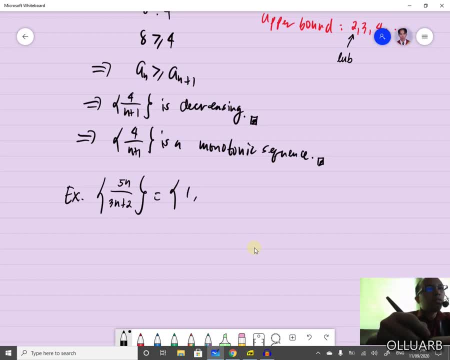 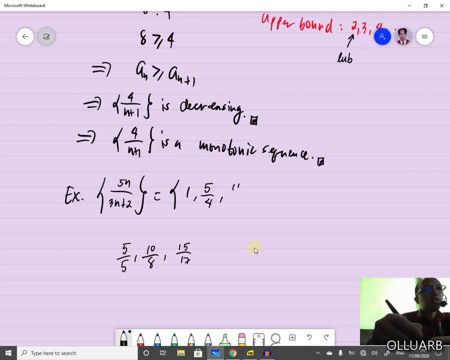 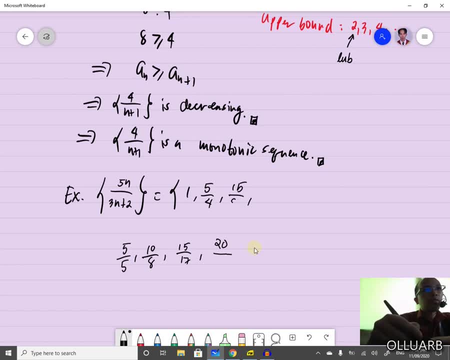 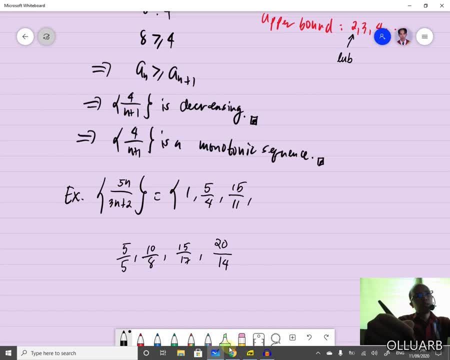 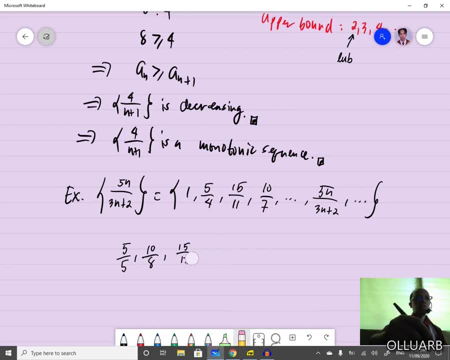 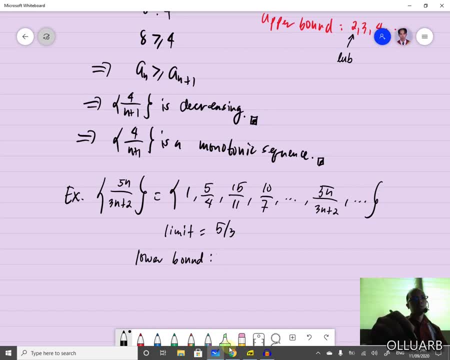 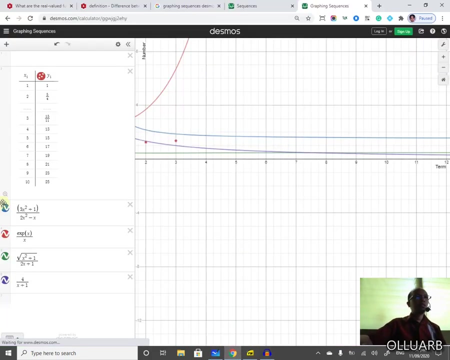 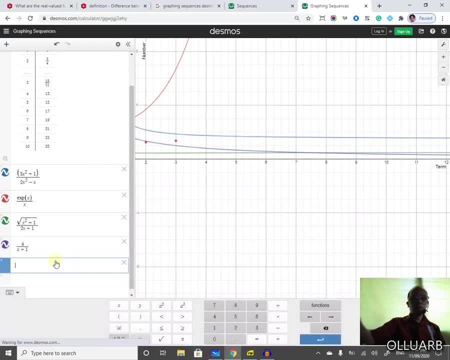 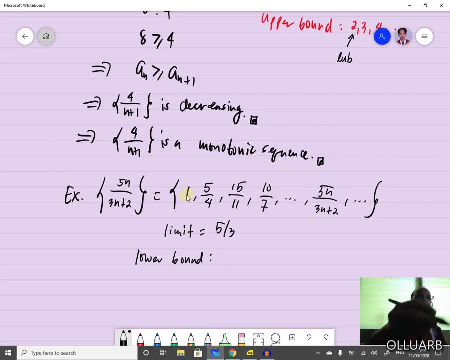 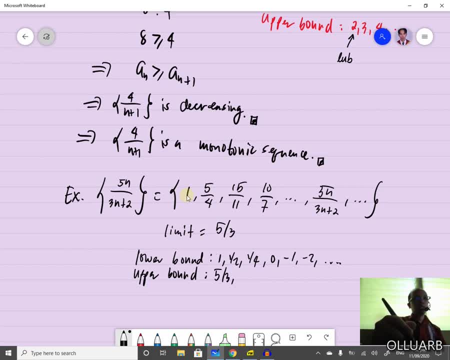 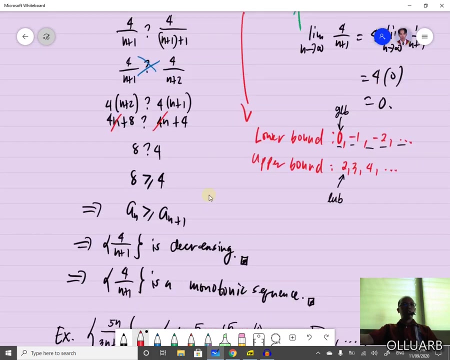 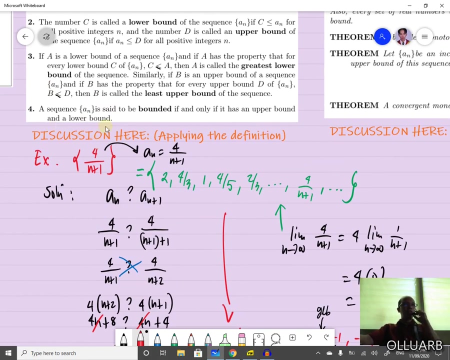 uh, greater than five thirds. we have two, three, four and so on, but what is our greatest lower bound? so the greatest would be this one greatest lower bound, and this is our least, will be our least least upper bound, luv, okay, okay, let's go back to definition number four. a sequence, an is said to be bounded if. 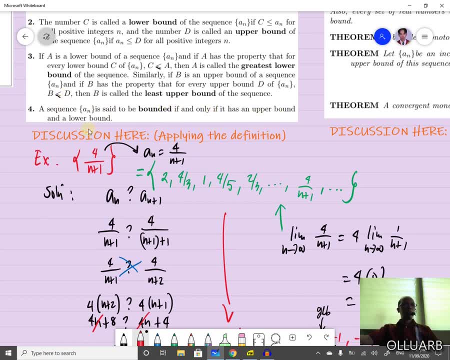 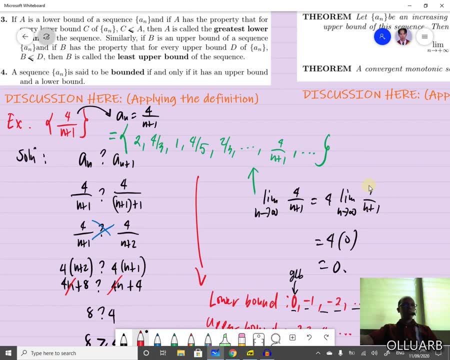 a. it has an upper bound and a lower bound. so, as you can see, as you can see here these two examples, is an example of a bounded sequence. okay, this is a bounded sequence because it has an upper bound and a lower bound, and look at the definition. it doesn't mean that it says: 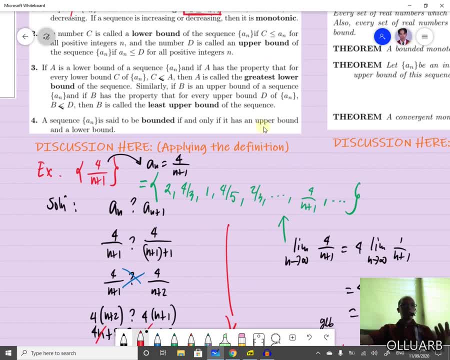 a greatest lower bound or a least upper bound. but it says it has an upper bound and a lower bound. so if the sequence is an upper bound or lower bound, then that sequence is bounded. so this example: four over sequence, four over n plus one. and okay, below the sequence, five: n over three, n plus two. 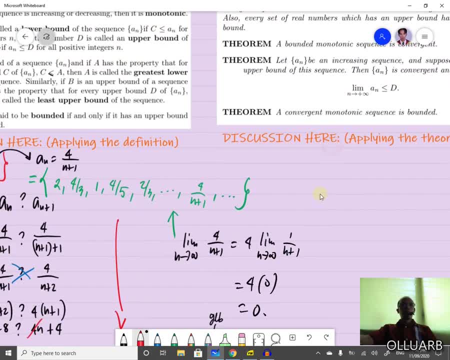 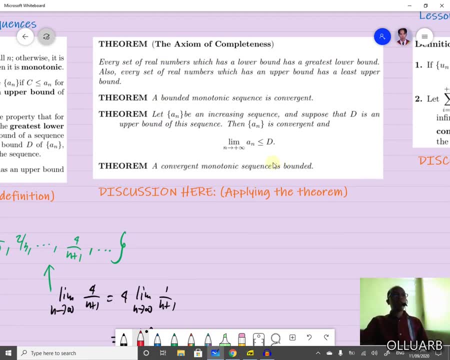 is an example of a sequence which is a bounded sequence. okay, let's have this theorem during the action of completeness. this is a very uh, familiar theorem in mathematics. uh, every set of real numbers which has a lower bound has a greatest lower bound. so if the, if it has an upper bound, then the sequence has a least upper bound, and that's what it's said by. 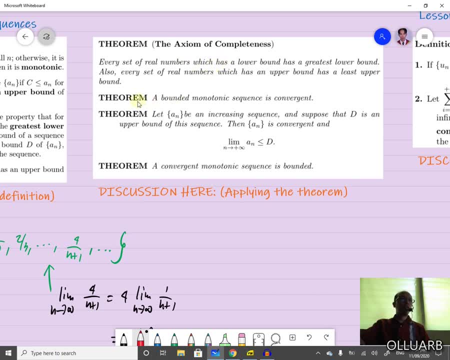 the theorem, the option of completeness for this theorem- bounded sequence, a bounded monotonic sequence- is convergent. so what does it mean? so we need to say, when you say monotonic, it is increasing or decreasing, since it is bounded, so it has an upper bound or and a lower bound. so meaning to, 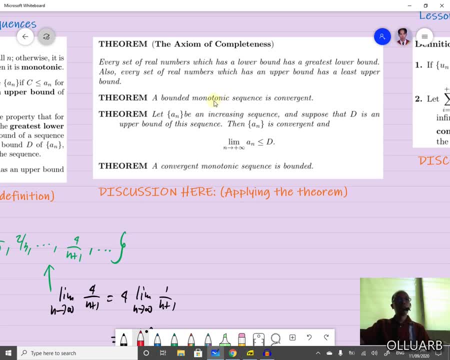 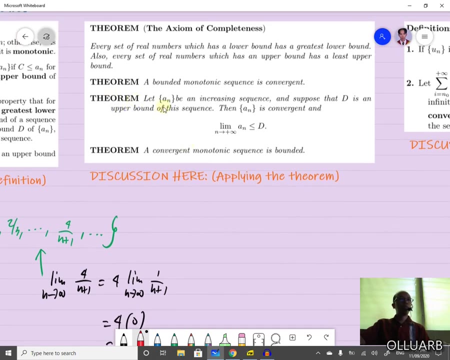 say, if that sequence is, if the sequence is monotonic and at the same time is bounded, then it is convergent, to mean it has a limit. and for this theorem, third theorem, if you have, you are given a sequence which is increasing and suppose that this, and it is an upper bound, the sequence, then the sequence is: